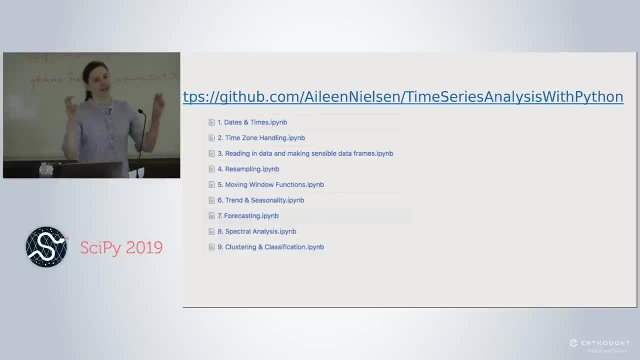 So I'm just going to give you a couple of slides about how we've been working with time series professionally. Even though those methods are sort of low tech or less modern, they are very much relevant today. They still perform exceptionally well and they also give you a really good conceptual foundation. 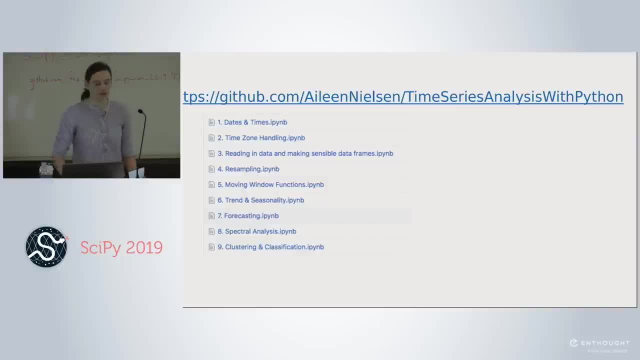 And similarly it's good to be comfortable with data cleaning of time series and all of that. So that's a little bit about me. I'm also just a little bit curious about people in this room, So I guess I'll just do a quick survey. 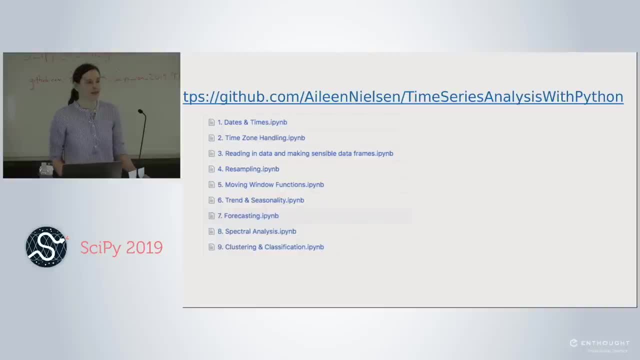 a show of hands. If you already work with time series data at work, Okay, I hope there will still be stuff for you, If not no hard feelings- And you can certainly pipe in with your own suggestions and input as well. And how many people have never worked with time series data? 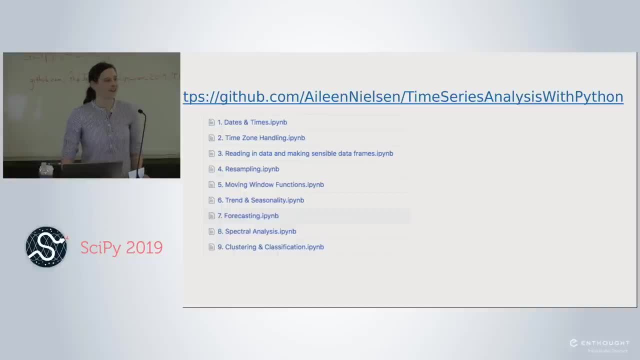 Okay. Or very limited. How about very limited? Okay, Fair enough. And how many people work in a scientific sector broadly defined? Okay. And how many people don't work in something you would call remotely scientific? Okay, Fair enough. 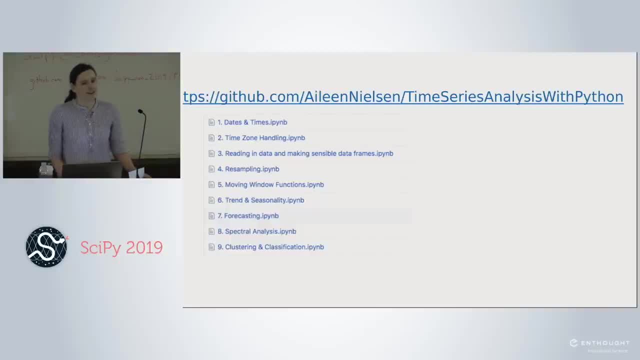 So good for me to know. And then, just out of curiosity, who thinks they came the farthest to get here? Singapore. Can anybody beat Singapore? That's really tough. Yeah, that's okay. There was someone on my flight who claimed they'd been traveling for two days. 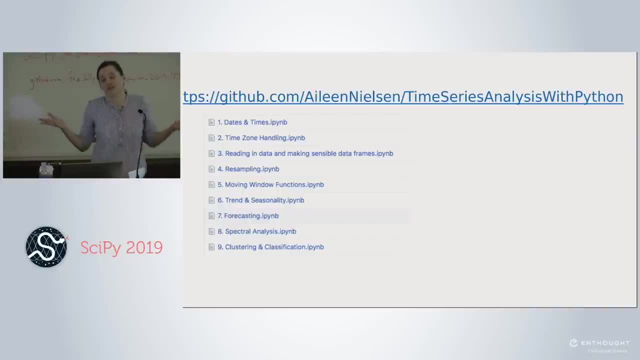 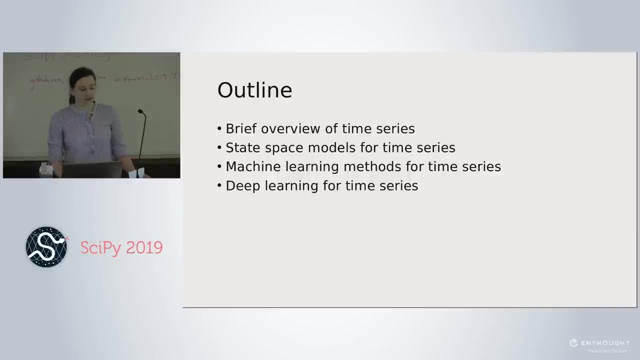 but they didn't come to this conference. They might have you beat them as far as like time or whatever. Okay, Okay. So here's an outline of what we're going to be talking about, Just a very brief overview of sort of what makes time series data special. 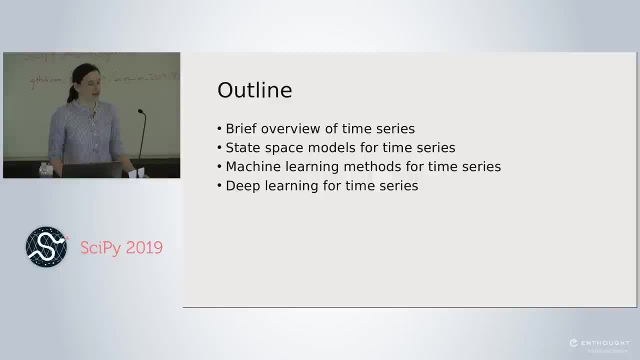 some things you want to keep in your head when you're looking at time series data, especially if you're new to it or haven't worked with it for a while. And then we're going to divide our discussion into three components. We're going to be looking at state space models for time series. 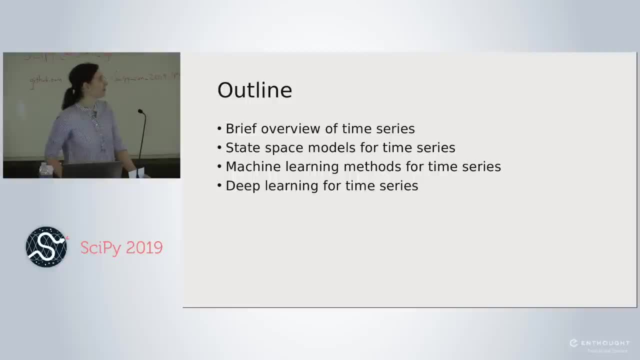 just an overview of what those are, And we're going to cover two methods specific to state space methods. We're going to talk a bit about the time series model and then we're going to talk about applying traditional machine learning methods specifically for time series and what approaches you can take there and what you want to look out for. 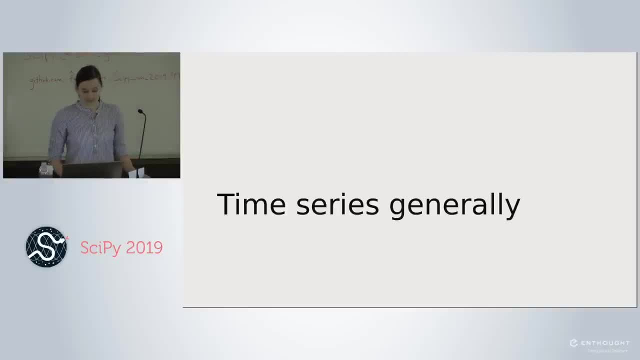 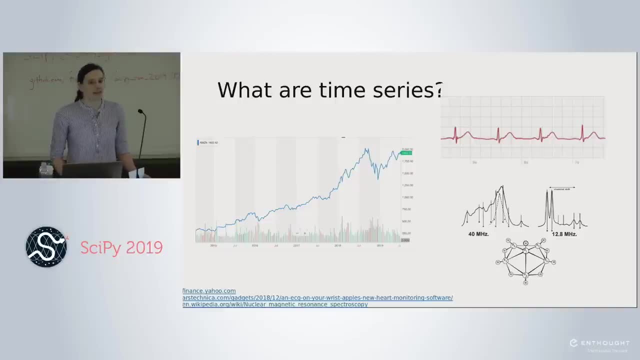 And we're going to wrap up looking at some deep learning for time series. Okay, So time series generally. What are time series? It seems like everybody has a good idea of what those are, given that you work with them, right. So the classic example: I think in every time series book, almost always, you will run into many 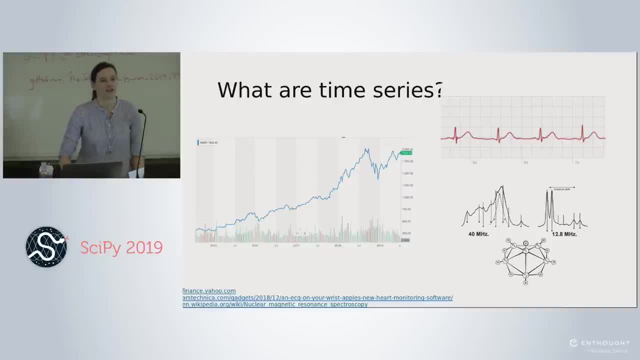 many examples of something like stock prices There are readily available, usually free, fairly chaotic time series, So they're really interesting to look at, And of course nobody is all that good at modeling them, because if they were they'd be filthy rich. 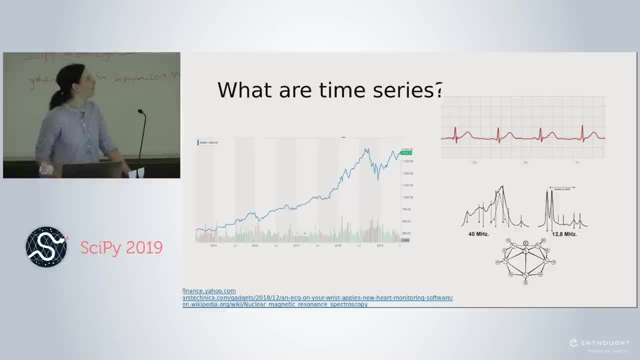 So it remains sort of an open problem, which is also interesting. But I want to point out that many other things are time series that don't get called time series and even get analyzed in their respective disciplines without anyone using that word, even though that's what they are. 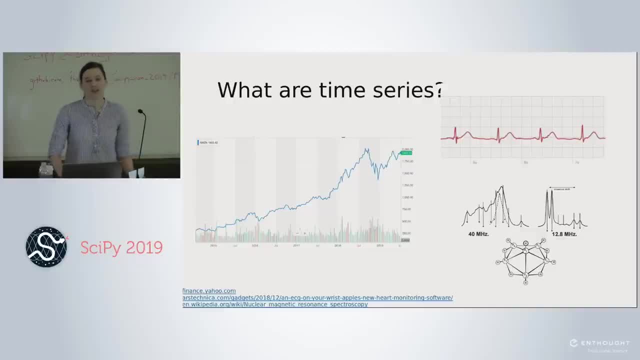 So on the upper right-hand corner of this slide I have an EKS diagram, which is an EGS diagram. I've never heard a doctor talk about time series data, but actually that's often what they're looking at, right, They are taking some sort of measurement over time. 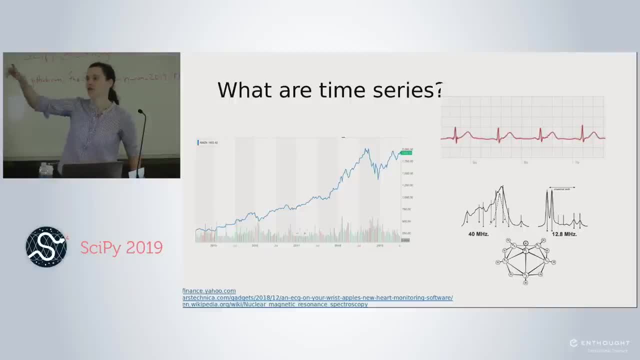 When you're hooked up to any device in the hospital, it has some kind of digital or analog curve, That's a time series right. So I think data science or time series analysis, or whatever you want to call it, has a lot to contribute. 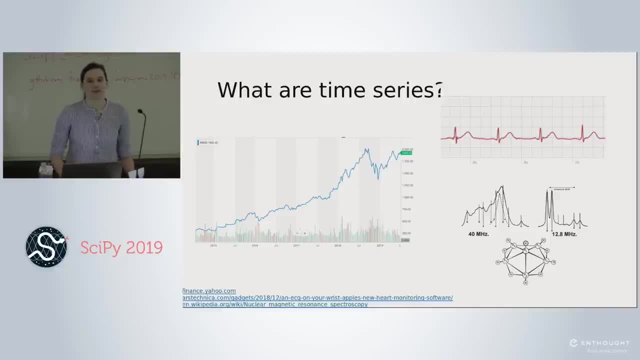 to this field, and while we keep hearing about the benefits of healthcare for data science or deep learning, we don't hear about it so much in the time series context, even though there's actually a lot of time series data in the health field, as well as many others. 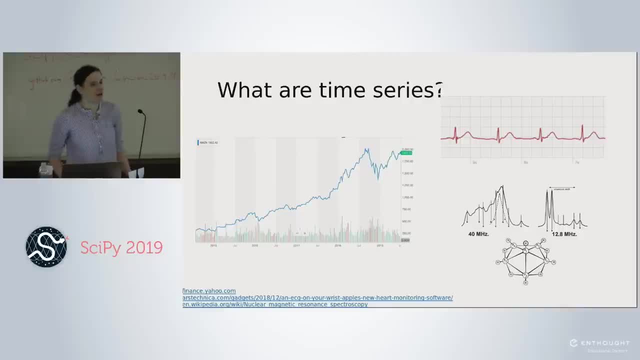 Similarly on the bottom. I think this is an NMR, but I might be wrong if a chemist wants to correct me and tell me this is some other kind of spectroscopy. But this is some kind of NMR looking at molecular structure, right? 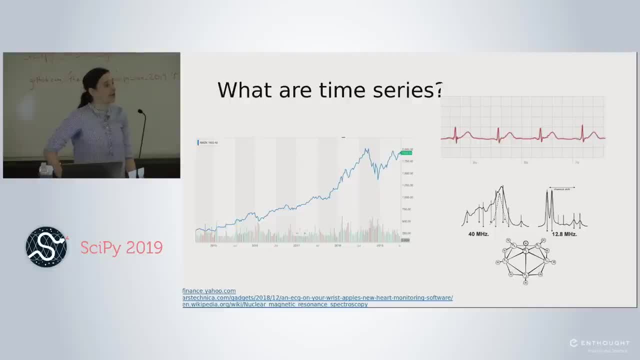 This is also a time series by my definition, even though here the x-axis is not time, It's actually just wavelength. Got it, Thank you, Because you can use many of the same methods on it, and what you have is: you have a well-ordered, well-spaced temporal axis. 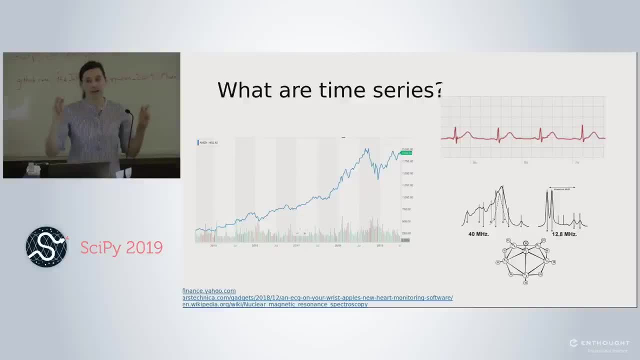 So we are even going to be working with some data today where your temporal axis is not time per se, but it's something with this sort of well-ordered metric between different points in time, right? So that's what makes time series different from anything that's cross-sectional analysis. 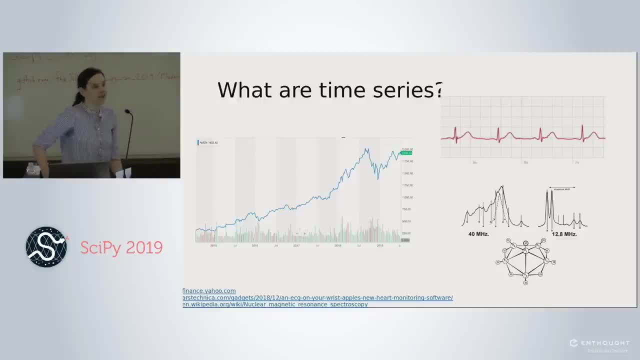 And here's an example. So what might I do with something like that? If I don't have time as an axis, am I really going to do prediction? Well, probably not. right Prediction might not be the most useful thing, although maybe you can contrive an example. 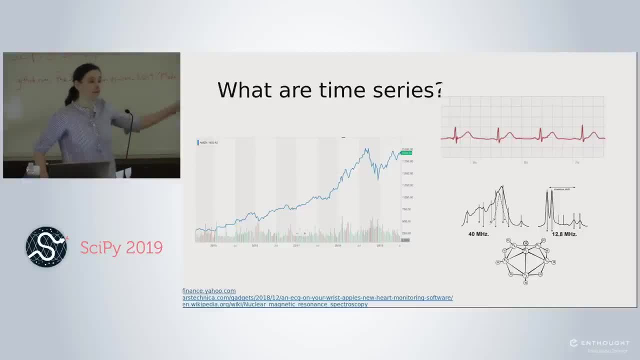 But you can certainly do something like time series clustering, right. You might have multiple NMR spectra and you want to find a way to classify them without having hundreds of grad students slaving over it, right. If you can find a way to replace those grad students, even better. 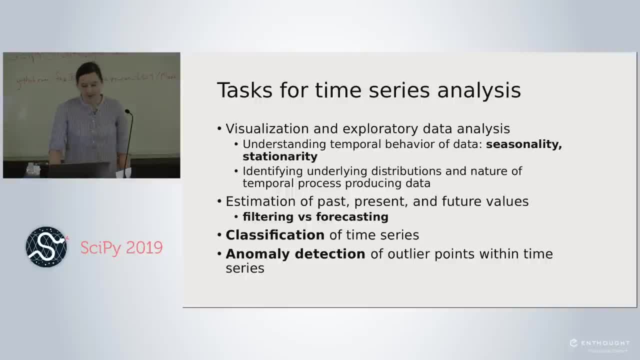 Okay, So tasks for time series analysis. What are things people do Well as usual? visualization And exploratory data analysis. When you do this for time series, often you have specific time-related temporal questions, such as understanding the temporal behavior of the data. 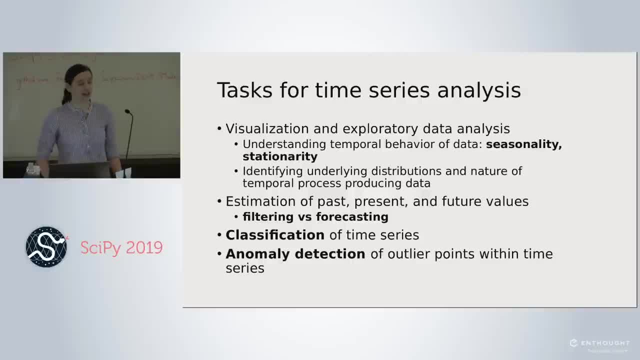 especially if your time axis is actually a time axis such as seasonality, right? Is there some kind of recurrence in your data, some kind of seasonality? You can also look for cyclical data- not quite the same as seasonal data, right? 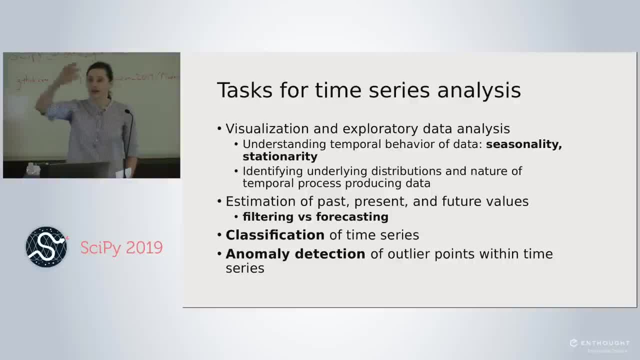 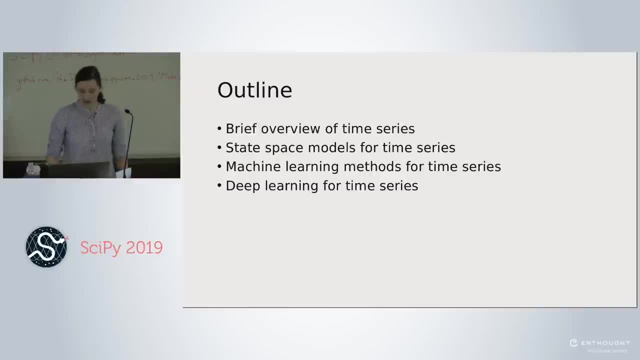 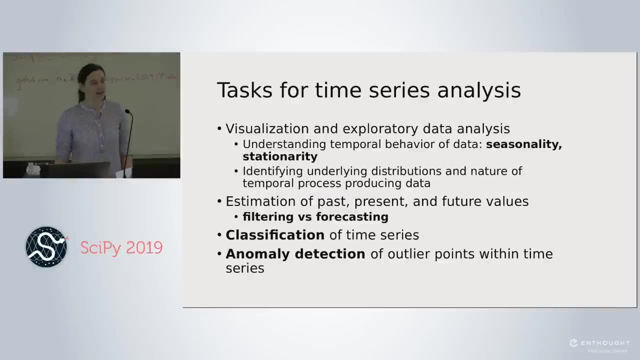 So cyclical data will have some sort of recurrence, but it can be damped and it can also sort of change its period over time. So an example of seasonal would be something like the weather and an example of cyclical would be something like people hypothesize. there's a business cycle, right? 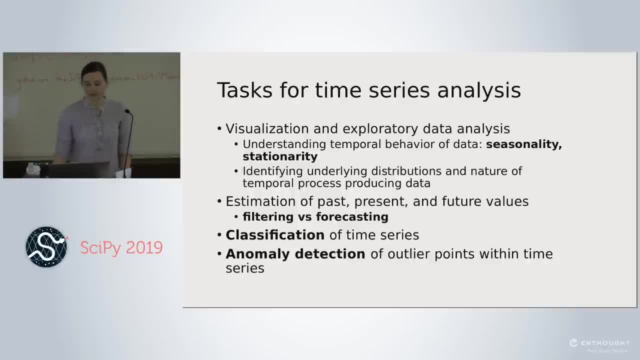 Some sort of boom and bust cycle in banking or stock prices, that sort of thing. And what's another thing we usually want to do is sort of identify underlying distributions and the nature of the temporal processes producing the data right. We want to get a sense of 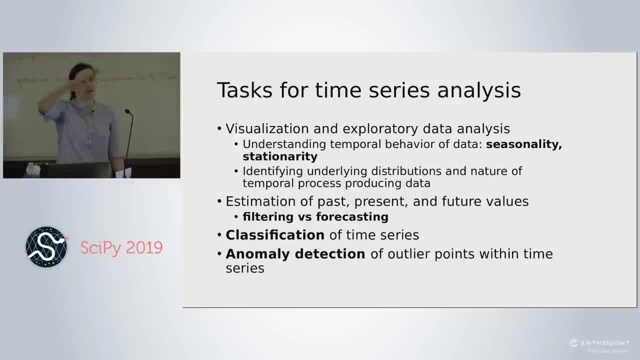 I have a hypothesis that I see this sort of river level over time and I want to get at sort of what describes that river level more fundamentally. That's another thing I might want to do: not just predict, but also have a way of describing the dynamics. 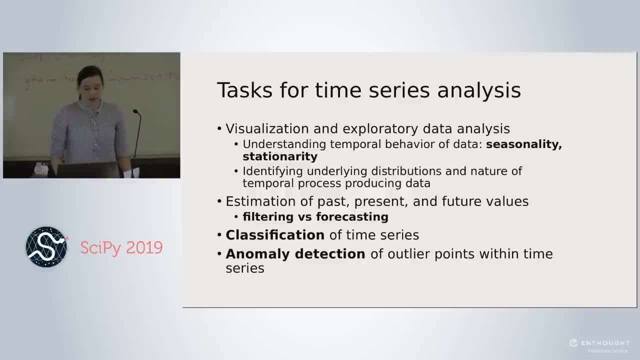 What else do we need to do? Well, we can do estimation of past, present and future values, right. So there's also this distinction between, say, something like filtering and forecasting, or also smoothing. We'll talk about all of that in the context of state space, but the idea is: 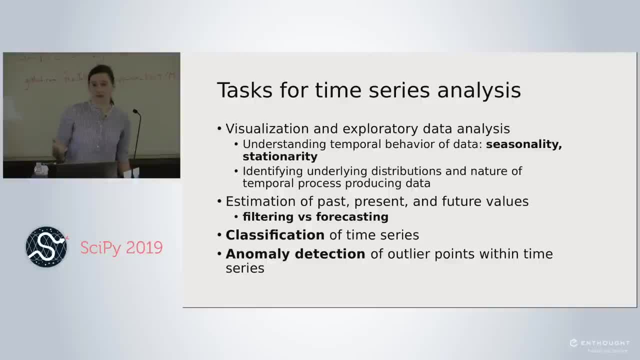 if you have noisy measurements- and you can think of all sorts of things as noisy measurements, such as stock prices, where maybe you think the market got it wrong and there's a real price that's separate from what the market says. or it could be a medical sensor that has some sort of known plus or minus. 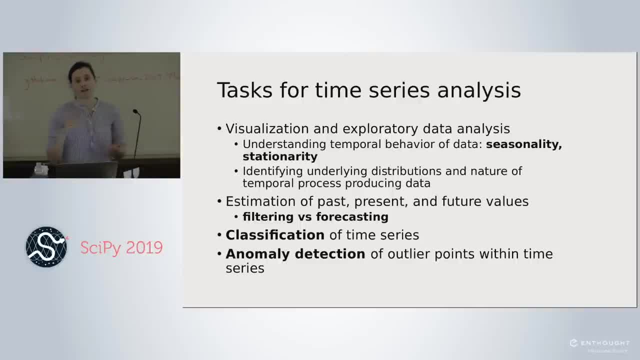 So, let's say, even if you measure your blood sugar within a minute on the same device, you will still have, you know, a 5% discrepancy, And that's something that's actually accepted by the FDA right now for devices used by people with diabetes. 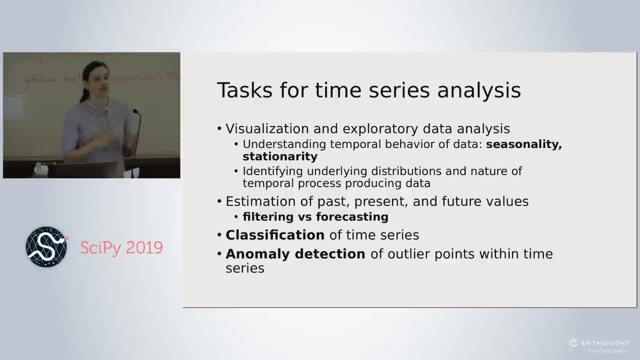 So there's an example of: you know you can't get it perfect, and so you could have a time series with just lots of measurement error. So you can have tasks of figuring out. well, what was the true value at all these time steps right? 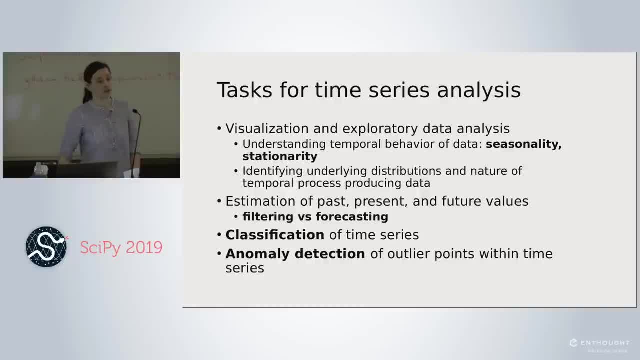 There was a value I measured versus the value that is actually true, and is there a way of getting at that? Next up classification: That's another common time series task. This could be both in something like the medical field, right? Can I classify what kind of EKG I'm looking at? 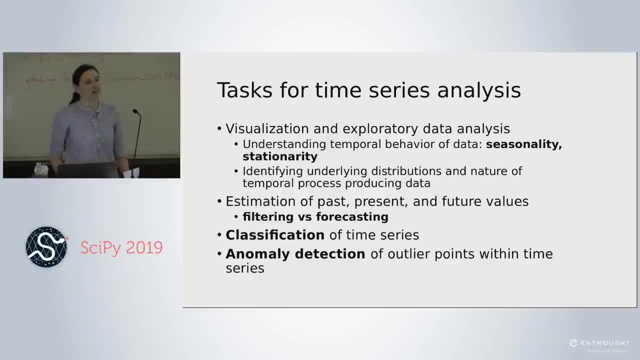 Is this showing me normal heart or some kind of arrhythmia? This could be classification of NMR spectra, like we talked about. This could be classification of retail behavior. Do we have sort of distinctive trajectories through our website, right? Things like that can also be time series analysis. 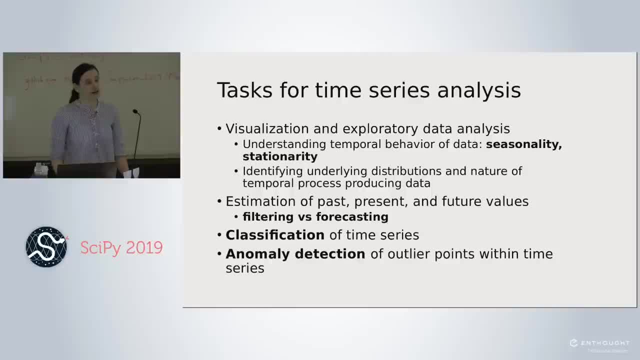 And then another major task is anomaly detection. right, Can we figure out which points are the problematic points? right, And the better we can do that, the less often, say, a bank will have to cancel credit cards or a doctor will have to run tests. 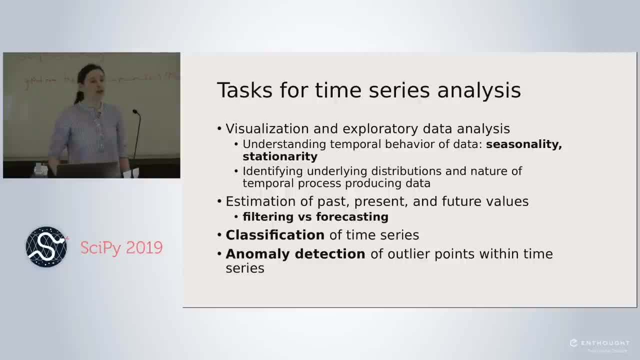 that weren't really necessary versus run the ones that we really need. We don't always think of these things as time series analysis, but increasingly we have panel data for all these things right, Increasingly for things we think of as cross-sectional data right. 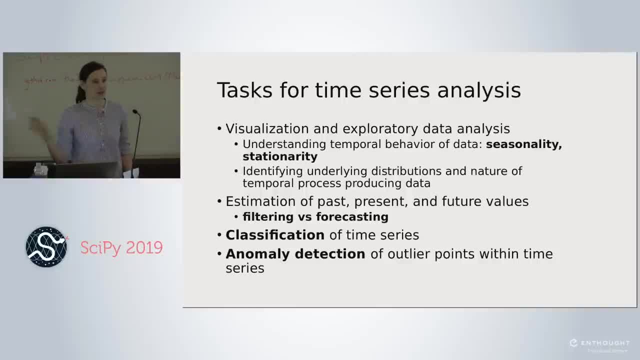 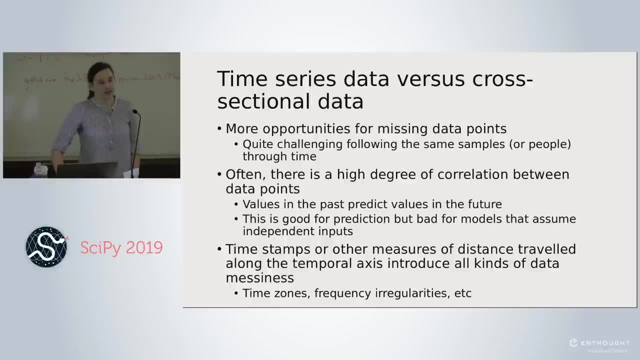 Surveys or whatever, we're better able to track people, and so we have a sense of how things are evolving over time. Okay, Time series data versus cross-sectional data. What are some of the challenges or things to keep in mind? Well, number one: there's more opportunities for missing data points. 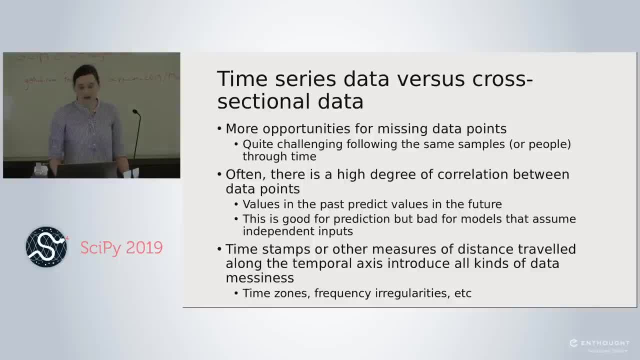 It can be quite challenging following the same people or even samples over time, and I imagine anyone who has worked especially in sort of human-related sciences knows about this problem right. Good luck finding the same survey respondents year in and year out. 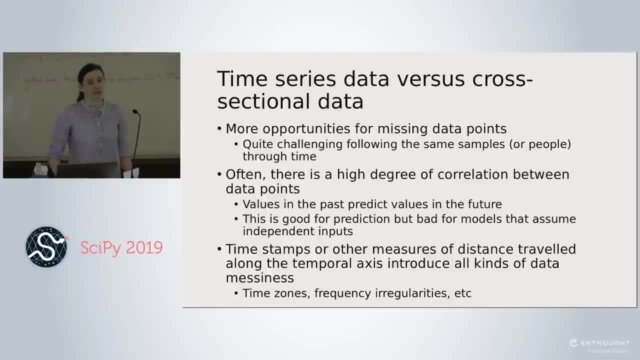 That's sort of an epic task. Even for really simple scientific data that can be a problem. For example, when I was putting together the data for this tutorial, I was trying to use some Colorado River data from the federal government and I kept getting bombarded with this sort of bright red text. 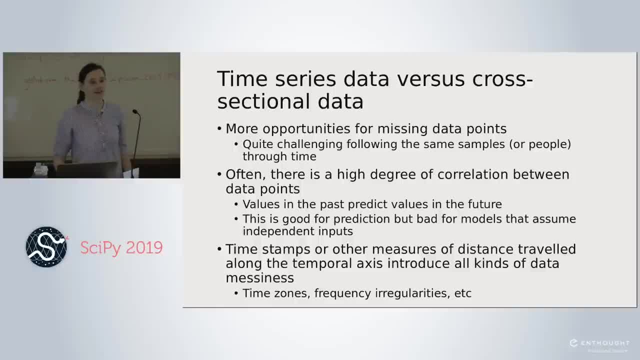 indicating what measurements they had discontinued due to funding cuts, right, And so time series, especially anything that looks at government data sets, is even affected by politics to some extent, which is kind of funny, right? You'll just run into it more than you might if you were just doing panel data. 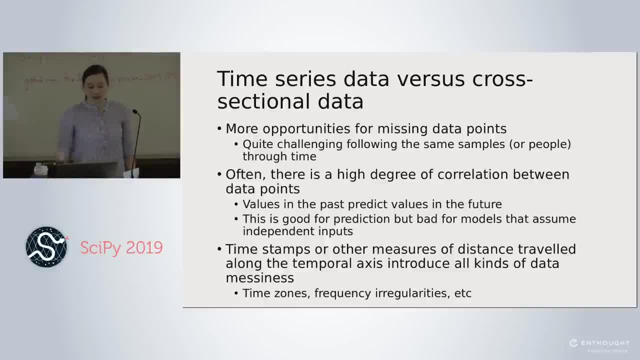 Second major point: there's a high degree of correlation between data points: Values in the past almost always and, we hope, predict values in the future right. So you have to think about what your errors look like. You have to think about what your relation to points in time looks like. 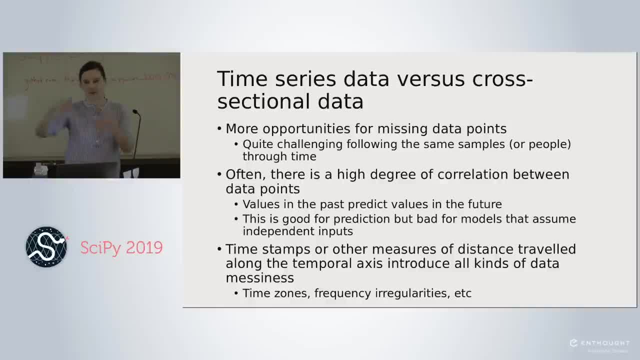 as opposed to correlations, where cross-sectional data, where you tend to throw things in and these are different people and hopefully, to first order, they're not super correlated with one another. So this is good for prediction, but it can be bad for models. 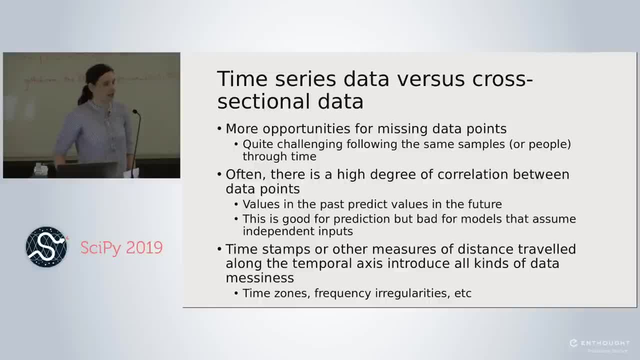 that assume independent inputs right. So, for example, when we are looking at some machine learning techniques or when we're thinking about how can I apply sort of non-time series statistics to time series analysis, we might very readily violate the assumptions, whereas if we're sort of careless in general about running linear regression, 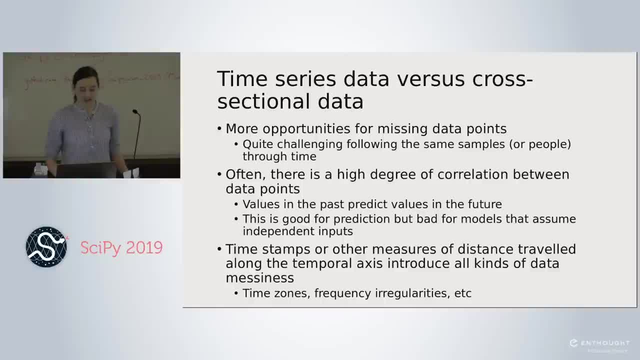 that's not so likely to be true. It's very likely to be true in time series analysis. And then there's also just the hassle of dealing with timestamps or other measures of whatever your distance metric is along your temporal axis. right, You have things like time zones, frequency, irregularities and so on. 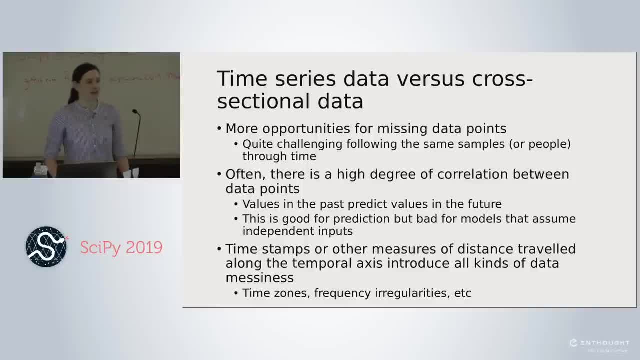 Even if you only work with sort of scientific data where things like the exact timestamp, like day of the week, doesn't matter, because as far as I know, that doesn't affect physics- you might somehow find that, for example, your timing measurement is a little bit off right. 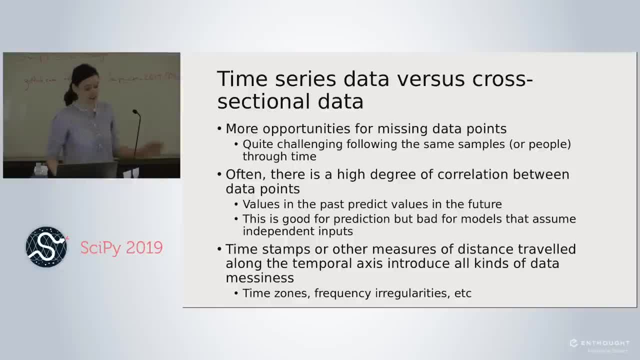 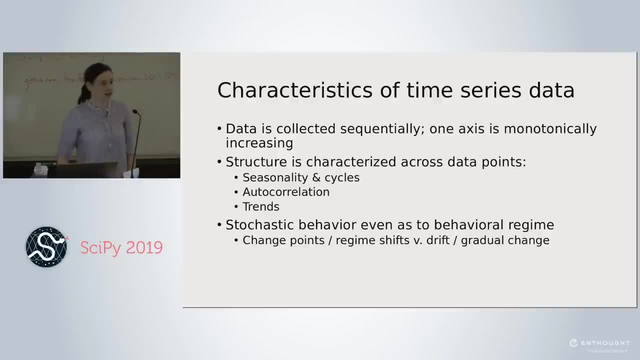 You have some sort of bias problem, so it doesn't go away even in that case. Okay. Other characteristics: Data is collected sequentially. One axis is monotonically increasing, right. So, as I mentioned, that's my definition of a time series. 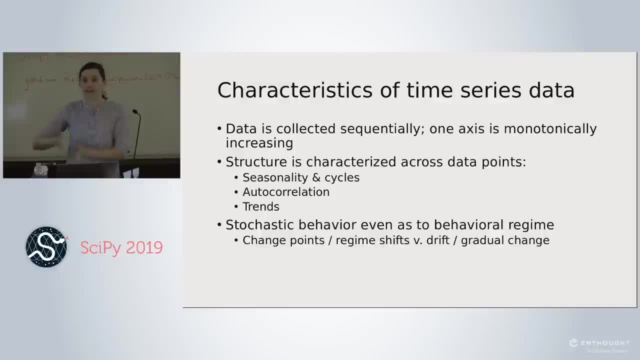 It's got to have a meaningful axis with measurable distance. It doesn't have to be time. We do want to characterize structure across data points, right. So again, seasonality and cycles, autocorrelation and trends. Who is familiar with the concept of autocorrelation? 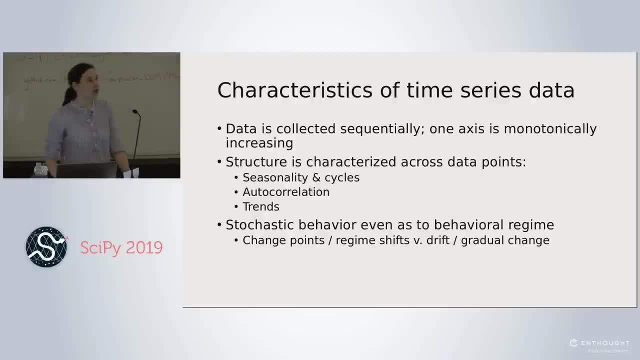 Just want to make sure that's fairly familiar. So just a quick overview for those. For those who aren't, autocorrelation is just how a point at time t is correlated, say, with the time t minus 1 for the entire time series, right? 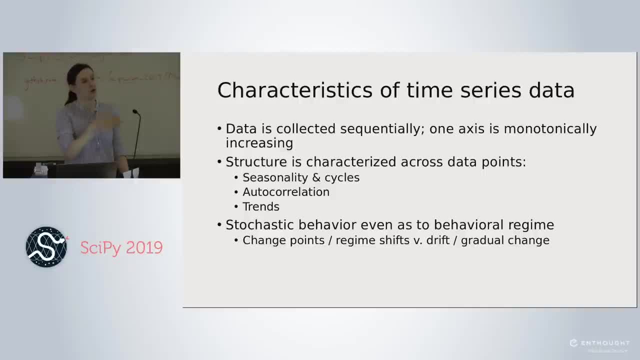 So, at time t, how do I relate Like this value? how does it always relate to the value before it? right, in a probabilistic sense? That's autocorrelation. And then, finally, stochastic behavior, even as the behavioral regime right. 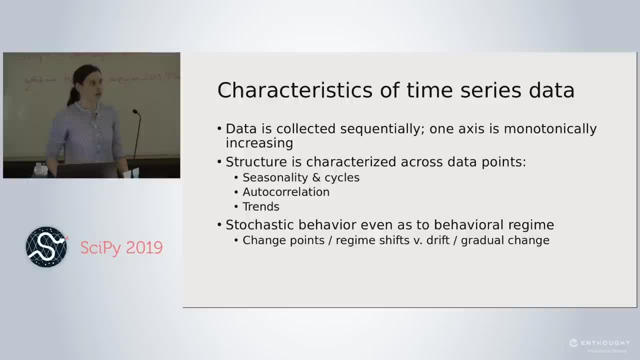 So in cross-sectional data we're used to thinking about: oh, if I see sort of qualitatively different behavior, I might be identifying sort of different subgroups in my population, right, Maybe I'm looking at two molecules or sort of two types of consumer or whatever. 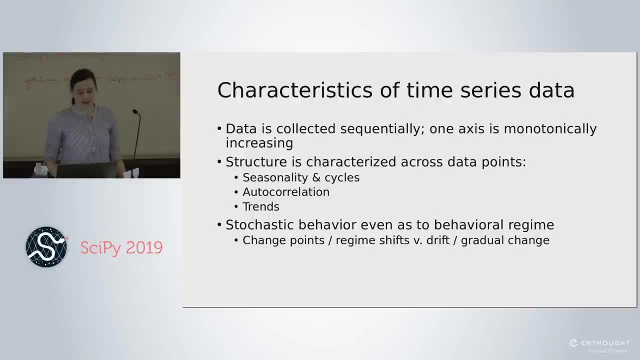 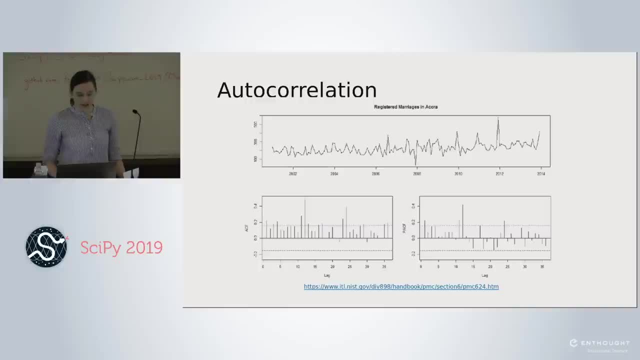 But in time series you can just have, within the same series, some kind of stochastic shift to a different regime and you need to think about how to identify that, That's sort of change point identification. Okay, Here's a slide on autocorrelation and in case anyone's not familiar with it, 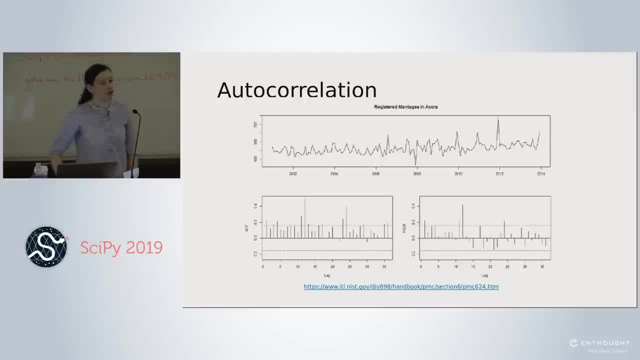 even if you are. I guess the main point I want to make is that you don't always know from eyeballing your data what it's going to look like, right? So we might think, oh, I'm just sort of looking at this top panel. 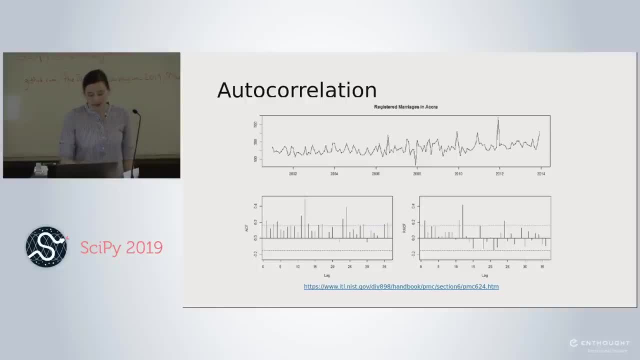 I have a sense of how correlated these things are, but I personally, when I then look at the lower panels, this series is much more sort of self-correlated than I would have thought. from just looking at it right, It looks kind of noisy and maybe there's some kind of seasonality. 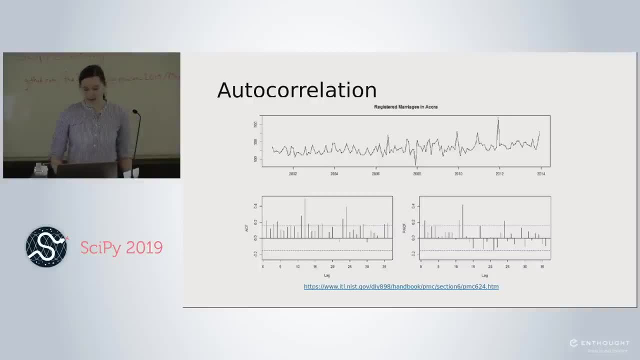 but not to the extent that I see with the ACF, So that can be good to keep in mind too. Your data is never clean enough, or never sort of noisy enough or white, noise-like enough or beautiful enough That you should not run basic diagnostics. 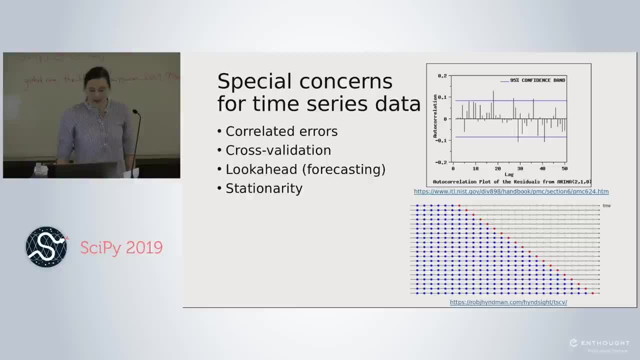 Okay, Special concerns for time series data. so correlated errors right And on the right-hand side, on the upper right-hand side, this is actually the errors or the residuals of a time series model. So at this point I say: already wrote a model that I thought accounted. 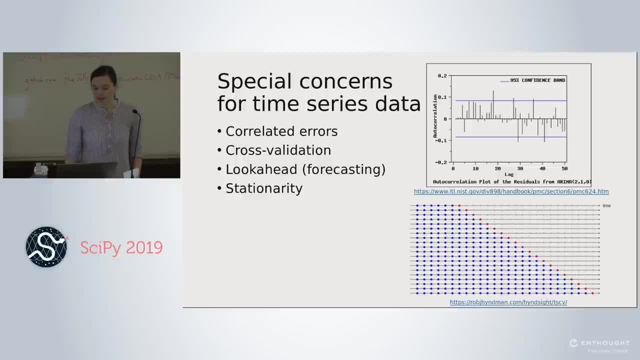 for the seasonality and the self-correlation, But what we can see is these blue lines give us the significance levels. You can see that this model actually is failing to describe all the autocorrelation of the time series right. So this is something you need to keep in mind. 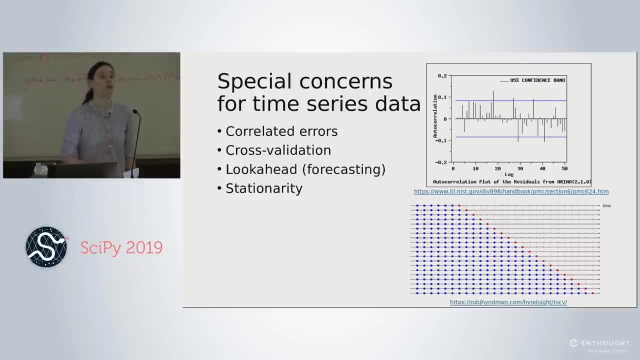 For time series there's special diagnostics you need to do that are time-aware. In addition to having time-aware modeling, we need to have time-aware diagnostics. Cross-validation also will usually look different in a time series context, right? So there I'll draw your attention to this plot in the lower right-hand corner. 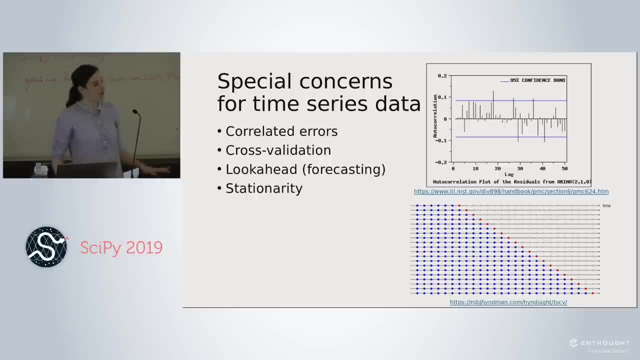 For cross-validation. it depends on what you are modeling and the nature of your data, but often, if you are trying to predict the future, you want to make sure that future information does not leak backwards in time, influence your model and make your model look a lot better than it does. 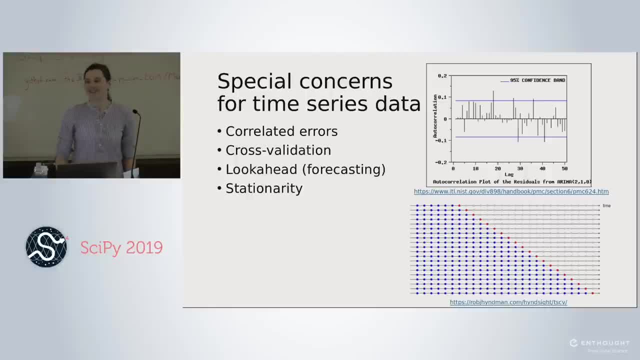 That sounds like common sense, right? We're all professionals. We would never, ever do that, right? And yet many people, myself included, will find themselves very embarrassed when something does much better in training and you think you properly cross-validated it. 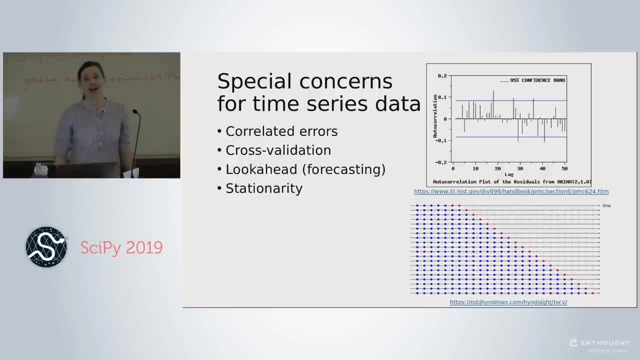 and you roll it out to production, which is really the ground truth, And it doesn't, And so you can really never, ever ever be careful enough about the cross-validation and the next bullet point, the look ahead. So one thing you can do, as is illustrated in this lower right-hand corner, is you sort 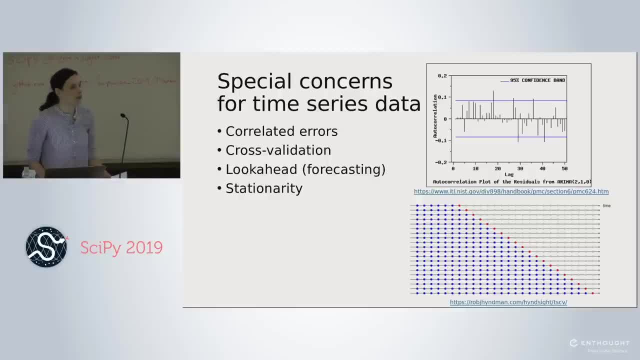 of roll your training data and your testing data forward in time, And the idea is you never want to test on data that is in any way older than what you trained on, because you don't want information propagating backwards. That's another thing about time series and temporal axes. 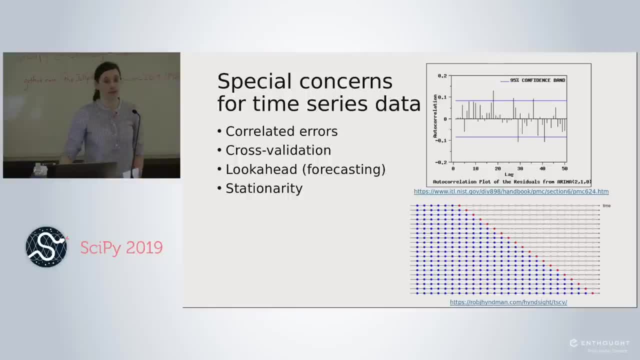 Most of the time, right. the information should really only propagate in one direction. You can write models that are the opposite, right. You can have causal time series and you can have the opposite, where information goes backwards in time. That doesn't tend to be interesting for modeling, though, right. 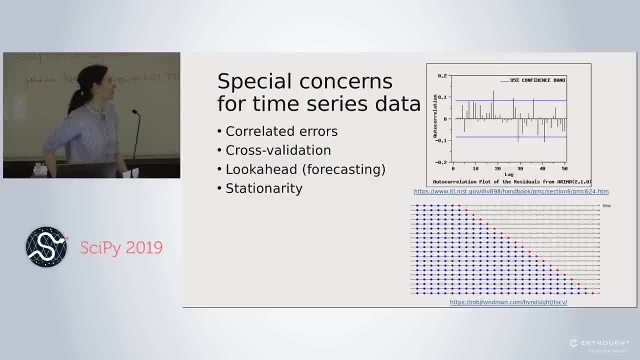 That doesn't tend to be the questions we're trying to answer at work or in research. A few other notes on look ahead. right, So this is just for cross-validation. Just because you've covered this does not in any way mean you've avoided look ahead. 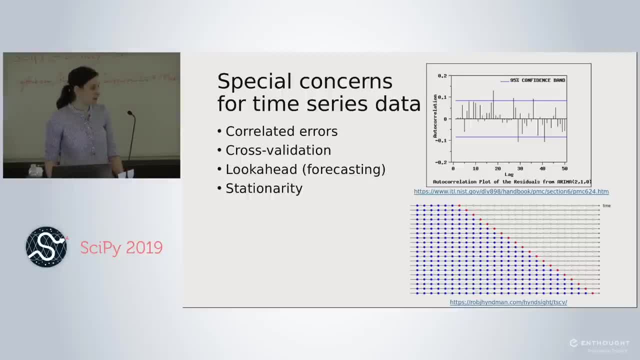 Just because you've properly cross-validated- there are all sorts of other things to look ahead. Just to keep in mind: time stamping right: Just because you have data available, time stamped at a particular time as an input into your model, doesn't mean that that time stamp reflects, say, when you would actually have. 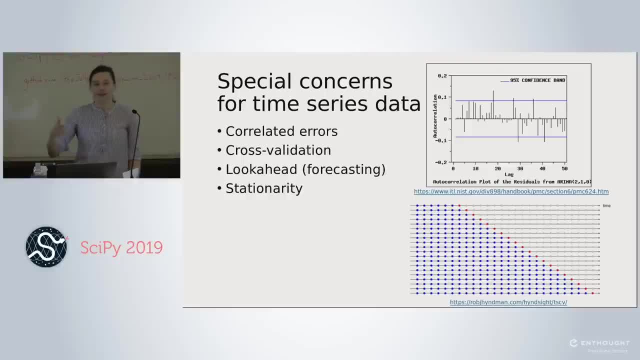 that data right. So you might have, for example, let's say, you're trying to predict the jobs numbers and you might have some sort of survey of how people are feeling and you have the date of the survey, when it was taken, but you forget that maybe it doesn't get input into the system. 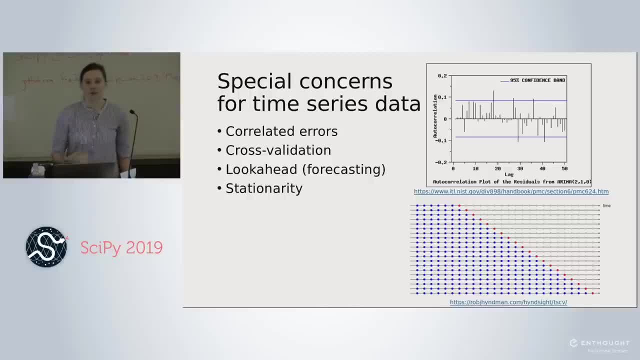 available to you for a week, And that's the sort of thing that can happen when you move from research to production- is suddenly you realize that your inputs that you thought were available, actually are it right And maybe it took place in the past, but it hasn't been registered yet. 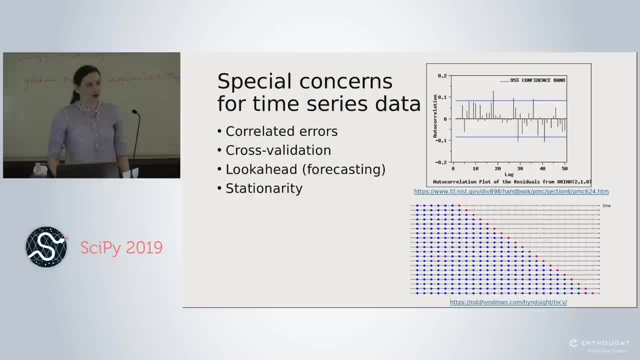 So there's another example of look ahead. There are many more and as far as I know, there's not sort of an automated way to diagnose look ahead. You just have to really keep your eyes open, and it depends a lot on what your field is. 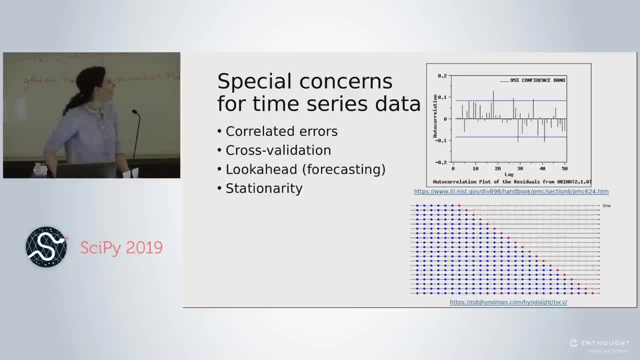 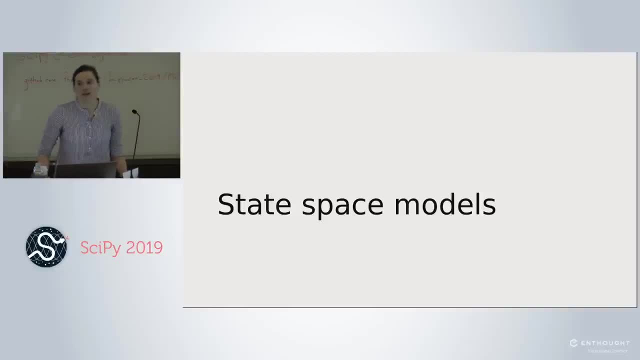 And sometimes it's not even an issue depending again on the field, but especially tricky with human data. Okay, So just a brief overview. Any questions or comments or anything people with experience would want to throw in on top of that. 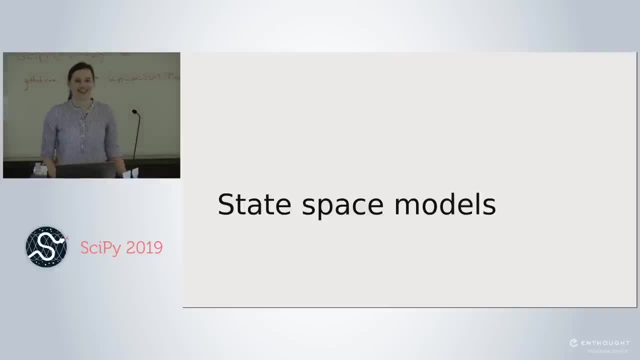 I know It's like 8.30 in the morning. Oh yes, Somebody does. My first introduction to time source analysis was all about understanding the frequency space for things like nightless frequency and sampling rates. Is that part of the modern time source analysis or is there a statistical sense to it? 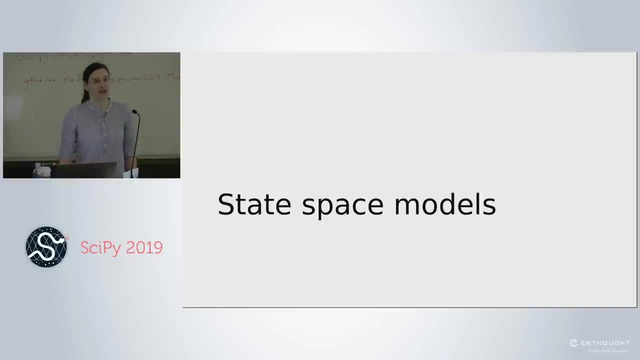 Only in a statistical sense. So I have no frequency domain examples here, although I can speak about it briefly when we get to deep learning, because certainly there's a lot done there And that's a good thing to highlight, right? So there's a whole sort of other domain of time series analysis that looks at time series. 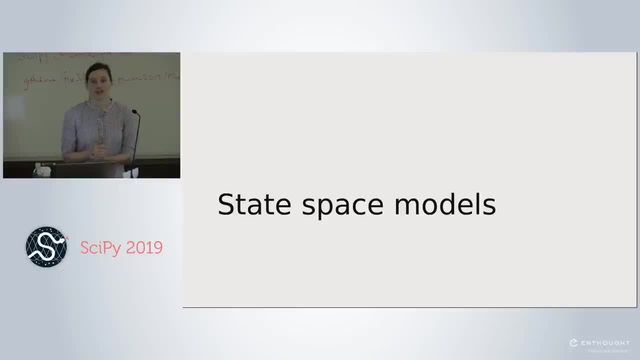 in the frequency domain Very successful, especially in certain fields And actually, for those who are interested in a brief tutorial, I have that in my first tutorial posted, so that's a good point to raise. Yes, You mentioned that part of this is doing missing data. 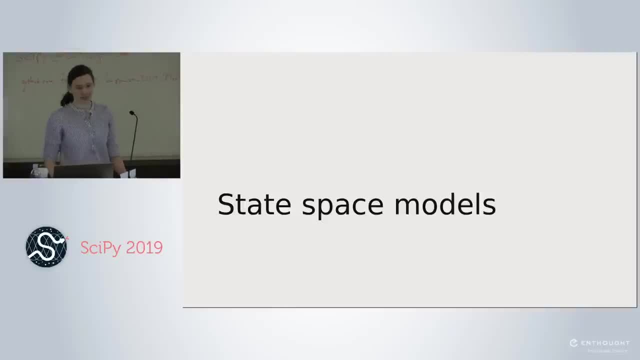 Are you going to get into imputation and how to know? No, I won't be discussing data imputation, although all of the methods we use can be applied to data imputation. So I'll make sure to comment on that as we go. 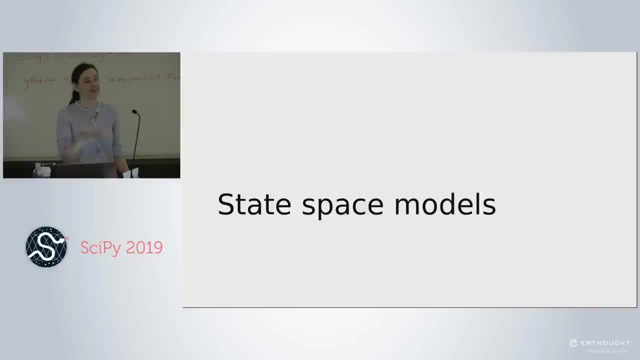 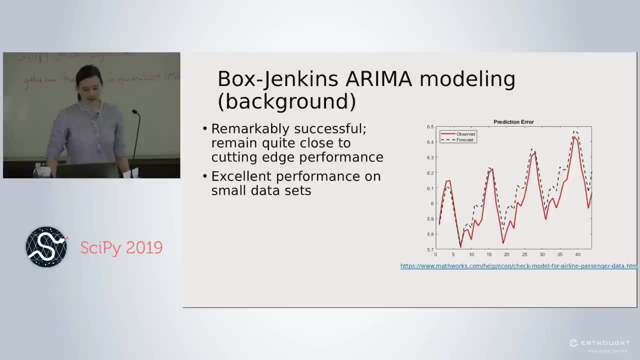 But there are no examples, And that's another. given what I highlighted about the missing data, this can often be important, Okay, Okay. So let's talk about state space models. We'll start with some background On Box-Jenkins ARIMA modeling. 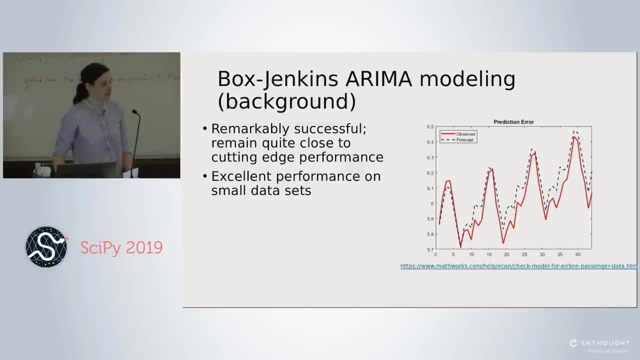 So ARIMA modeling- if you haven't used it, you've probably at least seen this term, ARIMA. or maybe you've seen ARMA or AR or MA. These are all sort of the same class of models- statistical models developed a very long time. 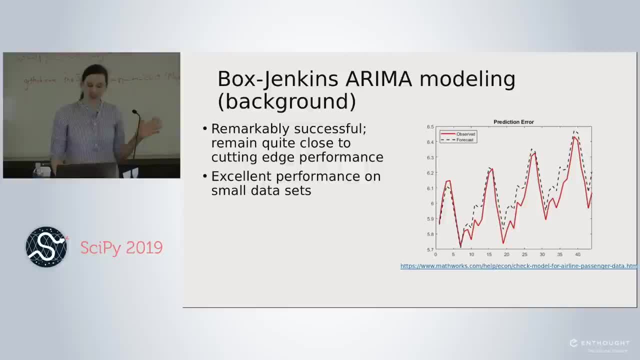 ago at this point, sort of early to mid-20th century. As you can see, though, they can have, despite sort of being old, traditional, they have excellent performance, Especially on small data sets. So here I have the example of the airline passenger data set, a very famous data set. 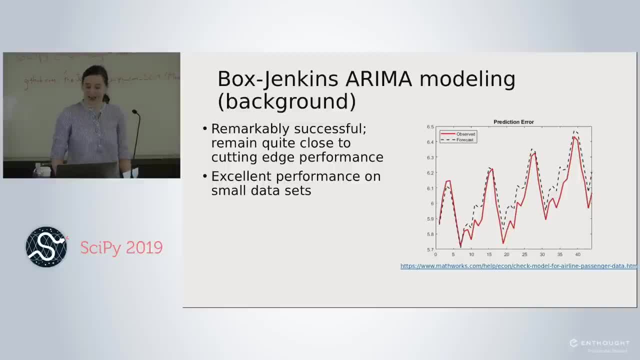 if you look at time series textbooks, This is always there You can see. so the forecast versus the observed are pretty close right. This is already pretty good, And so one of the interesting things about modern time series analysis: right are sort. 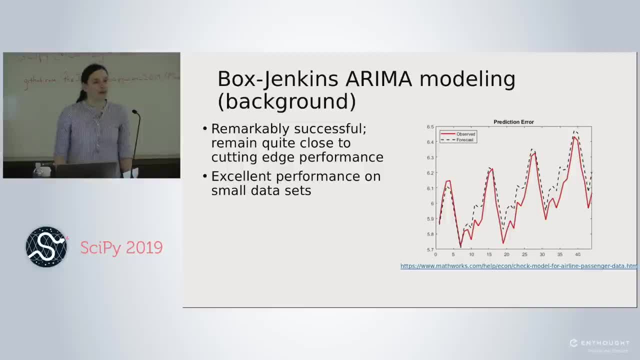 of nontraditional methods, however you want to call them, is, you always want to make sure that you are actually contributing something that you couldn't get, say, with an ARIMA model, And that is surprisingly difficult. Not just that, it's also surprisingly difficult sometimes for an ARIMA model to be an even 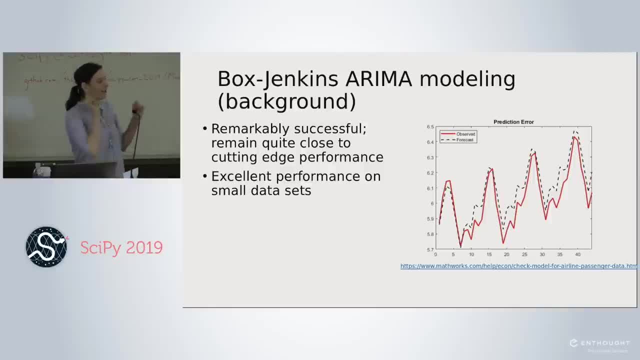 simpler model, which is just sort of your null model, which could be something like I will predict for time: t plus 1, the value I have at t and just leave it at that, And that itself can be an extremely good model. 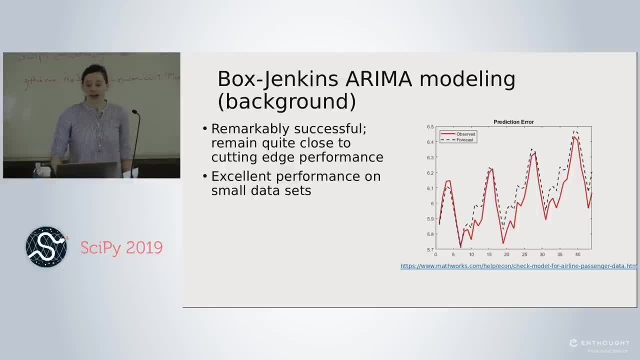 So I just want to point out that we are starting with a fairly high bar, especially in certain domains. right, If you have certain kinds of data sets that don't have too much noise or that have, say, a strong seasonal component, You can do very well with this sort of model. 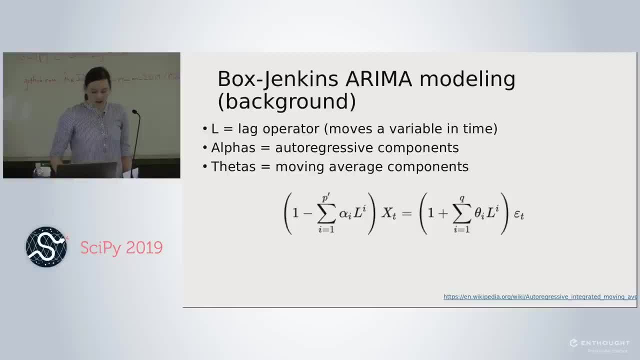 So what does an ARIMA model look like? Well, I just want to show you sort of one way of thinking about it. If L is your lag operator, a lag operator means, if I apply L to x, sub t, x at time, t. 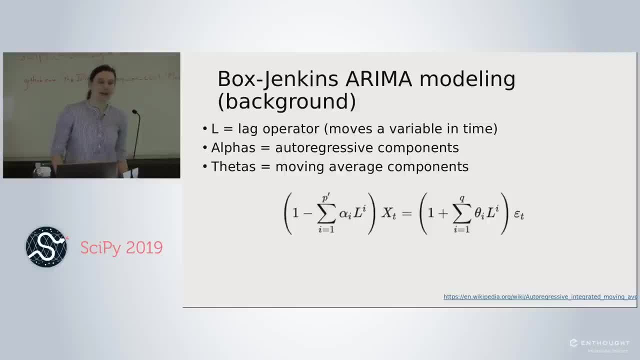 I get x at t minus 1.. If I apply L squared to x sub t, I get x sub t minus 2, right? So it's just a way of expressing that we're moving something back in time, In this case. now my alphas, my alpha sub i, on the left-hand side. 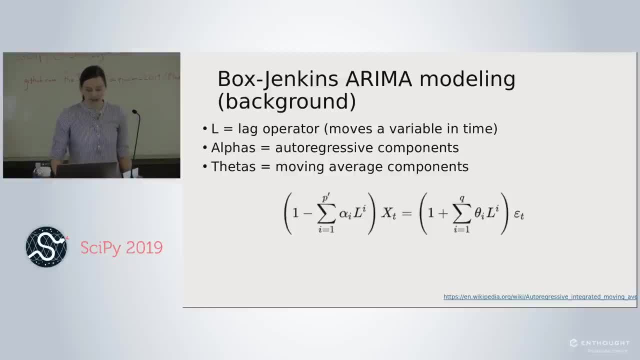 Those are my autoregressive coefficients And my thetas. on my right-hand side are my moving average components. So this is sort of the traditional way to express an ARIMA model. It's some sort of, Or this is an ARMA model, rather. 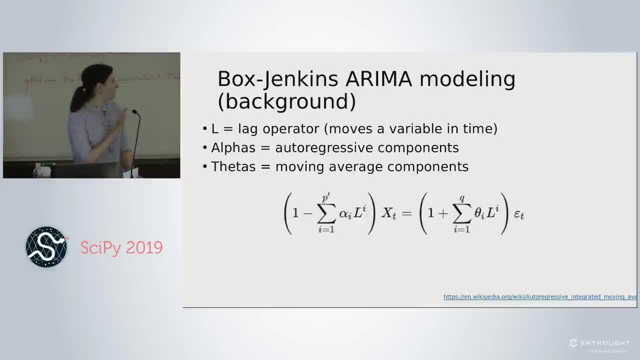 It's some sort of on the left way of operating on the data itself. So this is going to have coefficients that apply to past values And then on the right, you're going to have coefficients that apply to sort of past errors. 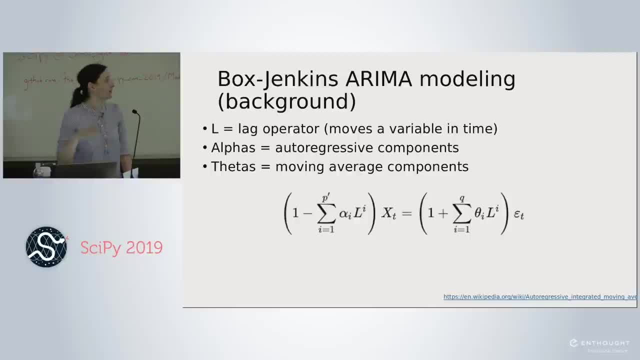 right, And those could be noise in the system, stochastic noise, They could be measurement noise. You can interpret it in a number of ways, But the idea is that your future value is in some way going to depend on your past values and your past errors. 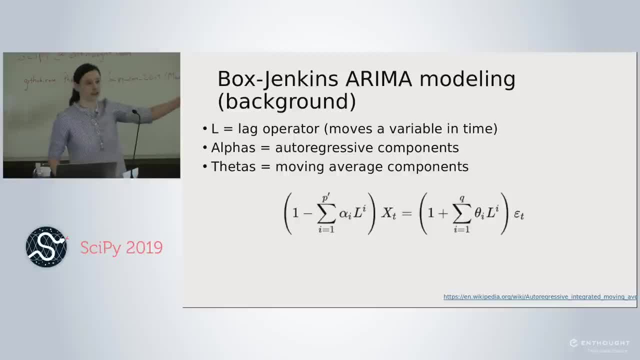 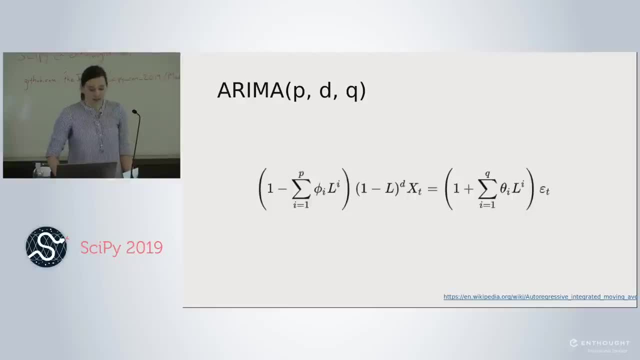 And what sort of values you choose for p and q. your summation are part of how you do your model tuning. Now, if you go to an ARIMA model now, you have all of that plus a difference. So all that means is you have this additional 1 minus L to the d, which means you're going. 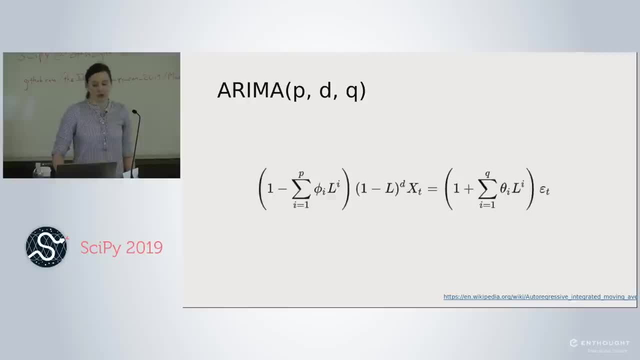 to difference your time series. So that means, instead of drawing my original time series, like my error, you're going to convert my time series, like my error, passengers, with the absolute number at each time stamp. I'm going to convert my time series for a first difference to the delta. 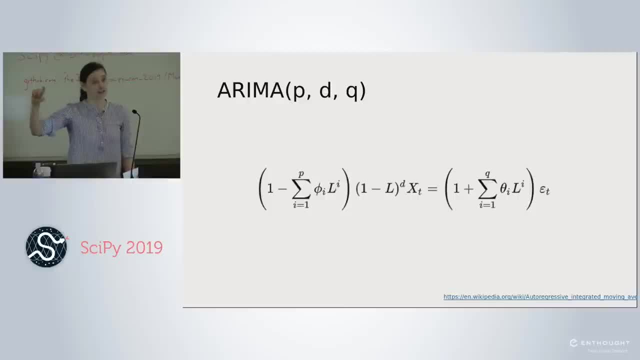 So the time series becomes a series of delta x's instead of x's right, So you have the exact same information. You haven't lost any information, except maybe your offset. And what that does is it often converts your time series to a more tractable form. 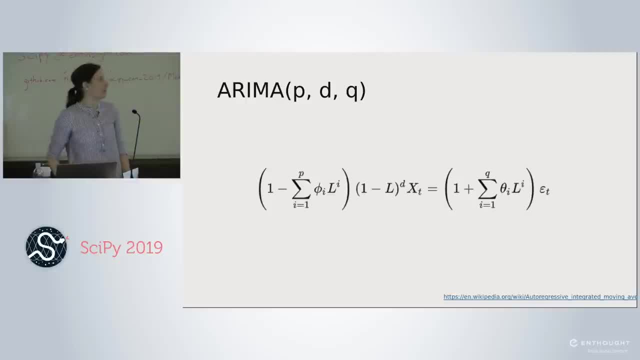 Maybe it won't have such differences in volatility over time. Maybe it won't have the trend. Maybe it will now be eligible. There are models to apply that wouldn't otherwise right. For example, ARIMA needs stationary data. So often you're going to be differencing to get that stationary data. 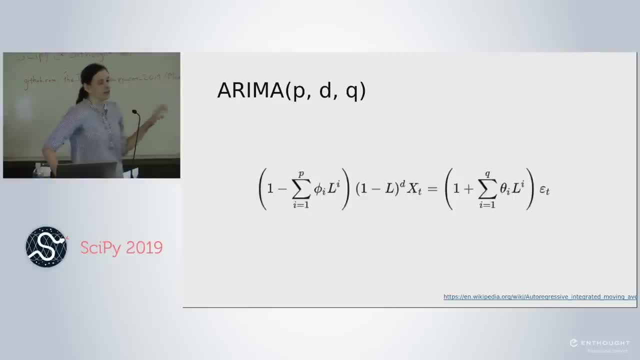 So that's the model. That's as much as I'm going to get into this model. for those who don't know it yet, All you sort of need to know is this describes future data in terms of past data and past errors. It's as simple as that. 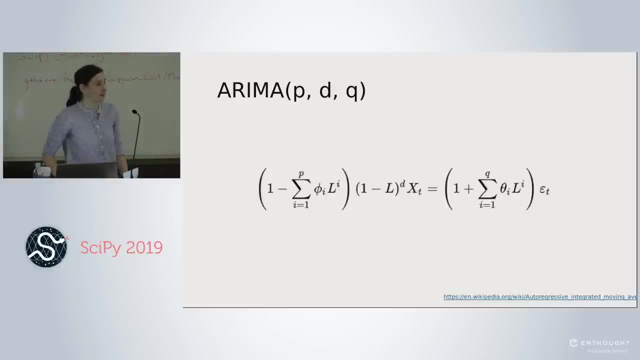 And I should also mention fitting these things is not easy. Fitting these things can be a bit of an art or it can be a matter of sort of optimizing your AKK information criteria and depending on who you talk to, there are sort of different. 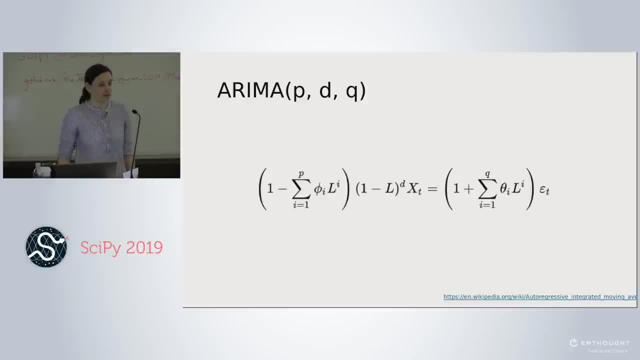 schools of thought. But everyone agrees this is a fairly difficult problem And it's easy to sort of overfit, It's easy to specify an overly complicated model and so on, And that's the sort of thing where you can then get embarrassed later when you roll it. 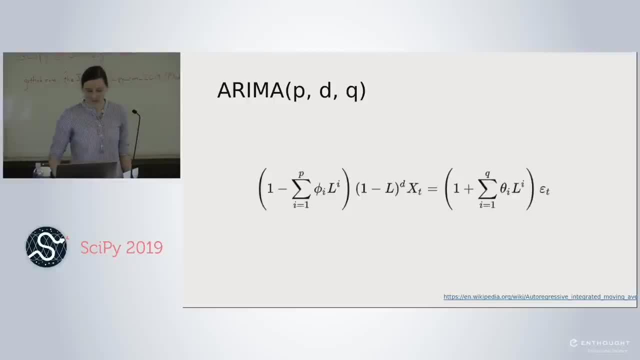 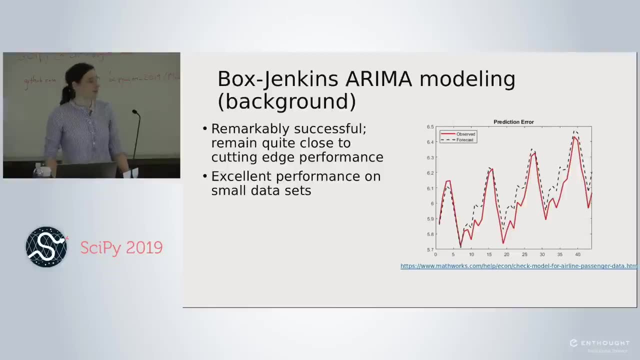 into production and it turns out to not be as good as you thought it was Okay. So why are people not happy with ARIMA despite, for example, this beautiful plot I showed you right? To me this already seems pretty good, right. 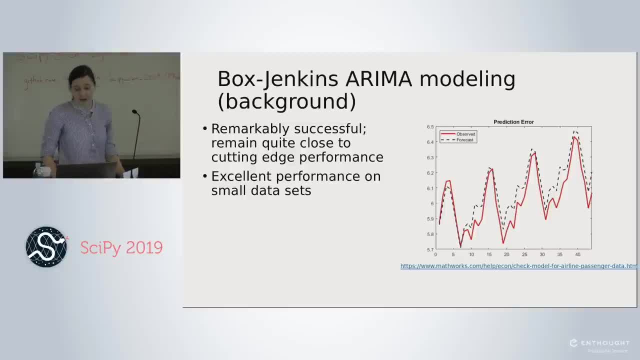 I'd say, if I could get this on everything I'm trying to predict, I would be happy. I would be happy. I would have liked to have it in the world. That's already enough to buy a house or buy some stocks or something like that. 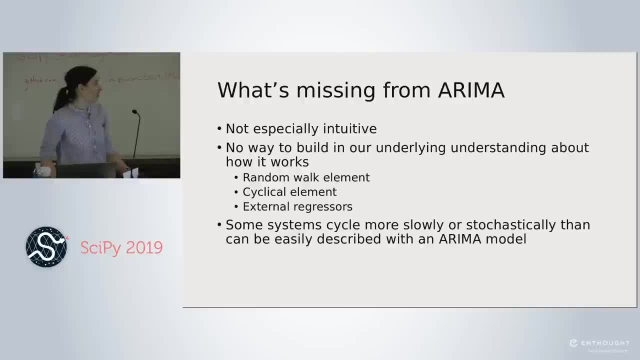 But there's plenty of problems, right. So I think the first one you probably noticed as I took you through it is: it's not especially intuitive, right? I just showed you this equation. The equation itself is a little confusing if you haven't worked with these sort of forever. 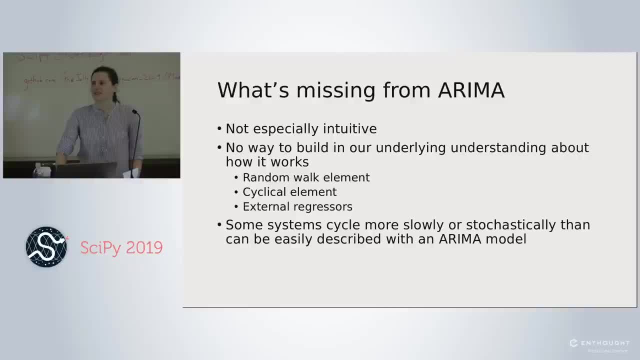 But on top of that, when you get coefficients, that's also still kind of confusing, right. What does it mean that you know, X sub T minus one, the coefficient is .3 or something, or 0.7.. What's the difference between the 0.3 and the 0.7?? I don't really know, And especially 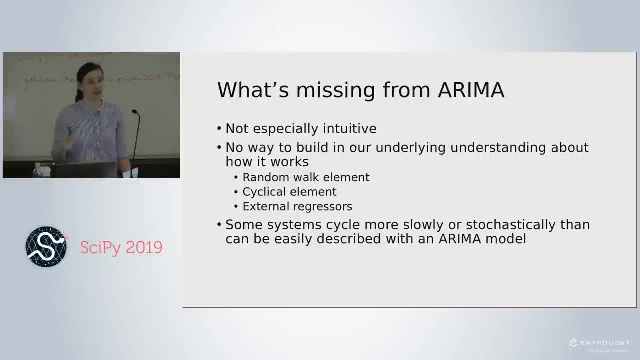 when you have multiple inputs, right. So if I'm saying x sub t is going to be a function of x sub t minus 1,, x sub t minus 2, x sub t minus 3, and they all have coefficients, then it really becomes. 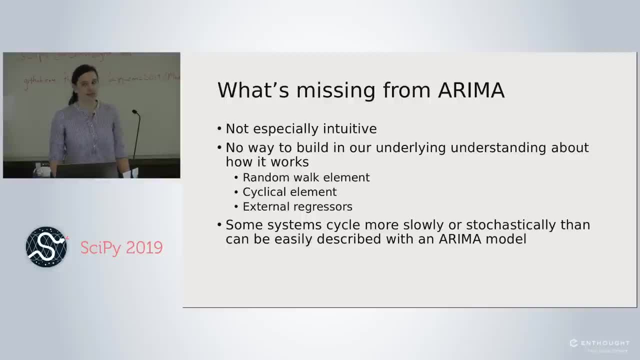 kind of difficult to think about what that dynamic looks like, And you'll see this in time series textbooks Mostly, when they give you examples, they'll stick to something with just one or two inputs right, So like an AR1 or 2 model, precisely because the more complicated it gets. 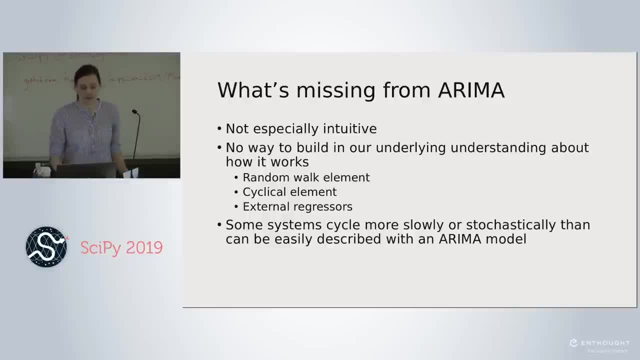 the more difficult it gets to even think about where different behaviors are coming from. There's also no way to build in an underlying understanding about how it works right. So, especially if you come from a discipline with sort of a well-developed set of time series data, 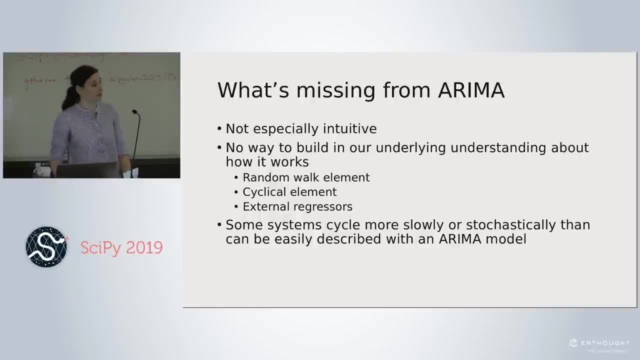 maybe people have been staring at it for five years or 100 years, right, depending on what discipline you're in. Usually, there's some knowledge about that system and there's also some theories. people want to test, right. So they might even say, well, it's not enough to be able. 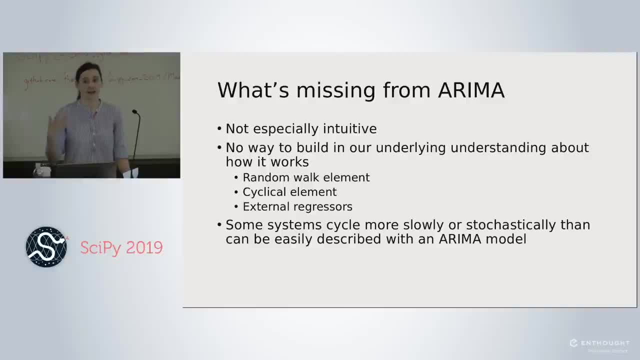 to predict or describe this model. But if you come from a discipline with some kind of dynamic, that's AR, MA, whatever, that doesn't mean much to me, but I'm aware that, say, there's a random walk element to this kind of data, or I'm 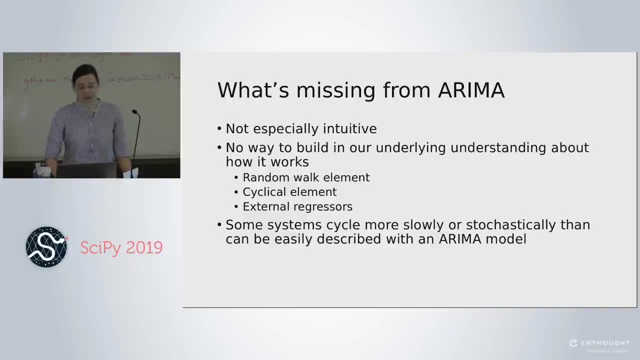 aware that there's a cyclical element which can't really be described with an ARRIMA, or there are external regressors I'd like to include, And then you know, you get into more complicated models or you start looking for models that are a little bit intuitive. Also, some systems cycle more. slowly or stochastically than can be easily described with an ARRIMA model. So ARRIMA models are also called P-W-S-E-A models. but ARRIMA models are more popular models And ARRIMA models are more popular models than ARRIMA models. So ARRIMA models are more popular models than ARRIMA models. So ARRIMA models. 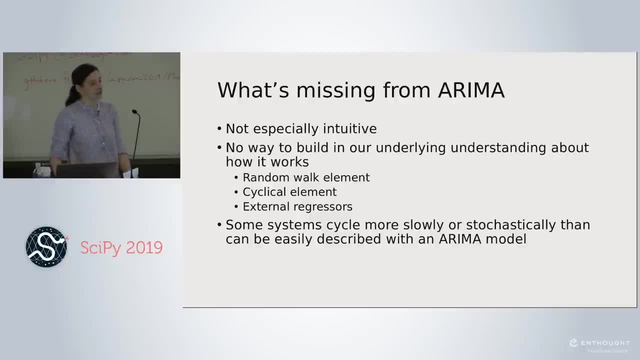 So ARIMA models do really well with sort of short cycles, right, Maybe seven days on daily data, things like that. But when you're already even getting to sort of 24 hours in hourly data, ARIMA models can get really ugly. 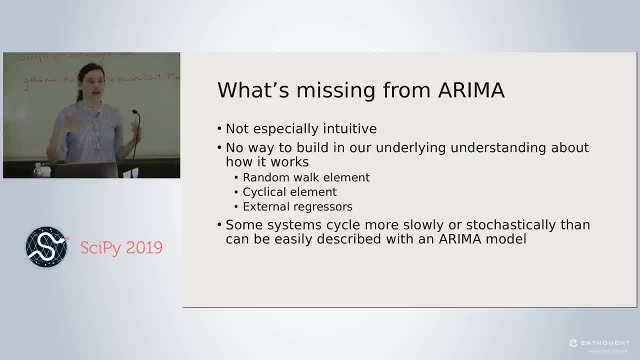 And it's unlike machine learning where you sort of throw more data at it and you might get a better result. ARIMA models sort of level out, So they do really well with small data sets. Arguably, they still beat everything else because you can give it just a 40-point time series and it will do really well. 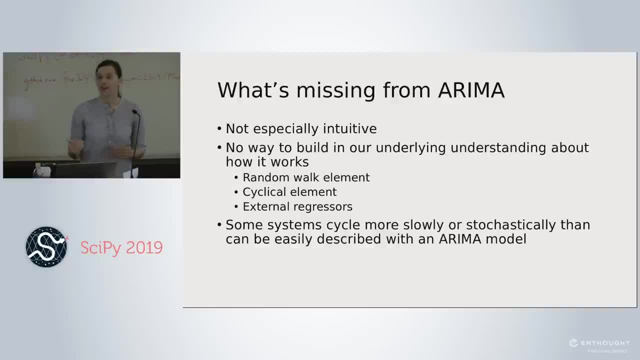 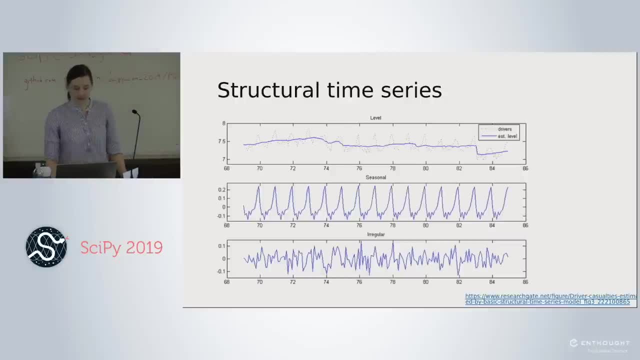 And good luck doing that with a tree or a neural network. But on the other hand, when you give it 40,000 points instead of 40, it's not clear that you get much better performance. Okay, So enter structural time series. 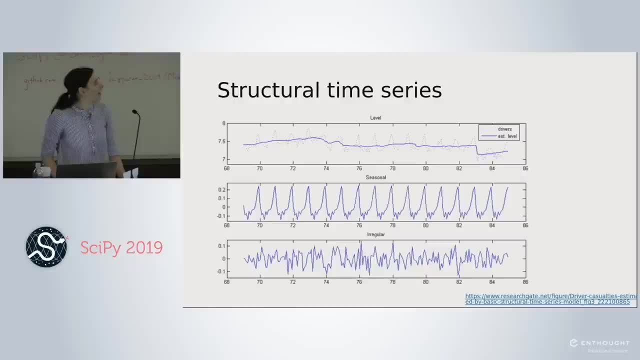 So these have been around for quite a while. They're not new, but they're sort of much easier to implement than they used to be a few decades ago. right, You get much more computing power now, And what that means is you can have a way that's a little bit more intuitive of understanding your system. 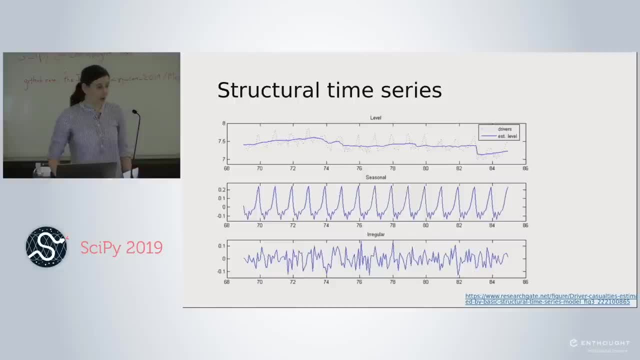 So here's an example of a model that has a level component and a seasonal component, And then there's a component they call irregular is just sort of everything else that can't be explained. That's sort of the error term we're going to add at the end. 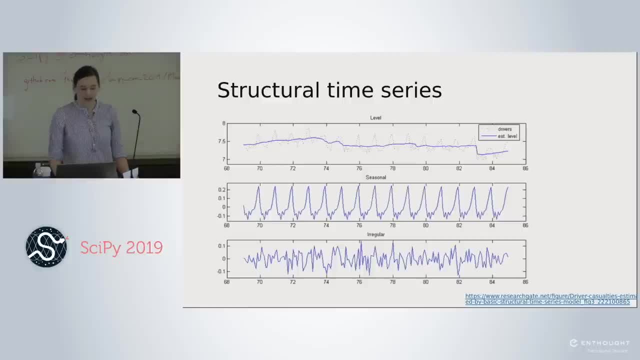 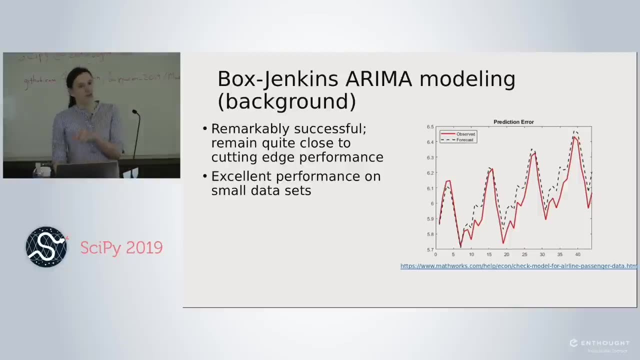 And so here, arguably, we already get a much better sense, right? So compare this- sorry to flip back, but compare this to that right This: I don't really have a sense of why my model is doing well or what's contributing to it, right. 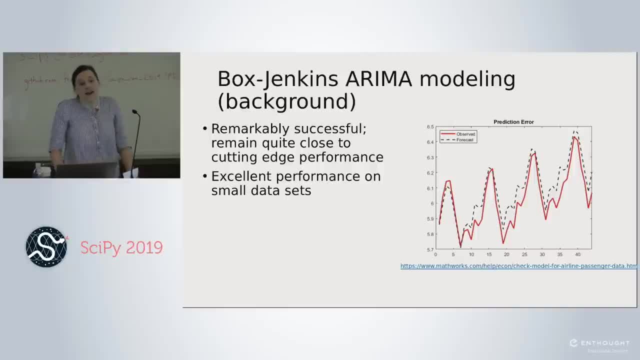 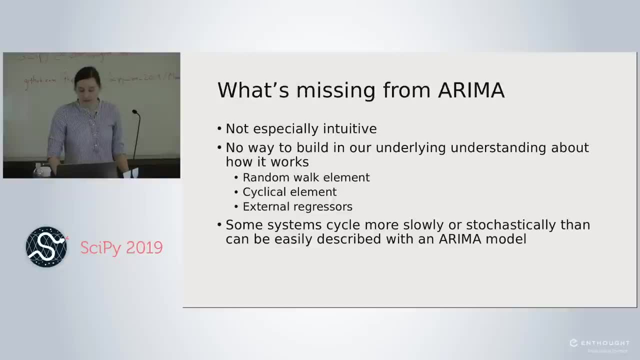 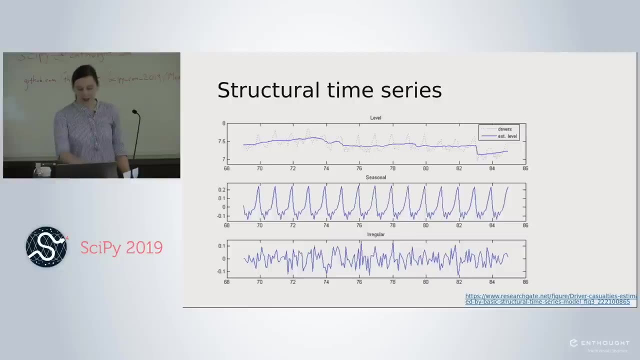 I can see that my model is describing the seasonal data. I could look at my coefficients from my ARIMA model and try to puzzle it out, but there might be quite a few of them so it's difficult to see, Whereas here I feel like I can look at this and say: well, you know, we have this underlying level, that sort of stays quite steady up until like sort of 83, and then it takes a dip. 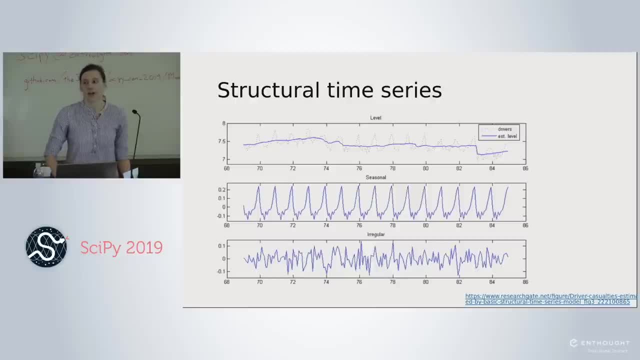 And I feel like I know a little bit more about what's going on and I can possibly use this as supporting evidence for a hypothesis, or maybe evidence that goes against my hypothesis- about how my data is doing. So these are how we use structural time series. 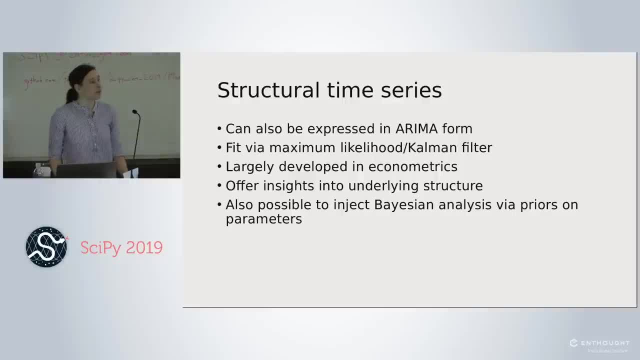 Interesting thing, they can also be expressed in ARIMA form. So in a way, we're not actually doing anything novel. We're not actually- if you're going to be like sort of a very formal mathematician about it- we're not contributing anything new. 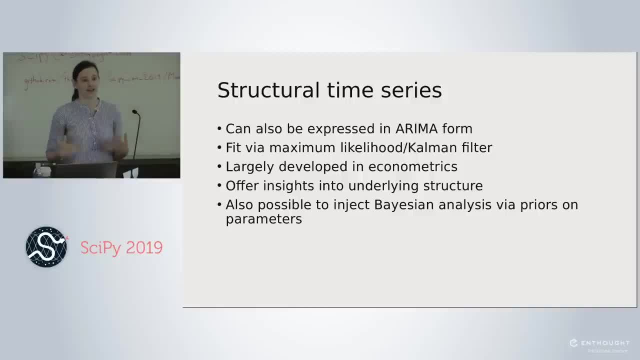 But to my mind we really are, because we have a way of inspecting and enhancing sort of the human intelligence rather than the statistics. These are fit via maximum likelihood or a Kalman filter, right, So you can have an MLE interpreter. 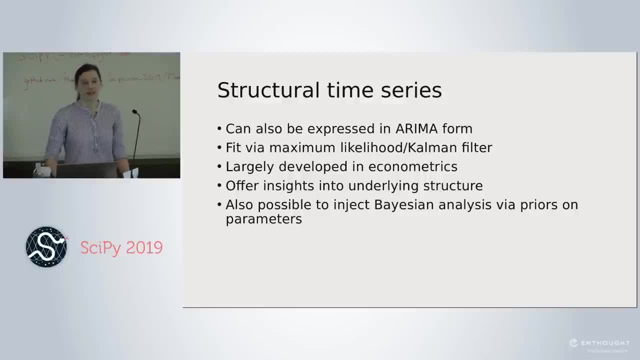 You can have a Bayesian interpretation of that. You can have a Bayesian interpretation of that. Interestingly, Kalman filters, again not super modern, I believe. they go back to the time of the Apollo mission. At least that's the story everyone likes to tell at conferences that they actually wanted to use a different way to estimate the trajectory of the spaceship. 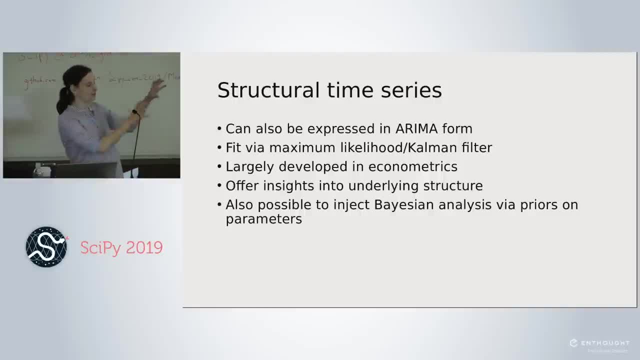 but they realized they didn't have the computing storage space where they'd need to store many points in time to continue their estimation. So they had to roll out something where you only need to store one data point at a time and you just update. 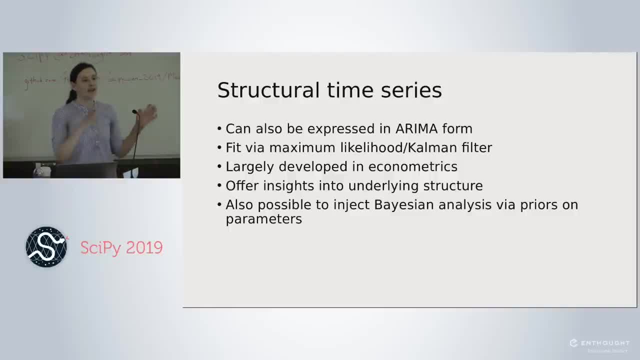 So that's part of the beauty of something like a Kalman filter method is you estimate your whole time series and you just keep a couple of numbers around. So even if you're estimating a time series that's millions of points, or you know 10,000 points, something more reasonable- 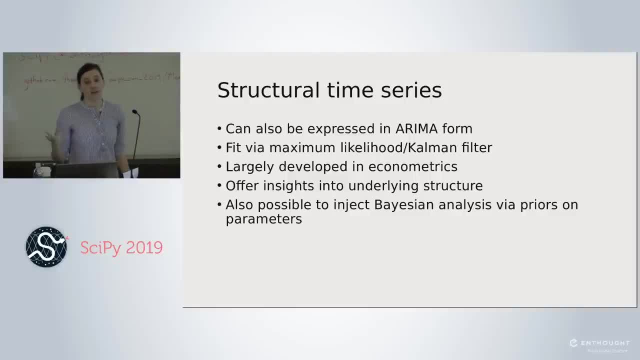 you're only keeping one number, You're not storing the whole thing. So this can be really good on small machinery such as the machinery of, you know, the computers of the 60s and 70s, Still useful today. These are largely developed in econometrics. 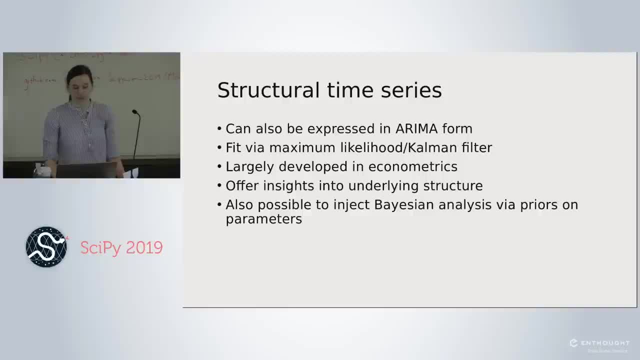 So if you have an econ background, you probably have seen these quite a bit, whereas they are otherwise, unfortunately, fairly underutilized. They offer insights into the underlying structure, as we just illustrated, and it's also possible- not in the package we're using. 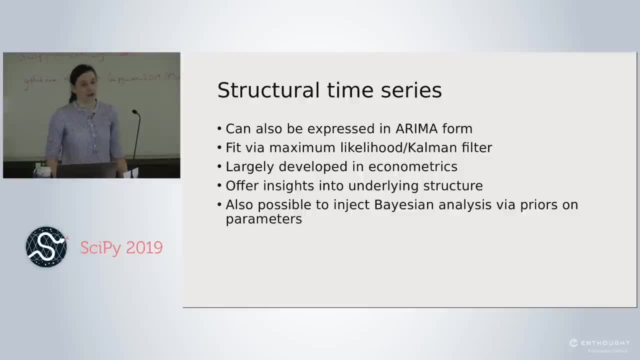 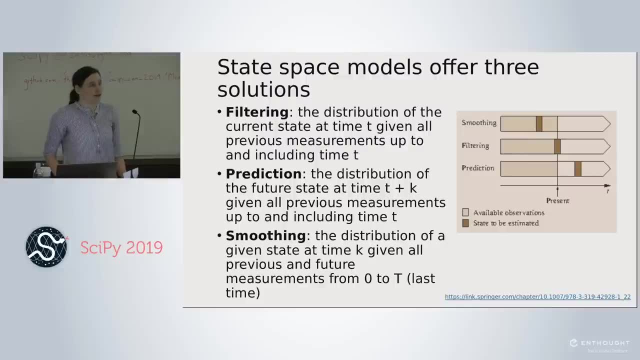 but there are packages where you can inject Bayesian analysis via priors onto your parameters, So you can sort of build these out quite extensively. State-space models: generally right. What's useful about state-space models? also compared to traditional ARIMA models, They don't just offer forecasting and a set of coefficients. 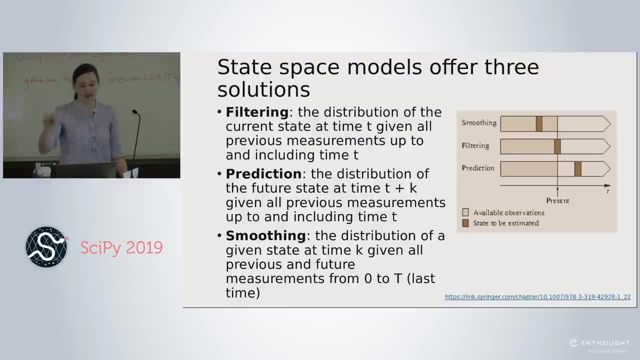 They sort of offer three different stages, and these are all inherent to fitting them. Stage number one is filtering. Filtering is this: Remember, I have this underlying assumption, I have some sort of noise in my data where I have these underlying components. 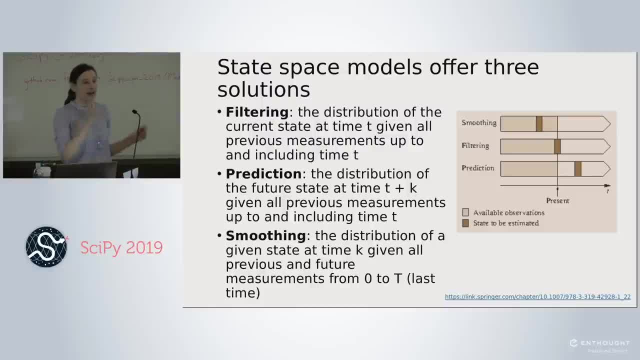 but I only get to measure the one thing right. Filtering is a way of at time t. I take all the data from zero up to time t, including time t, and I use that to make an estimate of sort of what is the true value right now. right. 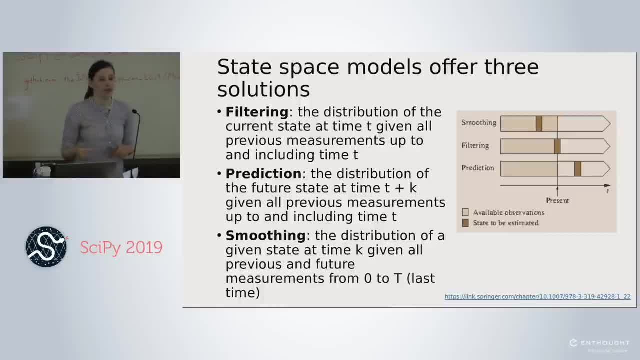 There's a value I'm seeing, but that might be fairly noisy versus the true value, and so you can see why that would be useful. on the Apollo mission right, Where actually is our spaceship? right, Our sensors say this, but is that actually where they are? 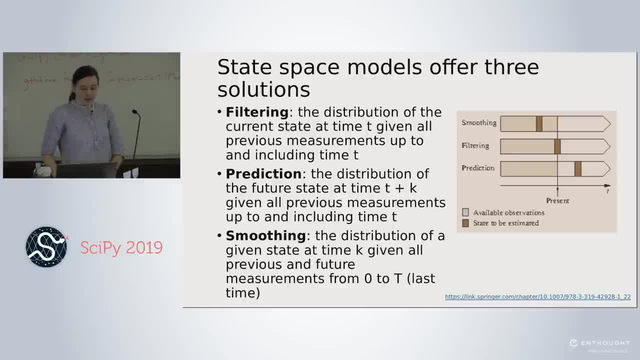 Because it's pretty important to have a good idea of where they are. Next step is prediction right. So in this case, at time t, I'm going to look t plus 1, or maybe even t plus k into the future. 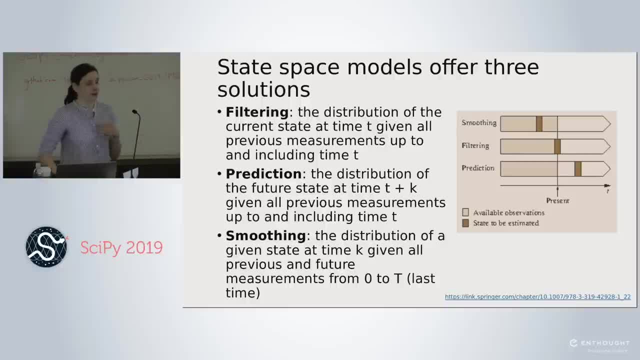 and that's something else I can do with a state-space model right, So I can both update where I think I am now, I can think about where I am in the future, and then, finally, I can do smoothing, which essentially is you have all of your data. 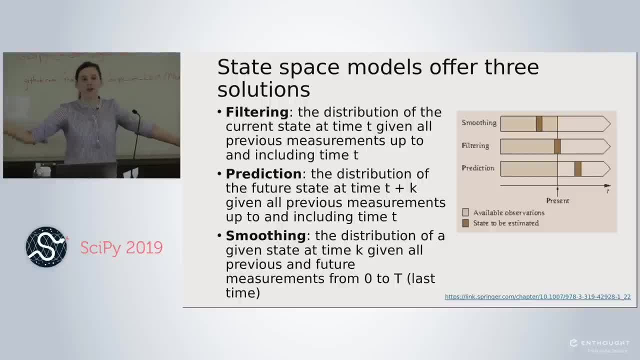 or all the data of relevance up to say big T, and I want to go back to some earlier time point and say, well, at time 10,, whatever, at time 10, I thought I was at, you know this point. 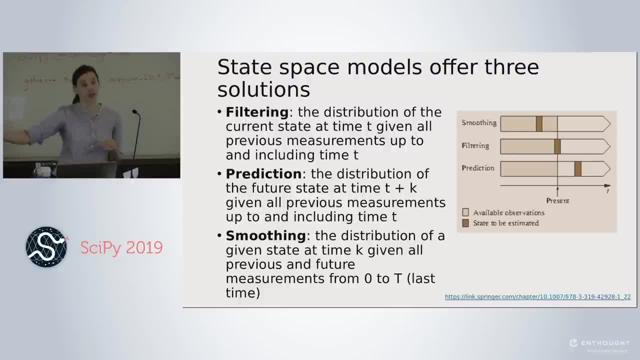 but now that I see where I ended up at the end, I realize I even get additional information. I can sort of back-propagate that and get an even better estimation of where I was at that time. So that's called smoothing. So this is all functionality: the filtering and the smoothing. 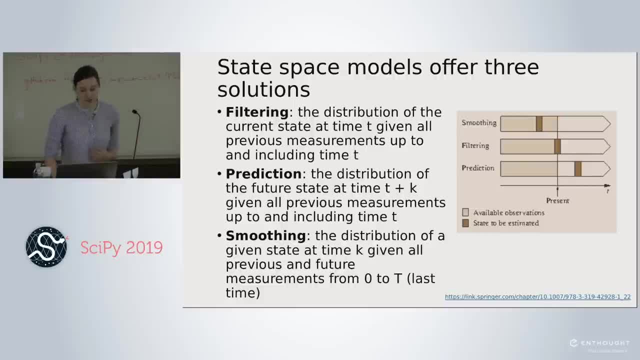 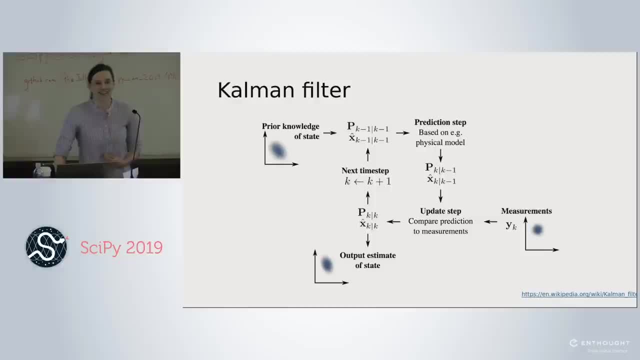 that you don't get with an ARIMA model right. So you actually do have new technology from having this perspective. Common filter. I thought about having everyone code this up, but I decided this was not the best use of our time, So this is just to sort of give you an overview. 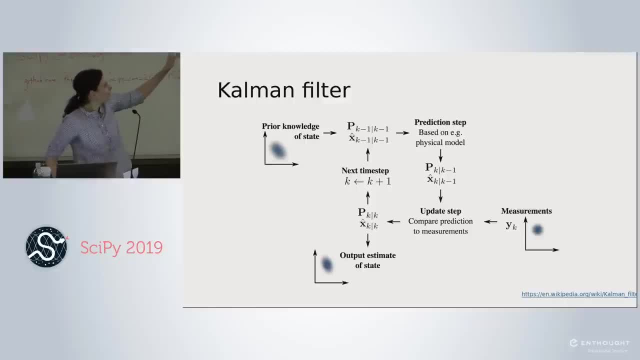 This is just sort of a high-level overview wiki graphic of how this works. You start with some sort of prior knowledge, usually just some sort of vanilla Gaussian distribution. You have your underlying state and you have some model for how you should update that underlying state. 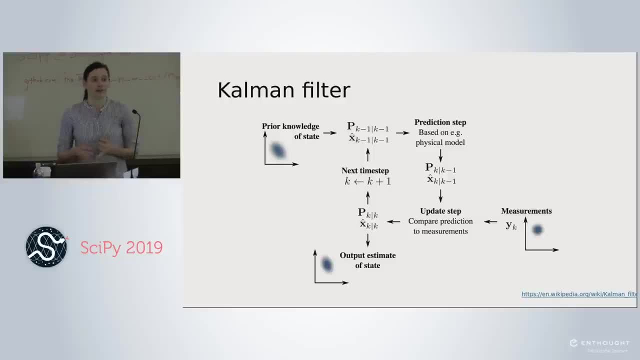 So you make a prediction as to where you think it's going, based on your knowledge of the system dynamics and its current trajectory. Once you make the prediction, you use that to do your update right. You compare how your prediction right At time t before I measured at time t. 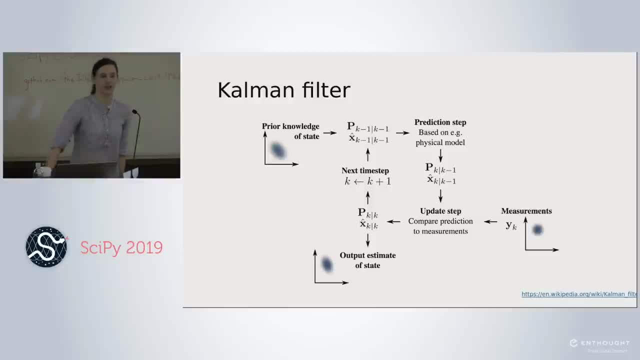 or at time t minus 1, the state of the world I saw was such that I predicted my time series would go this way or my measurement right. My measurement would go this way, But at time t, when I got to time t and got my measurement, 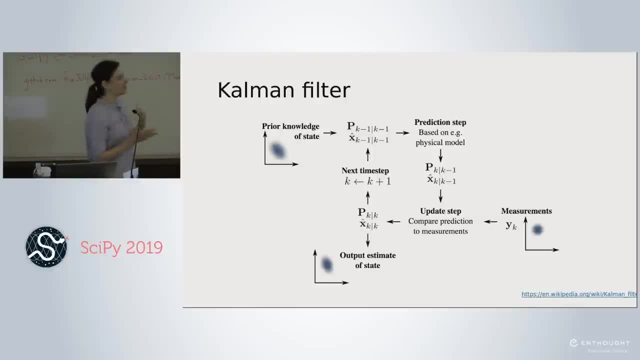 my measurement had actually gone the other way, right? And so this becomes a way of balancing. well, my forecast wasn't totally meaningless, right? So I don't just discard that because I have new data. What I do is balance. why does what I'm predicting versus 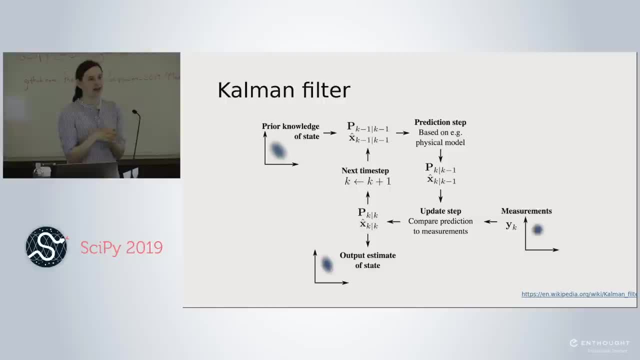 what I actually measured. why are they so different and how should I combine them to have something reasonable, rather than just picking one or the other? So you do your update step and then you go back to do your next time step And then. so this is sort of the forward propagation. 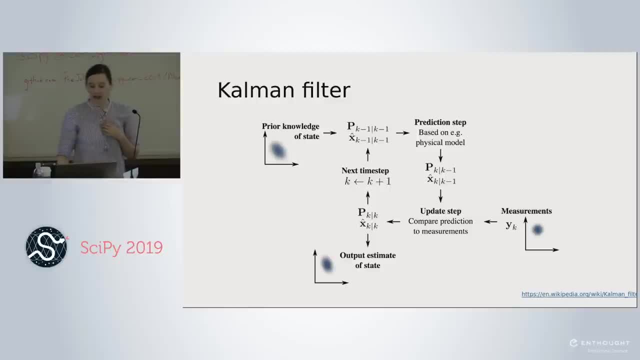 and then going backward in time. smoothing is very similar computationally, but it's a separate cycle. So there's your common filter. The underlying model for what something looks like is something like this. So with a state space, you have an underlying state. 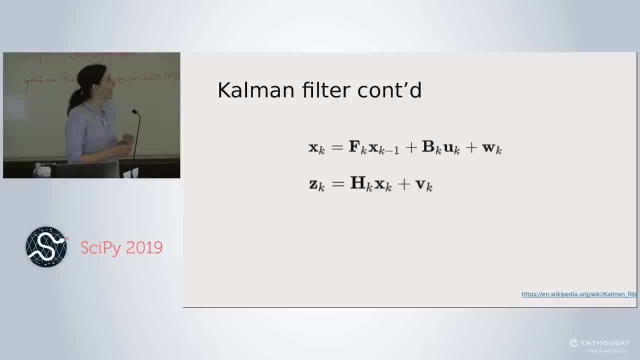 and then you have what you can measure, right. So your underlying state x is going to be some sort of model based on your right-hand side of your equation. You have f sub k times x times k minus 1.. So how do you update your state? 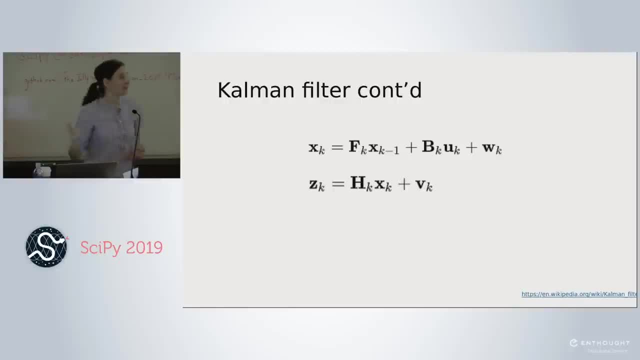 based on what was earlier, That looks a lot like an autoregressive model, But on the other hand, you also have the option for inputs such as bk times uk. That would be what, to your knowledge, was happening at time t. 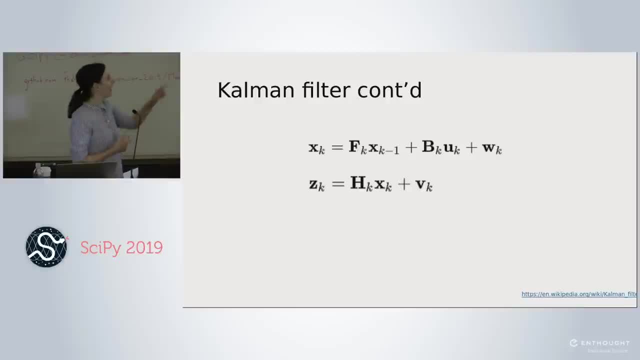 not time, t minus 1, right. So, for example, in the case of Apollo, x sub k minus 1 is where they thought Apollo was at time: k minus 1.. But u sub k was. well, what are we doing with our motor? or our rocket? 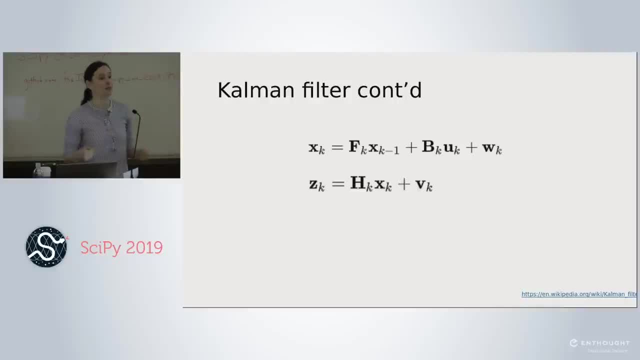 Like: how are we positioning our propulsion system at this moment, or is it even on? That's what's described by u sub k right, So you can also, if you know sort of what your astronauts are doing up there, you can factor that in as well. 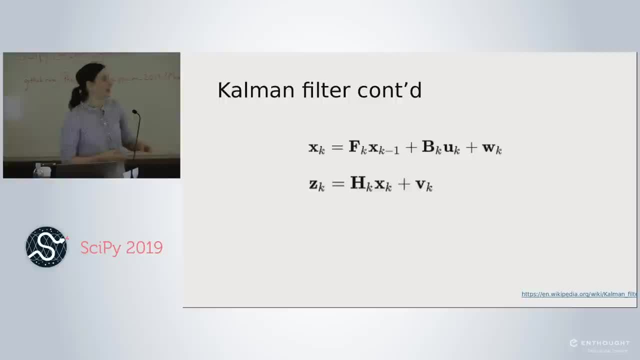 and then you have some sort of error term. So there's your description of your underlying state, and then you have your measurement, which we'll call z sub k here. right, You recognize that in some way your measurement might not be directly the same as what your x sub k is, right? 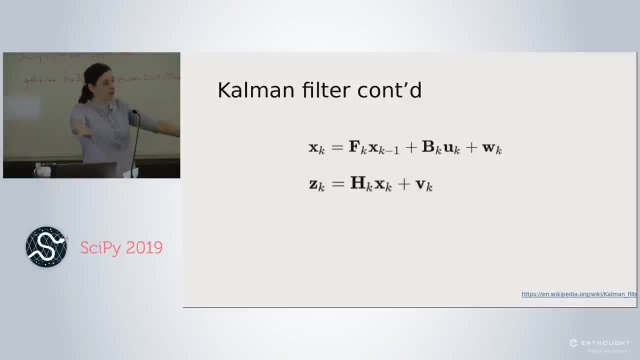 So in the Apollo example, your state where you are and your position that you measure should be the same thing. We don't have some sort of translation? These are not in the same space, right? It could be that I'm actually x. 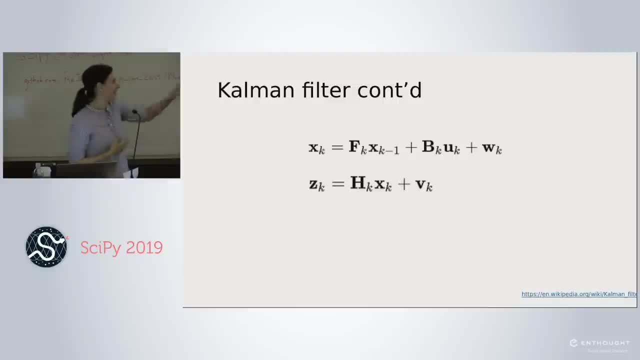 maybe I'm measuring only velocity and acceleration, not position, and then somehow, with my observation I only get position and I'm trying to find a way to translate between them. So the point I want to make here is just that these are really flexible. 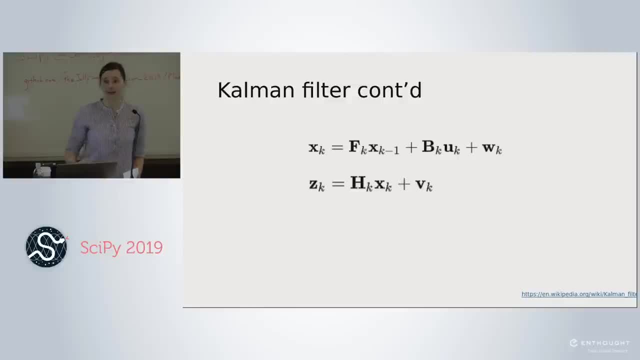 You can describe all sorts of dynamics, but it does require that you have some kind of hypothesis about the dynamics of your system to really be interesting, right. So you might not want to throw this at a model of, say, really noisy stock data. 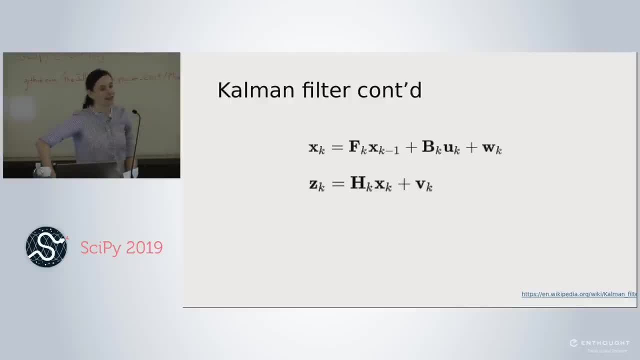 so let's make up a model and just put it in, because you probably won't get sensible outputs. but a model like a rocket, where you have Newtonian physics and you have a flight plan, makes a really good case for this. Okay, And this is just spelled out more in detail. 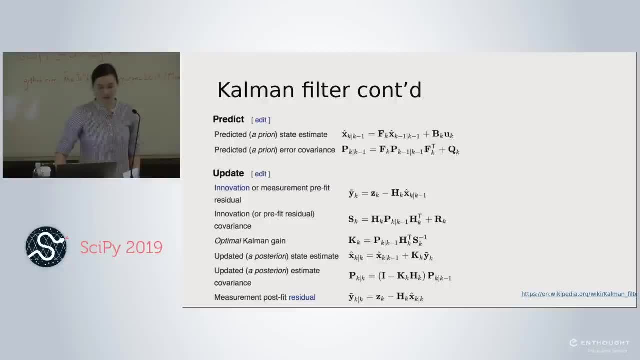 You usually won't have to code this up yourself, but it's good to feel empowered and able to do so. It looks really awful, but actually it's just a bunch of matrix, multiplication and inversions, so good to remember that You can look it up and code it if you want. 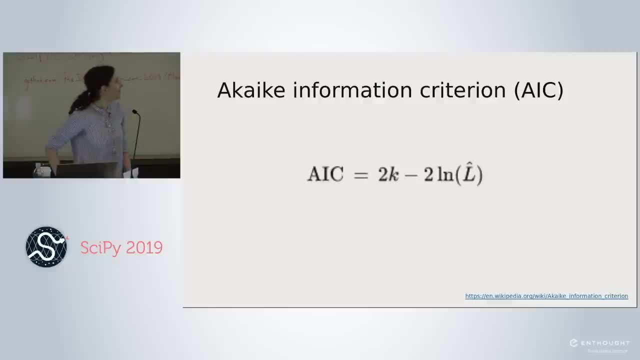 Okay, And then how do these models tend to get evaluated? Usually with your Akaki information criterion, your AIC. So just for anyone who's not familiar with this, I want to put it up: It's two times your number of parameters. 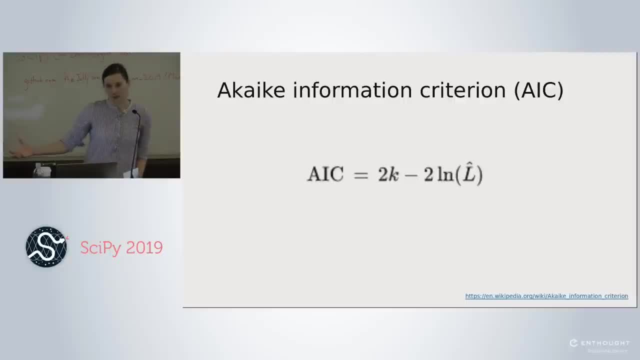 minus two times your log likelihood, right. So you want it to be more negative. when you're evaluating models, This is just one way you might evaluate models, such as states-based models. Okay, So here are some models that we're going to look at. 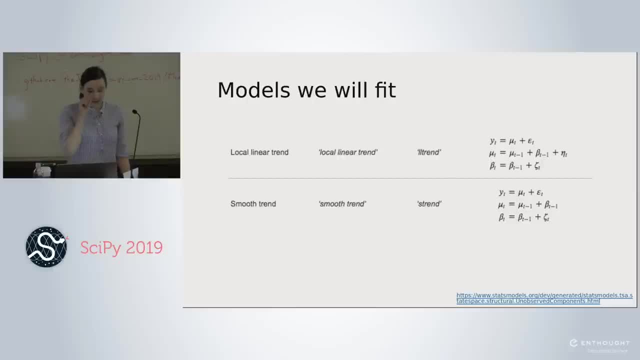 in a Jupyter notebook right after this. So we're going to look at things like local linear trend. so this I pulled directly out of the stats models package for the unobserved components model. So let's see, Can you see this? No, 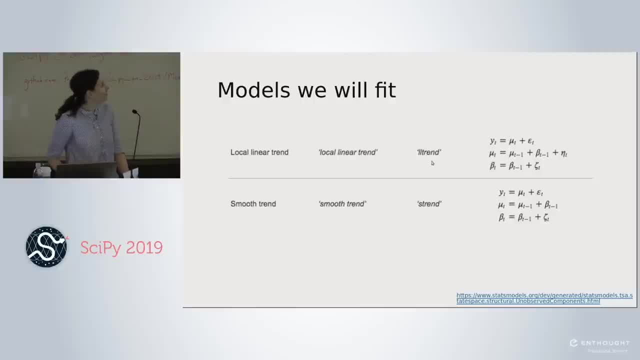 Oh, yes, here's my mouse, Okay, So it can give you either two ways to select these. Either of these can be your inputs, And then this tells you sort of the underlying model that it's using. So in this case, we have an underlying model. 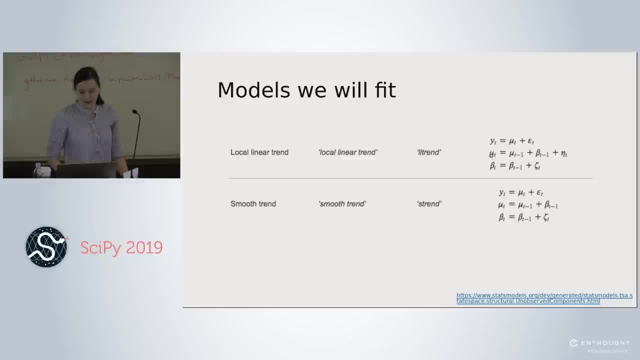 where our observable is some function of the underlying state plus epsilon, some kind of error, And then our beta itself is a function of its former state and also some sort of velocity-type term, some kind of trend term of where it's moving. That's our beta. 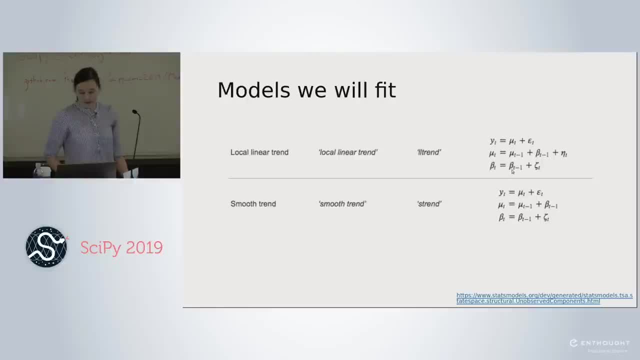 Plus some sort of error, And then our beta itself can change. So that's our local linear trend. And then take a look at the smooth trend and see if you spot the difference. They look quite similar, But there is one difference. So what's the difference? 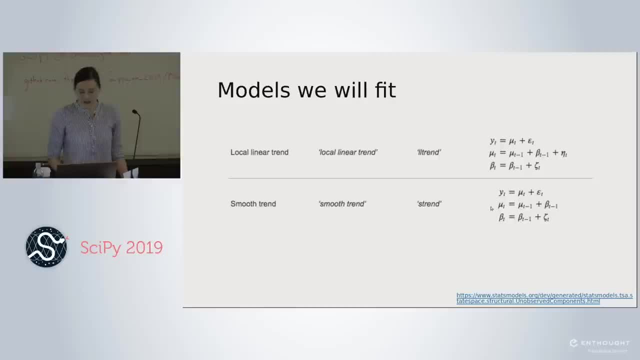 Yeah, right, So no stochastic term here. in the smooth trend In the middle equation, there's no stochastic term. So that's just to give you a sense of the distinctions that people make. People sort of make these slight tweaks and they have different names. 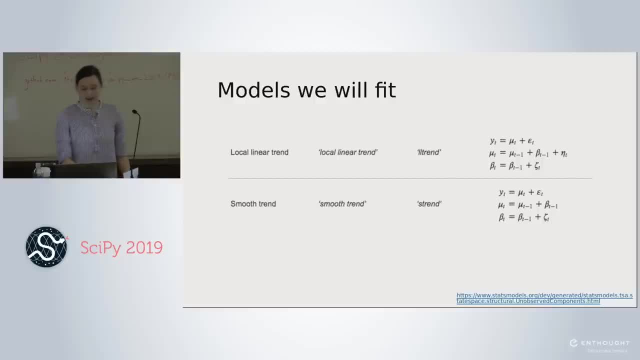 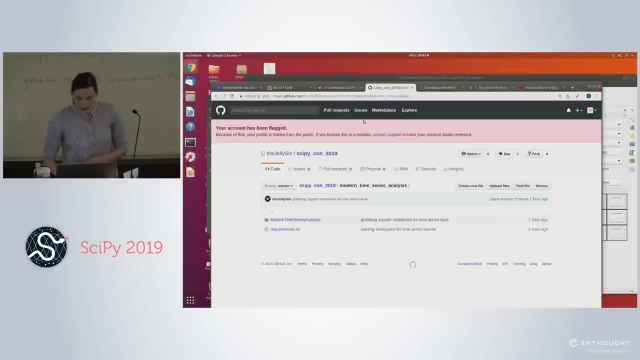 But it's always best to just go look at the equations to see what they look like. Okay, so now that I have bored your pants off with a bunch of slides, I think it's time to open the first Jupyter notebook. Okay, 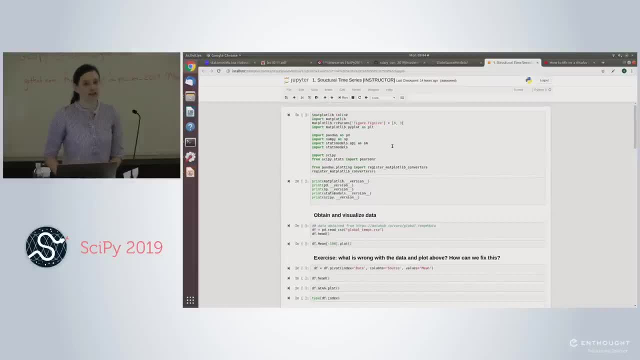 So people should feel free to use either the instructor or the student version. Student version is if you don't want to be able to cheat. You know that can be a good way to discipline, But you can be your own judge of what makes the most sense. 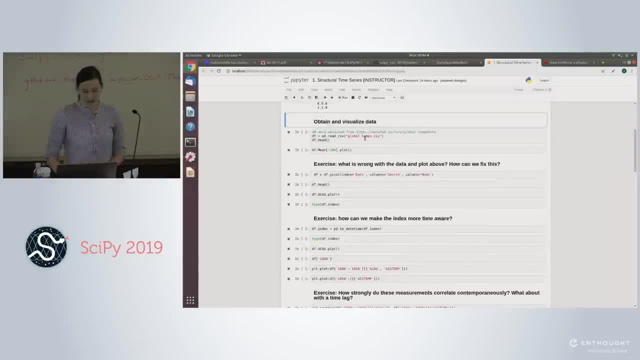 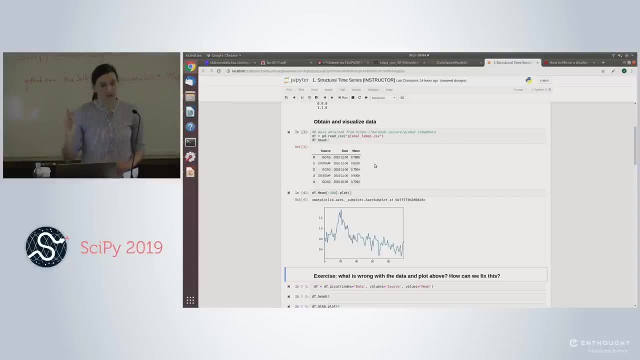 Okay, So the first thing we need to do is obtain and visualize our data. So in this case, I had downloaded two different measurements of global temperature data. Yes, Yes, okay. So thank you, Excellent point. So from the base folder. 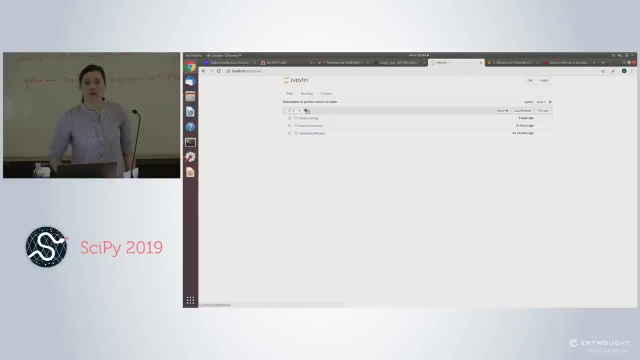 these are in the state space models folder. Okay, I'm sorry, So for anyone who walked in late. no worries, The set of Jupyter notebook slides are available on the Slack channel and someone has helpfully posted them here, So I'm the one who posted them. 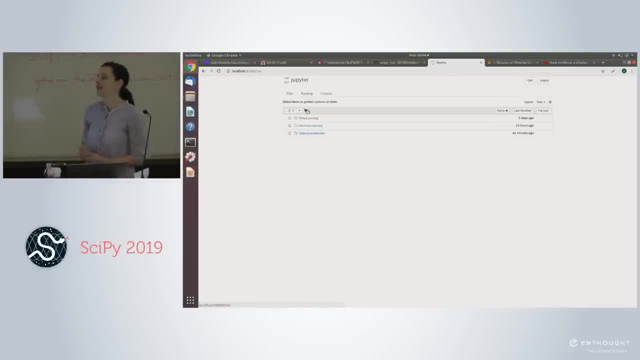 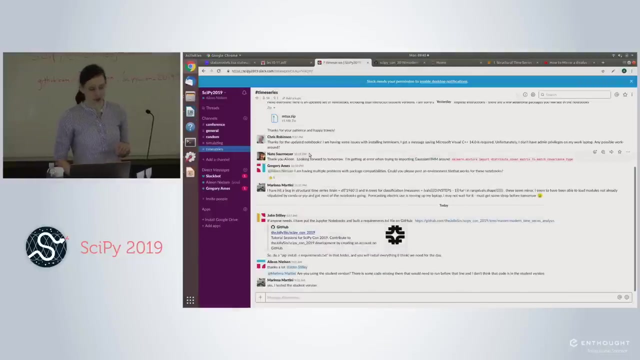 I guess whatever version I grabbed didn't have student versions. Ah, I see That's the older version. Sorry about that. Okay, I really appreciate that. So just want to confirm: do most people have the student instructor version? Let's see. 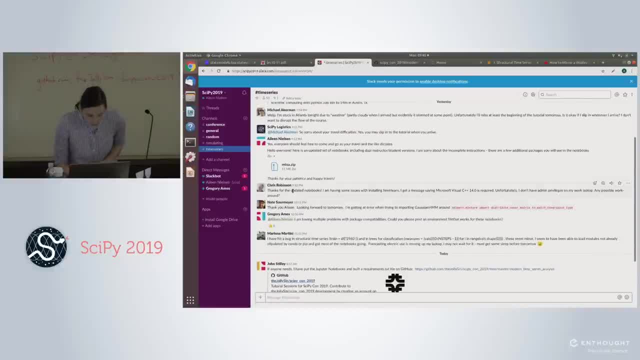 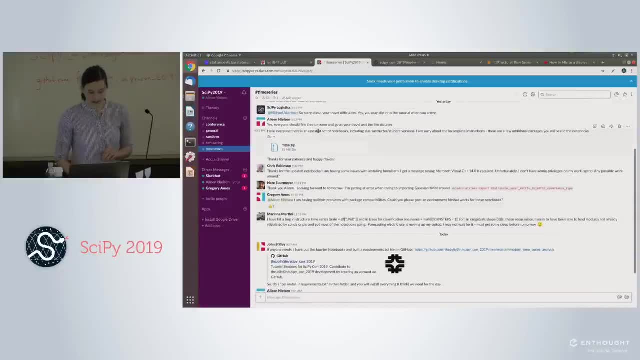 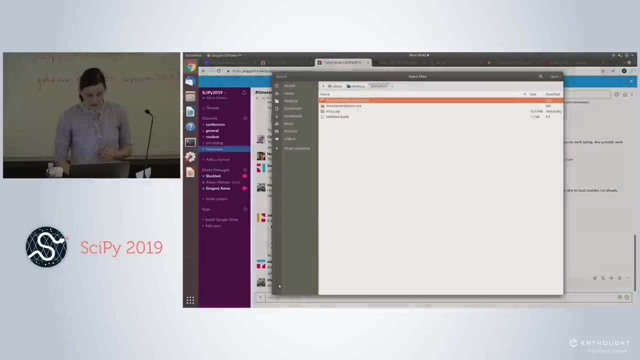 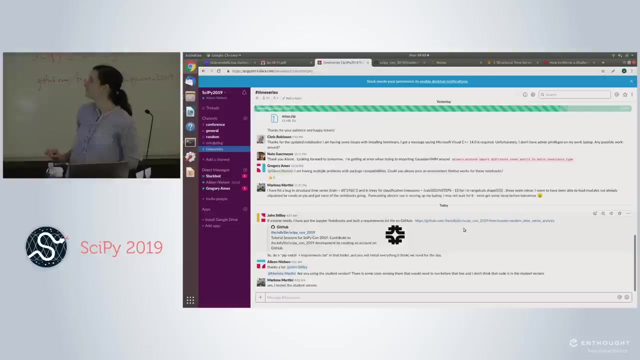 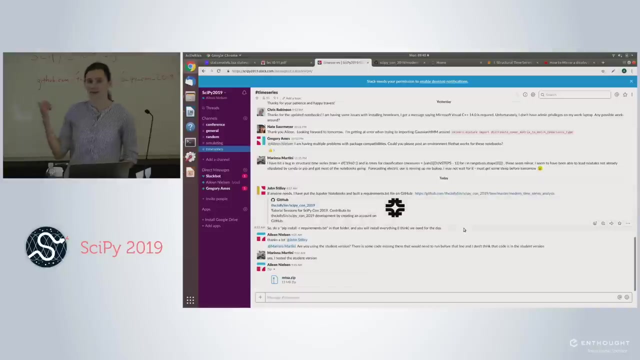 So if you scroll up in the Slack, this was sent at 9.13 pm last night. It's the second version rather than the one that's pinned, And I can upload it again, so it will be the newest thing. Okay, so that's the newest thing. 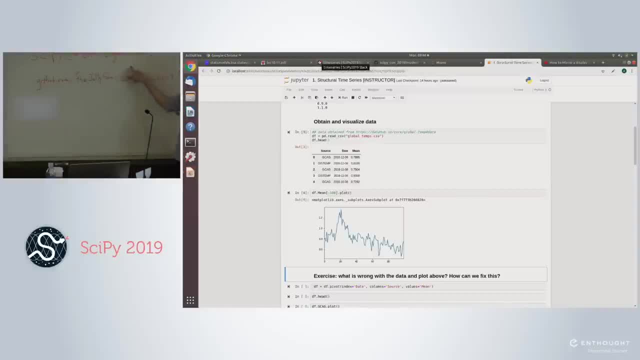 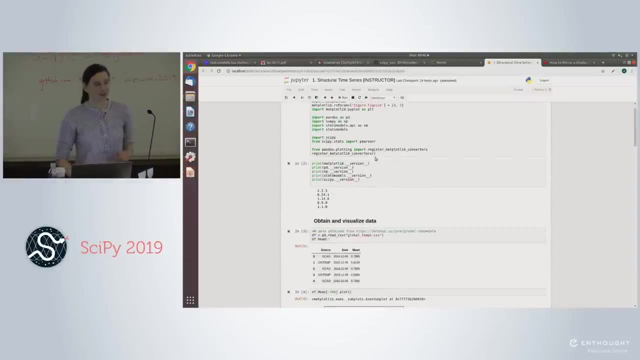 So in that case you should email scipy at nthoughtcom and they will just tell them that and they will almost instantly reply. I think someone's just manning that continuously. Other questions? Okay, Okay, so for those downloading, it's a pretty small zip file. 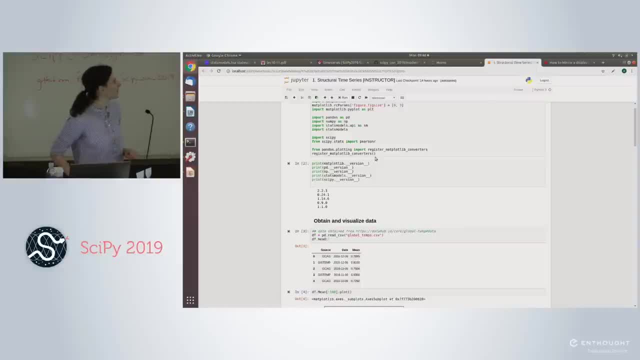 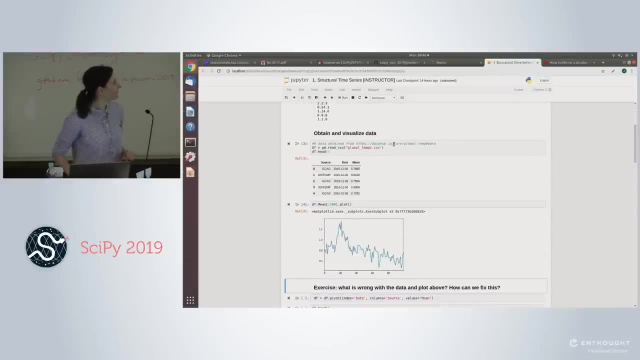 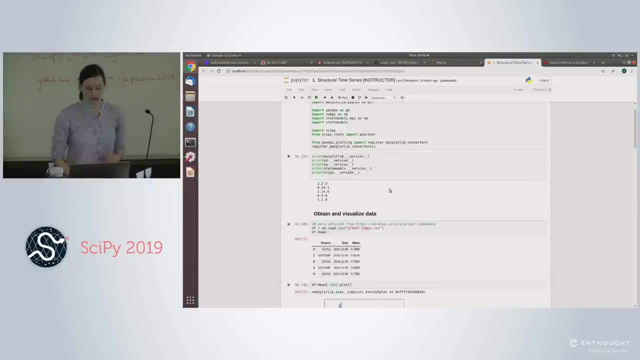 so I think you should have it pretty quickly. I'm just going to just slowly look at this data and you should be caught up pretty quick. Oh, GitHub is updated. Okay, great, thank you. So GitHub is also updated, if you find that more useful. 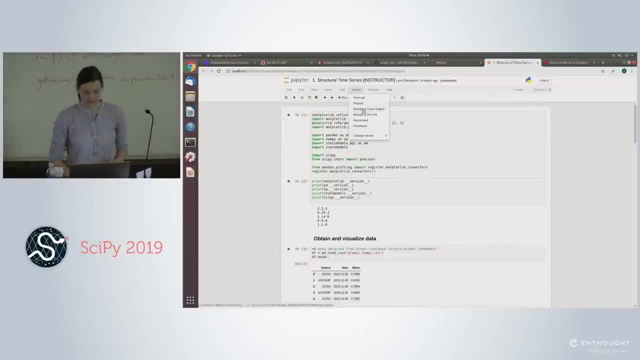 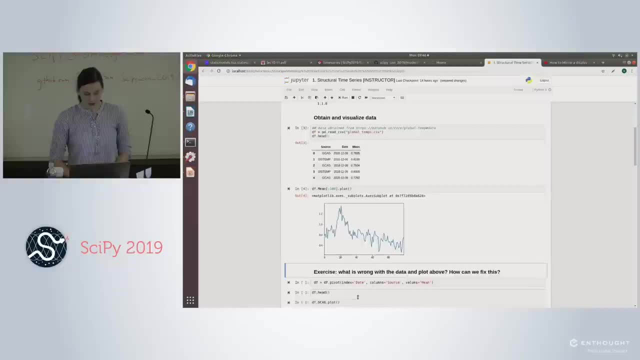 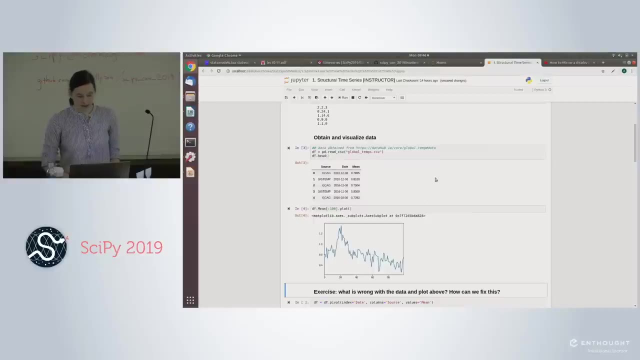 That's this, Okay. Okay, so we're just at obtain and visualize data. So this CSV should be available in the zip file and I have the source listed here. This is just two sources of global temperature data, Obviously, climate change data. 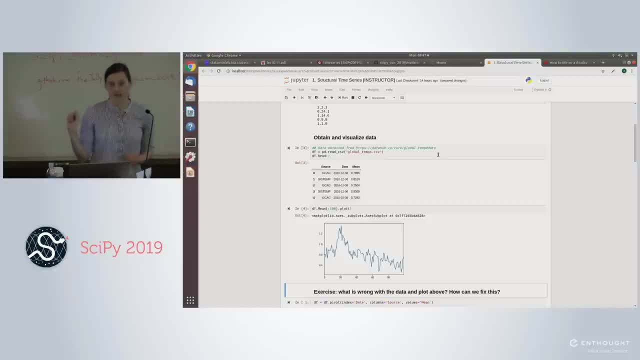 is a great source of arguing about time series, a great source of possibly ambiguous time series, depending on your politics, But it's a very important source of data. It's a very rich source of debate, so I grabbed some of that and the point of this data set. 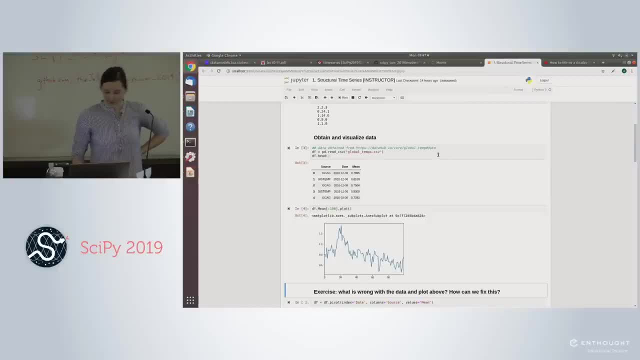 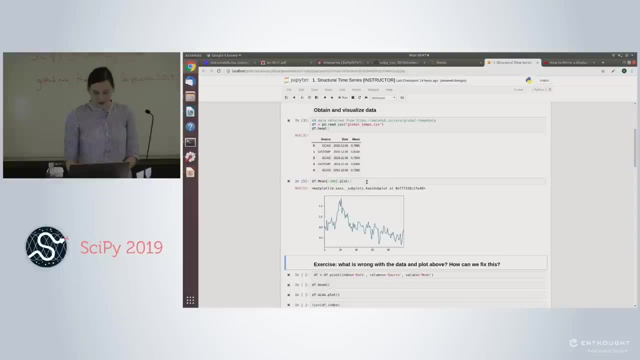 is they have sort of two sources of the data that we can compare. So if we load that data and take a look at it, the first thing I do is just basic time series plot. I also recommend sometimes that you don't plot the whole. 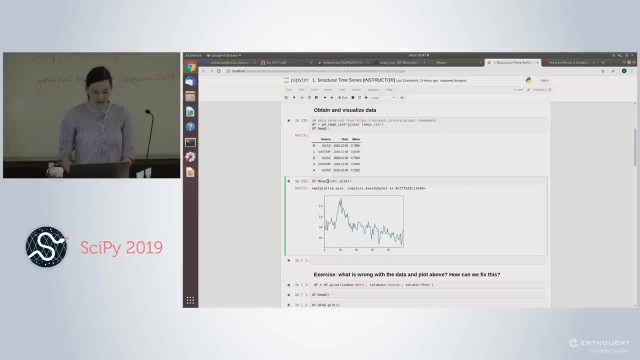 data set all at once. So, for example, here I just looked at the first 100 data points- I recommend that or why you might feel the same, That versus let's look at this one. Yes, Let's see. Maybe I'll zoom in. 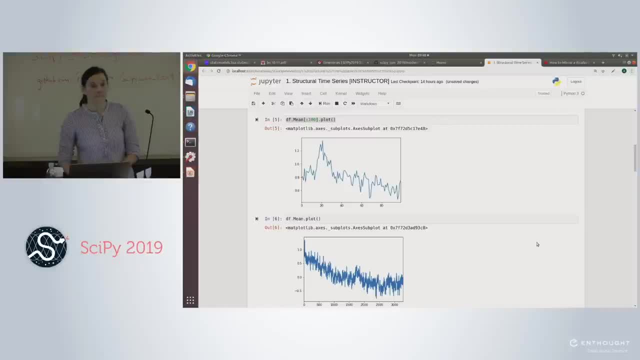 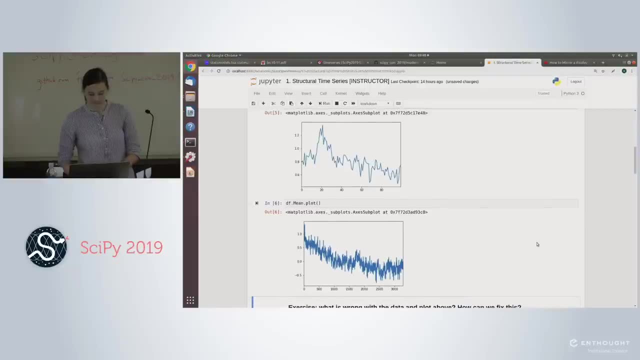 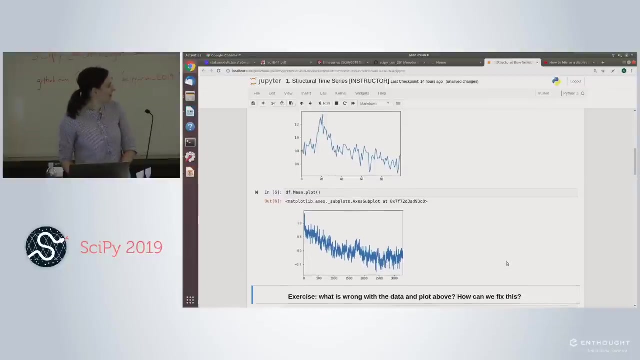 How's that? Okay, So I'm not especially satisfied with these plots. Does anyone feel satisfied with these plots? I hope not. Okay, So that's actually the first exercise I have for you. I'm not going to scroll up for those who want to have it be a secret. 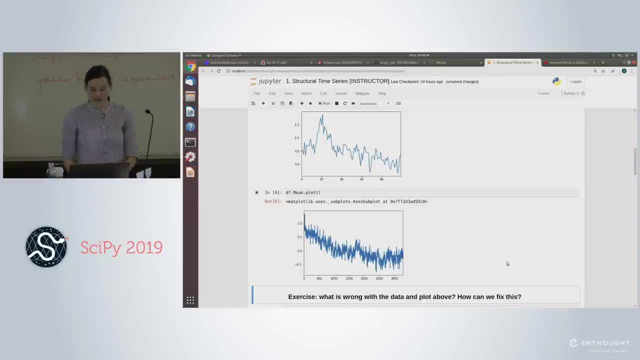 until you figure it out. But so the first coding exercise for everyone to figure out what's wrong with the way the data looks now and the plot and how can we fix it. Because it's not even just an aesthetic problem. There's an error right now. 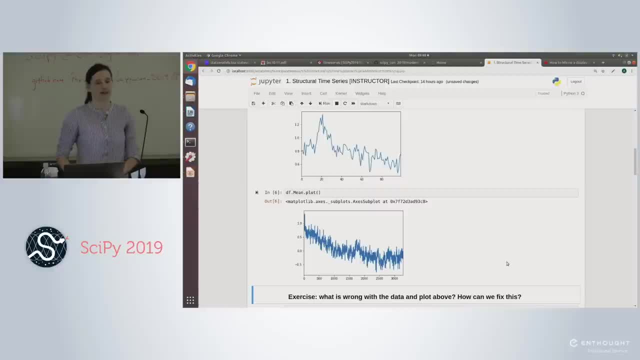 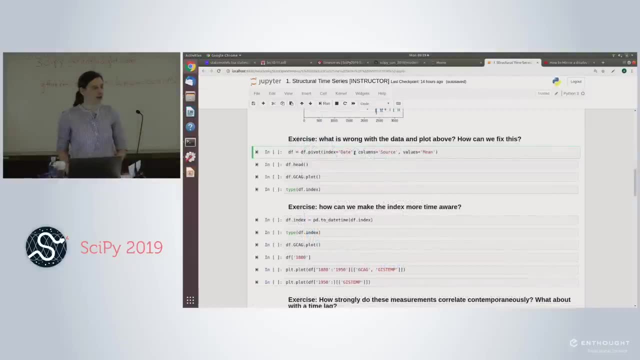 So this would be one of these. if I presented this to my boss, I should be really embarrassed in kind of situations. So think about what that is and how you could correct it. Okay, So I think we had already covered the problems, right. 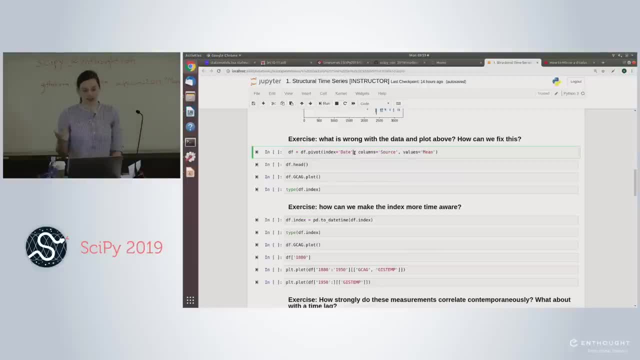 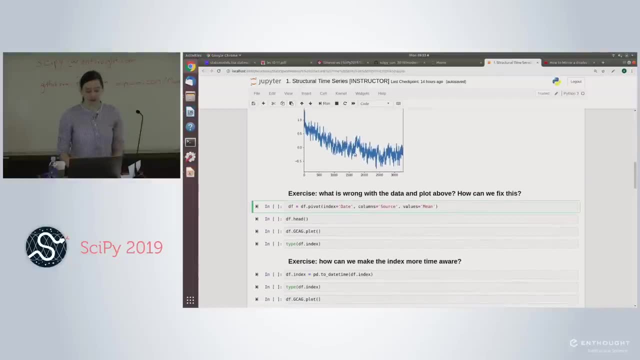 We've got data types that are not especially helpful. I should have been a little wary of that, given that already even in my plot. I don't have time displaying right. I have just sort of a random index. So the first thing we're going to do 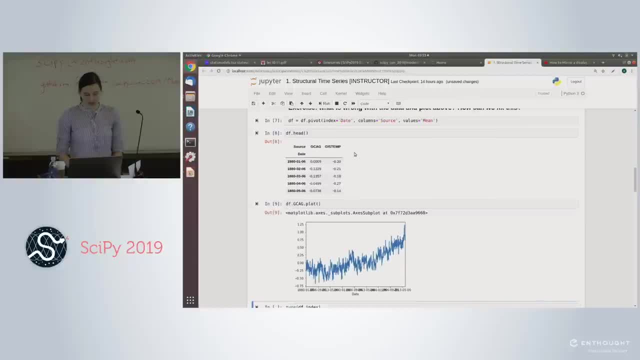 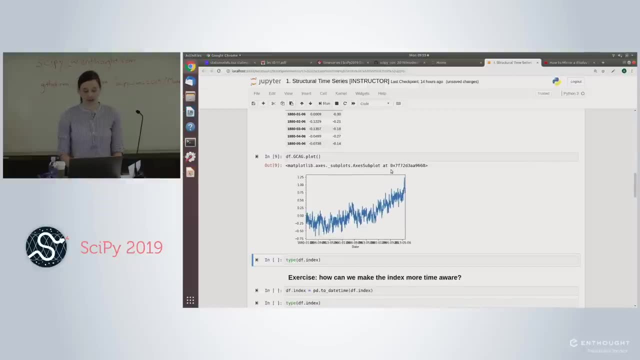 is we're just going to pivot our data And then, if we plot our data, incidentally it seems like that has reordered our date index appropriately, and now I'm seeing something more like what I expect. And now I'm looking only at one type. 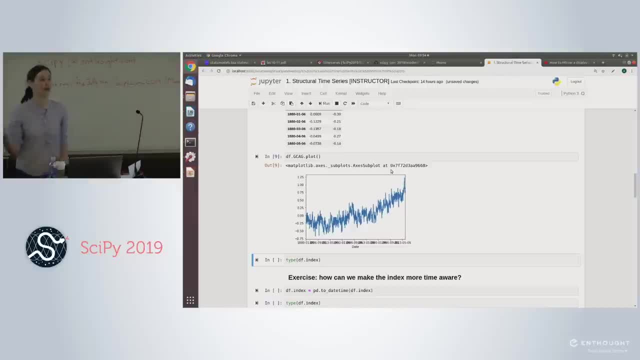 one time series instead of two. right, I actually have two time series in my data set. I should not plot them as one. Unfortunately, often- and this is something that's tricky about time series- you can be plotting it the wrong way and it will still look reasonable, right. 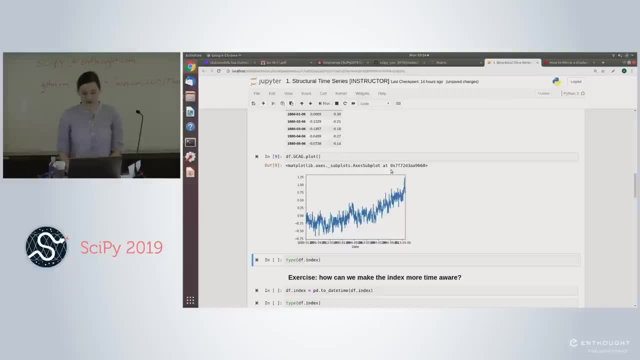 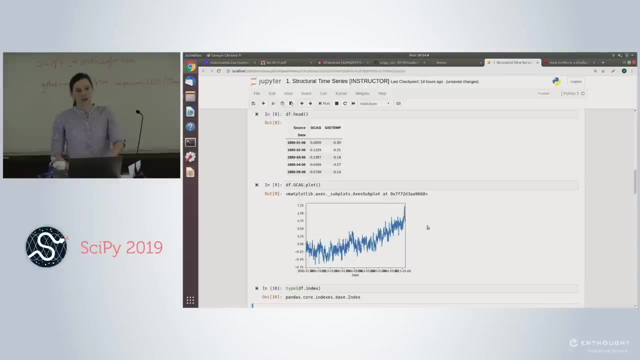 Especially if I didn't have domain knowledge about sort of global warming. that would have looked fine to me, and maybe I would have foolishly carried on. Another problem though: is I still so? now my dates seem to be in order. right, I could check more extensively. 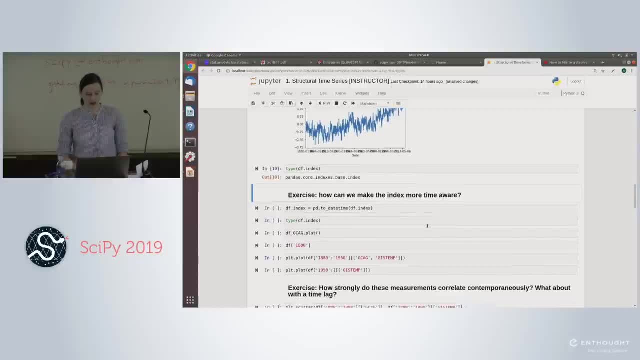 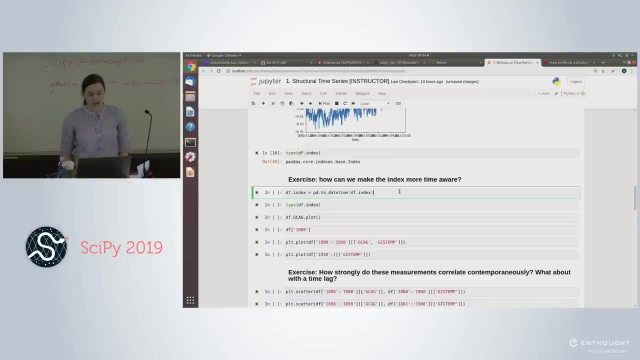 but they're still only useful as an index, whereas I would like something a little more useful. So let's just go through this. I won't do this as an exercise. How can we make the index more time aware? Well, nicely, pandas provides date time. 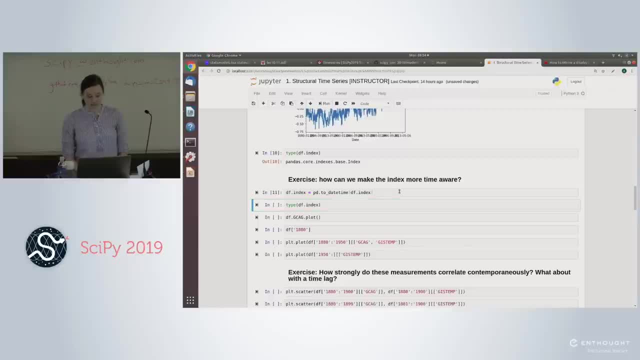 and also period time indexes. so we're going to use date time And if we do this, we see we now have a date time index instead of a base index class. So what do I get from that? Well, already, notice, compared to this plot, 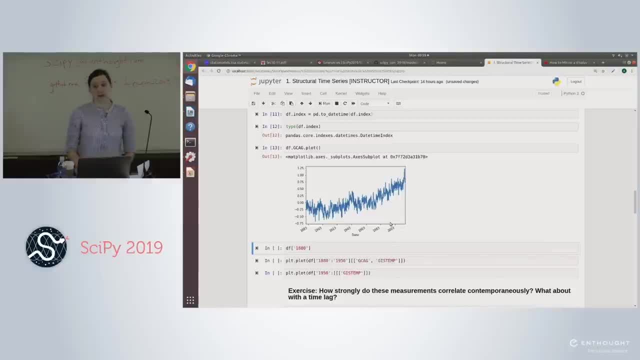 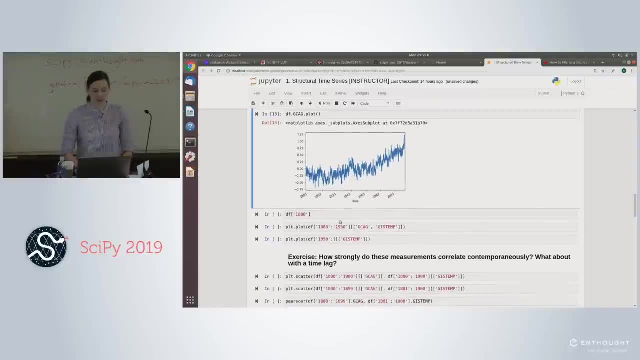 which I already thought was okay. I've now got a plot where these are not being treated as strings, they're being treated as actual dates, and so pandas can fill in a little bit of background knowledge if they're reasonable. And then I also get sort of handy indexing like this: 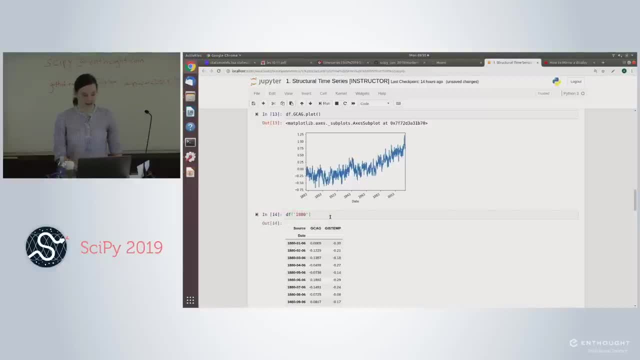 so now I can now index, say by year, right, Just df1880 is going to show me all the 1880s, which also is just going to make my life easier. I can do some plotting like this. so now I plot both series from 1880 to 1950. 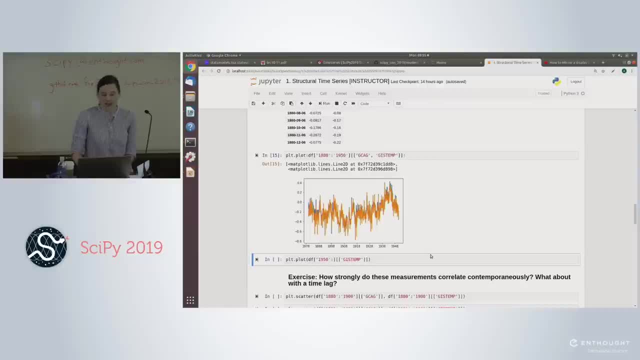 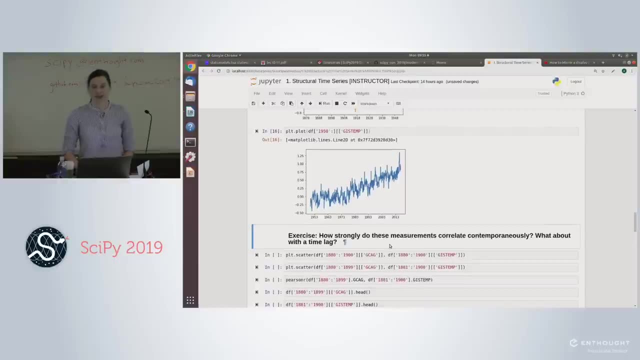 and get a sense of how correlated they are. Or I can just plot everything from 1950 onwards and again get all that nice functionality with the date time. So this is just a reminder that that's available to you and it can be very helpful. 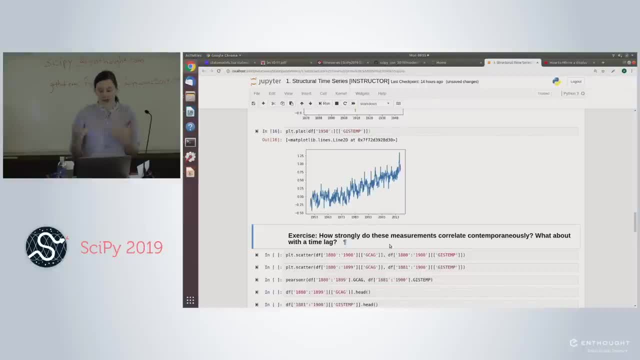 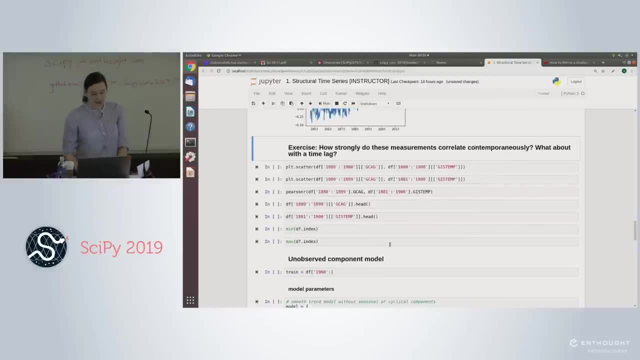 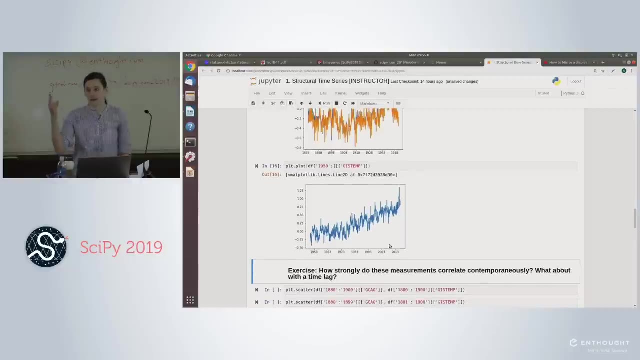 So I'm going to go ahead and show you how to do that, And obviously always look carefully at your data before you get started. Okay, so quick exercise: How strongly do these measurements correlate contemporaneously? What about with a time lag? So now we've got two groups of data. 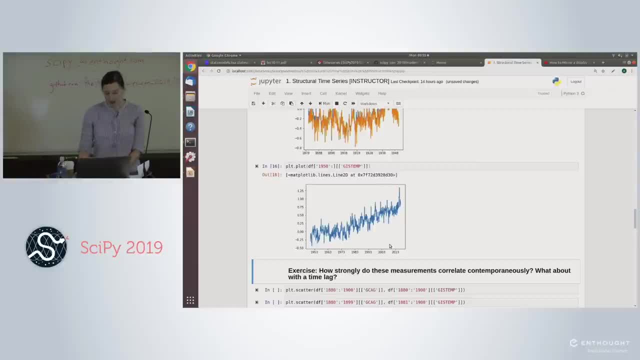 Just quickly, two minutes. How helpful are they for predicting one another or for understanding one another? It can depend a lot on from one package to another. I guess one critique I would even have of the Python space is there's not a lot of uniformity. 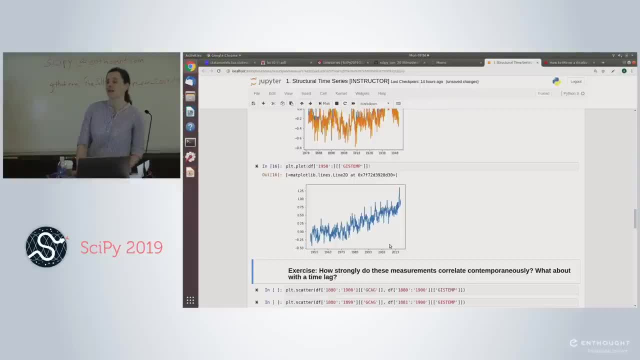 around this because the functionality is spread out among many packages, And not to be anti-Python because Python is my favorite, but not to be anti-Python because Python is my favorite, but not to be anti-Python because Python is my favorite, because Python is my first love. 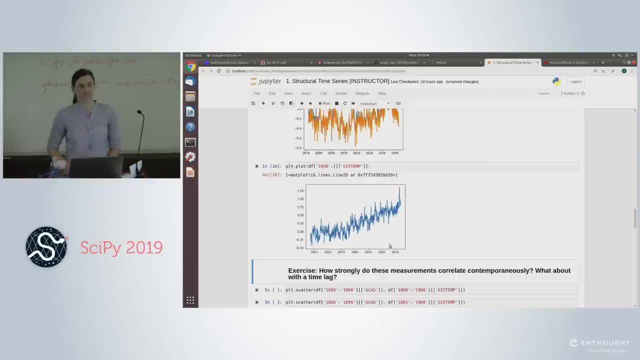 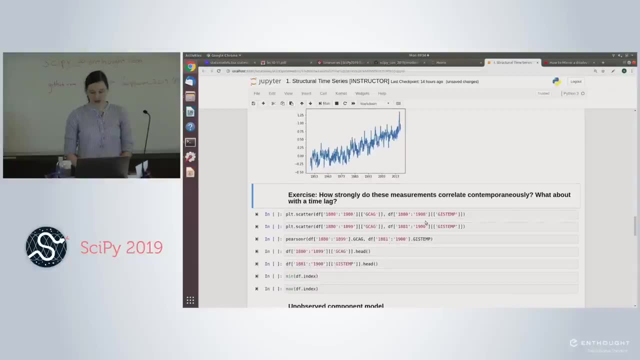 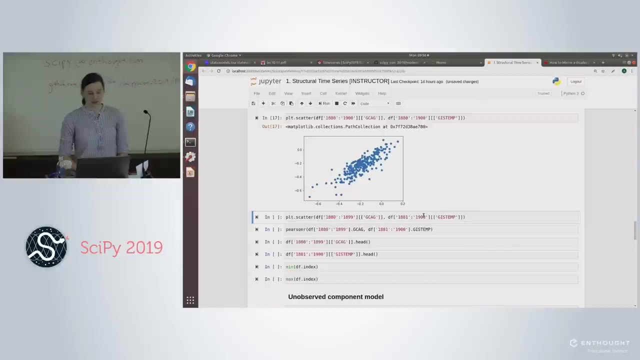 but R actually does a better job of having more of a unified interface. Okay, so how strongly do these measurements correlate contemporaneously? There's all sorts of ways to think about that, But just want to point out we can just do simple things like scatterplots, right? 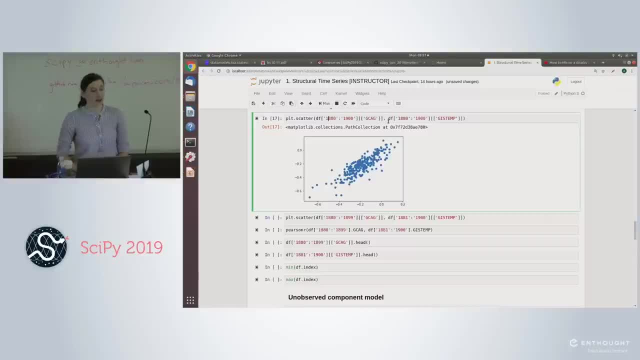 So now I'm plotting the two measurements, the GCAG and the GIS temp, against one another for the exact same time period. They seem to correlate pretty strongly. If I saw something like that at my work more often, I would be delighted. Similarly. 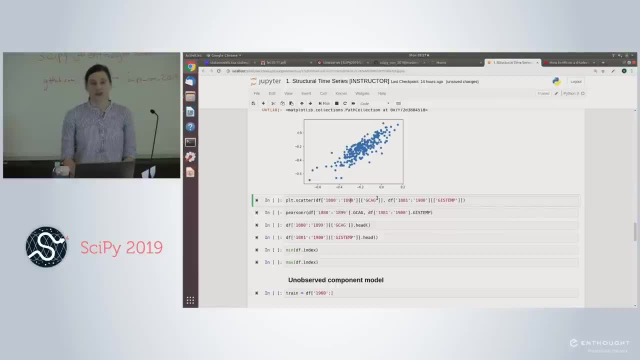 we can ask: what about with a year's offset right? Do these have any sort of predictive value for each other? So in this case I'm plotting 1880 to 1899 for one variable versus 1881 to 1900 for the other. 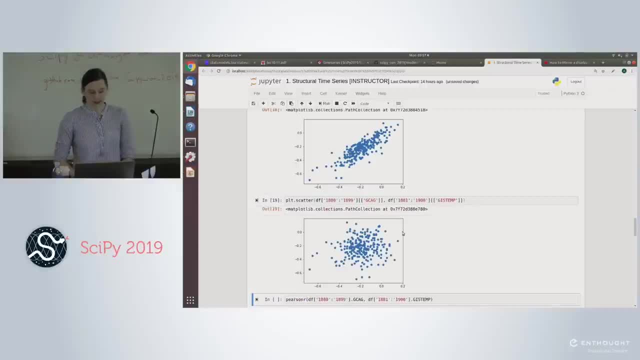 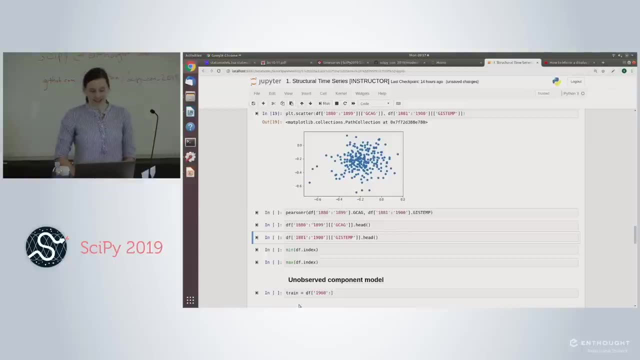 So I've just offset it by a year. What does that look like? That begins to look more like the real world than what I see at my job anyway. But is it terrible? Well, it depends on your domain, right? Maybe for predicting air passengers. 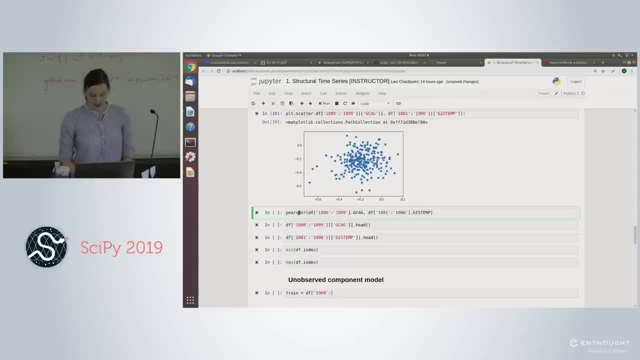 this would be terrible, Maybe for predicting housing prices. it's not so bad. We can look at the Pearson R and we see it's not zero, right. I mean, actually this probably looks worse than it is. So it can also be good to have different measures. 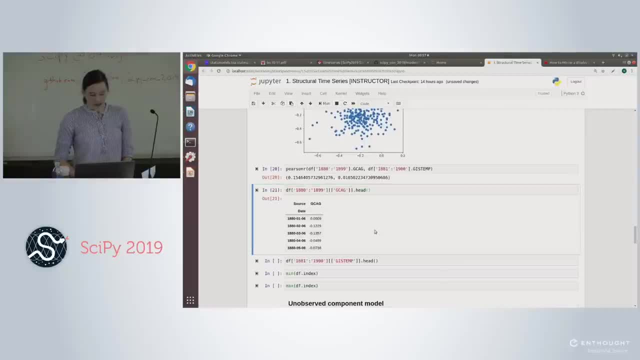 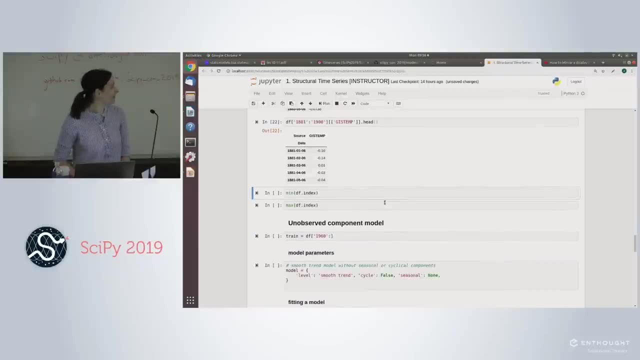 visual and numeric. And again, just as a reminder, we can sort of look at the data with standard, standard tools from Pandas. We can look at an idea of our date range. We can look at our min and max for our index right. 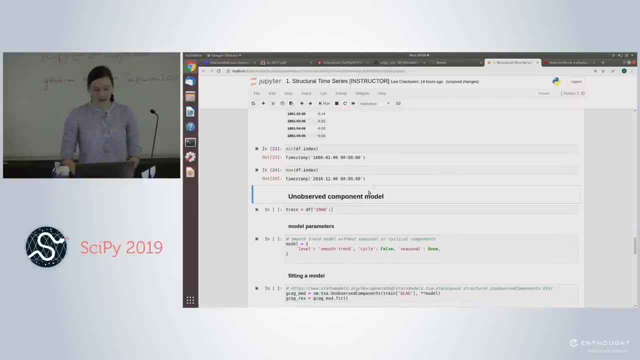 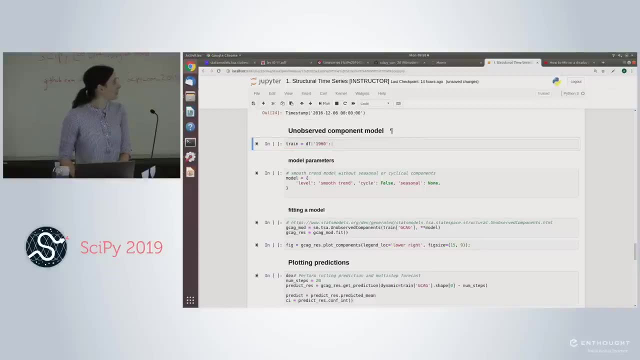 So all sorts of standard operations, Okay. so now we're going to throw this into an unobserved component model. I'm only interested in training on the data from 1960 onwards, Just personal choice. I thought that's a little bit more interesting. 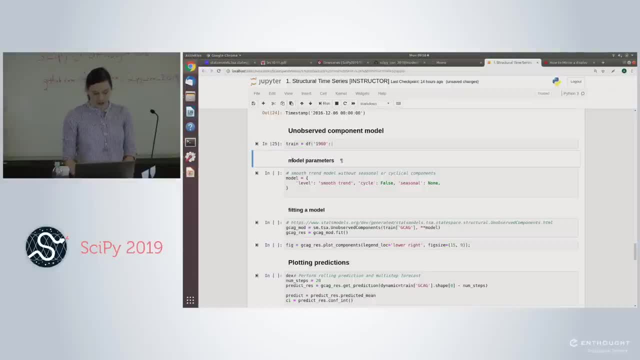 That's sort of where we see things taking off. We're going to define our model, So we have our model parameters and all I'm going to say is: I want a smooth trend for my level. I want no cycle and no seasonality. 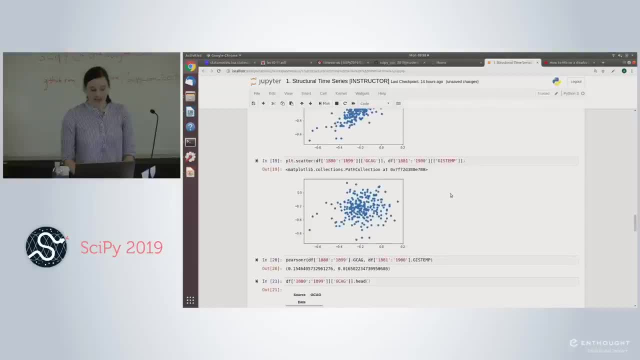 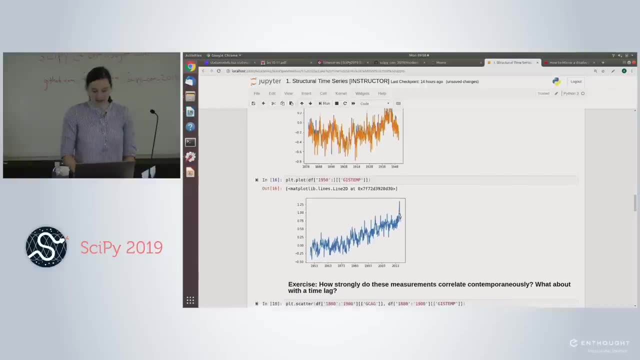 That's sort of my first pass based on these plots we did here right. So looking sort of at 1960 onwards, I'm like, eh, I don't know if I see much cycling or seasonality Arguably, I could be more careful about this. 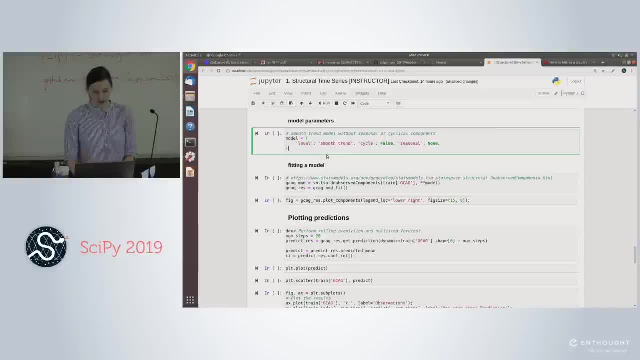 but this is going to be my first pass, So I build my model with a dictionary. I fit my model, so I'm going to make an unobserved components object from stats models, right? So stats models has a whole time series analysis API, including a state space. 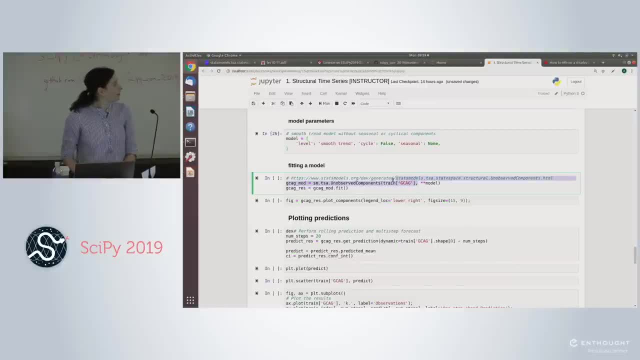 API with unobserved components. I give it my data and I just give it the model to unpack, right. And there's other sort of parameters you can tweak and you can read up about those in the documentation. but this is as simple as it is. 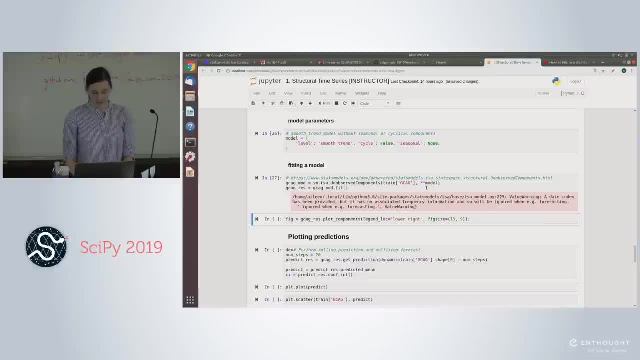 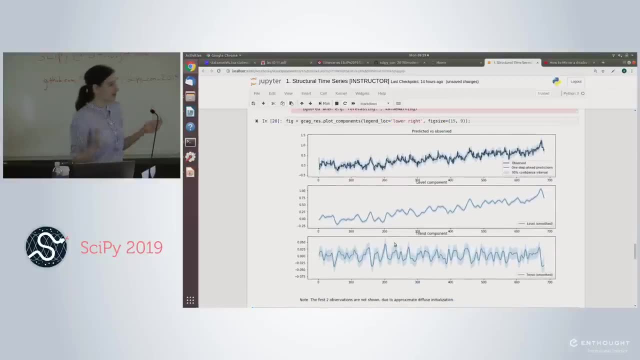 for a first pass. I'm then going to fit my model and I'm going to plot the components right, Because this is what I was talking about as being the great thing as compared to an ARIMA. Okay, so I've plotted my components. 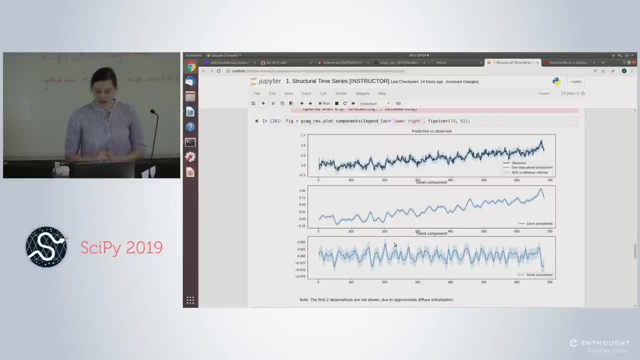 Let's see here I've got my predicted versus observed plot. So how do we feel about this fit Seems like we're always within our confidence interval. Seems to follow pretty well. This is a one step ahead prediction, right. So you also would want to think about whether 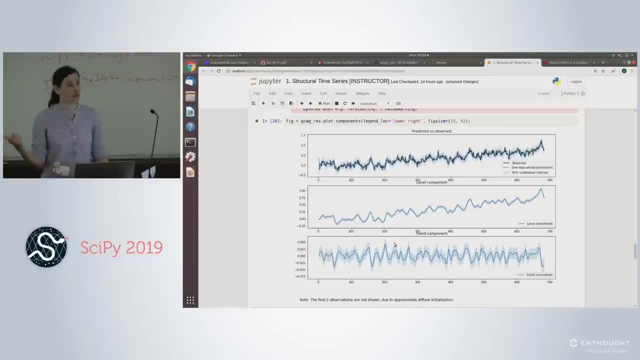 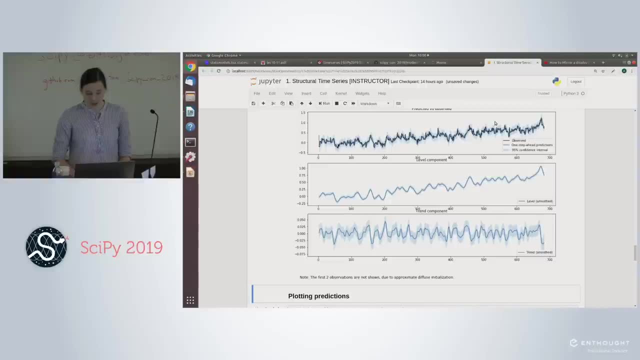 that's sort of interesting to you. Is it interesting to predict global temperatures one month in advance, or would we like to try more? We'll try more below. We also can look at our two components right, So we have a level component and a time component. 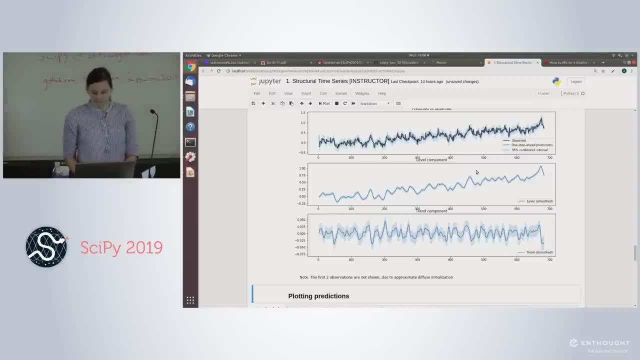 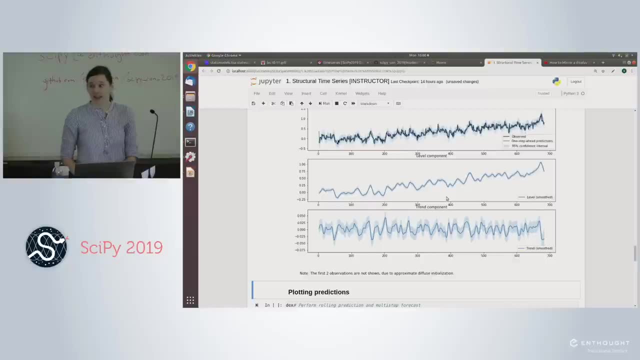 What do we think about these? How do these look? compared to what I showed you in the PowerPoint? I would say not great, right? They both sort of look like wiggly lines. I would say that I don't get a whole lot of. 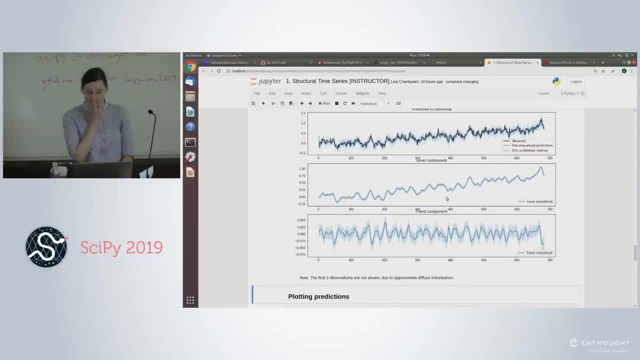 insight out of this. When I look at it I say, hmm, level versus trend, I mean they both. it looks like, hmm, okay, the model mostly gives the absolute value of the time series to the level, and then it's almost. 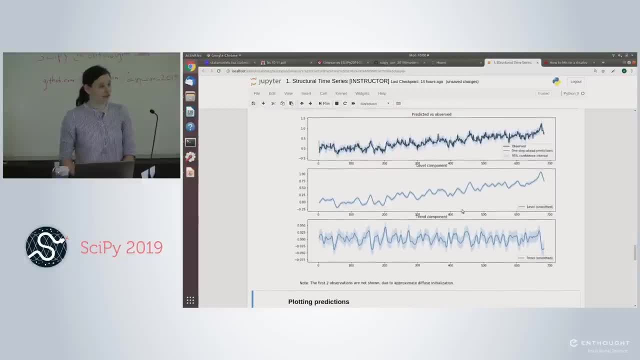 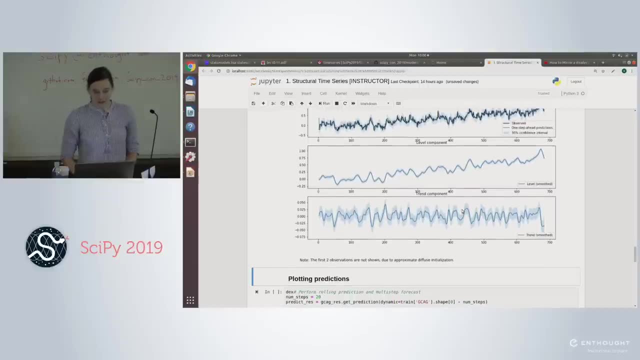 like the trend is just whatever was left over, but it doesn't look like a meaningful trend. So, thinking about that, I think, okay, well, let me revisit that, And we will revisit that in a couple of steps. We might also want to. 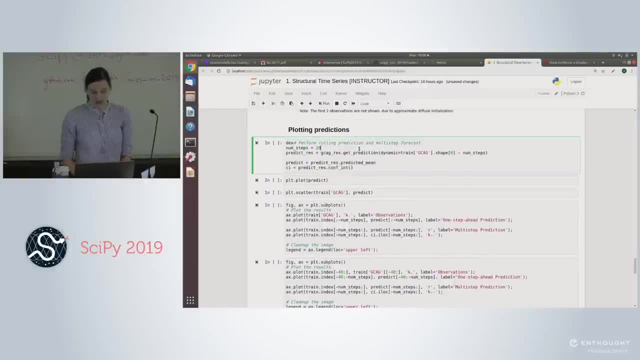 plot our predictions. So to do that, we can also set a greater time horizon to do at the end, to do dynamic predictions. So if you move down to the next cell, I set the number of steps I want to predict forward as being 20,. 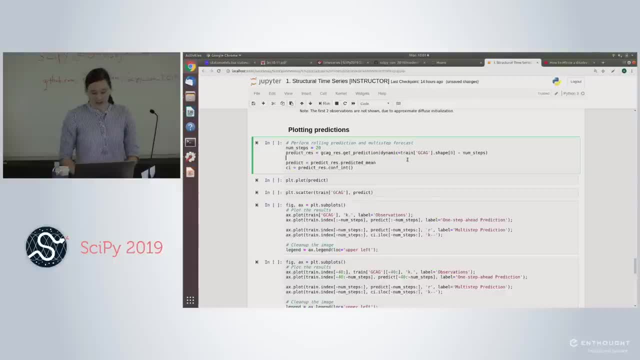 so 20 months, arbitrarily chosen. So now I want to get predictions and I want to do the last 20 steps as dynamic, meaning that now I'm not going to update at each step. right, That's when we do our one step ahead forecasting. 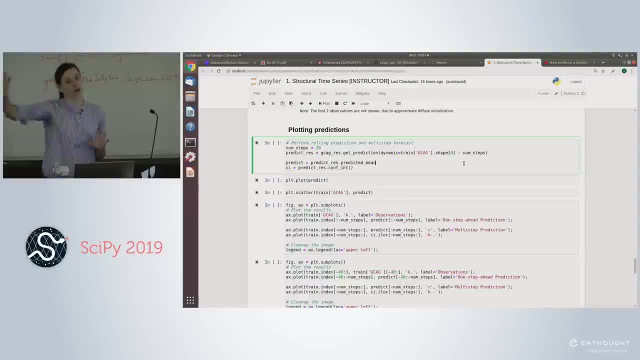 Now for my last 20 steps. it's just going to roll with those 20 steps. It's just going to take what it predicted, and that will be its new input. Take what it predicted, that will be its new input, and it's going to move forward. 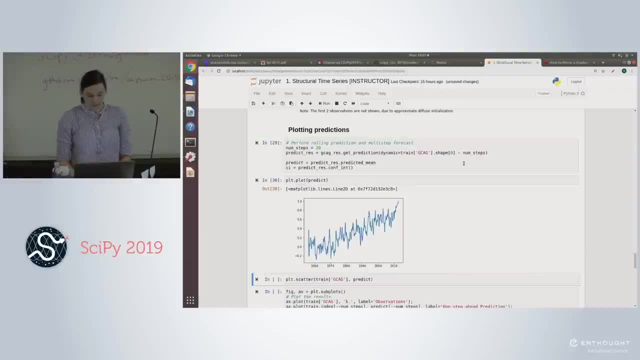 So if I do that, this is what I get, And I want to draw your attention to the end. What do you notice at the end? Sort of this upper right hand corner. It's just sort of a flat line, right. 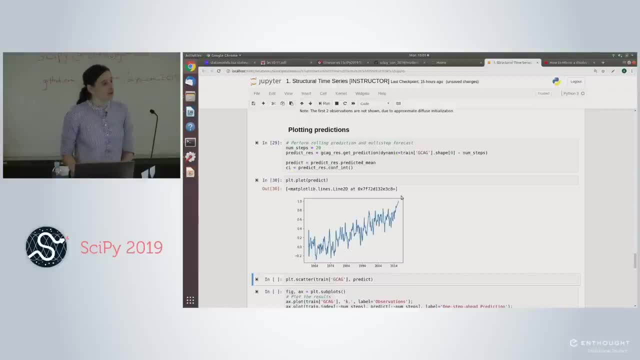 So that's another thing you're going to notice with these models, to be aware of, right, When you're doing sort of multi-step horizons, they're not so great in the sense of, since there's no error, they'll just assume there is no error. 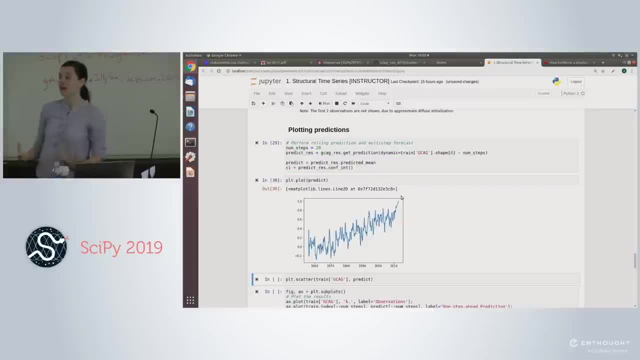 and they're just going to sort of keep going along whatever smooth trajectory is established by the underlying model. That can be a good thing or a bad thing, depending on what you want to do. This certainly will look a little bit different, especially from an ARIMA model. 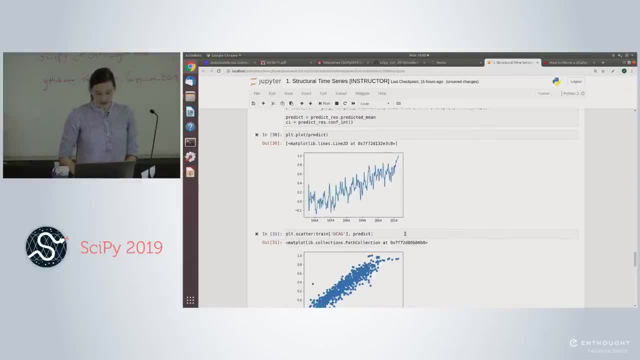 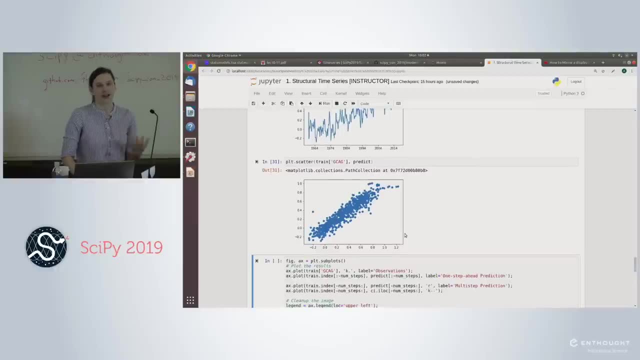 where you will sort of see more wiggles and things like that. Okay, and then how does it do? How does this model do? Well, it looks pretty good for one step ahead, right, But can I really decide if it's really good? 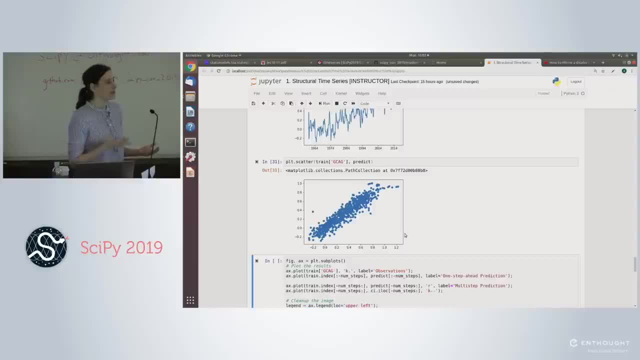 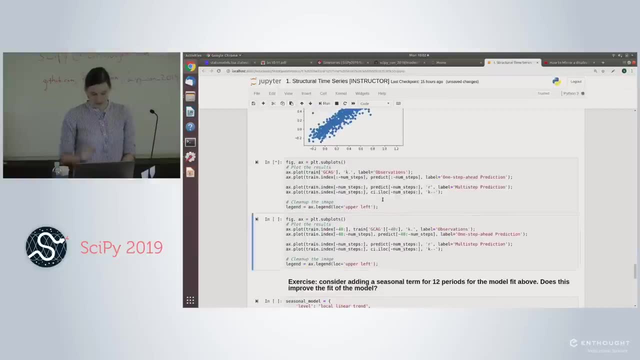 just based on one plot? Well, no, especially if I'm not comparing this to what would my null model look like? right, I need to think about what my null model would look like. You can also do a cleaner plot. So this is just to illustrate. 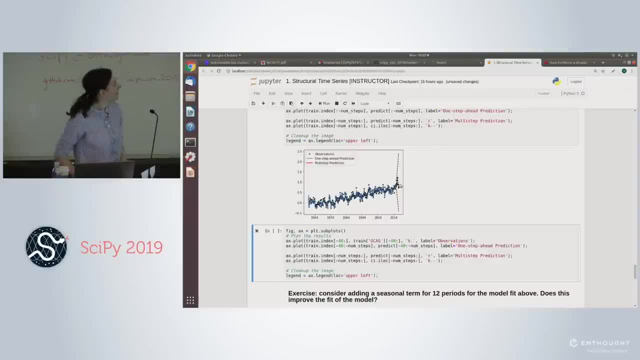 if you want to put in confidence bounds Again. this red now is showing your dynamic prediction. Your dotted lines are showing your confidence bounds. They don't look fantastic either, right? So here's another difference compared to if you're used to an ARIMA model. 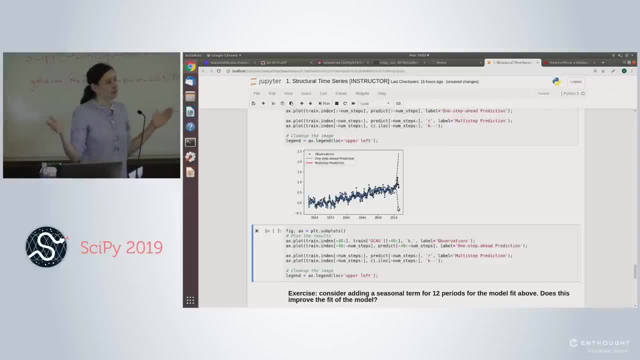 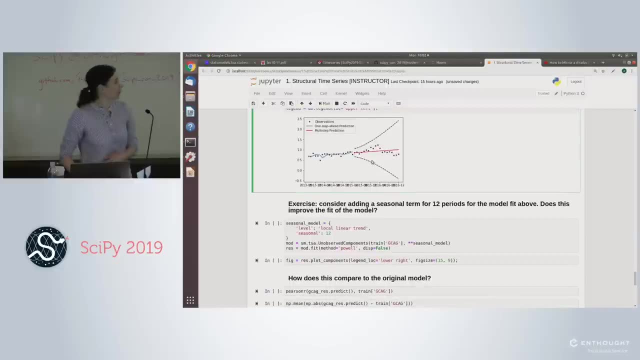 Your confidence bounds will rapidly diverge because of this unincorporated error that you're no longer able to handle. And we can look at this also more up close to get a sense And as you can see what we discussed: your forward-moving prediction. 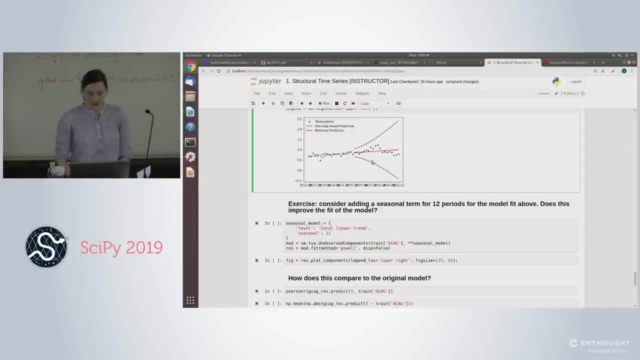 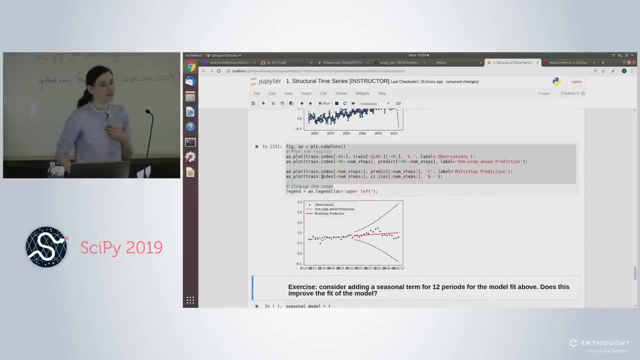 is just going to be a flat line for these simple models. So next exercise for you all is consider adding a seasonal term for 12 periods to the model fit above, And does this improve the fit of the model? So we had initially rejected seasonality. 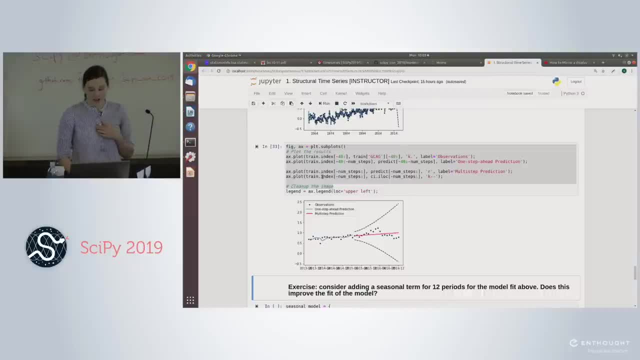 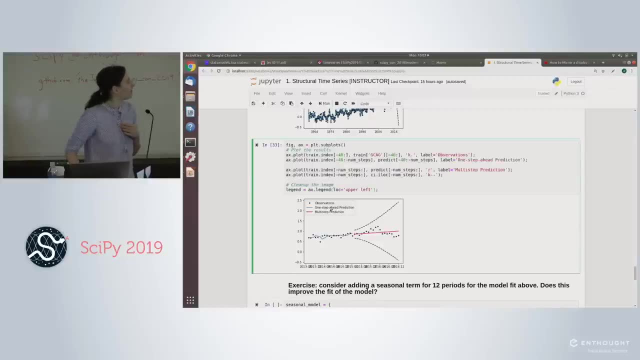 but should we revisit that And how do you do it? If you're not sure, go to the Stats Models API. You can Google that and look for the unobserved components documentation. So let's take a couple minutes to look at that. 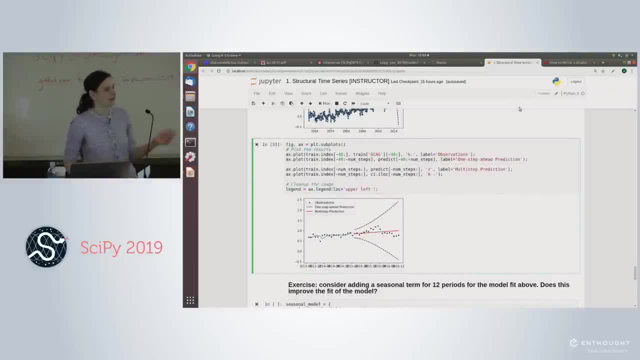 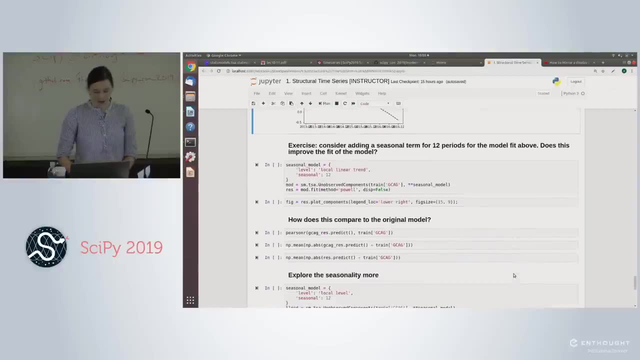 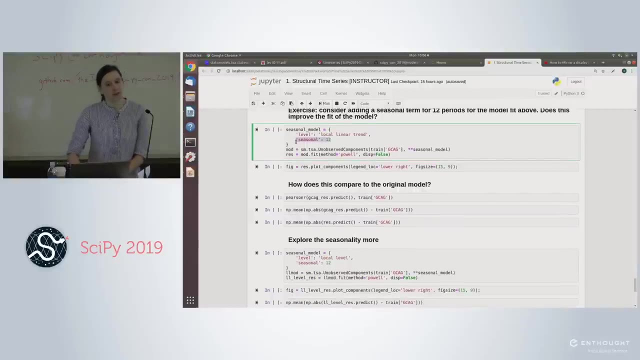 So also I've just posted the slides. I had a request to post slides, but they're also in the time series channel, Okay, so how do we add a seasonal term here? We keep a local linear trend and now we add a seasonal parameter. 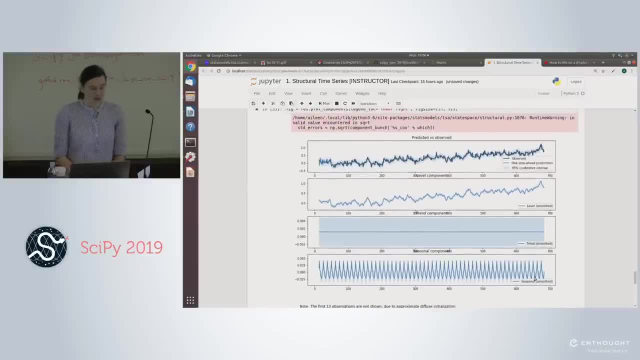 And if we now plot our components, we see something interesting. now, right, So we see what looks like a very regular seasonal component, which again shows how silly I was not to have done more exploration of my data at the start when beginning to think about what kind of model. 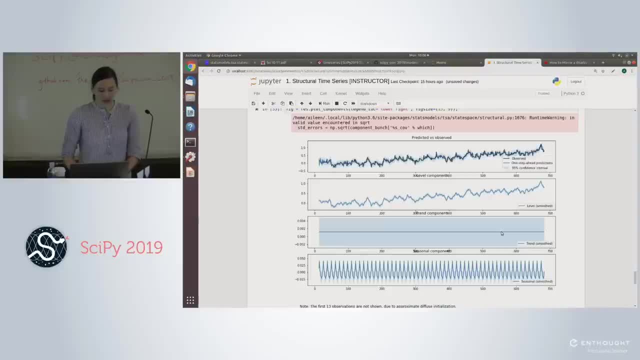 would be appropriate. We also see now that sort of the trend component has gone to just this negligible thing. It's not really adding to the model. We have a level component and a seasonal component and that already seems to do a pretty good job. 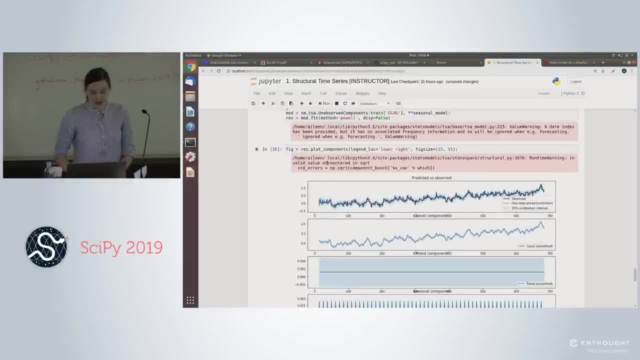 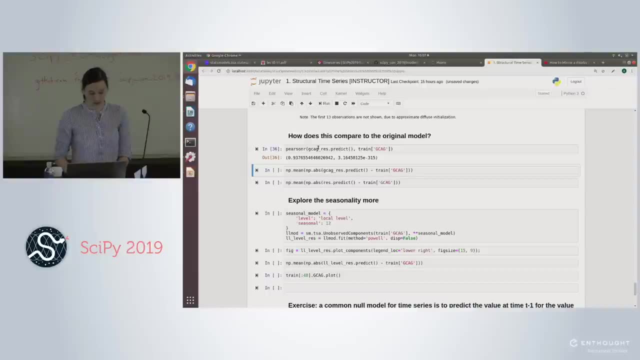 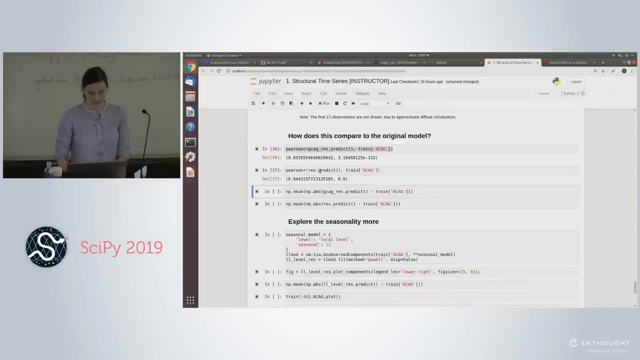 So how does this compare to the original model? If we wanted to compare them, we might think about, for example, comparing the correlation of the two models with the data, And we see these are sort of indistinguishable right. So that, to my mind, 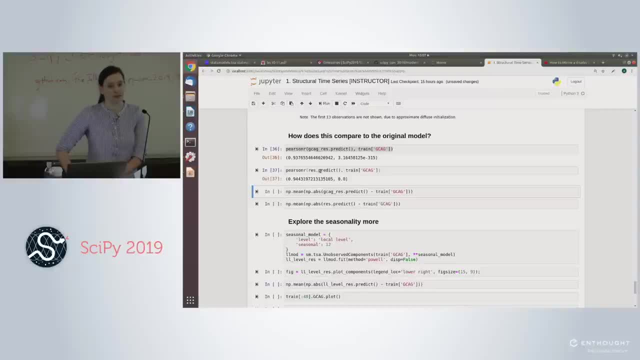 is not a very helpful metric and shows how we should be skeptical, because visually clearly one was doing a better job of describing the data. so that shows sometimes that these numerical measurements might not be very informative. And what about if we look at the mean absolute error? 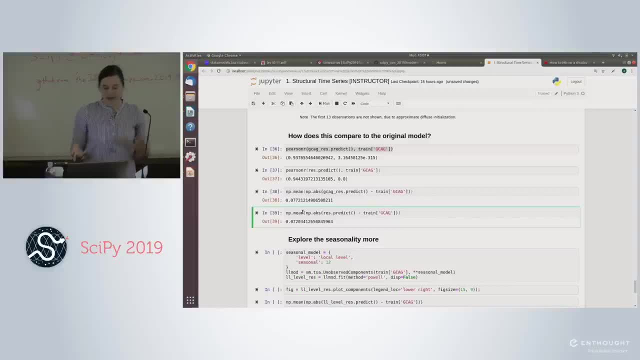 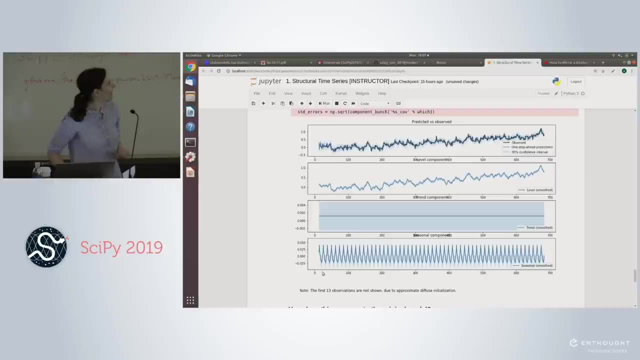 In that case. in both cases, we see that the new model does slightly better. but, yes, Okay. so if you look at the, I'll go up and hopefully you have this in your notebook as well. This is the seasonal component. 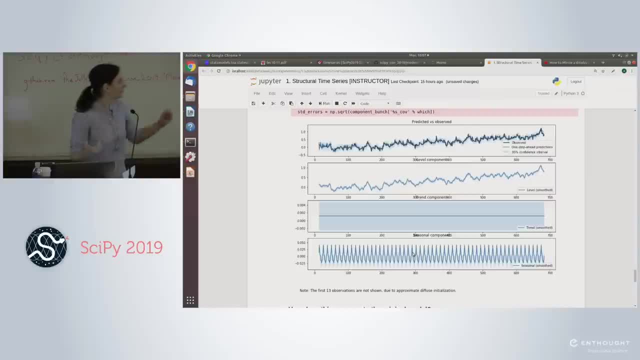 So the seasonal component is zero. It's clearly significant and it's showing sort of a pattern that makes sense based on our domain knowledge of some kind of 12-month cycle of the Earth's temperature. Okay, I'm glad people are just interrupting me. 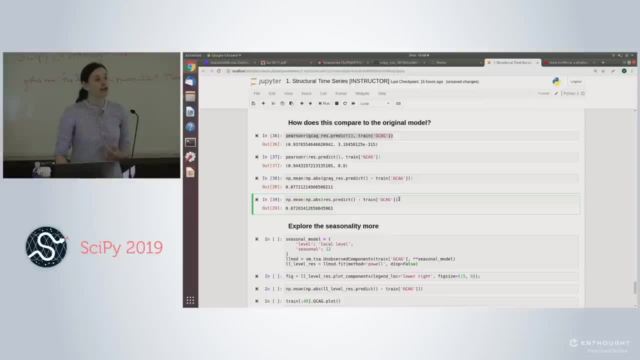 whenever it's helpful, because that's what this is about. Okay, so the point here is, especially with structural models, people sometimes try to optimize them. just looking at something like the AIC, and that's great, and it's at least some sort of measure. 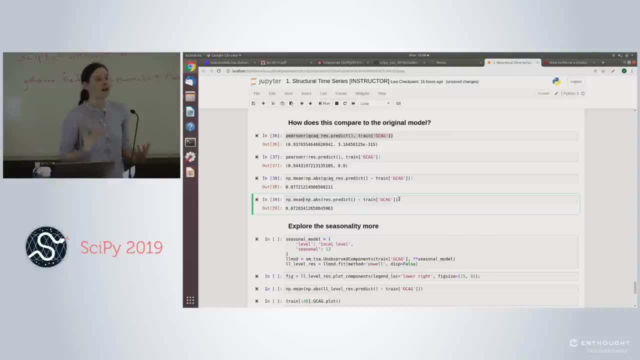 but if you look at your intuition and helping you understand the underlying dynamics, you might find that a model that looks much worse visually, that isn't offering intuition, doesn't do that much worse right, But then it's not offering any value. So a big part of thinking about when to use these models. 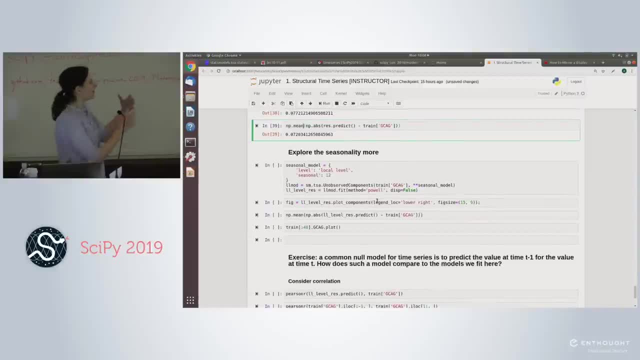 and how to use them is: what are they teaching you about the data? And it's really interesting to me that in this case we see an illustration of how just exploring models pointed out something that we sort of initially missed about this data because we did insufficient exploration. 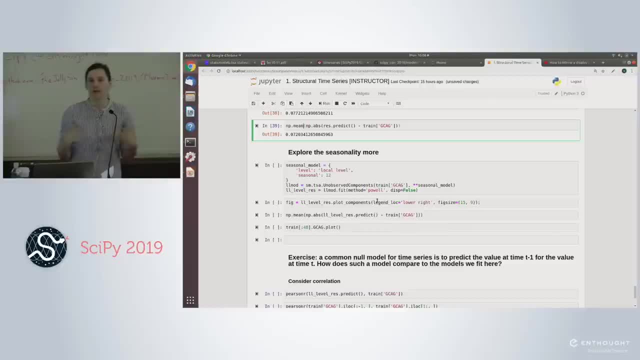 You might notice that your model isn't fitting your data very well, but you won't get such easy insights into why versus here we say: oh look, boom, I added a seasonal term and I can actually see the seasonality rather than just seeing a coefficient. 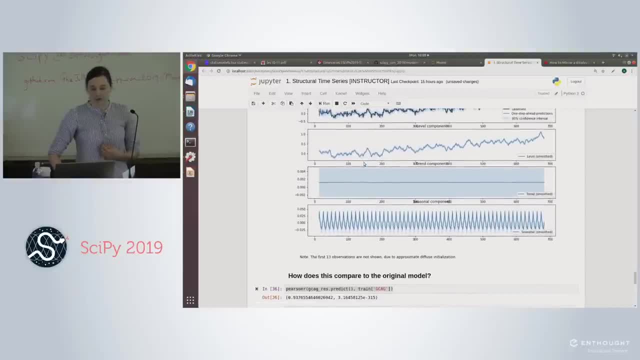 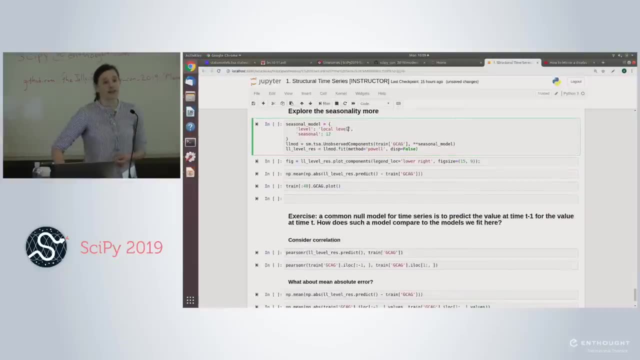 Okay, so now let's explore the seasonality more. What's something else we see here? We see that our trend component wasn't especially useful, so why don't we get rid of it altogether? How do we do that? We switch to a local level model. 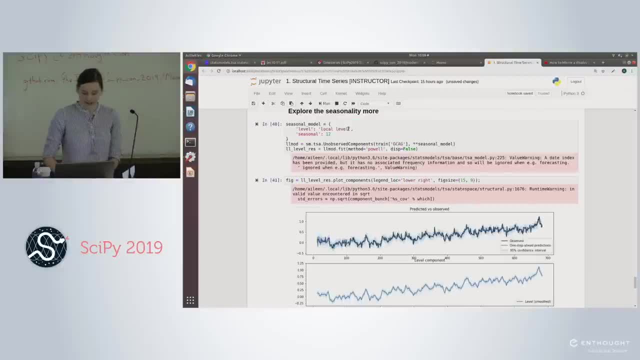 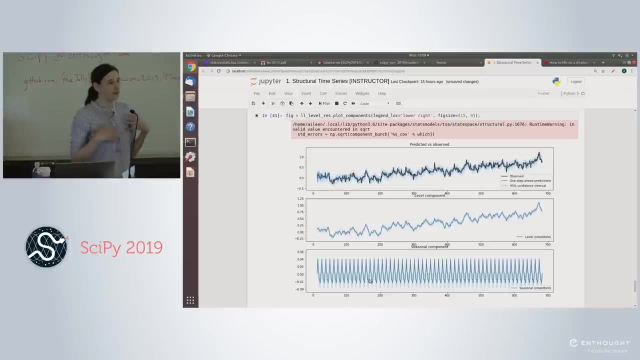 instead of a local trend model and we keep our seasonality. We really now we get something that looks really beautiful in terms of not having extraneous portions of our model like a whole trend component that we don't really need. We also see the seasonal component. 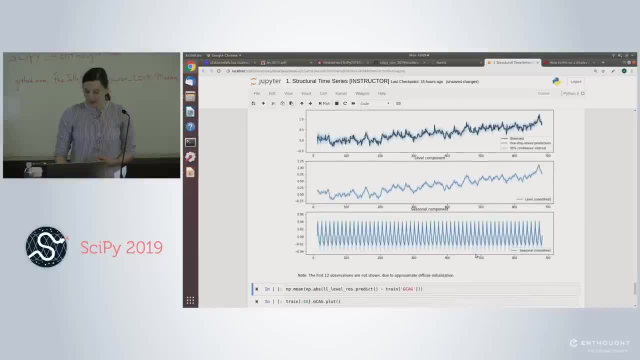 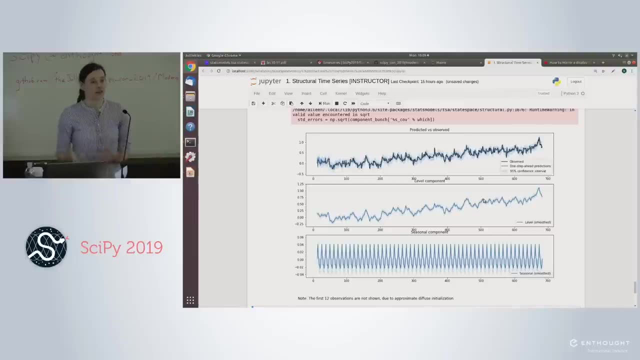 again, very strong signal. Interestingly, it is not time varying, right, It's just sort of uniform And we see sort of a level drifting, but tending to drift in the positive direction, right. So to the extent that we want to have, 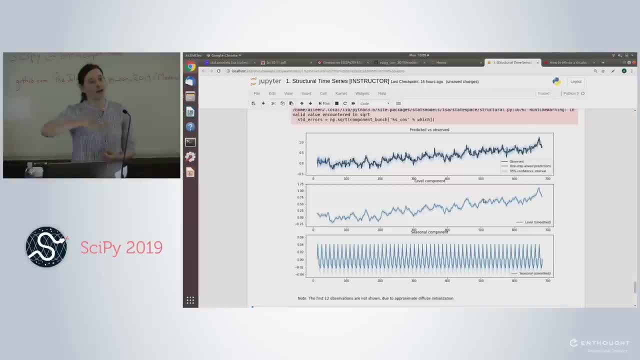 debates about climate change. this is one insight of like: oh, if we fit this kind of model, I see gradually that the level is going up and I see a seasonality, And that can be sort of first order way to talk about this data when you're first getting into it. 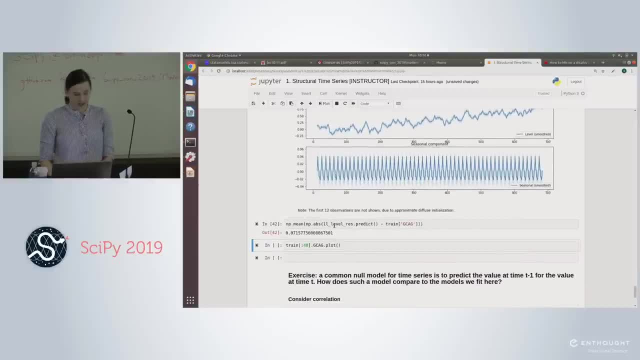 Question in the back? No, okay, Okay. And then we can again sort of look at the mean absolute error and we see that we are continuing to improve. These are sort of small incremental improvements, not massive improvements, but mainly we are having a more parsimonious model. 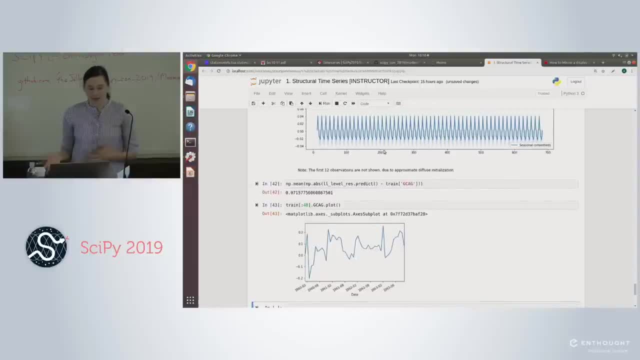 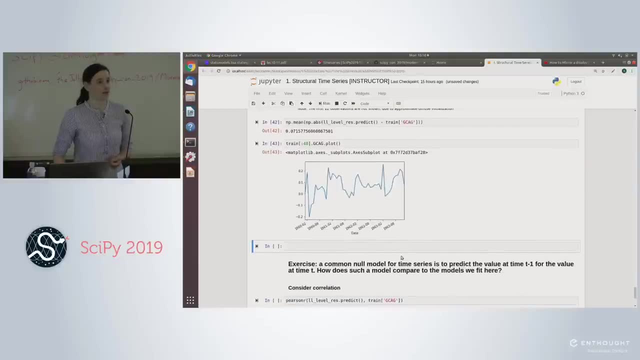 that gives us better intuition into our data. Once we see this, we realize we really should have revisited our data and thought about the shape of it, right? So if we sort of plot here, we can see more seasonality by looking more closely. 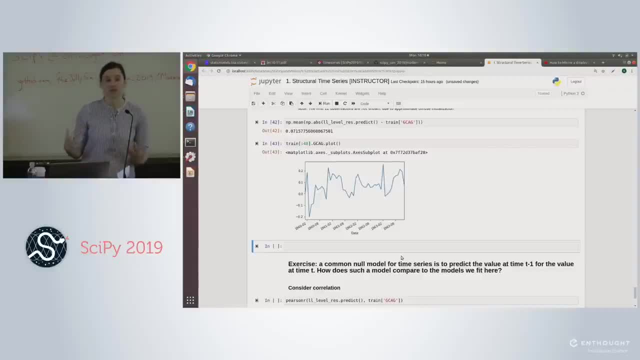 Although we see that this is not as clean a seasonality picture as we saw, say, with the air passengers data right, So it's a noisier seasonality and yet our structural model did a pretty good job of capturing it nonetheless. Okay, so final exercise. 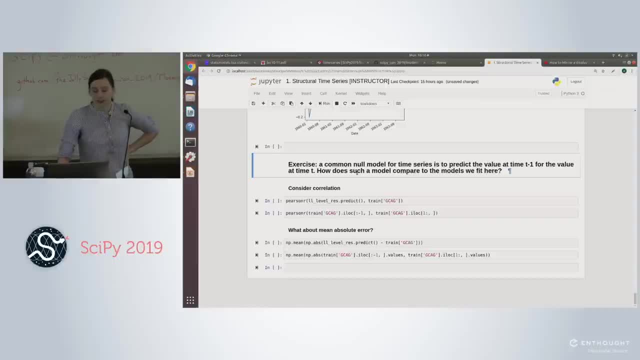 and then we're going to take a break. A common null model for time series is to predict the value at time t-1 at time t. So how does such a model compare to the models we fit here? Just take two minutes to compare those right. 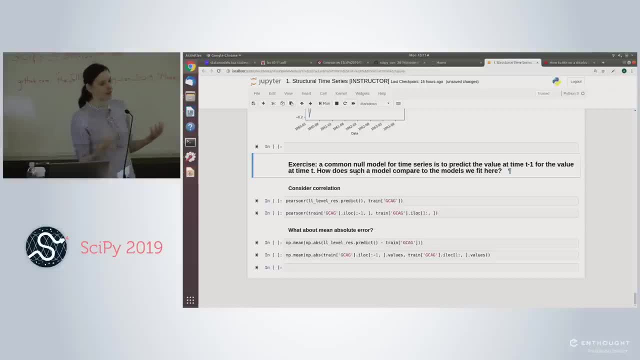 Have we actually done anything with sort of our fancy structural time series model, or are we just kidding ourselves, Something you always have to be asking yourself with the fancy methods? Yeah, exactly. So basically it will just have a coefficient, for it will have twelve. 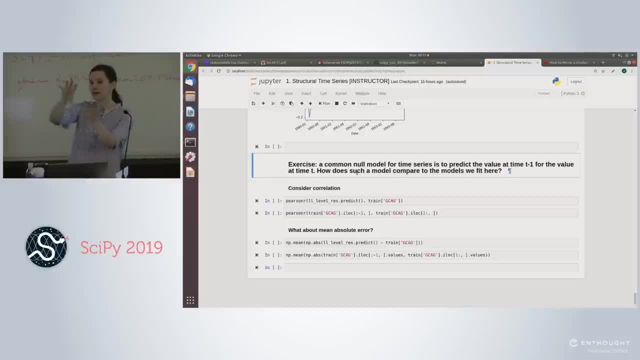 eleven different coefficients, right, You don't need twelve. right, You need n minus one for n seasons, and then you'll have a coefficient per and you'll say: oh, at this point we add or subtract this much, and that's where you get that seasonal component. 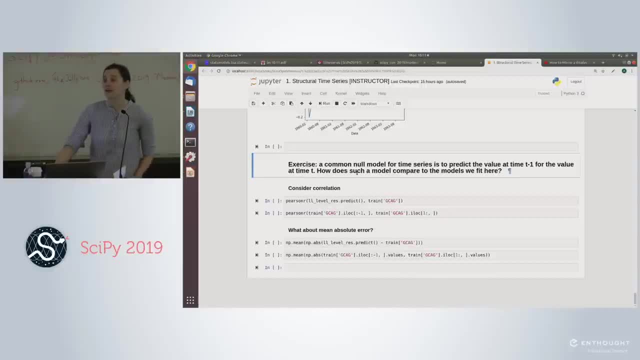 Yeah, So it can handle something like an incomplete cycle. Well, I should really be saying an incomplete seasonal cycle as compared to a cycle, because structural time series can also handle a cycle. What a cycle is is when you have some sort of repeated pattern. 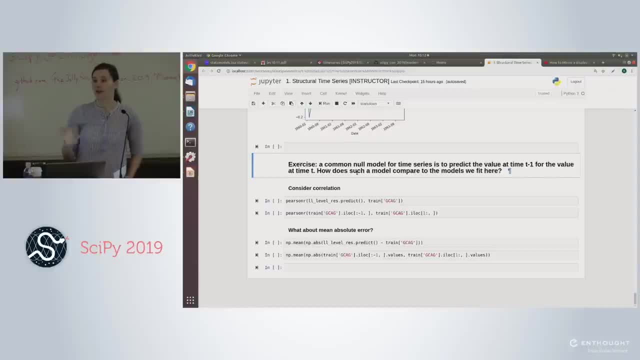 but it's not as regular as a season. So for a season the way that these models are fit is they're sort of a different component per season. So there will be eleven components to describe the twelve season model right, Because one of them will just be the null component. 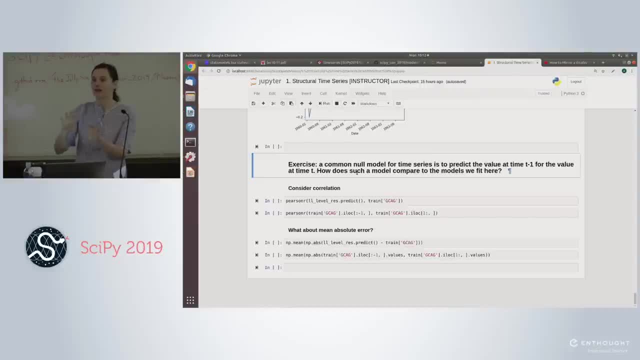 for every other kind of model that does this, And then, if you want to fit cyclical data, what that will usually fit to is sort of a sine curve, where what it's then trying to fit to is to determine the appropriate frequency to model the data. 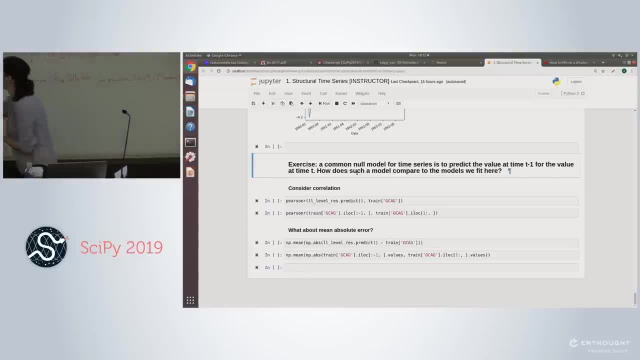 And you can also add things like a damping parameter, so you have sort of a sine curve right. This would be one way to start with a cycle, but then usually what you want to do is you want to both allow this to vary, so this will itself the frequency. 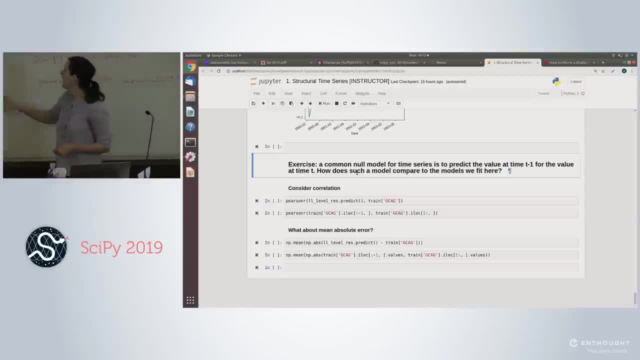 will be time dependent, so the frequency is fixed, and it will also have the option for those who are either physicists or remember, of some sort of like damping envelope as something else you can fit to. But that's not what we see in our data, right. 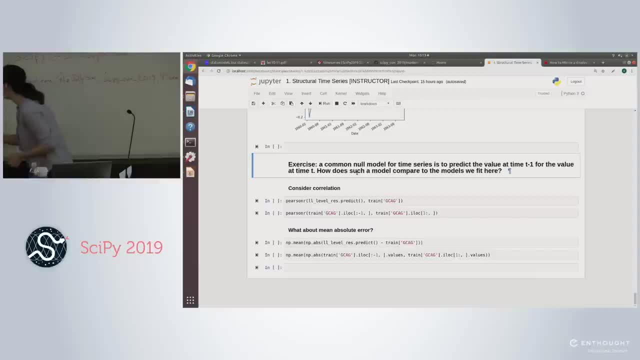 In this data, arguably, we see some kind of seasonal. so in that case, so for seasonal, you will really have like s sub one, s sub two, s sub three and so on, and it will just assume that s sub one is what you start with. It doesn't actually care. 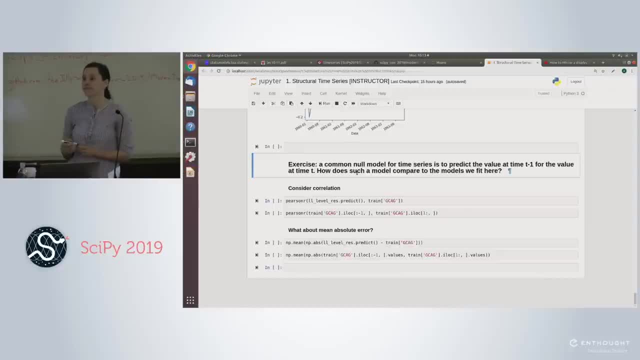 but for the first one it will just take that, and as long as it goes around in a circle, it's good. Okay, so how does our null model compare to what we did? Yes, Absolutely So. this is even a problem with ARIMA models. 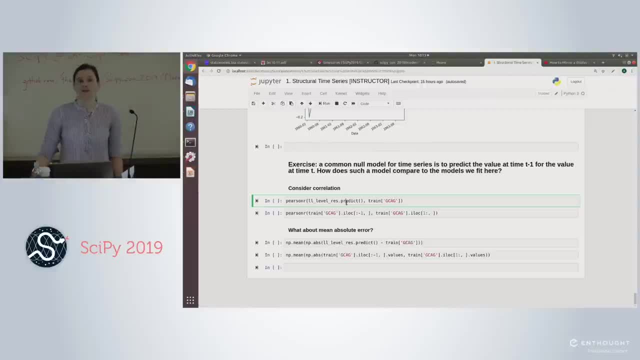 which seem sort of more traditional statistical. What's interesting, for example, just to back out for ARIMA, and then I'll come back to this case- you can actually have models that look different. they look like they have different parameters, but actually, if you do the polynomial math, 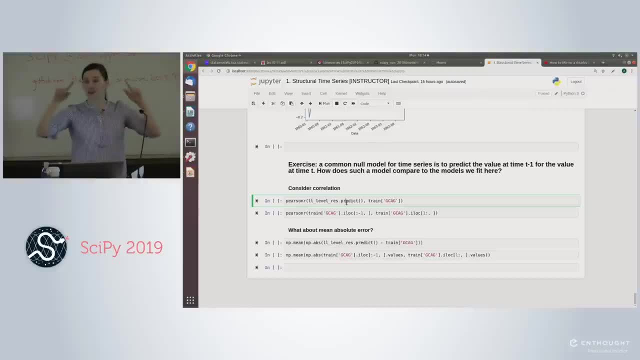 you can factor out and you realize you have sort of extra terms that literally just cancel out and you are literally fitting a model that math tells you is too complicated, like your model makes no sense mathematically. so even with a simpler method like that with structural time series, 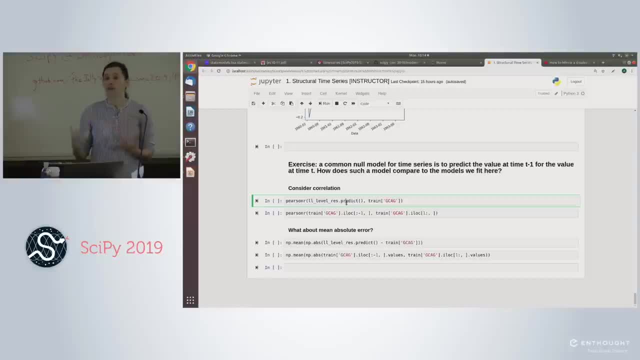 I consider them more useful, sort of as an exploratory tool. it's not something. I wouldn't fly an airplane or treat cancer based on the outcome of this. now, that's just me. many econometricians might feel a little bit differently. the more data you have, the better. 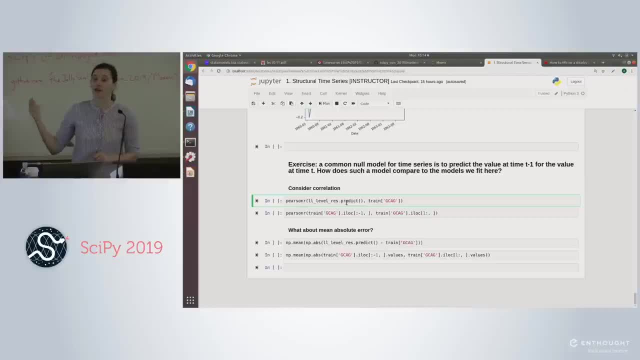 if you move this into a Bayesian model where you have a much stronger prior, that's also better- and actually Google has a great Bayesian structural time series package- because then you at least have stronger inputs into what you want. So if you inject higher from a Bayesian sense, 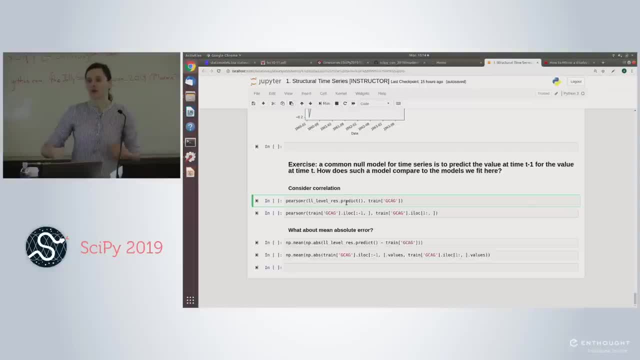 then I would trust these a little bit more versus if you are just using your default Gaussians and rolling with what it is Absolutely, and these can be very easy to over fit, like many sort of data intensive, computation intensive models, and there is no guarantee. also, 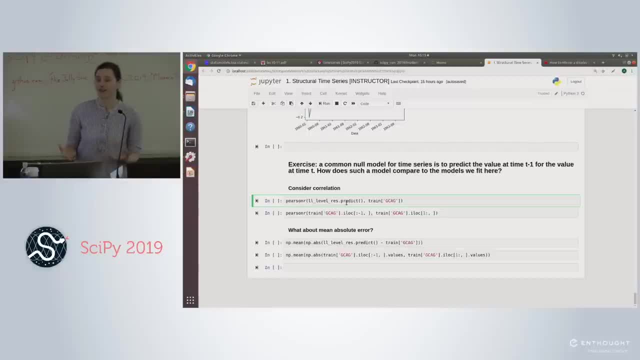 that you get to the optimum fit for your data, but arguably that's even a good thing, because getting to your optimum fit for your data could be over fitting as well. Yes, When we did the first model, we used like a smooth brand. so how do we? 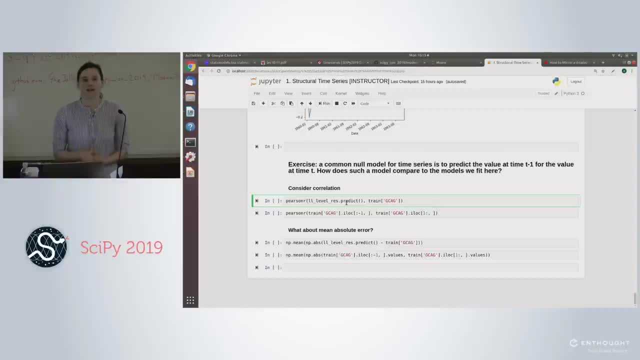 pick what to use in terms of the model. So this depends on the discipline. certain disciplines will have very strong priors, not in the Bayesian sense of the shape of the distribution, but in the definition of the model. so, for example, if you are modeling the stock market, you have to make 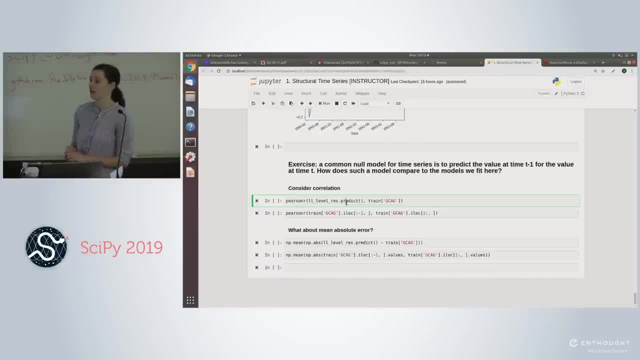 a very strong case for using anything stronger than, say, a random walk, and you would have to have a justification. another example I know of is people modeling hydrology feel very strongly that that should just be a local level model without a trend, so that tends to come from other domain knowledge. 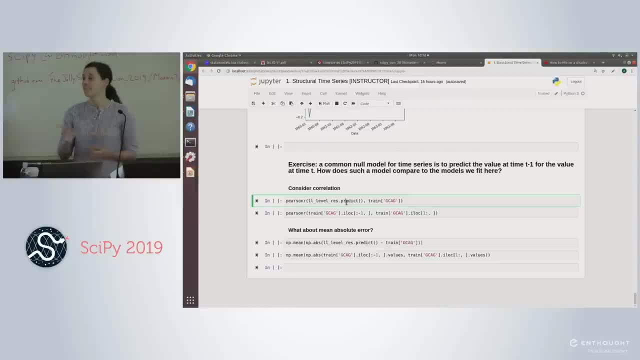 or theories about causation of the data you are seeing. Yeah, so in this case we are just exploring because we are not climate change experts. so, for example, I would be very skeptical if someone went to congress with this and said, look, I figured it out, for example. 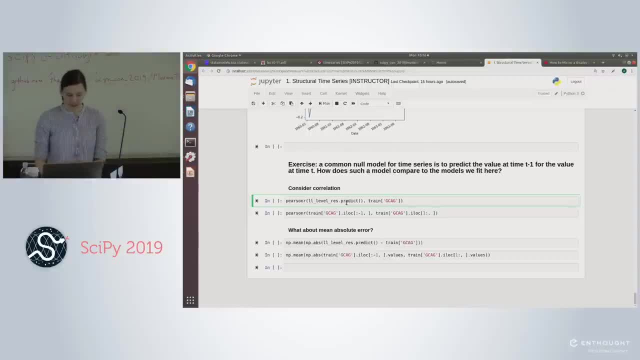 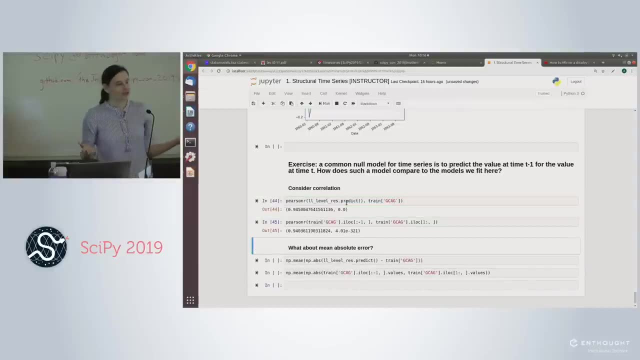 Ok, Ok, so very quickly, and then we will take a quick break. so if we are looking at our null model compared to this model, if we consider the correlation, they are not measurably different. so we have done all this work, fancy model, but it is not clear. 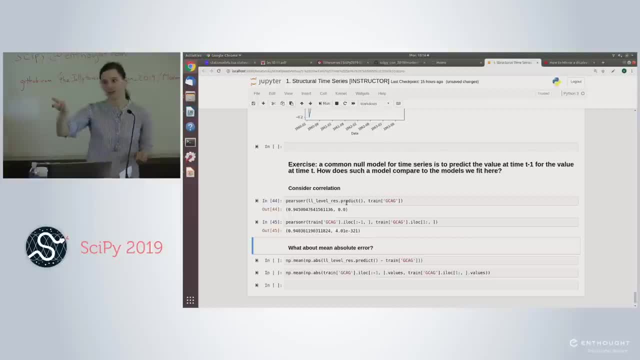 we have done much better. maybe we have done a tiny bit better and maybe that matters. but, as we were just discussing, since it is possible to over fit our models where there are so many knobs to turn, we have to look at skepticism, so whether this is a good model. 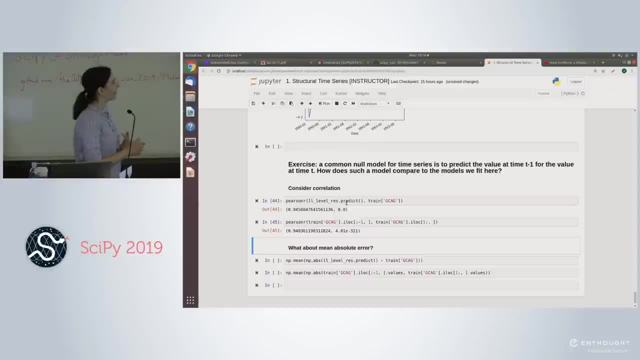 will depend on your purposes. what accuracy do you need? is half a percentage point improvement in correlation meaningful in your field or no? it is very context dependent. but otherwise, if you are someone's boss and they come to you with this, obviously the first thing you should do. 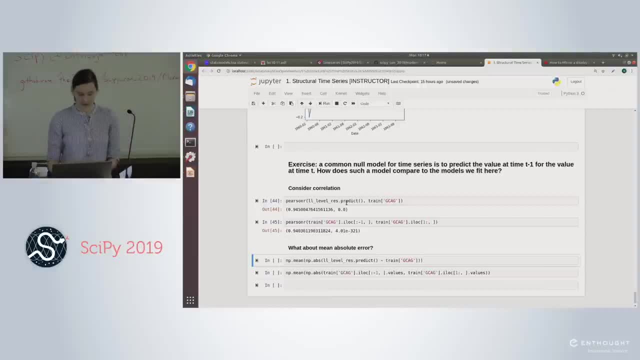 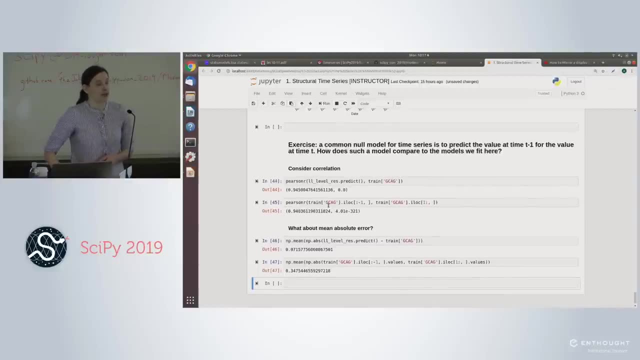 is shoot them down and say: do you really need this? because you have barely improved on your null model. so explain to me why you haven't. and what about in terms of mean, absolute error? well, here we have quite a difference, so maybe this is something worth thinking about. 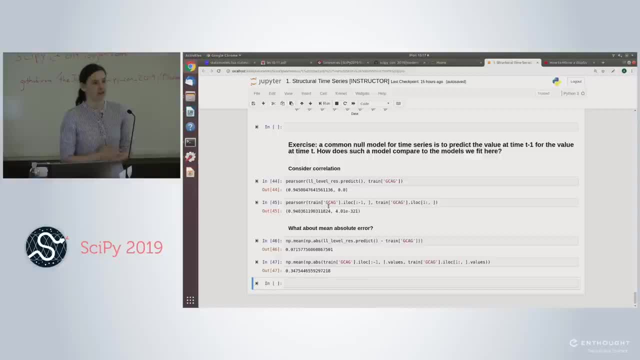 and maybe we should say, ok, well, why is that? what insights does that offer us? so, again, just a reminder to use different metrics and think about your context. ok, so those are structural models. we are going to take a short break and then we are going to come back and do hidden Markov models. 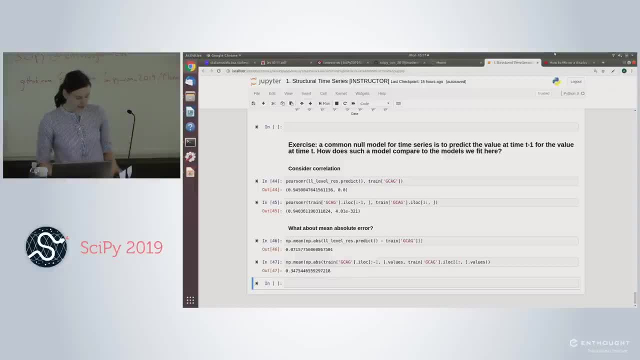 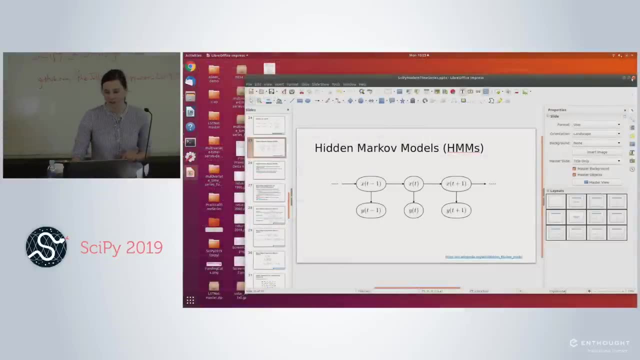 and that will be a wrap on state space. so let's just call it a 5 minute break and come back at 9.22. ok, so our break is over. I just dumped my email address in the slack, also in case that is not available on SciPy. 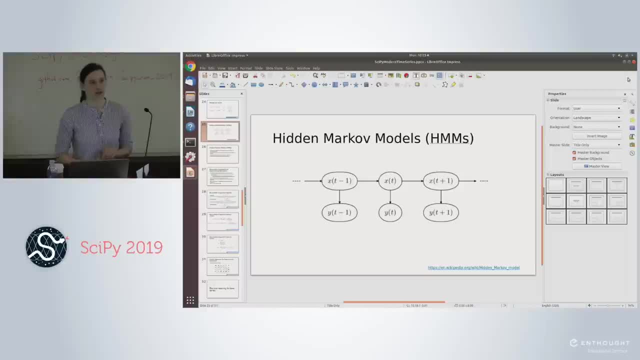 so if anyone has questions after the tutorial or follow up comments, great to hear from you. yes, so the slides are in the slack as a zip file and then, for anyone who wasn't here at the beginning, I am unfortunately locked out of Github at the moment for very 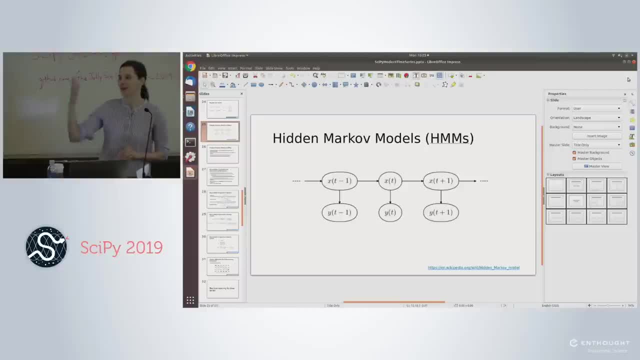 it's a very long story. so as soon as I am back in Github they will also be on Github, and someone has nicely posted them on Github now. but ultimately I would like to have the slides and the Github repository all together and also, if you email me once, I get that together. 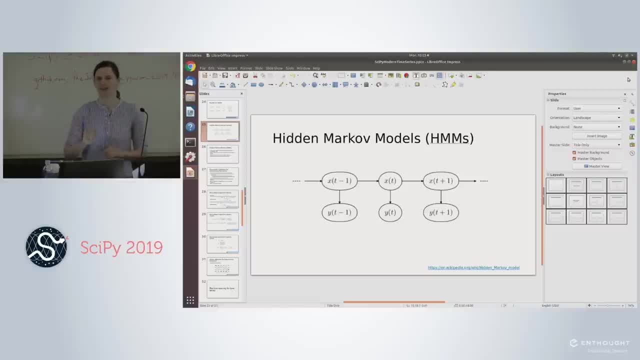 hopefully in a few days you can also have that. did that answer your question? yes, ok, any other questions? ok, ok, and then, just so folks know, we will definitely do another break before they stop serving breakfast at 10.30. in case anyone needs to pick me up, 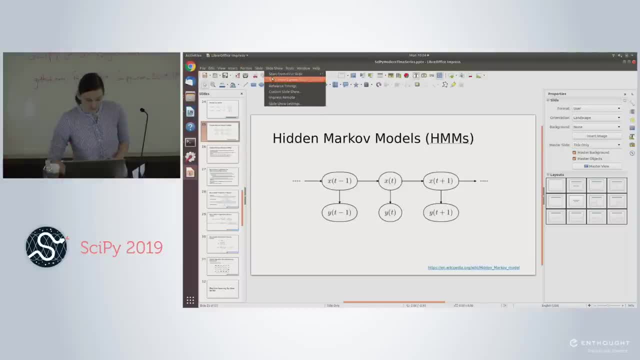 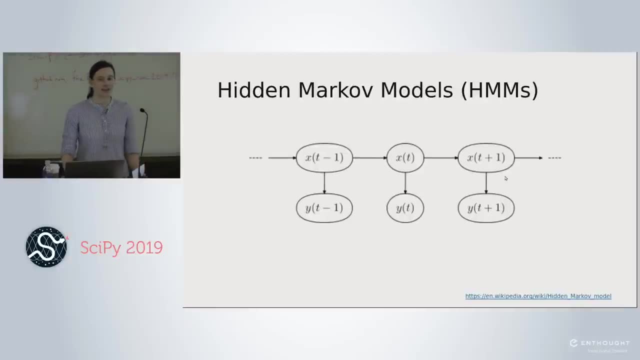 so ok, so we are going to be talking about hidden Markov models now. this is another technique. it's not especially novel or considered cutting edge, but it's increasingly useful because now you can actually get decent computing power, as opposed to when it was invented. you know, and maybe if you were at IBM, 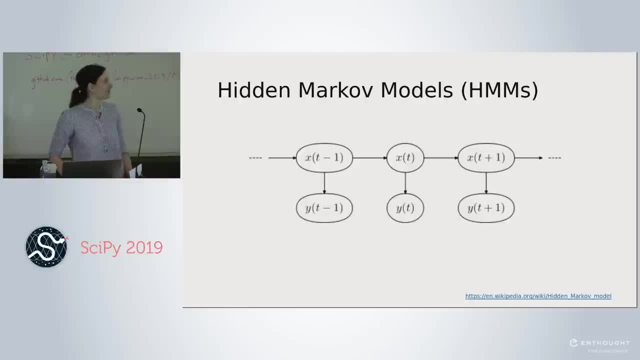 and had a really fancy computer or whatever, you might be able to fit it. now we can all just fit it on our laptops. so much more relevant than it used to be. why is this a state space, state space model? well, it's the same idea in the sense of having the idea. 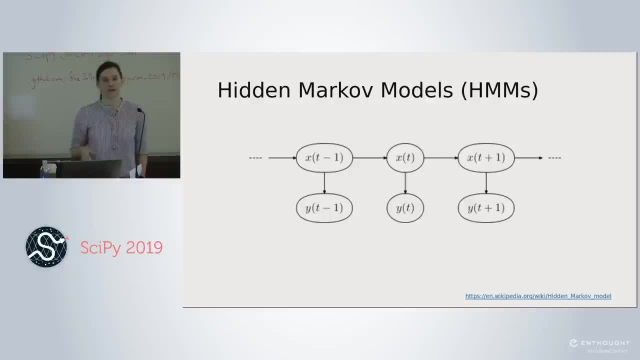 that there is an underlying state that you cannot observe and there is the output of that state which you can observe. in the structural time series models, we tend to have the model that the state and the measured quantity are basically the same thing, with error, but we can also broaden our perspective. 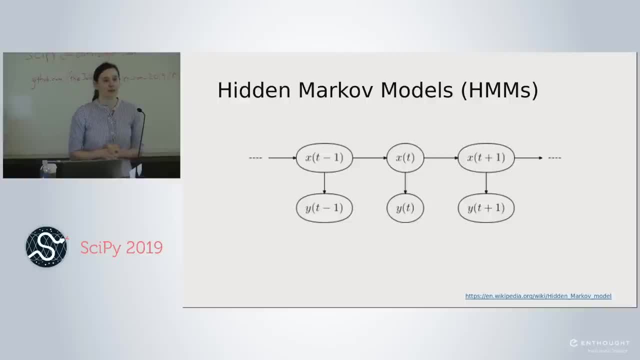 with hidden Markov models and think, well, maybe what we observe could be in the same physical or conceptual category as the underlying state that's producing it. so in this case, what we have? we have a sequence of measurements, as depicted here, where we envision. I feel strongly that people should be able. 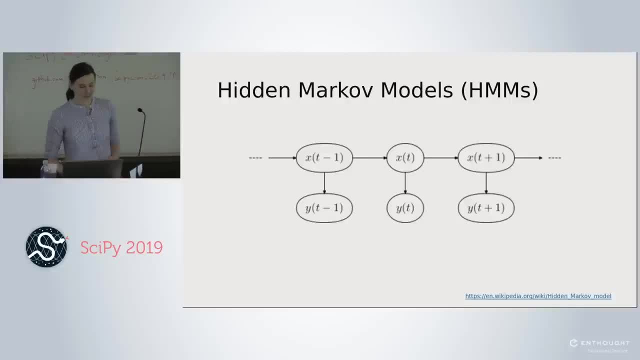 to come and go whenever they want, so no one is imprisoned here or freaked out on the way back. so, in this sense, what we envision is we have a sequence of states and, for whatever reason, the dynamics of that system, the states, are evolving over time. we conceptualize this in a discrete. 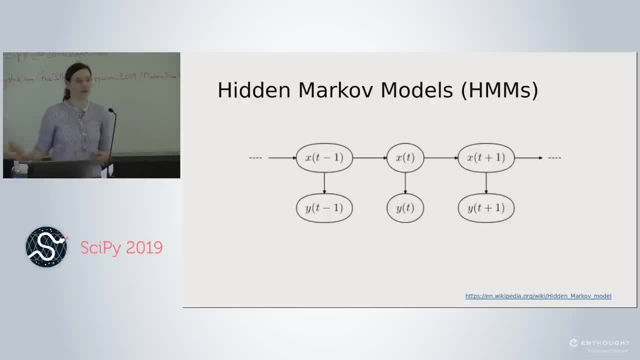 time framework, but this can also be in continuous time and you can do hidden Markov models in continuous time. we won't look at those, but if those describe your data, you can think about that. so we have a sequence of discrete times. we can't see that directly. 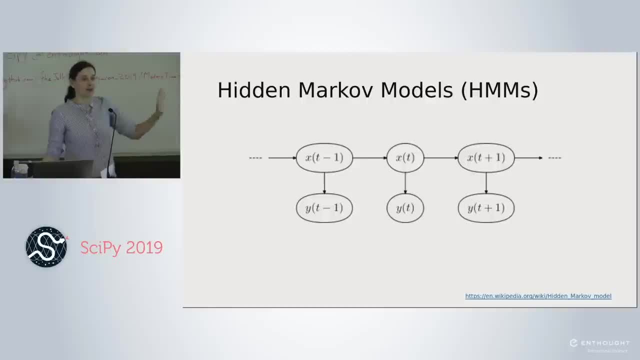 what we can observe is, whatever the observable is, y also at those times, and somehow x, the underlying state, is what produces a certain kind of y. so how do we make this more physical? well, one example where this is widely used and actually where you don't even need to have 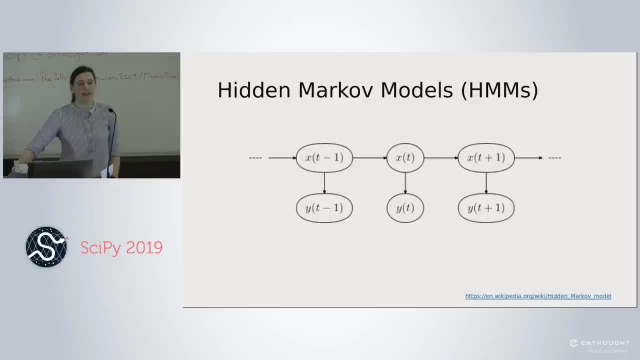 the fiction of discrete time steps is in DNA analysis. so when people look at DNA sequences and they're trying to think about why do I see maybe certain peptides in a certain sequence and what does that tell me about the underlying state of the DNA? I'm not a biologist. 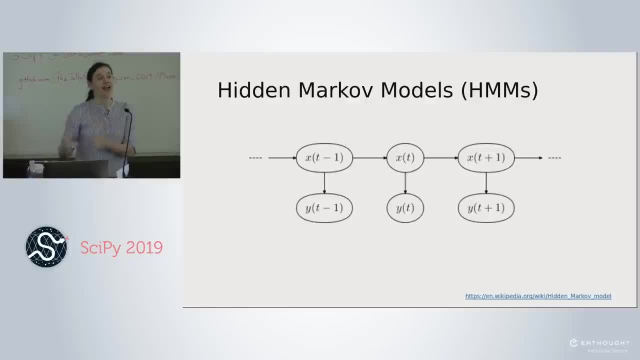 so I'm probably slaughtering this, but the point is is you have these DNA chunks that really are coming in discrete measures, and there's an example where it is a time series in the sense of having an axis that is well ordered and has a good definition. 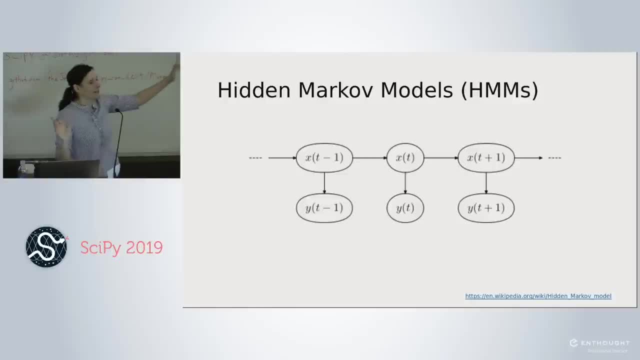 of sort of moving forward or backward along an axis. so that's an example where maybe your underlying state is a chunk of DNA and what you observe maybe is something like over time, like what kind of enzymes are being produced at this time, what kind of distribution. so notice that x itself. 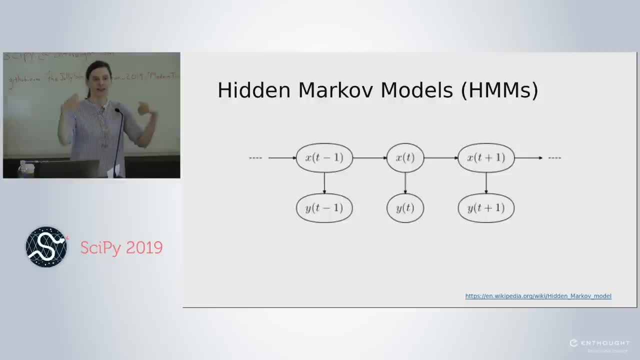 the underlying state. that's usually going to be something that's discretely defined. I have a countable number of states. these are discrete states. I'm not going to be in two at the same time, although, again, you can model anything. you can make things infinitely complicated. 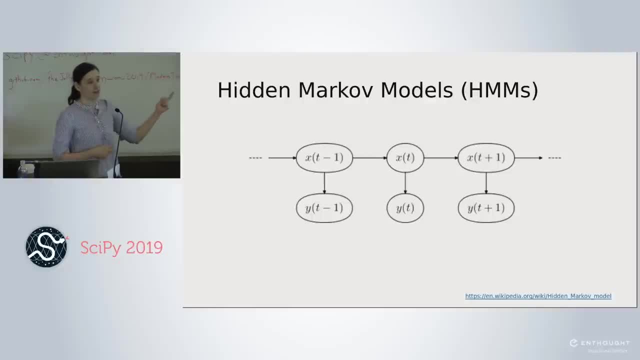 or they can be continuous. so in the discrete case it could be like: what kind of sequence am I observing? where that sequence is? some other kind of indicator, but not the state, or it can be some kind of continuous variable. so an example of that and the one we're going to model in our notebook: 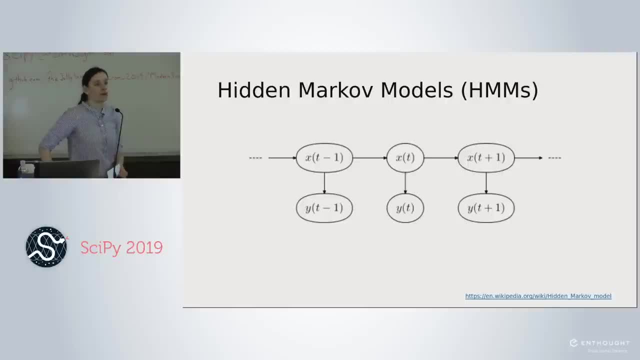 is, we can think of rivers as being sort of in high flow or low flow states, to first order, and then we can think about: well, if you're in a high flow or a low flow state, what kind of flow are you going to see? that's the y. 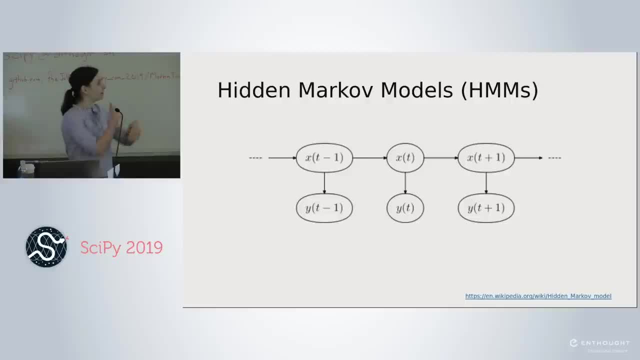 and the y is basically the same number for low state versus high state and there's a good chance that the distributions will overlap. but if I sort of look at the whole sequence I might get a sense of: oh, these were low and these were high and these were low. 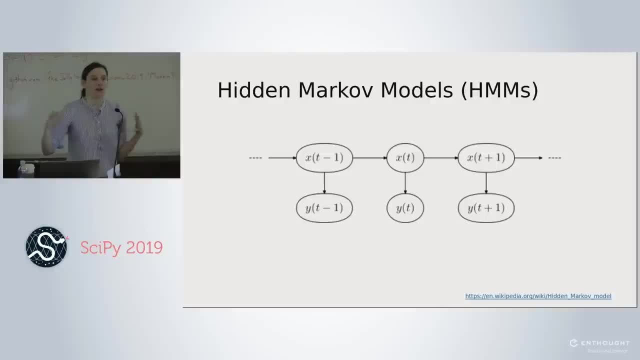 so why might I use this, say as opposed to an Arima model? and I don't mean to say that an Arima model is the be all, end all, but we should think well, why would I choose this model over, say, another one that's known to perform well? 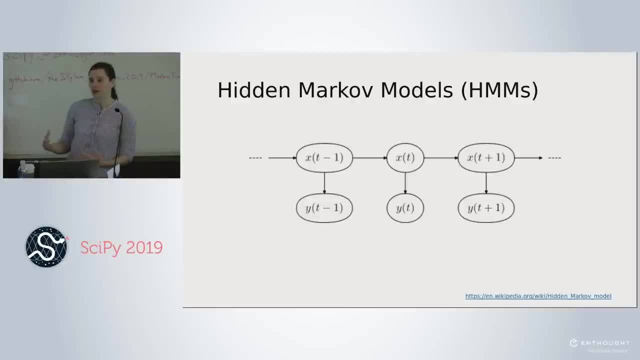 well, there's a couple of reasons. model of the underlying dynamic. so to the extent we have a model like that for a particular system like this, if it fits, then that's a good thing because it can offer us some kind of insight. Another thing, for example, in the case of river flow- and this I learned just from reading a 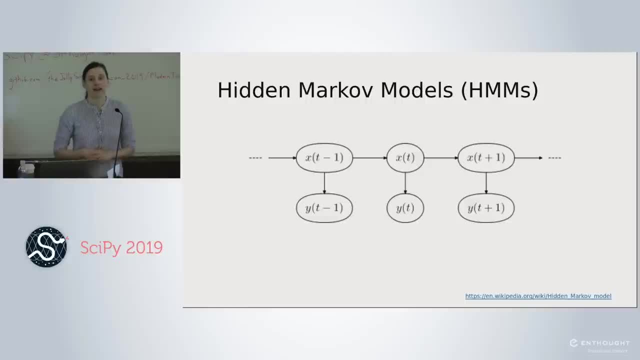 hydrologist blog who was blogging about HMMs, is that they find that AREMA models don't capture these sort of nonlinear dynamics of it's. not that you know time t minus one predicts time t, it's more of this sort of regime switching where you know kind of the probability of the regime. 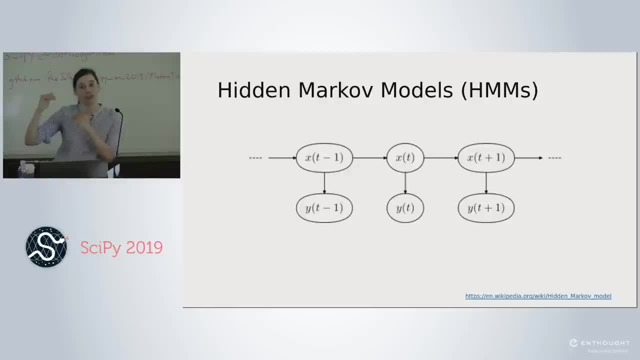 switching. but when you last switched regimes doesn't necessarily tell you when you will next switch regimes, And that's a feature of Markov processes in general. right, The whole point of a Markov process is that when I'm at t minus one, if I know my state at t minus one, I don't even 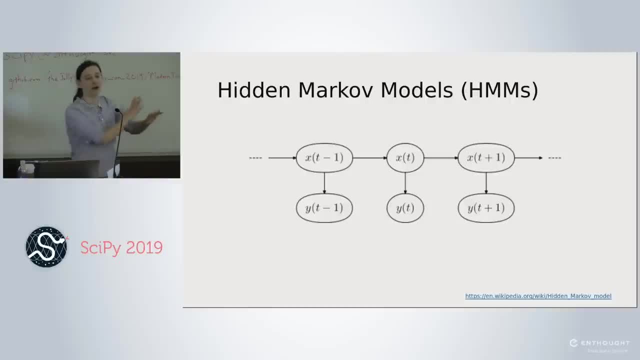 really care what came before. So that's quite different from an AREMA model where I say, oh, I'm looking at my whole history to determine where I'm going next With a hidden Markov model. I'll say, as long as I know, x t minus one. 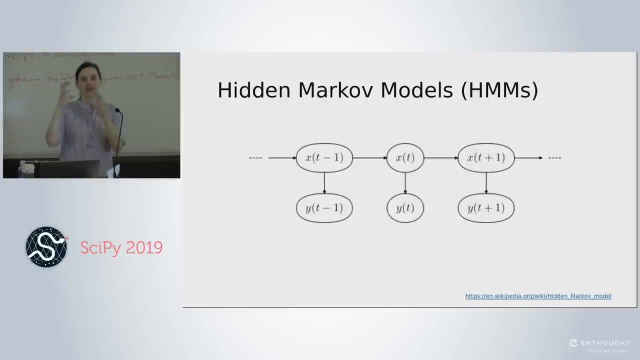 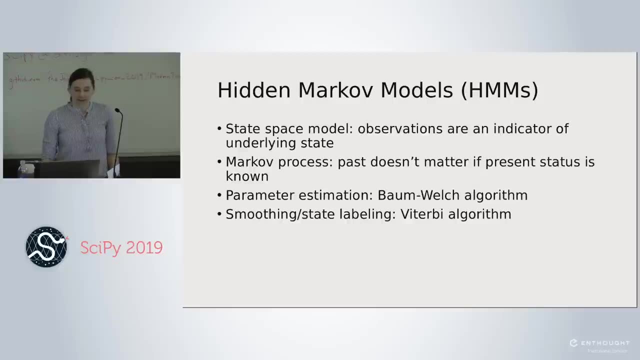 I don't need to look backwards in time. Sort of all the information I need is in that data point. So those are just a few observations about hidden Markov models and when you might want to use them. Okay, so they're a state space model. Observations are an indicator of the underlying state, but we 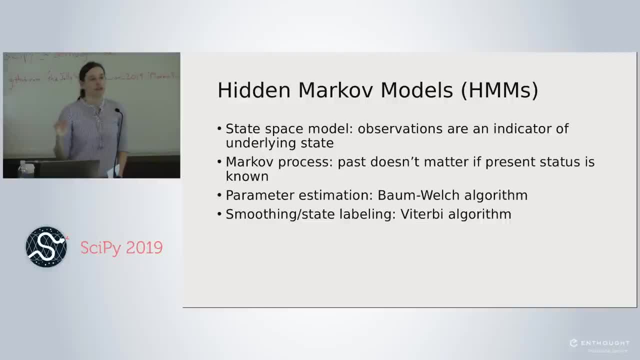 posit some separate underlying state, And in this case you really wouldn't posit that. your underlying state is just your observable with error. That's not sort of what you're doing with a hidden Markov model, unlike the structural time series In a Markov process. 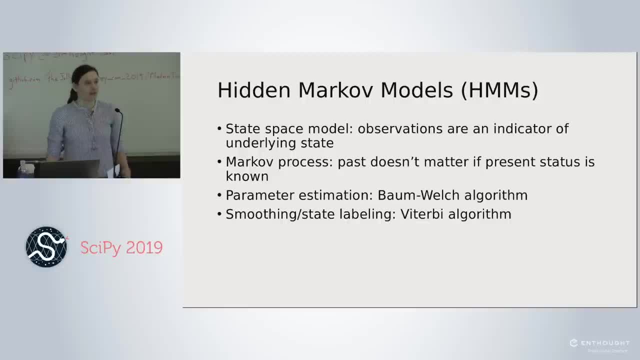 the past doesn't matter if the present status is known, right. So the most informative thing is just your most recent measurement and nothing else gives you new information. So these things, the two aspects computationally I want to talk a bit about before we fit- are: 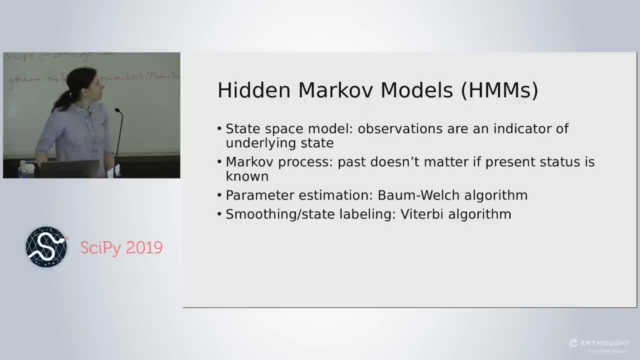 parameter estimation with the Baum-Welch algorithm and smoothing slash state labeling with the Viterbi algorithm. So I'm guessing you've seen these words floating around. I just want to give you an overview or an intuition for what they are before we use them. Okay, so the Baum-Welch 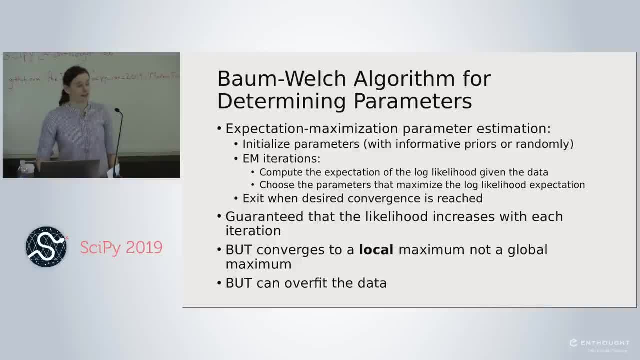 algorithm. it's how we determine parameters. So when would we use this? This is at the very start. This is like I have a time series. I have a sense that there's some kind of regime switching, but more than that. 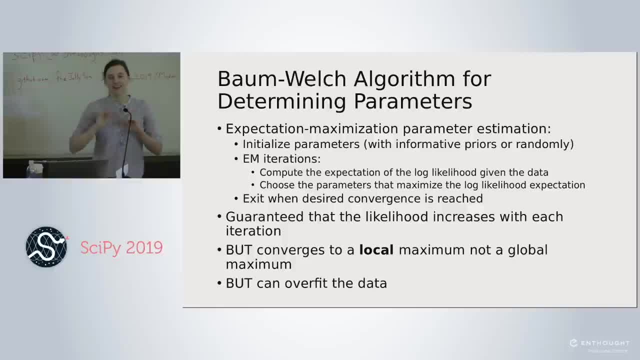 I really have no idea, Like I have no priors. There's nothing I know about, sort of whether you know the mean of one state is three or 17.. I have no idea. So this is really amazing in the sense of. 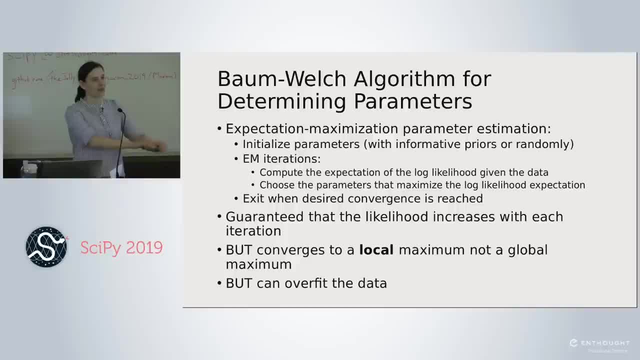 you can just say: here's my data and here's how many sort of underlying states I think I have, Go, And it will sort of figure out a set of parameters. Now, of course, what does that entail? It's the same concern we. 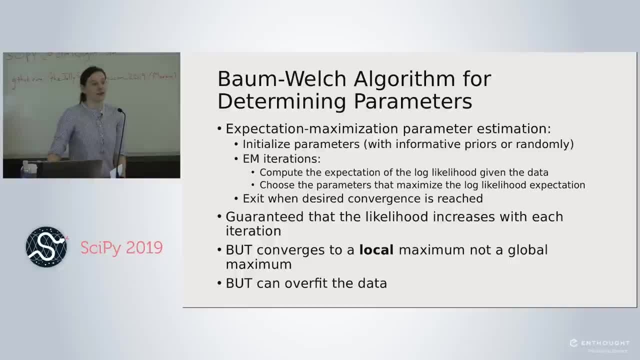 talked about earlier. You have a lot of knobs to turn. This is a very complicated situation. right when you start thinking about how you would code this up if you just had to code this yourself, It's sort of a nightmare. So basically what that means: it's not guaranteed to converge to a global maximum. You're not. 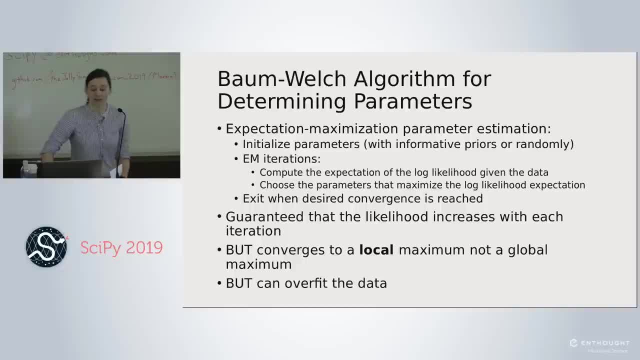 guaranteed to get the absolute best parameters to describe your data. What this algorithm does guarantee is that you will always get a little bit better with each set of parameters. So if you have a set of parameters, each cycle of this algorithm, So it's a forward-backward expectation. 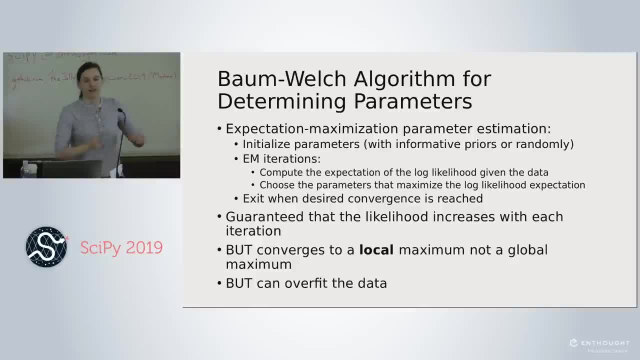 maximization algorithm right, which means you sort of first figure out what your likelihood expectation is given your data- that's your expectation step- and then your maximization step is you sort of update your estimate of your parameters to maximize the likelihood given that expression of the likelihood. 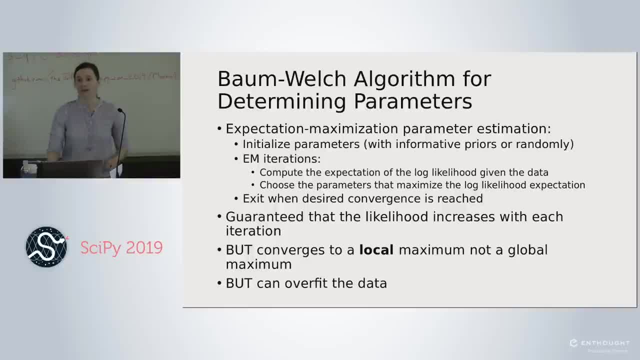 form. And then you do it again, right, and you just sort of do it and do it and do it until you get to what you think is an acceptable convergence level or an acceptable likelihood. but that will only get you to a local maximum. So 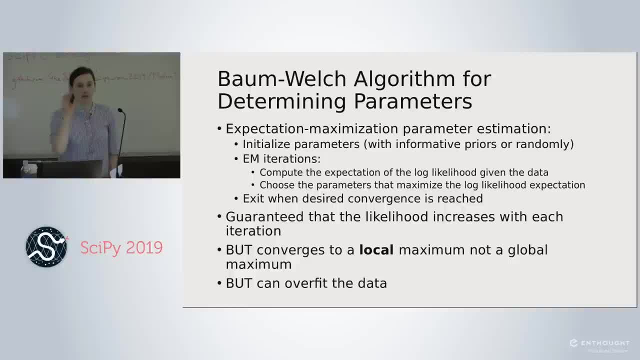 that's another thing to keep in mind with these models. right again, there's not some sort of unique, well-defined, closed-form solution, and often what people will recommend is that you run it many, many times before you sort of make any pronouncements on what this is showing you, right, so you don't just run. 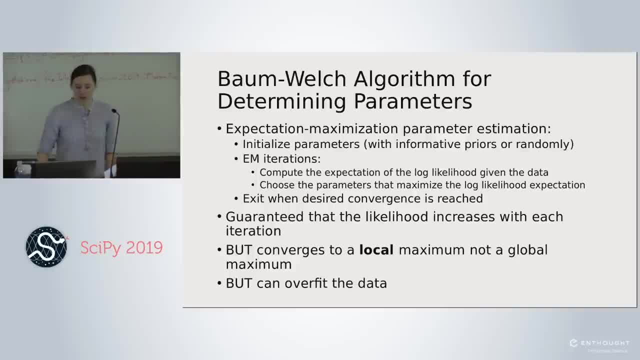 it once. maybe you run it a hundred times and look at what your your parameter estimations are and see if some sort of like narrative or some form is emerging from your many, many attempts. And of course, keep in mind you can over fit the data right. so it's quite easy to. 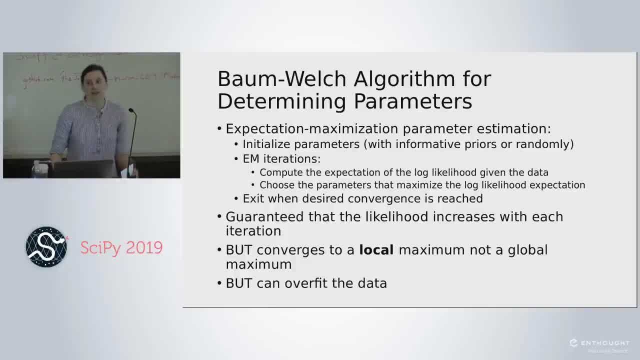 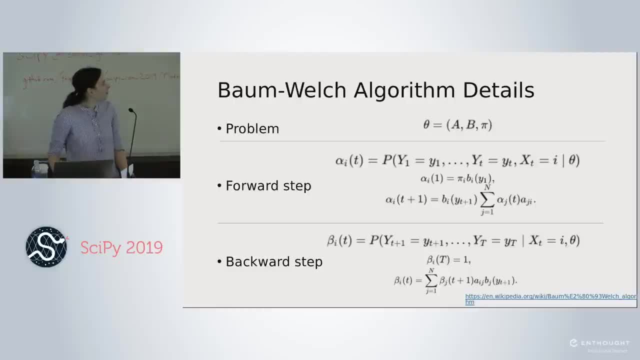 maybe choose a set of parameters that will do much better on your training data than on some sort of validation holdout. so that's always a risk with these sorts of things. Okay, so just a brief overview of the details, right? what's the problem? You're trying to estimate basically three things. You're 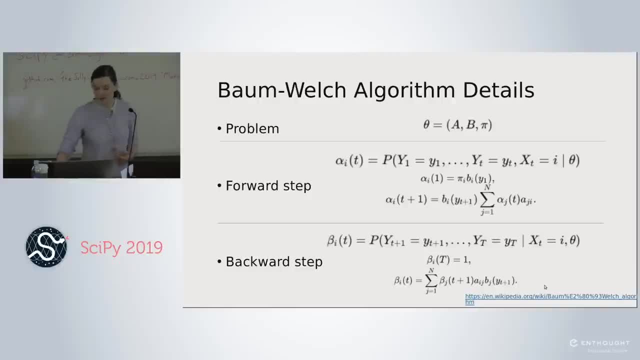 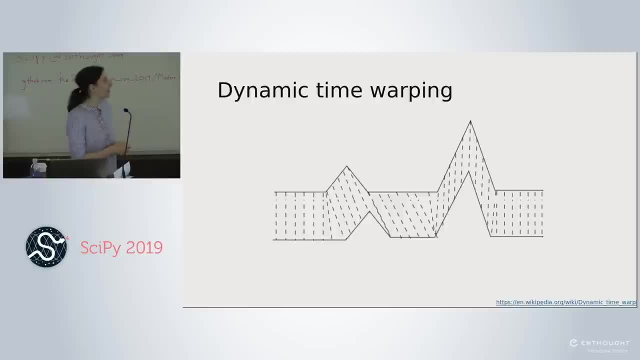 So what's that? If we go back, your A is sort of telling you how likely at X, you are to transition to A project, one onto the other, and you give yourself leeway to sort of come up with the best time. 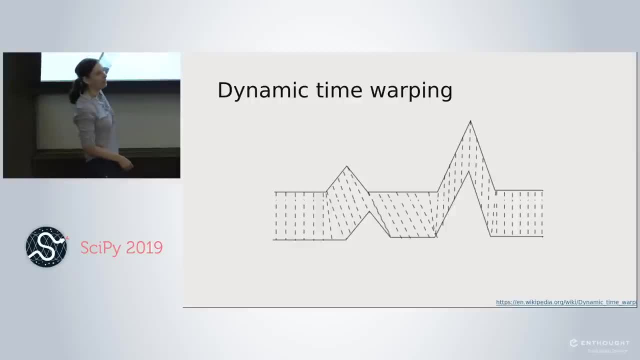 projection, which means you can sort of expand or contract time on one of your axes in order to enhance your fit, And the nice thing about this is that this tends to correspond pretty well with what we do visually without having to actually do the image analysis right. 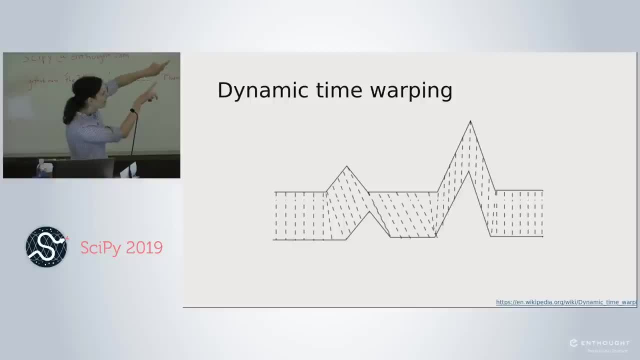 So this looks at it and just like we can sort of squint and we can see the two peaks at the beginning and in our brains we want to match them up, that does that computationally. So we're going to revisit that and see what that looks like. 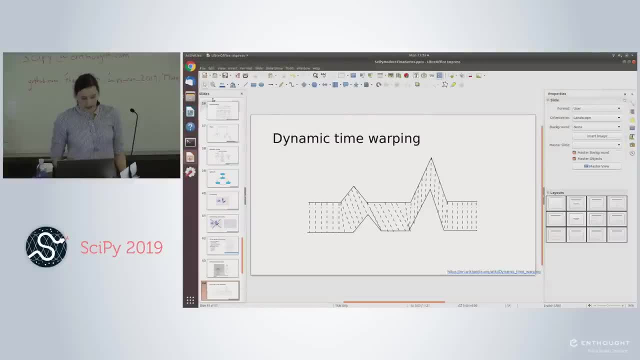 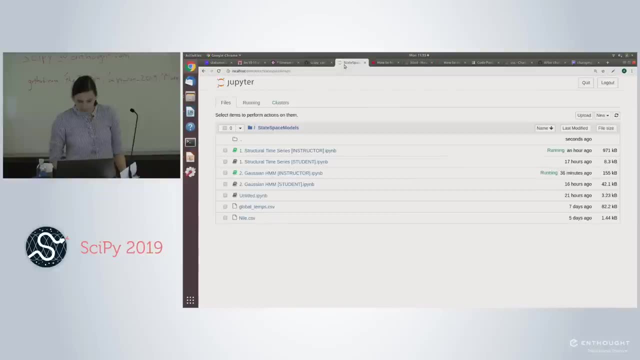 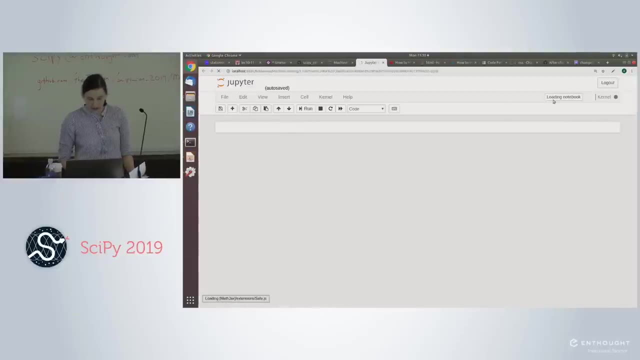 So that's an overview of what we're going to do in the notebook. so now let's go to notebook number three. So we're going to go out of the state space into the machine learning and we'll start with trees for clustering or classification and prediction. 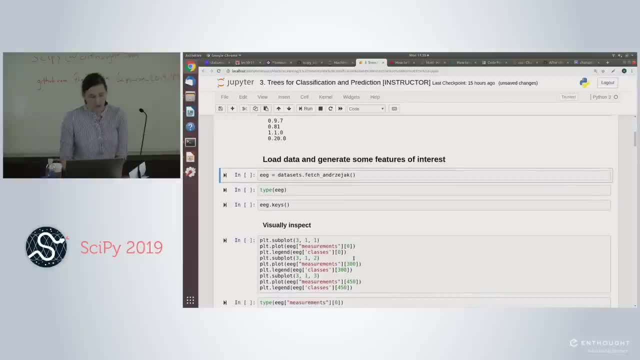 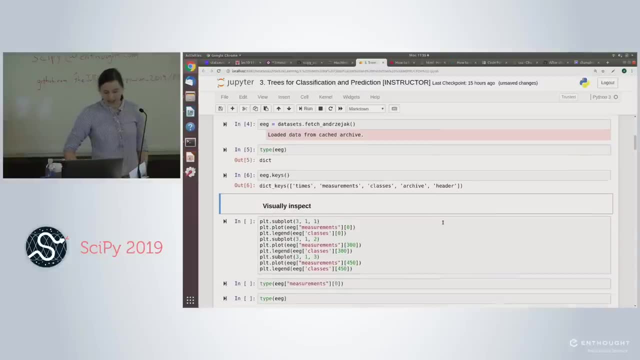 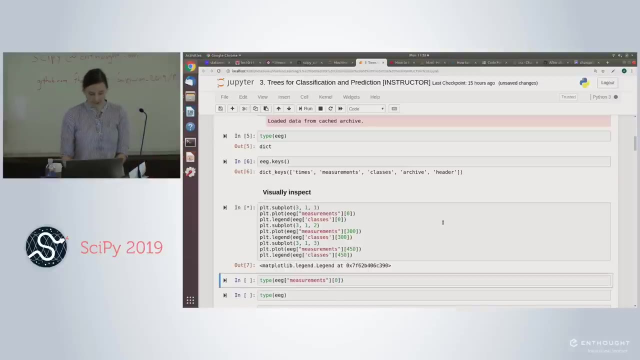 Okay, so the data set we're going to start with is a data set that's available via the cesium library and it is an EEG data set, so that's for the brain rather than the heart, and I'm sure somebody in this room knows a ton about it, so feel free to pipe up if you. 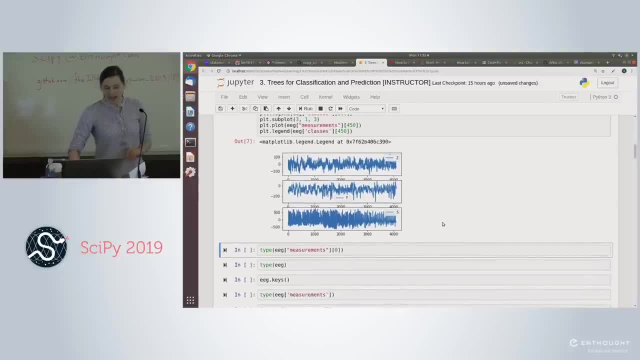 have any sort of input, always interesting. So we visualize this and we see that there we can even sort of qualitatively see a difference between three samples. We can see at the bottom here that there are three samples. At the bottom there's sort of one highly volatile sample. 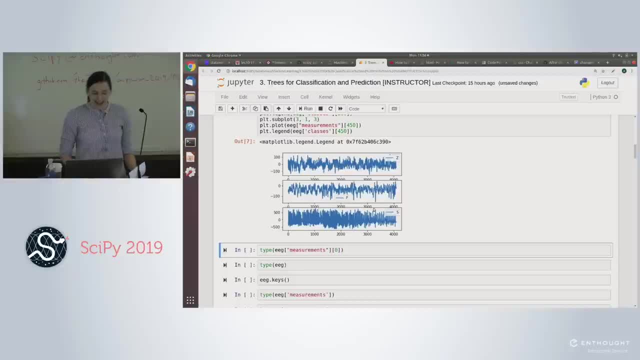 This is sort of all over the place, and then the top two are sort of less volatile. It's not just the volatility, though. If we look we also spot just differences in the values, right. So the top plot looks like it might be sort of Gaussian around zero, and it has sort of 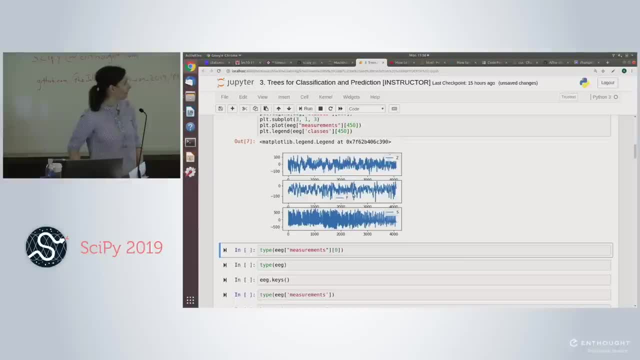 a range of like minus 100 to 100.. The second plot, if we were to just look at it visually, doesn't look that different from the top plot, but if we look at the values, this one only ranges from zero to minus 100,. 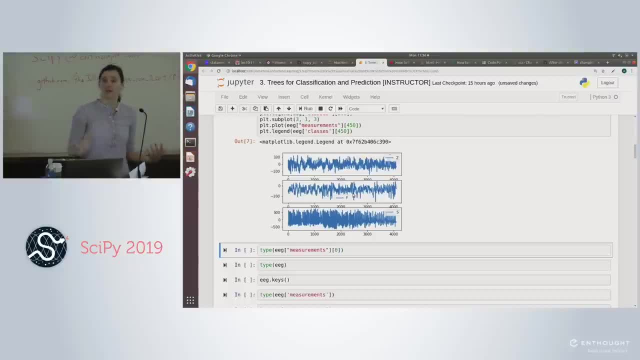 right. So the actual values in this case seem to be some kind of tip-off of the classes. And then again, if we look at the last one, this might be sort of Gaussian, hard to know from this, but we see the range is also quite different: 500 to minus 500, right. 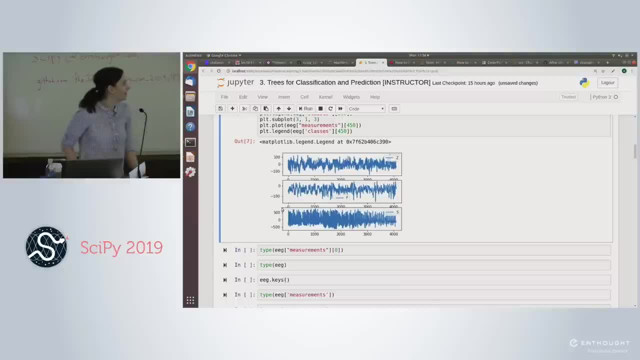 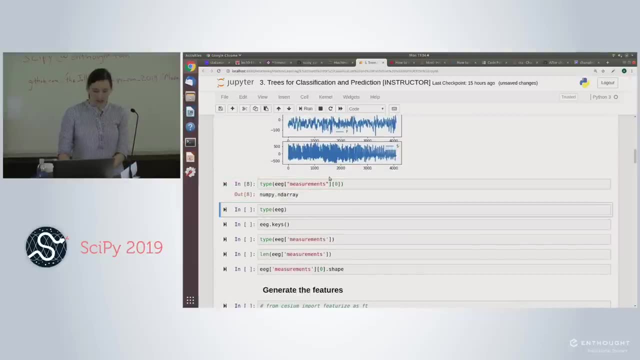 So already we can spot that we'd want to find ways to sort of preserve information about the values if we were thinking about generating features. As far as what kind of data we're looking at, we're looking at numpy arrays served within a dictionary, and they're giving us times, measurements and classes, so that's something. 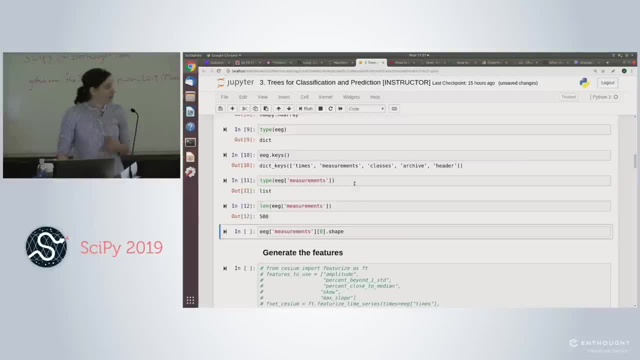 to be aware of. The measurements themselves are a list, and it looks like we've got 500 samples And then, if we look at just one of those samples, it's 4,097 points long. So you already get a sense of: oh my goodness. 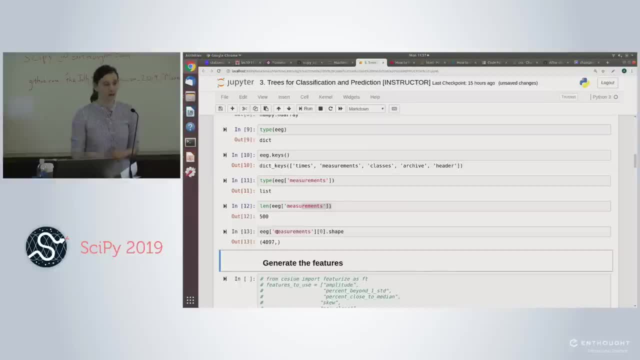 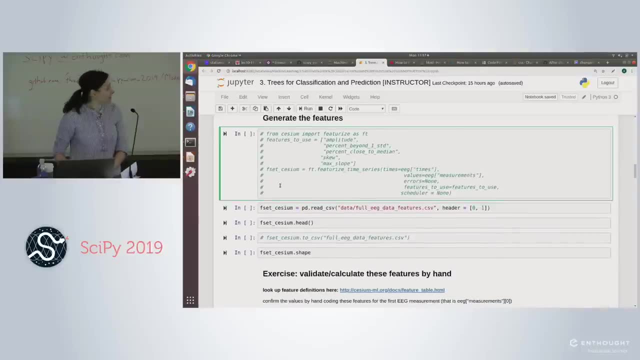 So if I have 500 time series and each of them has 4,097 points, you see already how it gets to be a little bit computationally taxing just to go through all of that. So next, if we generate features, feel free to do that. 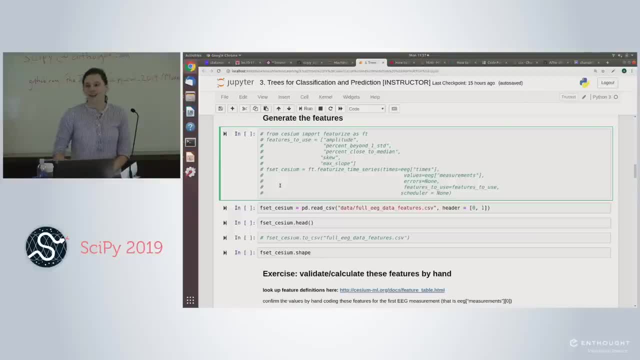 Feel free to go ahead and hit that button if you want, At least on my rinky-dink laptop. this takes a really long time, so I'm just going to load it up from prepared data. So that's the code I did write. 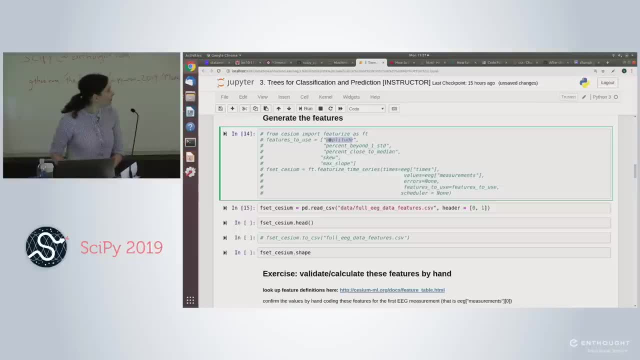 And what did I extract? I extracted the amplitude, the percent that's beyond one standard deviation right. So a measure of, like how many outliers we have and how spread out they are, The percent close to the median right, Some sort of measure of how tightly it's hewing to those central values. 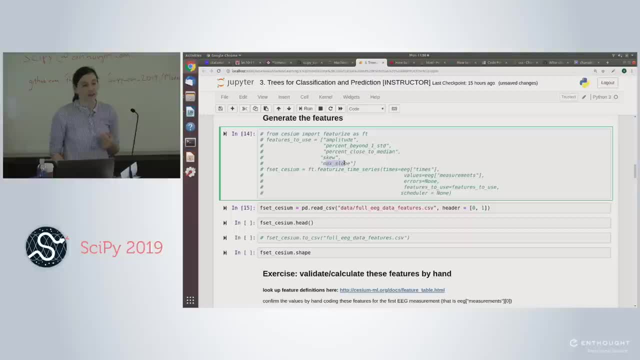 The skew in the distribution and also the max slope, which is sort of how much it jumped up or down absolute value from one data point to another. How did I find these features? Well, I just looked at my data a little bit, saw what will fit reasonably well, and then 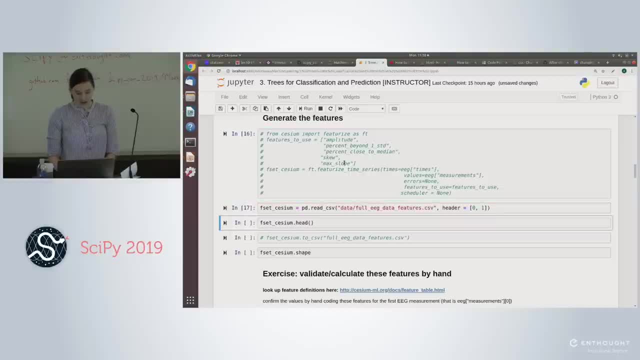 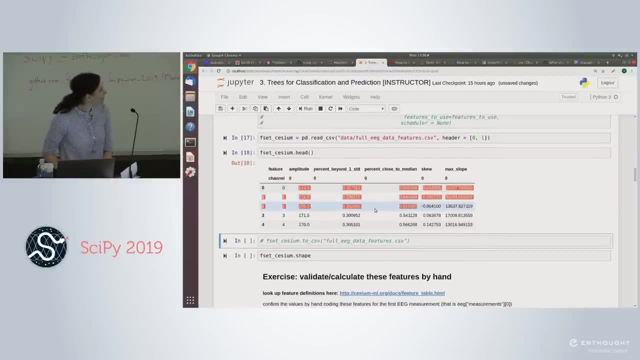 I looked at the cesium documentation and I generated those. So here you can see if you did just load it up from the CSV. this is what you see. And what do we see? We see some sort of reasonable variation. And if we look at the shape, what is the shape now? 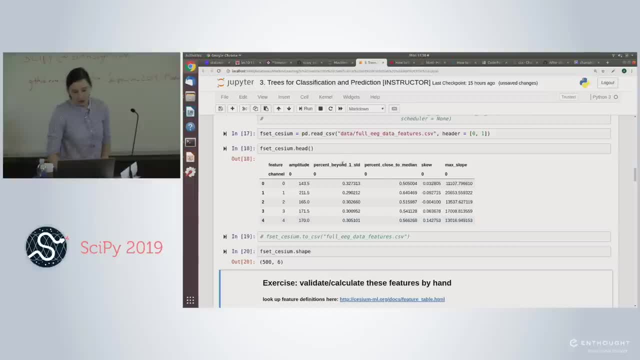 It's just 500 by 6.. And actually one of those is just the channel, so it's not even relevant, but I've digested 500 times 4,000 points down to 500 by 6 points, right? 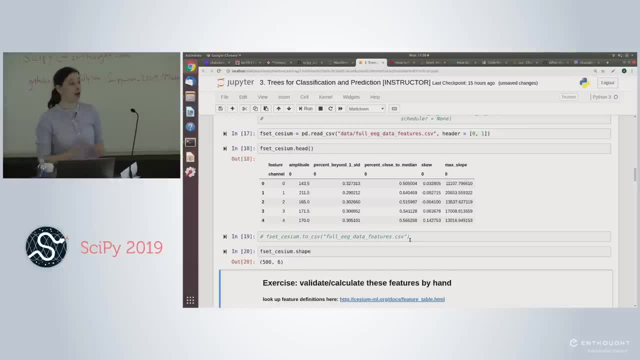 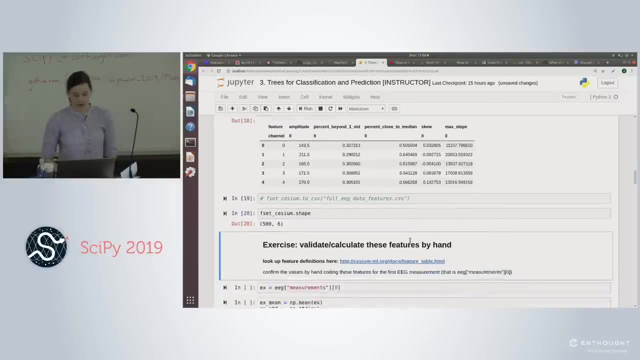 So if I'm in a rinky-dink laptop situation in particular, or if I'm not, but I have some enormous time series database and still need to compress it down, this is a way to do that. right. I've really shrunk my data down. 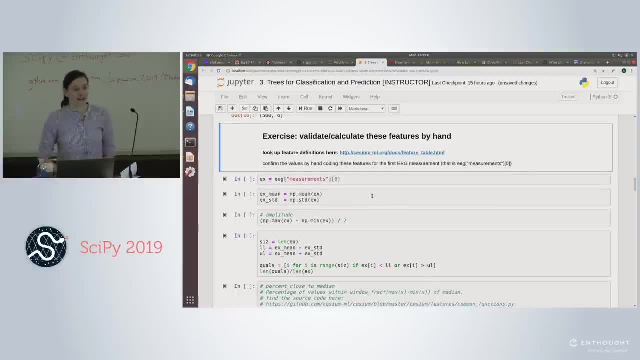 We're going to skip this exercise of validating slash calculating these features, but I just want to point out that you can right. So cesium is this feature generation library. It is not the only one. There are plenty of Python feature generation libraries. 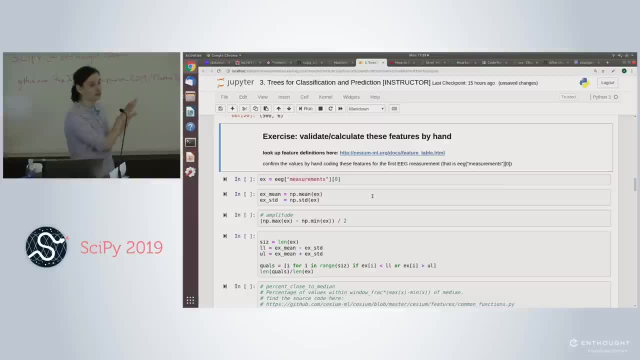 Some of them are general purpose, like I talked about that Catch-22 dataset. They have this general purpose library And some of them are specialized, such as I mentioned. there are astronomical time series, feature generation libraries. It's good to know these libraries are available, especially for things like these features. 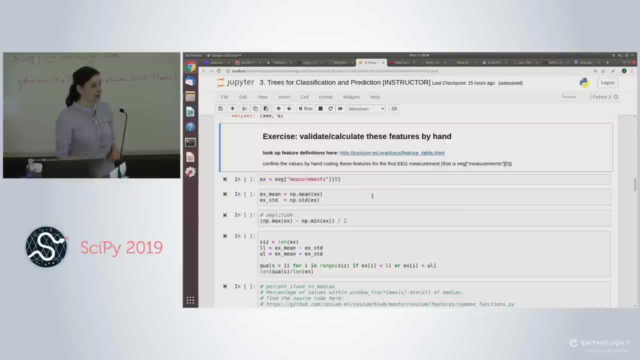 I can absolutely write out the code for these features, which I did here, but it's a pain in the butt right For sort of standard things like calculating the skew or calculating the max slope. why should I hand code this? all right. 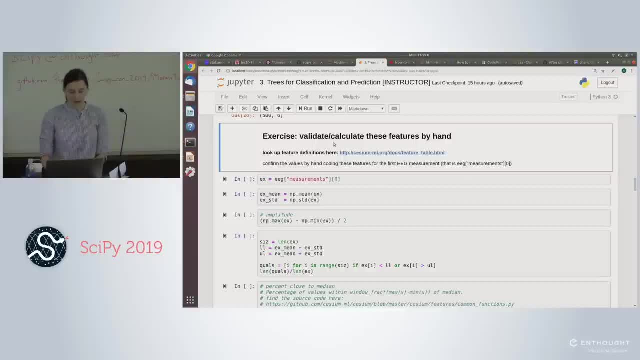 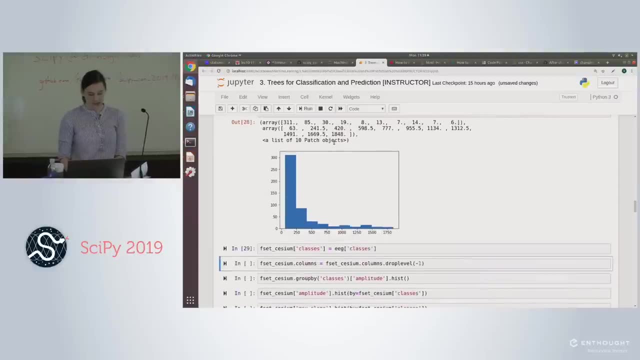 So, especially in the exploratory component, I might want to just farm that out to an existing library So you can check on your own time that indeed the features we calculate match the features that are produced by the algorithm. I just check for one data point. 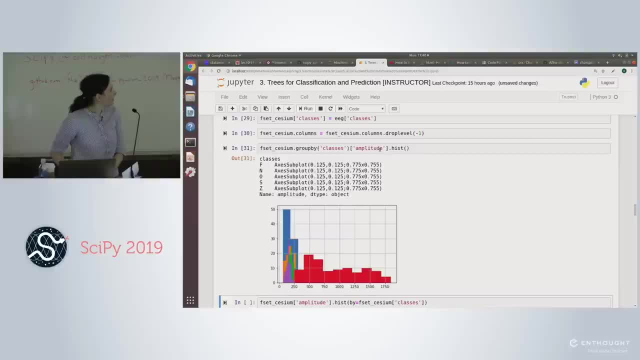 And we can also sort of think, OK, well, are these meaningful? So one thing I did, for example, is did a histogram of the amplitude feature by class, And it looks like at least for one class right, one class at least distinguishes itself. 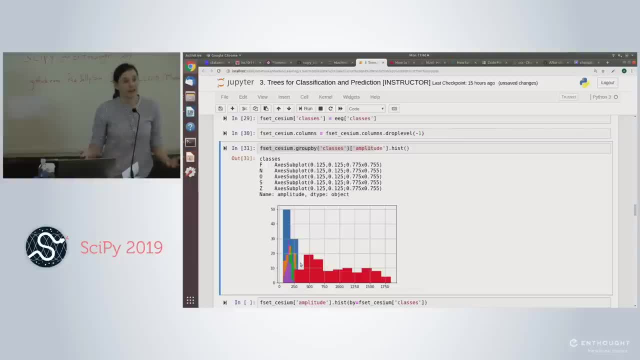 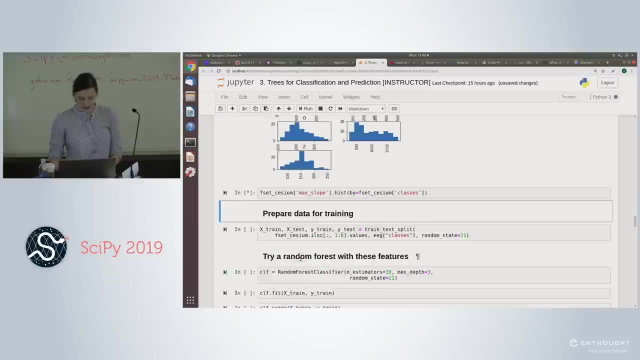 compared to the other. So, OK, there's at least some preliminary evidence that some of these features will help to distinguish classes, which is what I want to do. OK, So these are some other examples of plotting histograms. to again check, are these features? 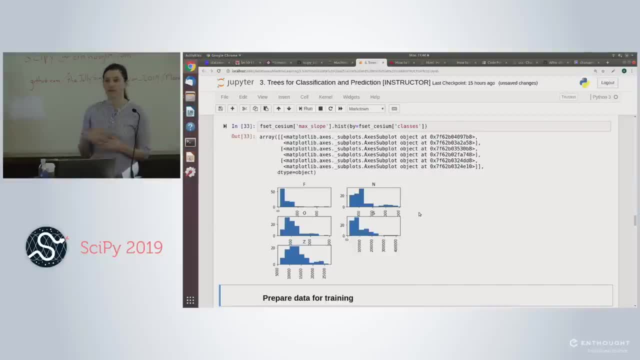 I generated, Are these features I generated somewhat useful And in fact, you can go through quite a bit of feature importance analysis By the time. you're doing that for time series, it's just like how you would do it for cross-sectional data, right? 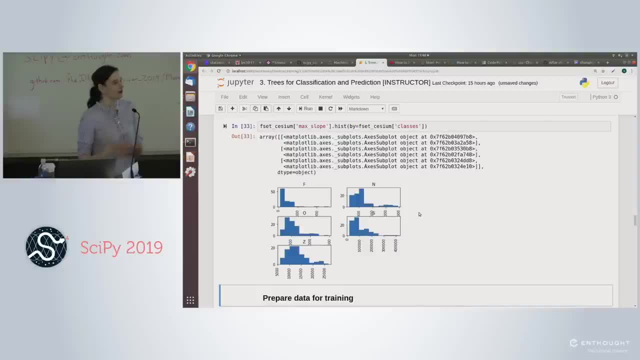 Do the features I'm producing tend in some way to correlate with the outcome I'm interested in, be that a classifier or a forecast or whatever it is? So you definitely would want to go through and check that they're sensible. You also. ultimately, if you have a well-developed set of features, you probably at some point 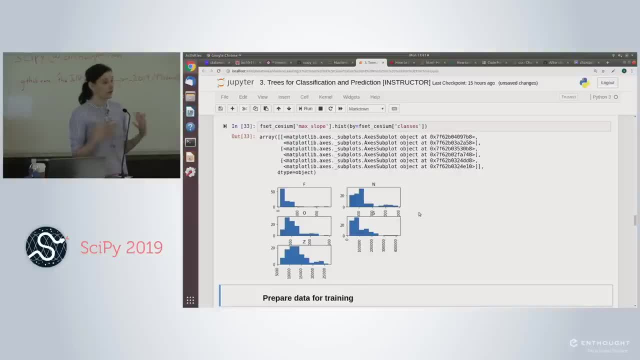 would want to code them yourself right. So if the features I'm using in Csium or other feature generation libraries are useful in the sense of, why should I code up the same things repeatedly? there's a few solutions to that. One is, if you do this enough, you'll just have your own library, which is even better. 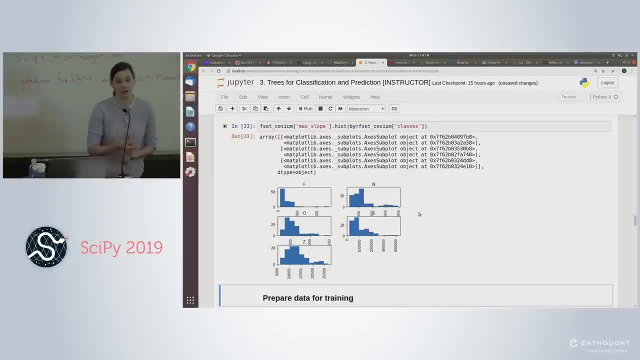 because you really know it line by line, and you know how it works. Ultimately, if you have a really well-developed set of features, you also don't want to use an out-of-the-box solution because that's coded to be very general. 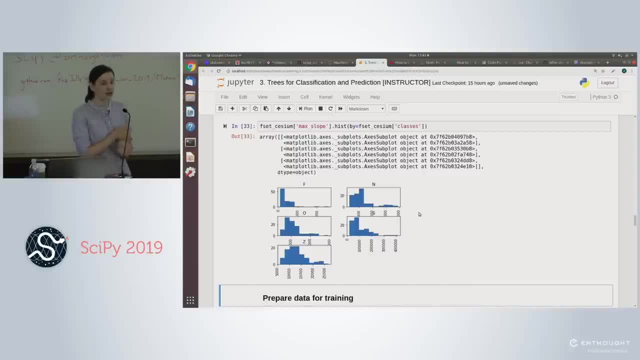 If I, on the other hand, know the same three features I always calculate. one thing to keep in mind is sometimes features can be calculated in a way that's not necessarily accurate. Sometimes features can be calculated together to cut down on computational costs, right. 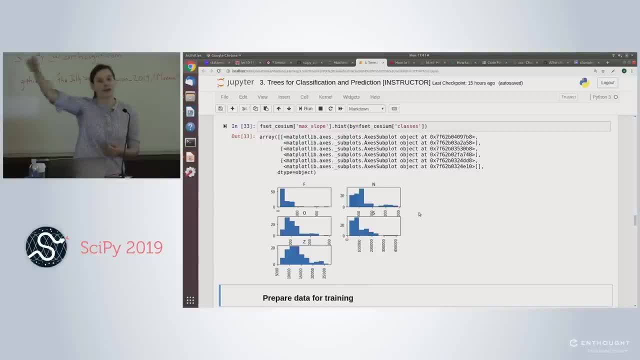 So if I'm looking at min and max, there's no reason to do one pass through the data to find the max and then another pass through the data to find the min, right, So you might want to group all things that go through the whole data in the same way. 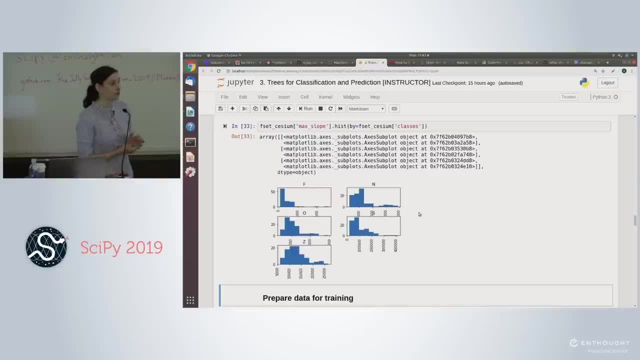 and do them all together. That's not something a feature generation library will do for you. I have not yet seen an example, though I'd love if anyone has one, of somebody sort of coding things up to take advantage of those. That would be a great contribution to the open source community if anyone wants to. 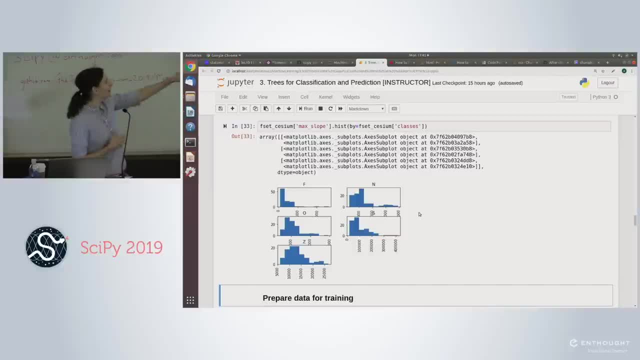 but it's not something that I would do. So in the meantime, be aware of that, because even in this really tiny data set, I found I had to wait quite a while to generate the features right. So this can blow up very quickly and you don't want to spend whole afternoons at work. 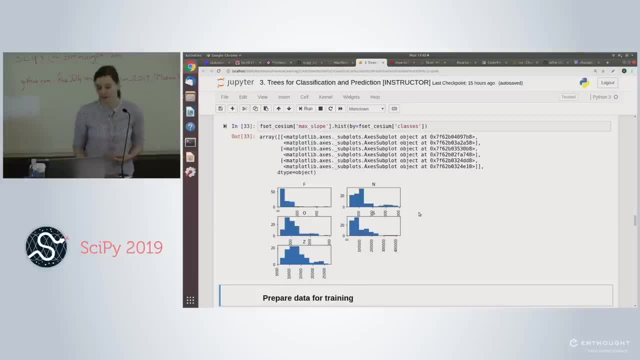 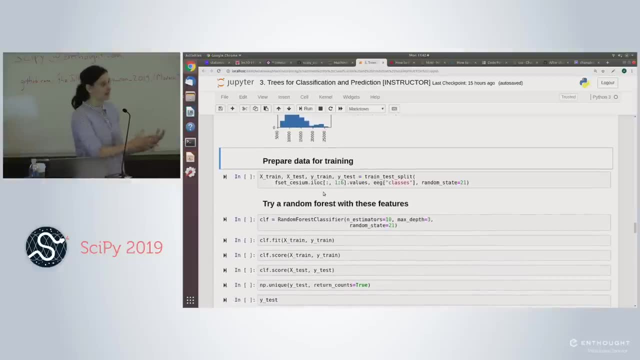 sort of sitting there waiting for features that may not even be very useful. Okay, So that's the feature generation. It can be quite straightforward. It should be domain specific, but in this case we sort of went with a few common sense features and we're going to see how they work. 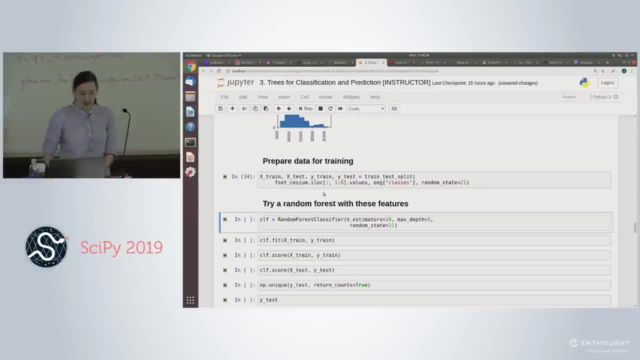 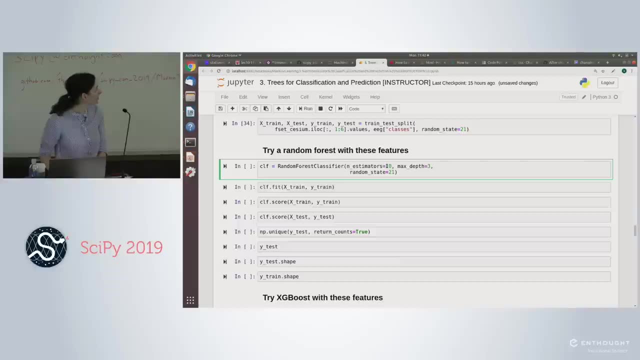 So we prepare a training and a test set and let's roll out a random forest classifier. we're going to use 10 estimators, a max depth of three, set a seed for no particular reason. We're just saying, okay, how does this random forest do? 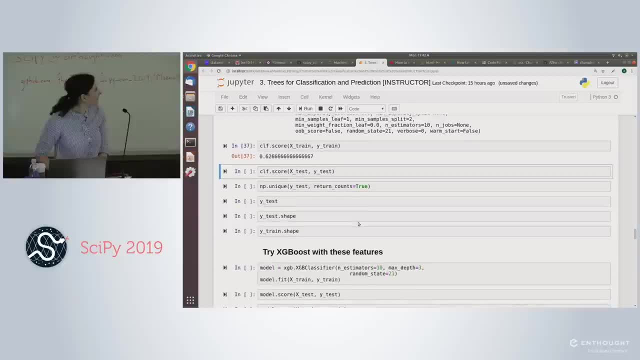 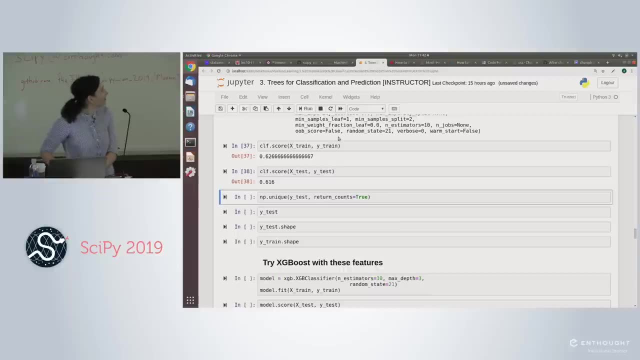 So if we fit it and score it on our training data, we've got like a 62%- 63% accuracy. The good news is our test data is not much lower, so it doesn't seem like we overfit. It seems like we have a reasonably generalized model. 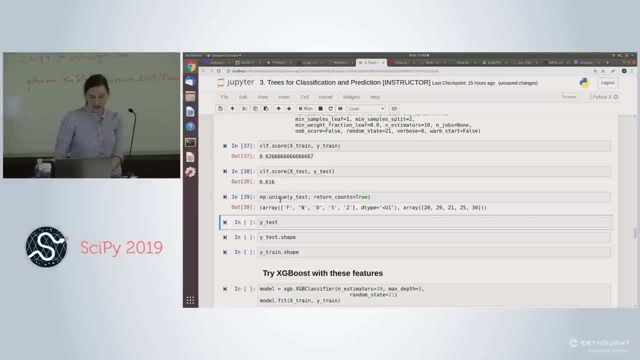 And if we look sort of at what came back, it also looks reasonably well distributed. So we have five classes. They're all sort of distributed in our underlying test data. So that's something interesting to know when we're thinking about our possible null model. 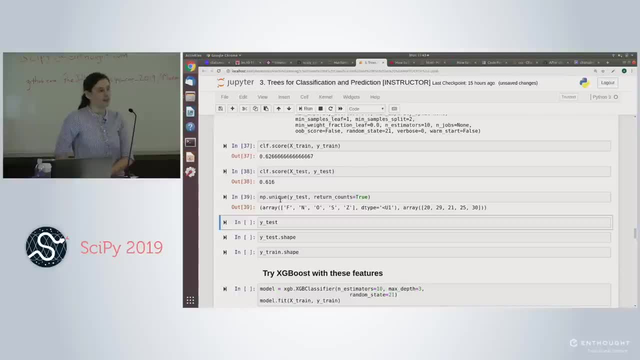 right? So when you think about, is 62% a good accuracy? of course you want to think about: well, what would even a really dumb model do, right? So if we have five classes, a dumb model would not be doing 60% accuracy, right? 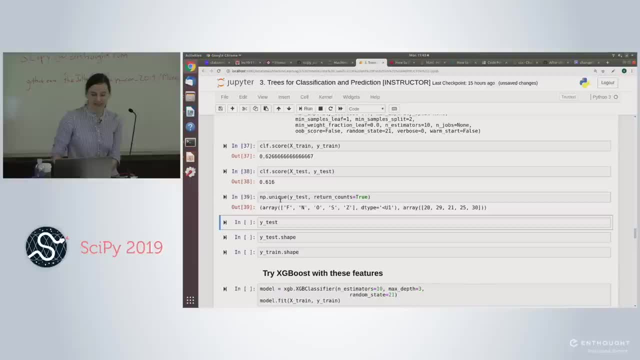 So it's just some sort of sanity test that Our data is indeed doing something. So that's our random forest, right? It's just to point out. okay, you can put some features in and get a classification. that is far better than a random classification with just five features. 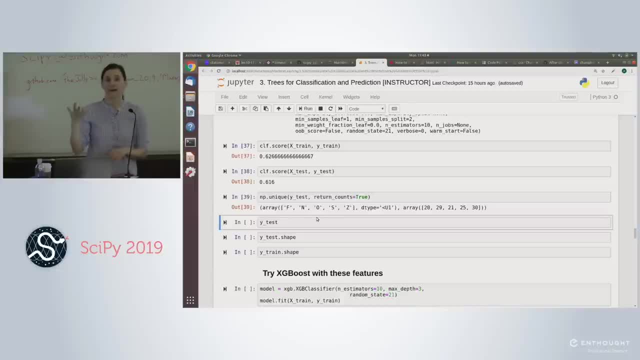 So I boil it down essentially 4,100 data points to five data points without even much exploration, and I could already do something right. So time series classification is not that hard to get some kind of result. that is better than random. 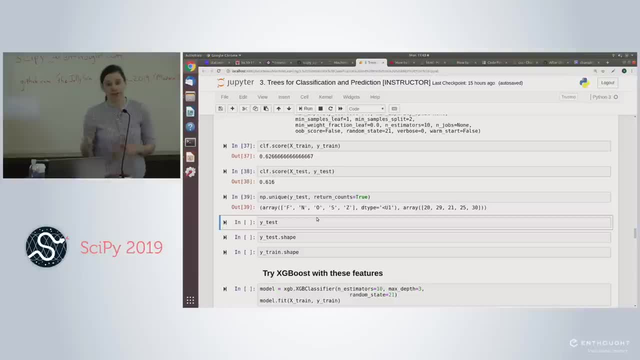 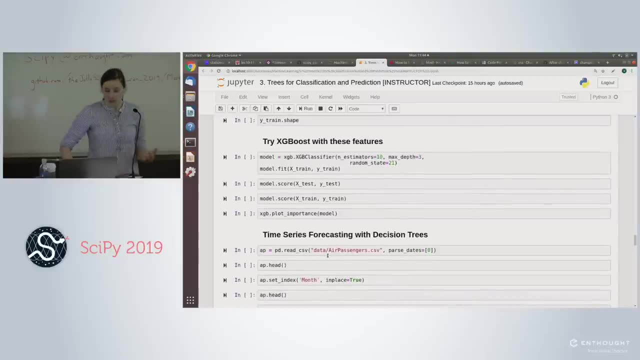 and that really boils a whole data set down to just a few numbers, And it depends on. It depends, of course, on the quality of the data and what you're looking at. Okay, So now we're going to run through the exact same analysis, just with XGBoost instead, right? 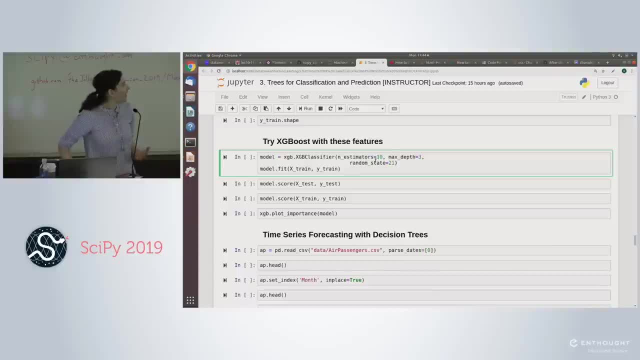 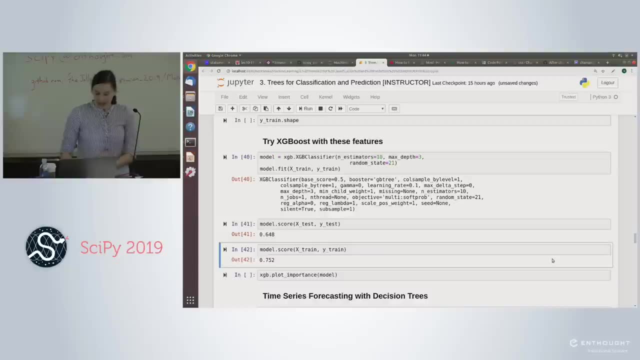 So now I'm going to use an XGBoost classifier, I'm going to again use ten estimators and max depth of three. I'm going to fit that and I'm going to score that. And what I see now is I have improved right away on my random forest model. 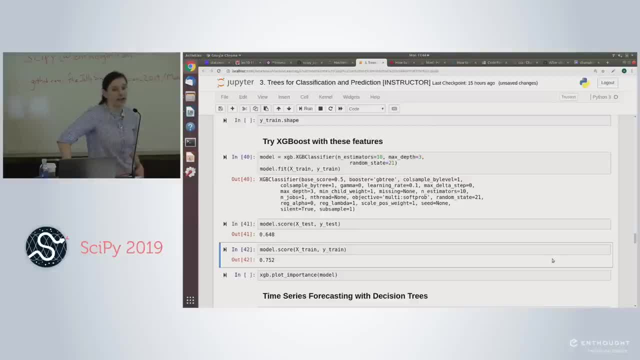 This is, as a rule of thumb, quite expected with time series. So, as I was mentioning, XGBoost and gradient boosted trees tend to do extremely well on time series data relative to what had been there before. So that's something to keep in mind, although, of course, here we do see a little bit of evidence of overfitting. 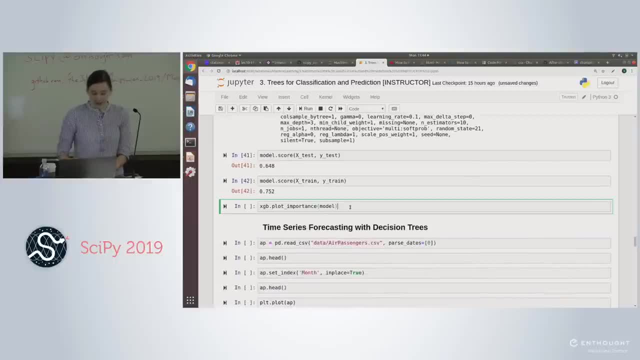 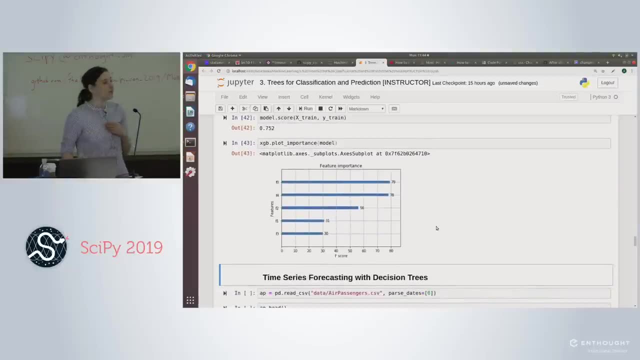 so I might want to prune that back. And, as a reminder, what you get with XGBoost that you don't get automatically with a random forest is some measure of feature importance. So if you were iterating and thinking about, okay, well, what features turned out to be useful? 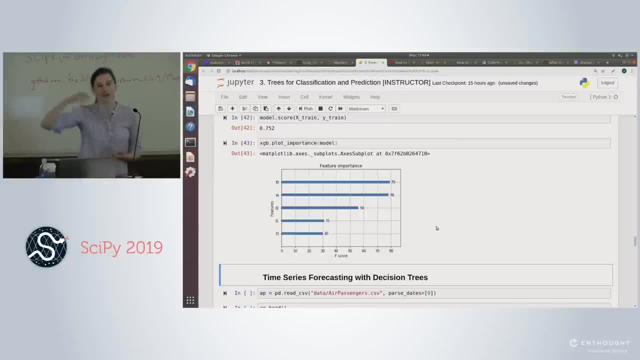 especially if you don't want to go through all the time series and plot them all, If you don't have time for that, or if the time series are just so noisy that the visual is not giving you much information. you can use something like feature importance as one way of thinking about what kinds of features are useful. 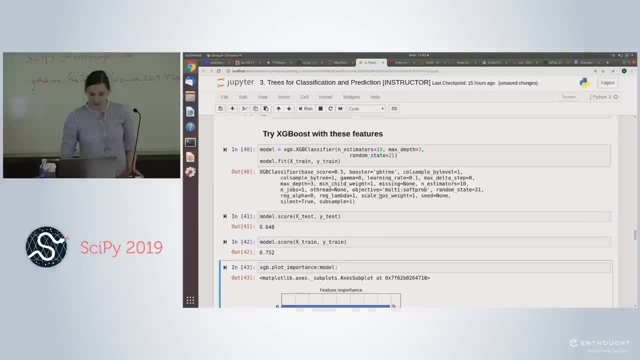 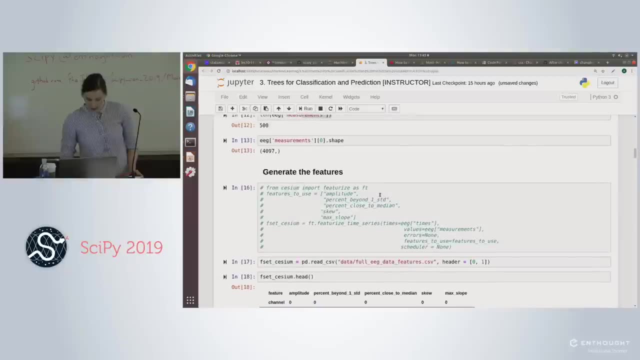 And then you might look and say, okay, so feature zero is useful. and what was feature zero? anyway, If I go all the way back up, what was that? So that was the amplitude right, And that was actually one of the things that jumped out at us. 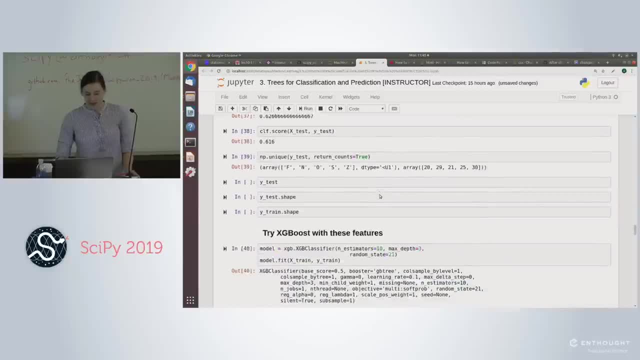 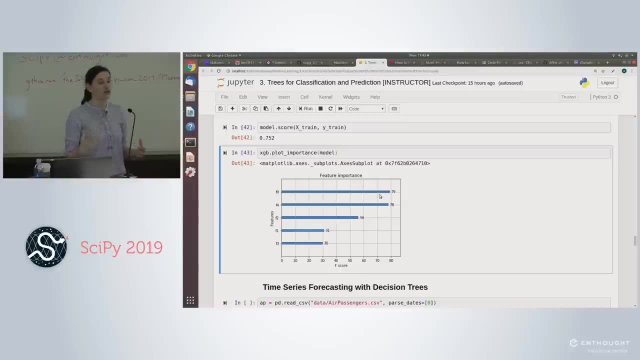 So if it says amplitude is useful, right, These indicators of sort of the numerical range is useful. One thing I might do to improve this model is say: okay, well, what other sorts of features provide similar but complementary information, right? So maybe, in addition to the amplitude, maybe I need to add the mean or something like that to provide more information. 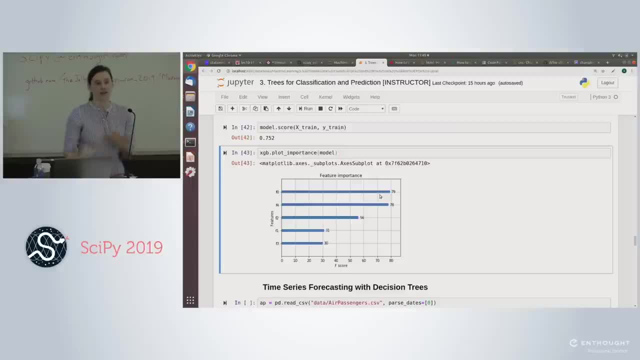 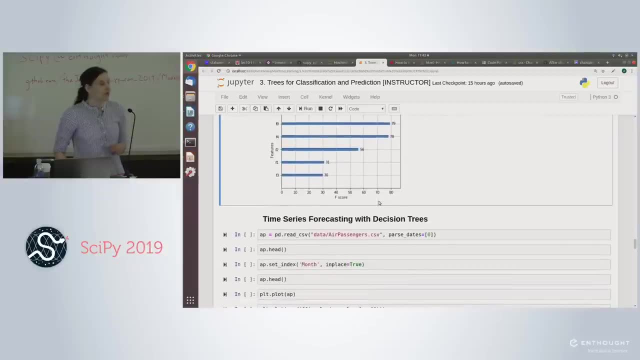 So you can use this as a way of sort of learning, also for this kind of data. what is useful, So that's classification. We also want to think about forecasting, though, right, So in this case, we're going to do this. 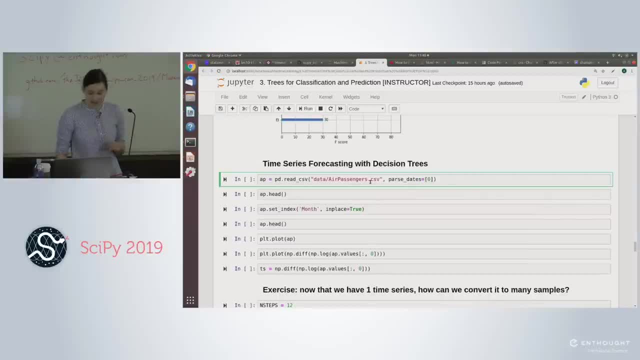 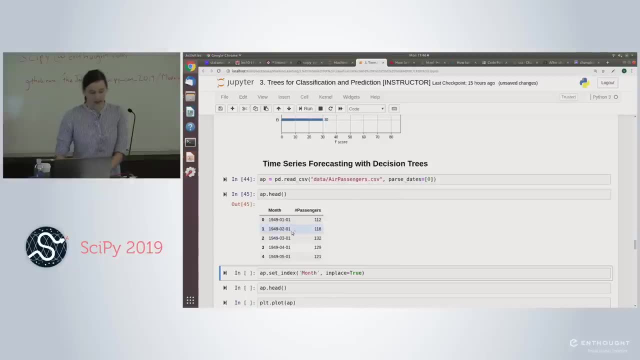 We're going to take a look at the air passenger's data set, which I highlighted in a slide at the beginning of the lecture. So we're going to load the air passenger's data set. take a look at what this looks like. So here we can see. we've got monthly data going back to 1949.. 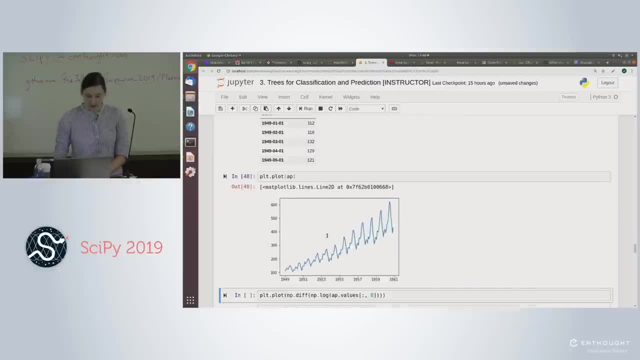 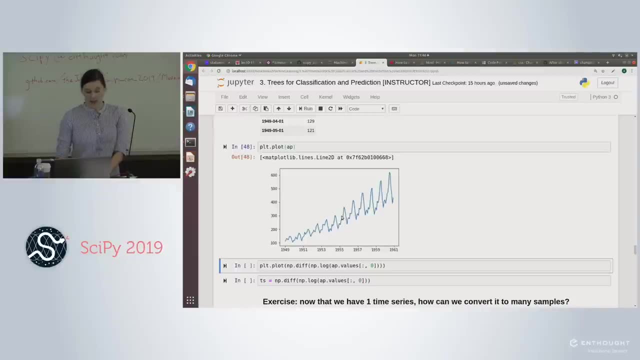 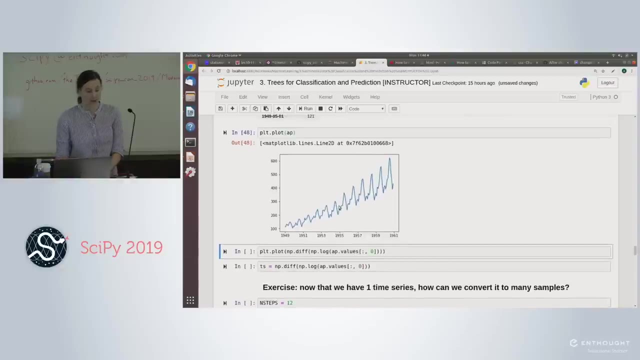 Set our index and take a look at what that looks like. Let's plot it, And so here we can see the plot. There's definitely some seasonal component and there's also some trend component that's going up Now. if we were doing, say, ARIMA modeling, we would definitely need to make this stationary. 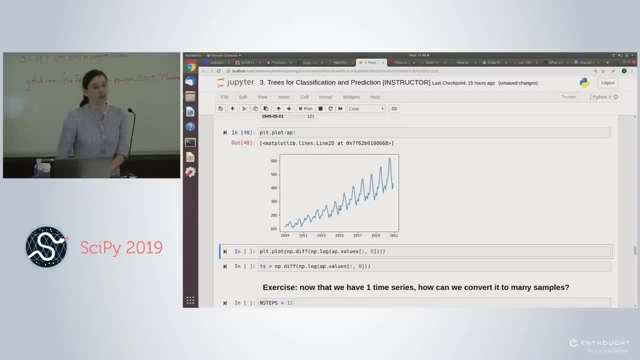 That's not a per se requirement with something like machine learning, but it is generally a good idea, right? So some of the same considerations about what your data looks like for traditional statistical models are still things you can do to make your data cleaner and easier to digest for a machine learning model. 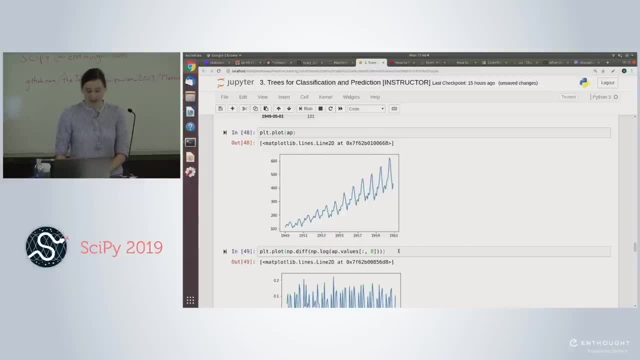 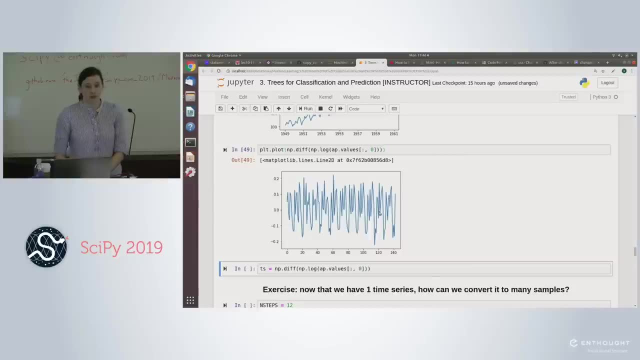 So let's think about log transforming this and also diffing it. So if we do that, we get a time series that is zero. We get a time series that is more uniform in its variance and values, right, Which has to be a good thing, because basically, what we're doing is making all the sub-series from this time series more comparable, right. 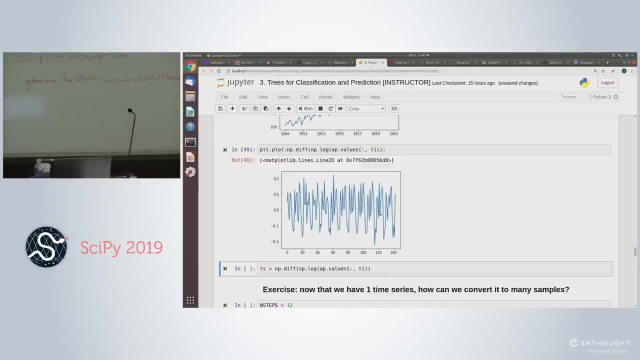 Because what we're going to do effectively to do some learning here- is we're going to slice the time series. So this one time series is going to provide us many different options and many different samples by having a sliding window right. So this could be one sample. 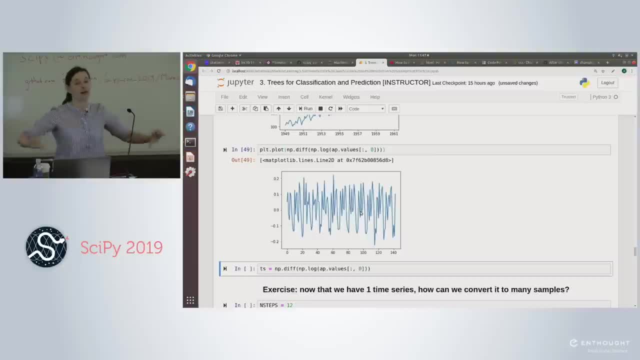 This could be another sample. This could be another sample. So if I have one baseline time series, I'm going to convert that into many samples for my machine learning algorithm. So here is where we see another difference compared to a statistical model or a state-space model. 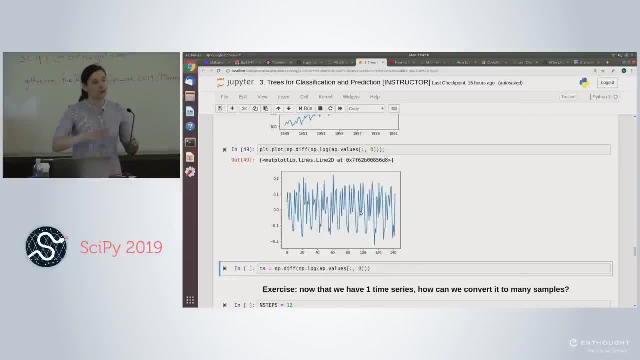 In the statistical or state-space model, the model for inputting your data is: you have one long time series and you throw that in. On the other hand, with machine learning, the model has nothing to do with being aware of this temporal component of the data. 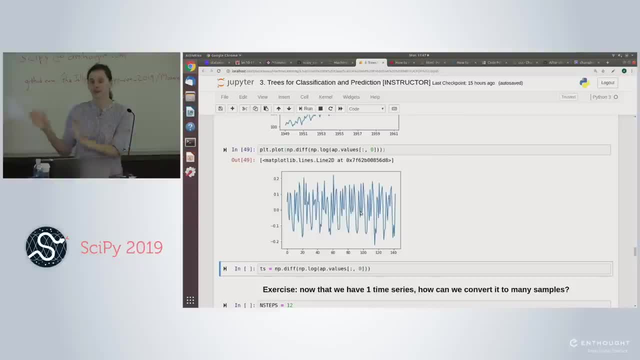 So instead we take different time windows, we chop up our time series and those become different samples. So here comes a way to use one time series and just model that one time series for machine learning. So why is this different from what we just did with classification? 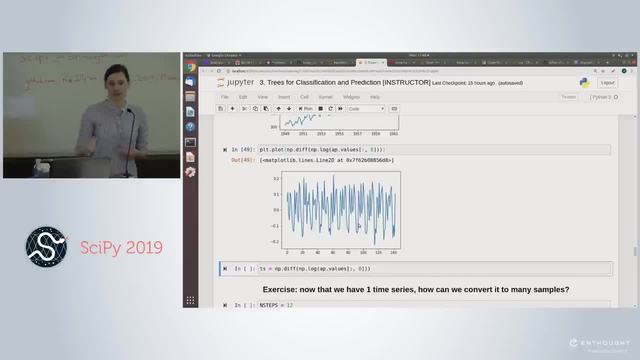 Because we're trying to forecast, and we're trying to forecast one series in particular. If we had many time series, then that would be a different consideration. Do we want each time series to just be one sample, Or, even in that case, do we want to chop up each of those time series into sub-samples and use them all? 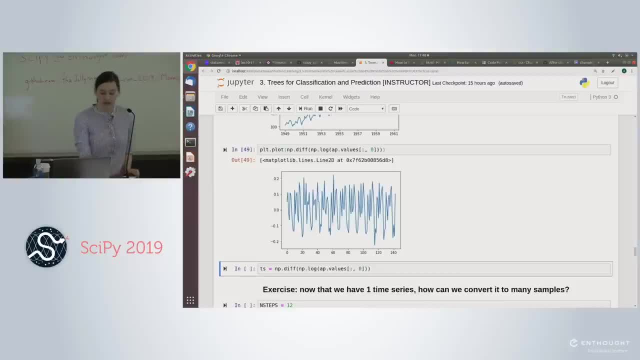 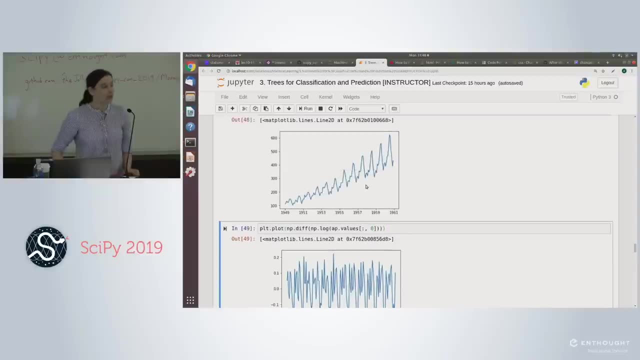 But, in any case, what you want to make sure you do, since you're going to be doing a sliding window across here- is you would like to make all these data points as comparable to one another as possible, Because if you think about a machine learning perspective- right. 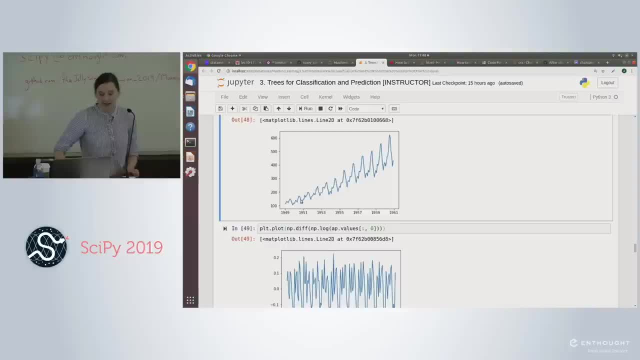 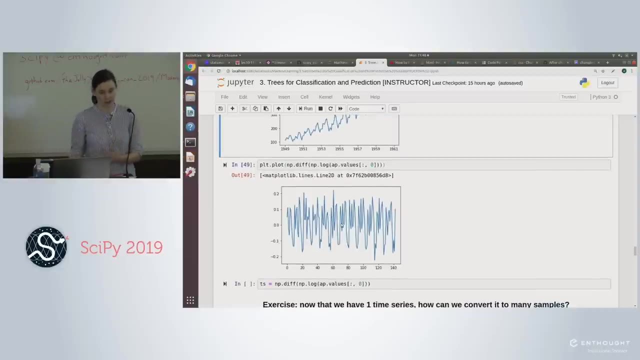 the machine learning algorithm just sort of sees a slice here and a slice here and it has no way of sort of knowing which dynamics should be carried around forward or which dynamics are unique to a particular aspect, Whereas if you give it this, they're all clearly more comparable to one another thanks to those transformations. 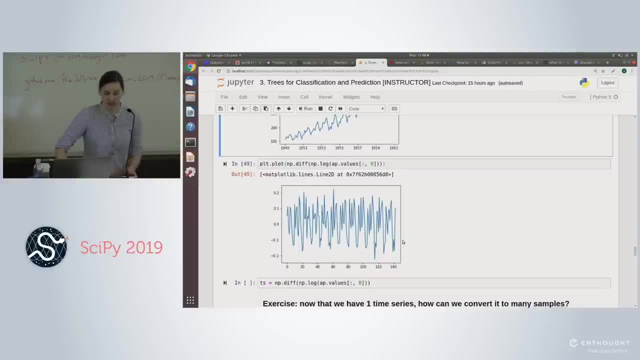 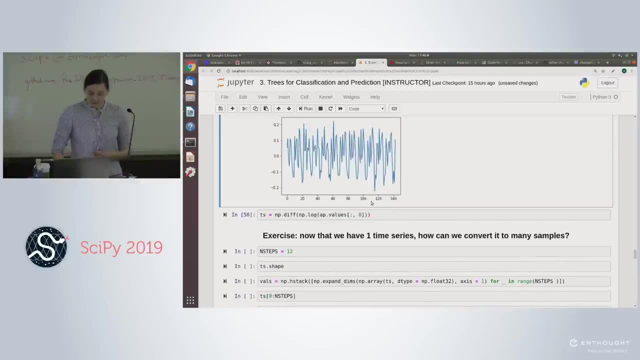 And then you would just need to make sure to transform back at the end when you wanted to check your predictions. So we're going to have a time series that is the diff of the log of these values And now, as an exercise, I'm going to ask you to think about: 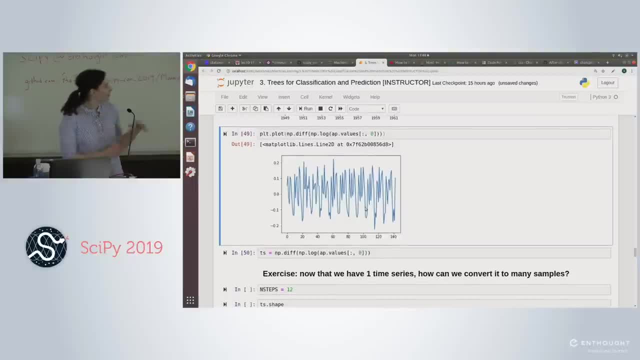 now that we have one time series and we have it in a form where sort of all components of the full range of time look very similar, how can we convert that to many samples? So take a couple of minutes and think about how you would chop this up to create different sub-time series as samples. 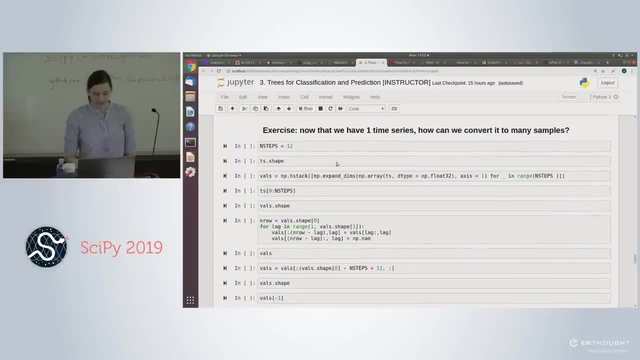 Okay, so let's take a look at this together. So what I decided to do- and there's no reason that this is especially great or anything, but I decided to break it up into 12 months, so to sort of look at a year at a time. a slice. 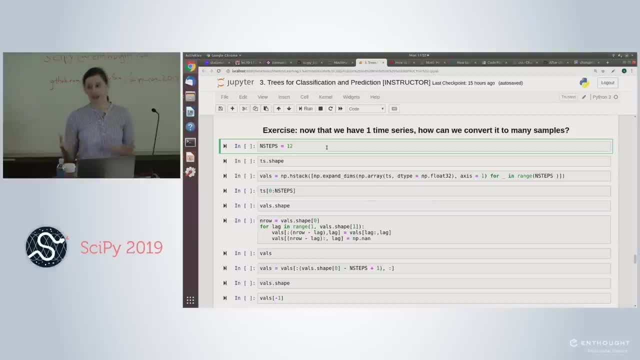 Now, arguably that's not so great, because you can't really capture the seasonality if you just have one sample of the season. But I said: what the heck? that's what I'm going to do. So 12 steps. I think what 12 steps does give you the opportunity to do though. 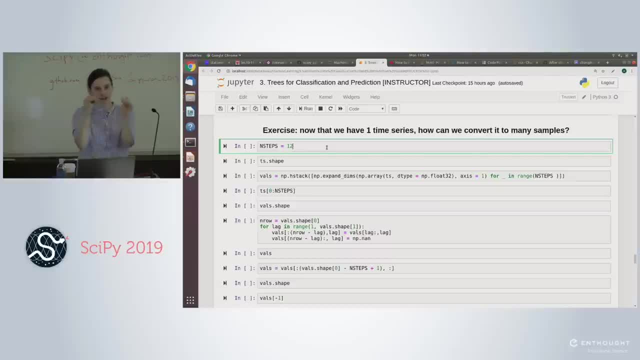 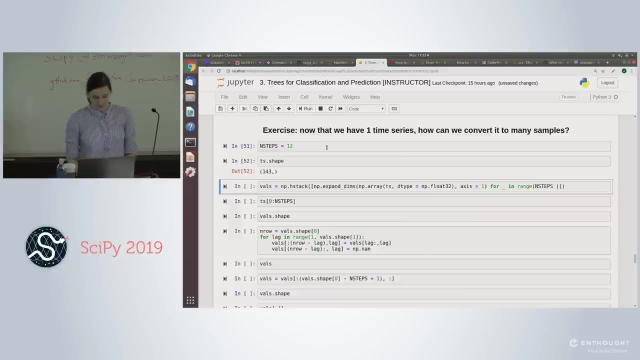 is maybe at least be able to pinpoint where in the seasonal cycle you are, when it's looking at many examples, Whereas if you have too few months, you probably can't spot that at all. So that was part of the rationale, And then what I did was I wanted first to just give it. I pre-allocated this array of vowels. 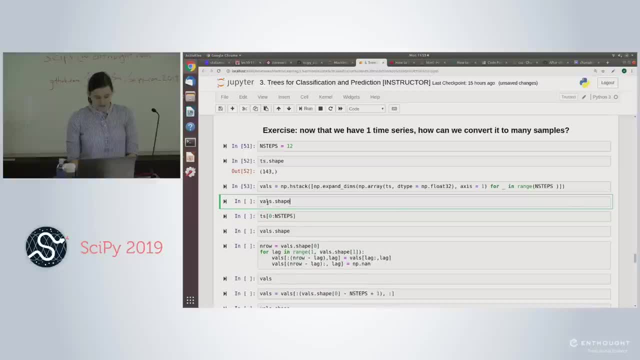 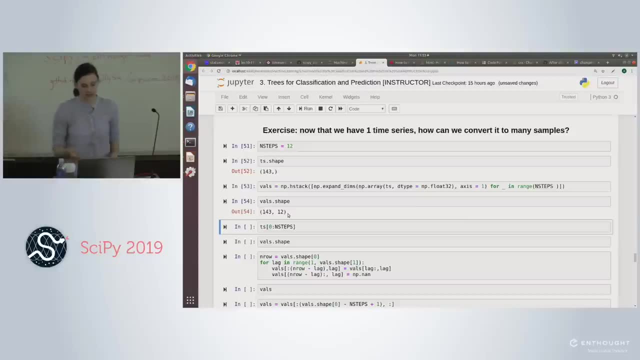 So if we look at this, it's 143 by 12.. So basically, I've just stacked the time series 12 times because I'm going to want 12 time steps, And then what I do is I'm just going to lag it. 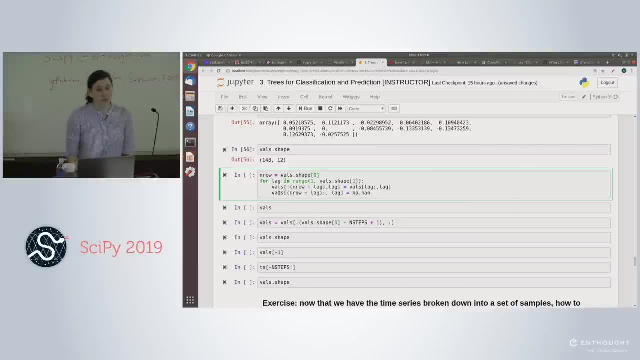 And I'm sure there's a more elegant way to do it. I used a for loop, just you know my janky solution and I don't have to think too hard about it, And basically I just, for each column, I shift it up by however many lags I want right. 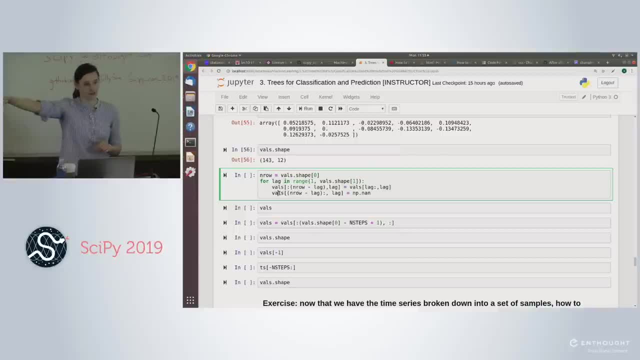 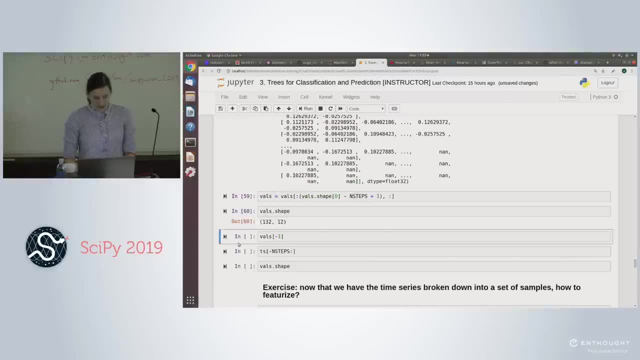 because I want the first value to be 12 months in the past relative to the last value, because I want to move forward in time. So if I do this, then I get this vowels. So now I have only 132 by 12.. 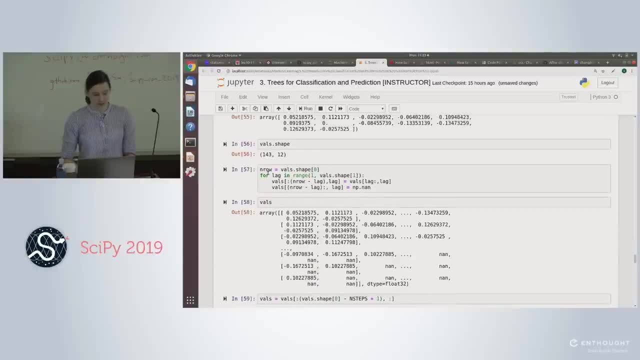 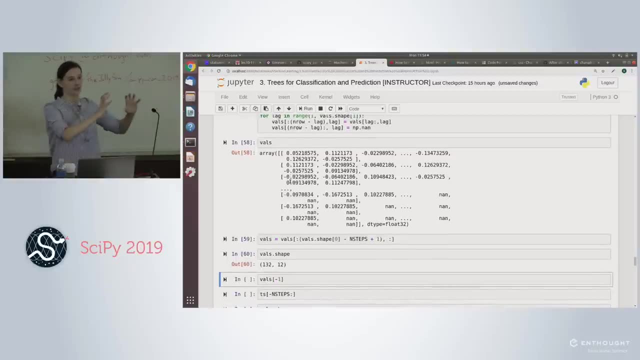 So why did I go from 143 samples to 132 samples? Well, I lost the samples where I was. I don't have a full 12 months right. So at the very beginning of the time series, I don't have those 12 months right. 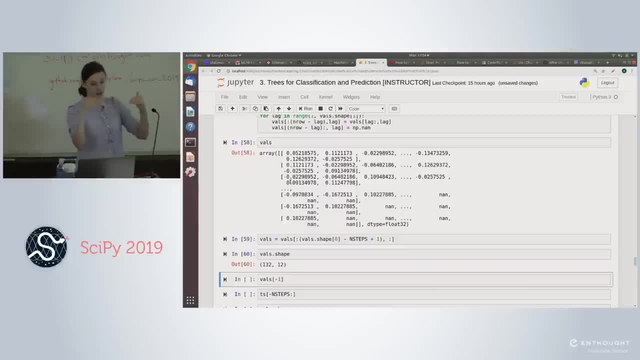 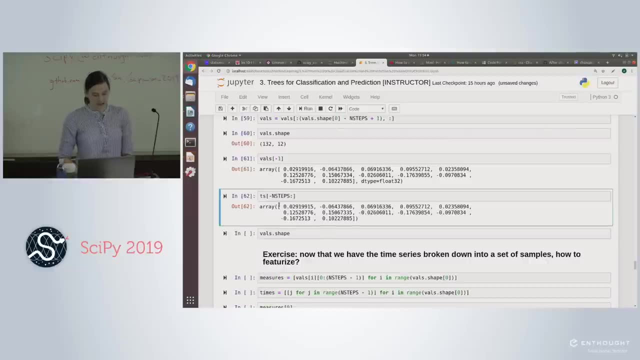 I have to go 12 months into the time series to even have one sub-sample of a time series. So if I look at that, I can then look at, say, the last n steps of my time series, right? So that's this time series I depicted up above, right? 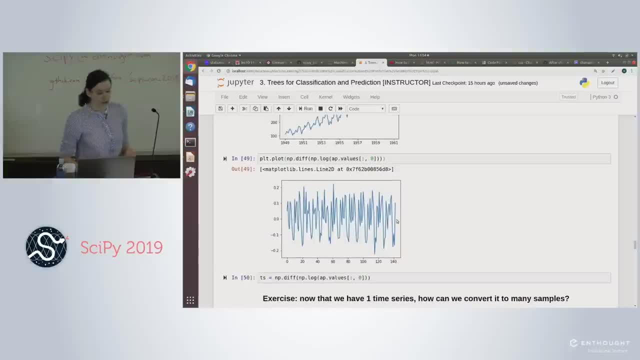 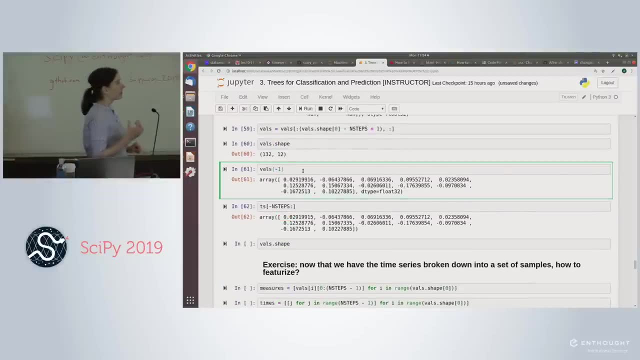 So my last 12 steps are these last values, right, the 12 last values of the global time series, And that becomes the last sample, now that I have broken my time series into individual windows, right? So vowels minus 1 is just my last sample that I'm going to in some way process for a machine learning algorithm. 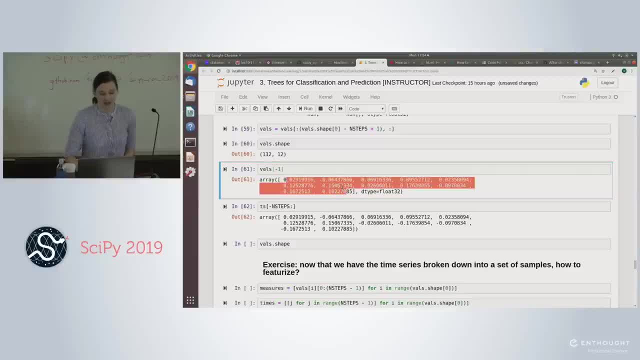 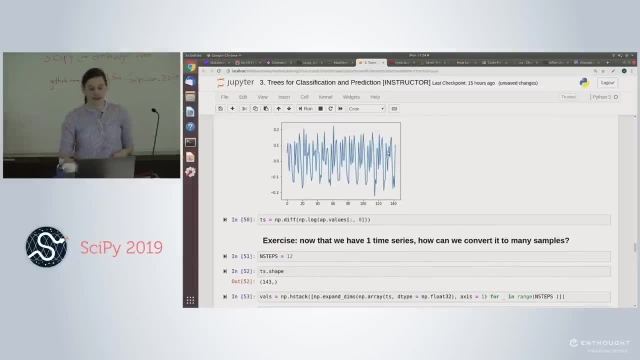 And notice these are the same values, right? So I basically I converted this box of, say, the last 12 samples. That's now sort of one sample time series. One thing I hope you noticed is that I could actually have more samples. 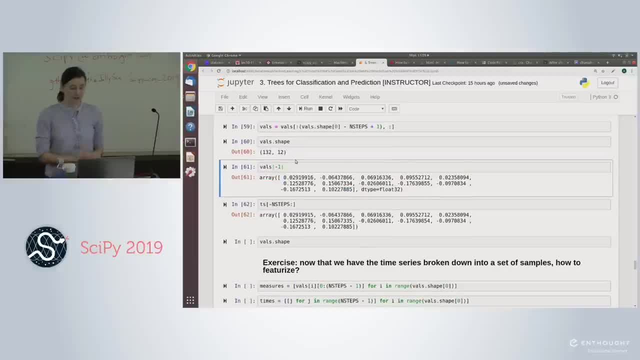 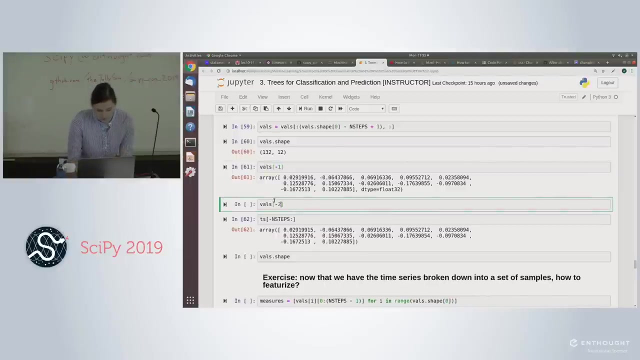 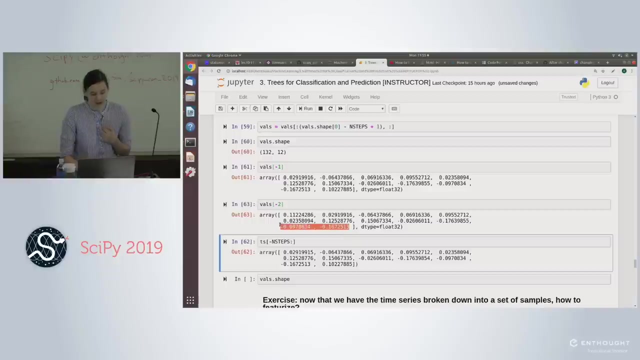 Right now I only have 132.. What would be some ways to have more? Or at least I can think of one way, Let's see. So minus 2. They do overlap. So if you look see, I have minus 167 minus 09 and then minus 167 minus 09 here. 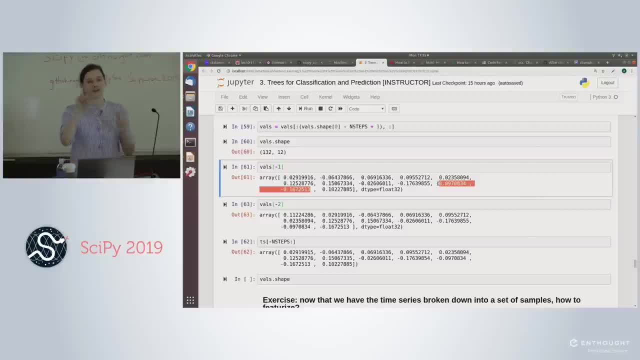 But actually that's a fantastic point And when I do my deep learning example, that was like my trick there was that we don't have overlapping and we could right So if I have chopped it up to have non-overlapping time windows, that's kind of silly. 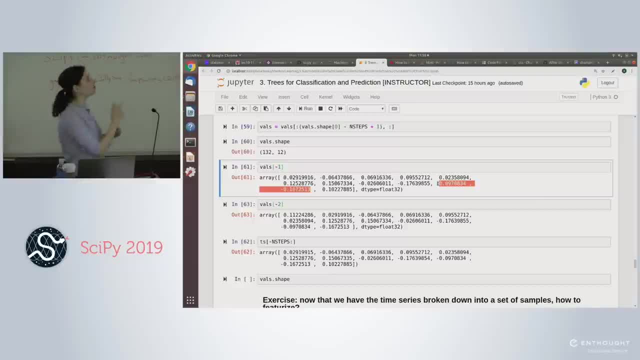 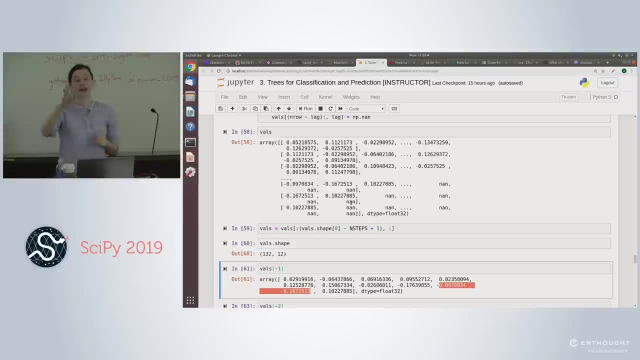 If I think I want more time series, I should just have a sliding window, which is actually what I've done in this case, the way it was coded up, just by lagging one at a time rather than chopping them up, Whereas if I had done, say, a reshape- 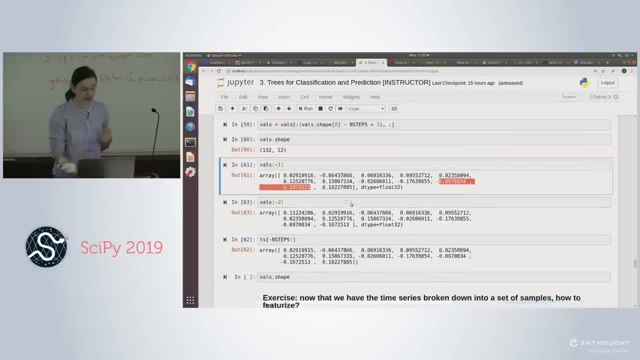 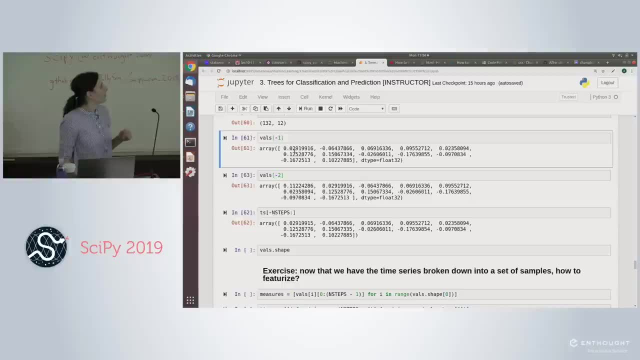 I certainly wouldn't have had overlap and I would have had to put that back in. So I do have overlap already. So I'm using each point as much as I can. I guess the thing I want to point out is if I reduced my number of steps. 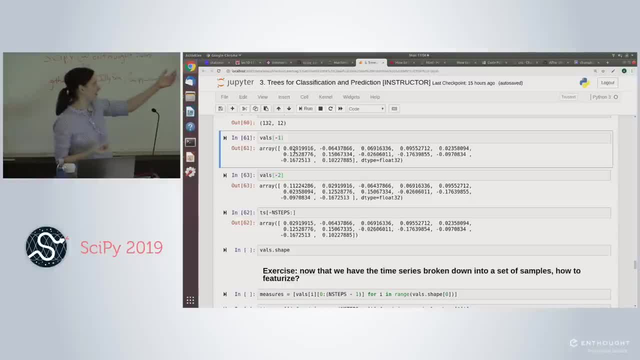 I could get a couple of more time points out of there, right? So if I had only six steps instead of 12, I would get six more sequences. Most of the time that won't matter. Maybe in such a small set it might matter. 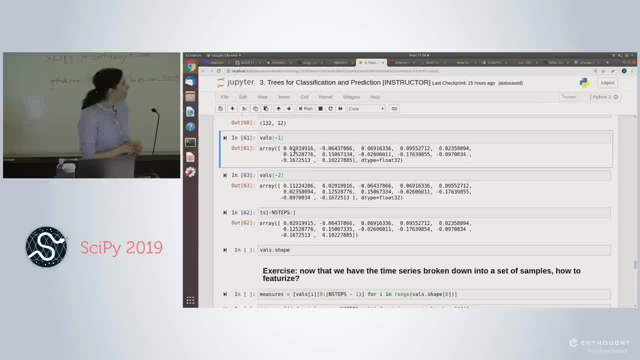 So that's something to think about. Another thing you could think about less used in machine learning compared to deep learning, but you could think about doing some data augmentation if you have some domain knowledge to think about ways to augment your data in a way that's realistic. 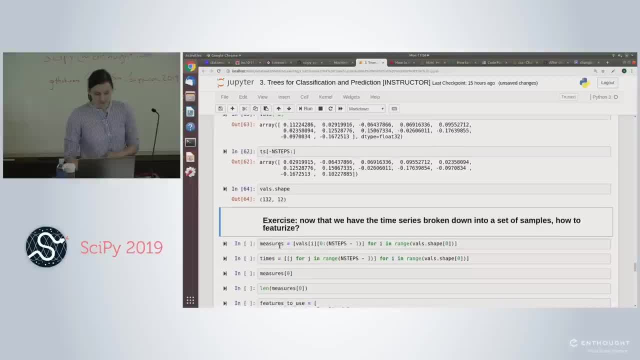 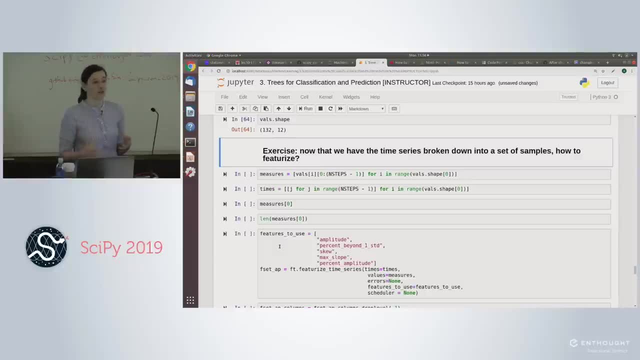 Okay, so that's how I prepare my data. So I've just created shorter time series. I haven't actually created features yet, right? So with forecasting we have this additional step of first we take our long series and we break it up into smaller series. 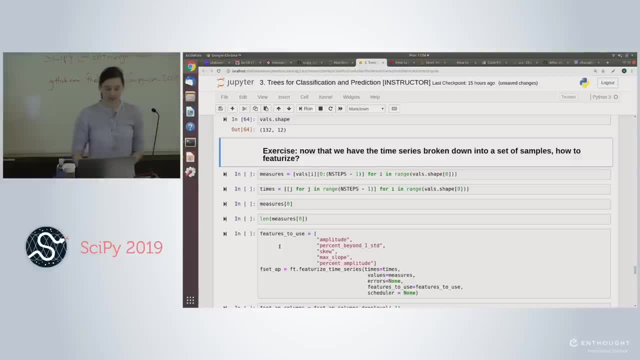 I still need to featurize, right. I still need to do the same thing I did earlier for the classification, So I'm going to do that here. So I convert my measures to a list, because that's what CZM expects, right? 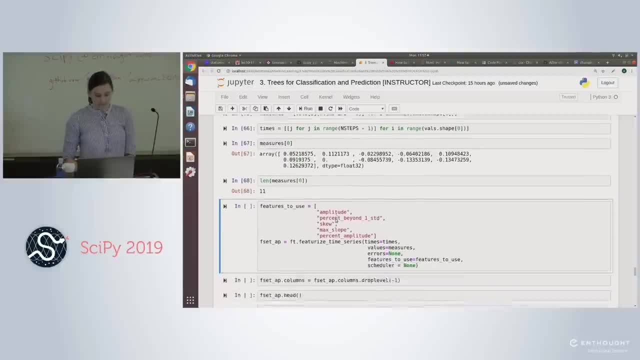 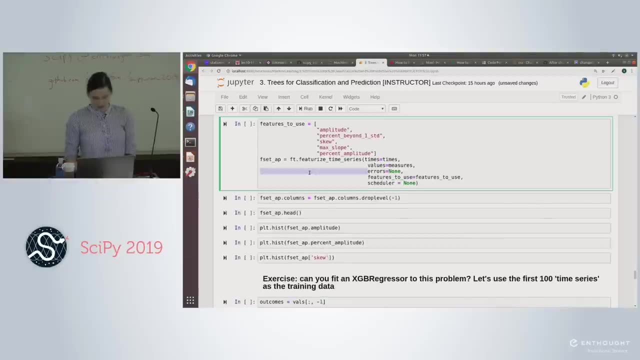 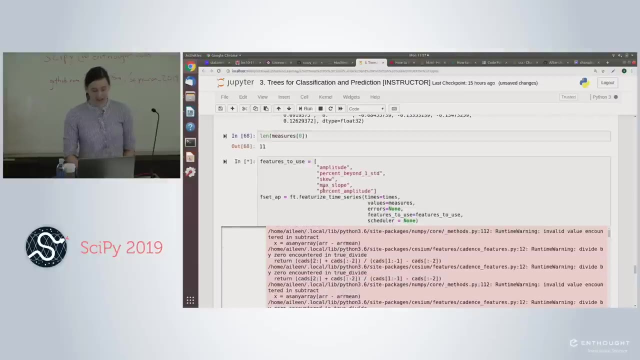 So I've got my list of measures And each measure is this 11 time steps long, And then I'm going to featurize This one. I'm going to run through just so you guys can see: This one is small enough, I can actually do it. 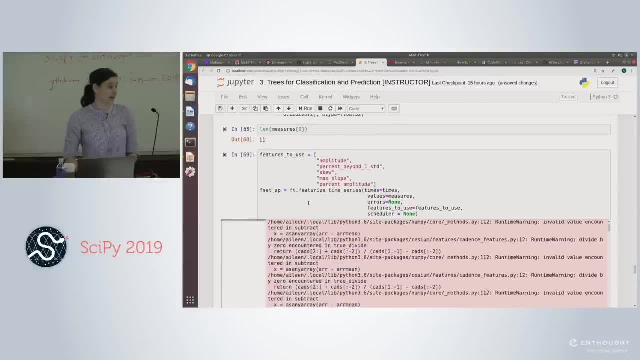 But as you can see, at least on my rinky-dink laptop, it still takes a while right. So even this really tiny data set, that should be instant, but it isn't, in part because this is not a very general library. 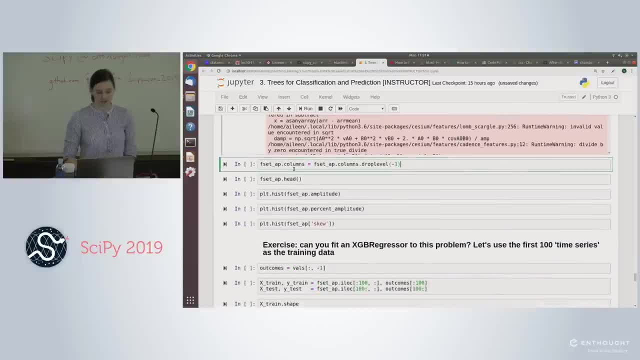 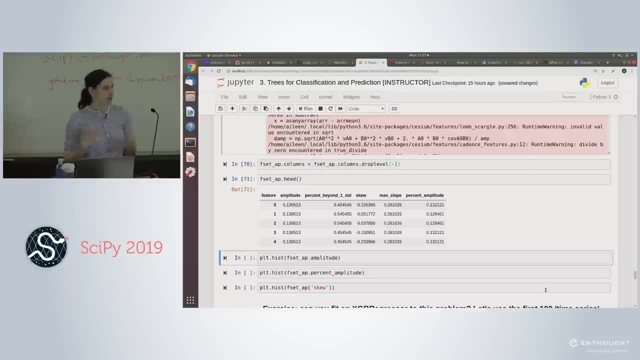 and in part because time series feature generation is just that slow. So if I look at these columns, what have I got? I think these are the same features I used above, so sort of a generic set of features. If I look at the histogram of these, let's see. 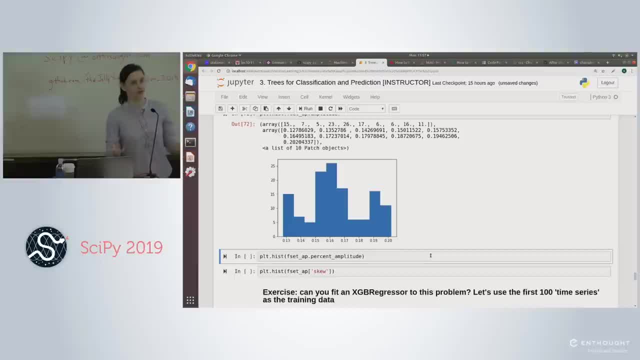 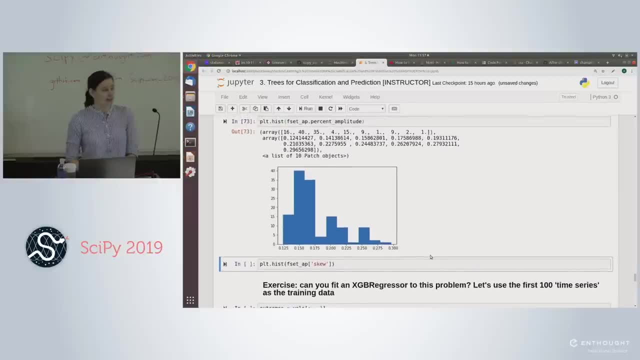 Oh well, I see it's sort of multimodal. I'm like, wow, that's cool. Maybe there's these underlying populations. I can get all excited about some possible structure. Similarly, if I look at percent amplitude, I see something that might potentially be multimodal. 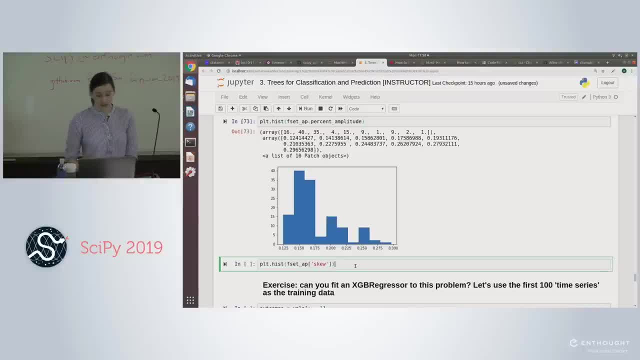 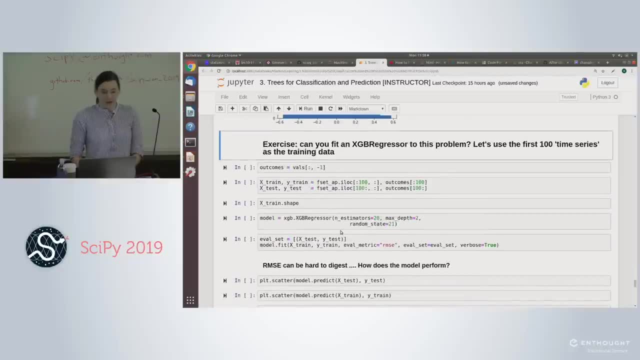 so that seems like maybe it could be good when I'm going to use a tree to do some kind of regression task. I like multimodal. It suggests there's some sort of meaningful data underneath, So I'm going to run now. I'm going to run instead of an XGBoost classifier. 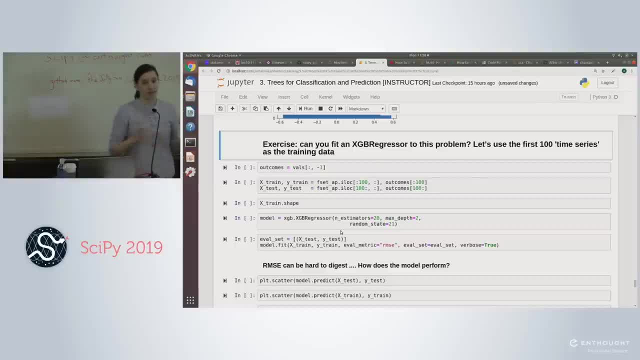 I'm going to run a regressor, So it's actually the same process. Now that I have converted my inputs to features, it's the same, except now I'm looking for a numerical output to forecast a value And my y instead of being a label. 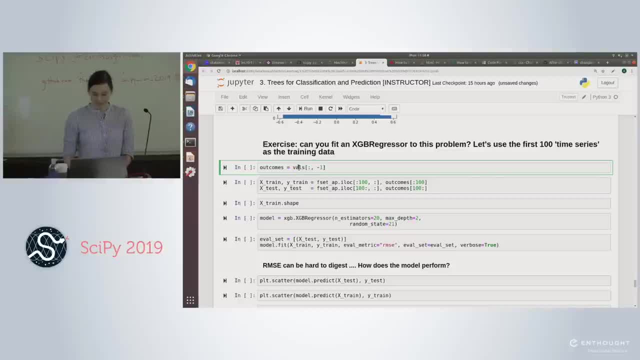 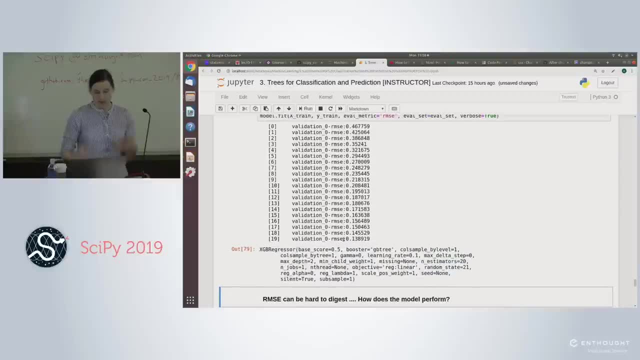 is going to be the forecasted value. So if I do that and I run my model, oh well, look, my RMSE is dropping. That's great. On the other hand, RMSE can be hard to digest, right? 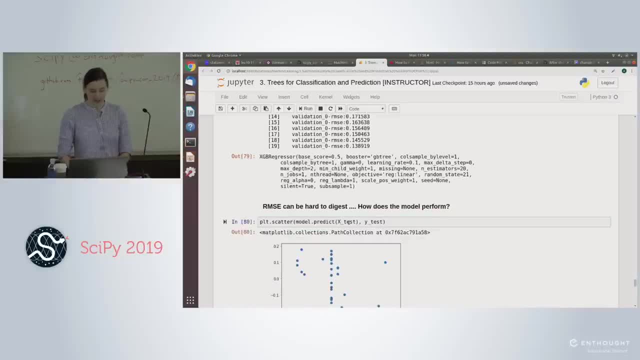 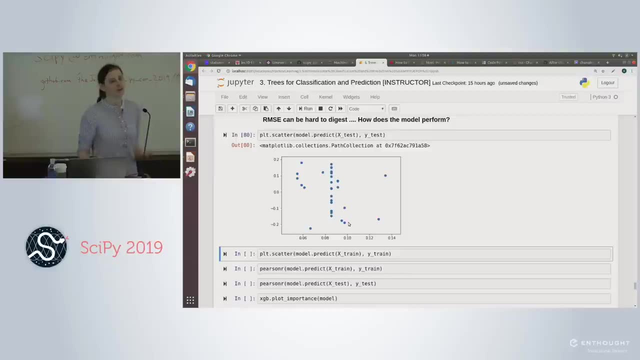 What does that really mean? So I can do a few things. I can do a scatterplot of my test data. Notice, I have very little test data because this is a very small data set. You'd never really use machine learning on such a tiny data set, right? 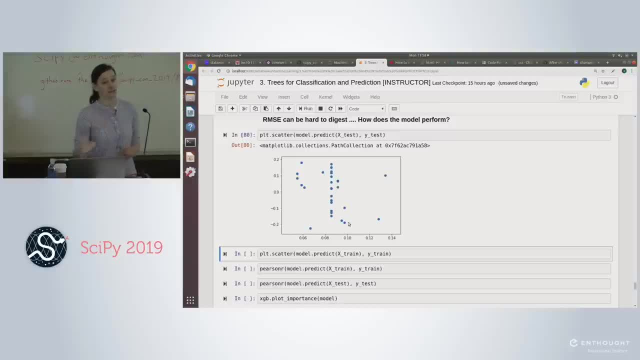 You know your real-world application, you would have more points, but that also means you could potentially be waiting many hours to generate your features. So obviously we're not doing that here, but do keep in mind your feature generation will just sort of blow up. 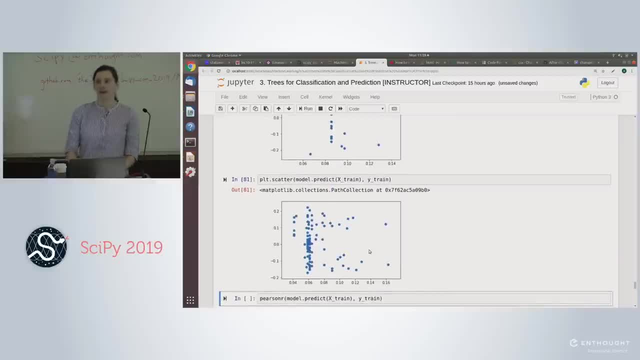 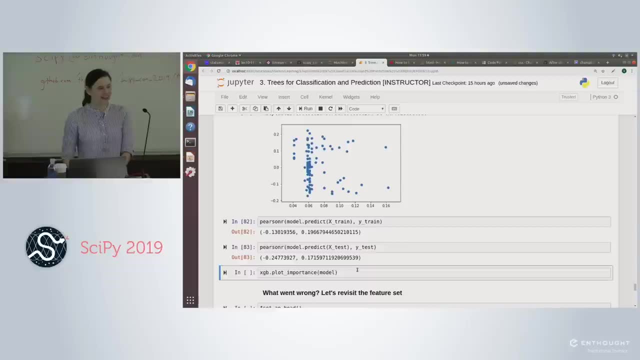 So if we look at our testing, and even our training doesn't look especially good here. This is really bad right? I was just telling you guys how amazing XGBoost is and how it has really contributed to machine learning for time series. 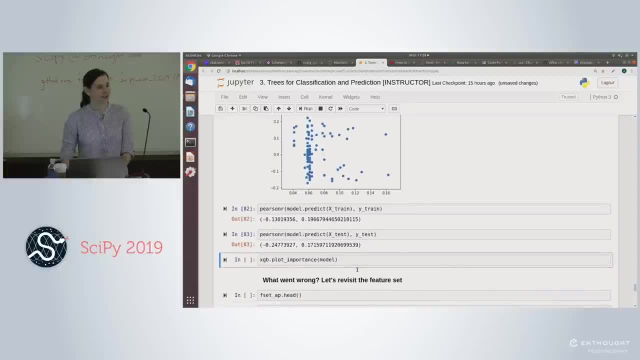 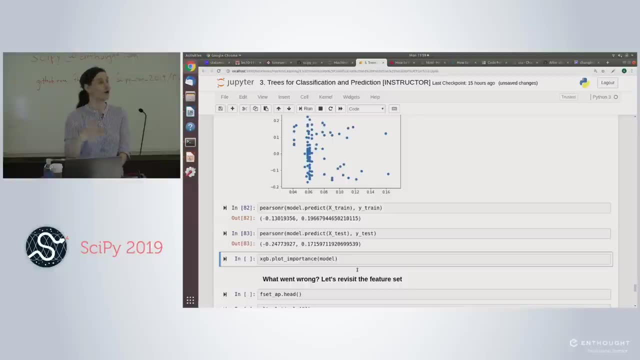 I even have a negative correlation and my actual value. That's really bad right. That means I'm sort of actively doing worse, even than chance. I would do better to just sort of predict zero always, rather than run my model. I certainly don't want to tell my boss this. 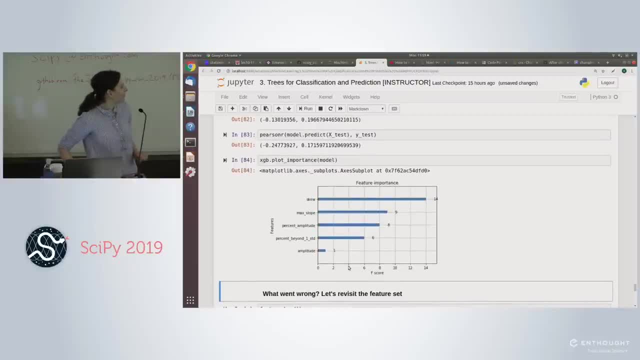 So exercise for the reader, although you can scroll down and see the answer. but just think for a minute What went so terribly wrong here? Remember this is actually a really easy data set right. I showed you at the beginning of this whole tutorial. 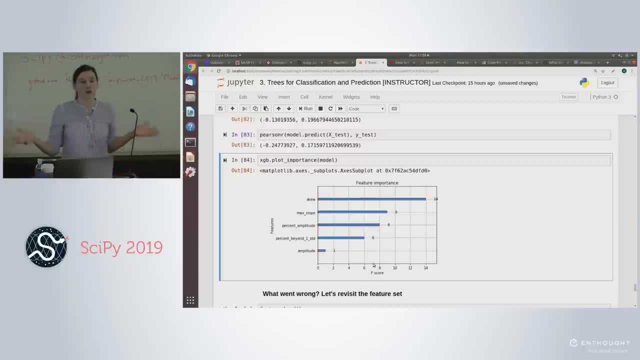 that our passengers' data and traditional ARIMA did great, So why can't I do anything? So certainly, transforming makes it harder, right, And that's actually. it's a frequent sort of mistake you see both in time series, research papers and also blogs. 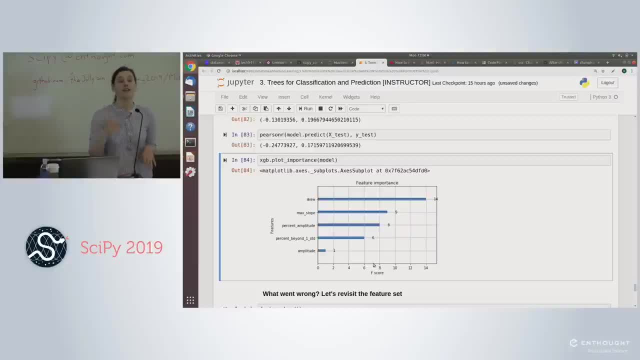 is, sometimes people get these amazing R squared values or amazing correlations, but that's mainly because they haven't transformed it And, sure, most of the prediction just goes into the magnitude. so especially when we diffed it, that makes it into a much harder task. 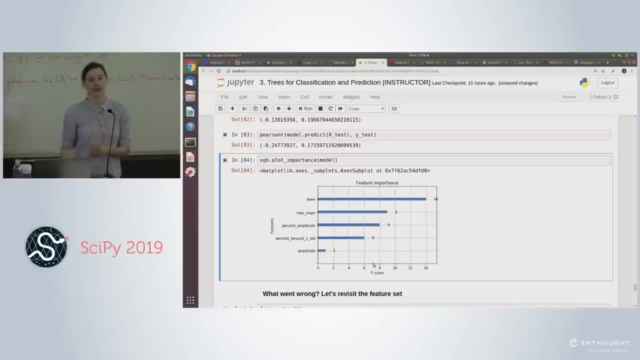 because once you diff a time series, predicting the last value for the next one is not a great strategy. So we have turned it into a harder problem. but actually, when you transform it and do an ARIMA model, you'll still get great results. 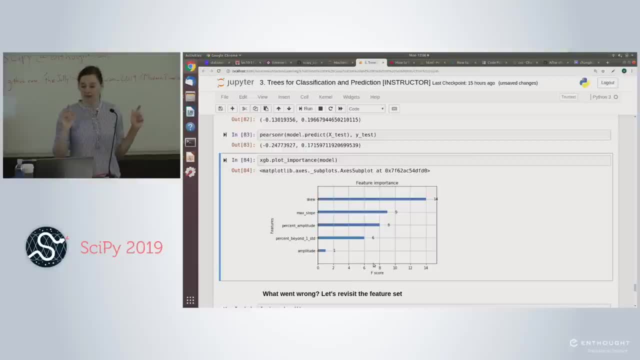 So that is not why- that's maybe why we don't get impressive sounding numbers, but that it still should do better than it's doing. So what? what could have gone wrong? So think about what we did. We sort of we took a sliding window of. 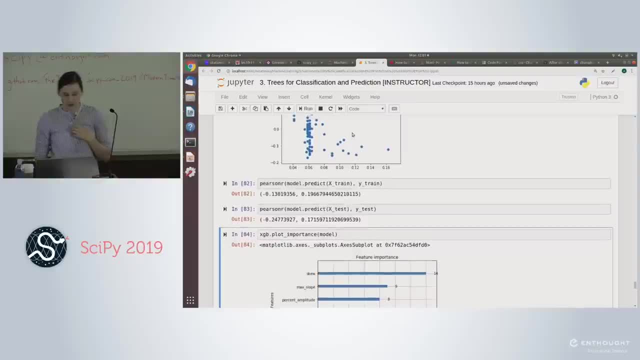 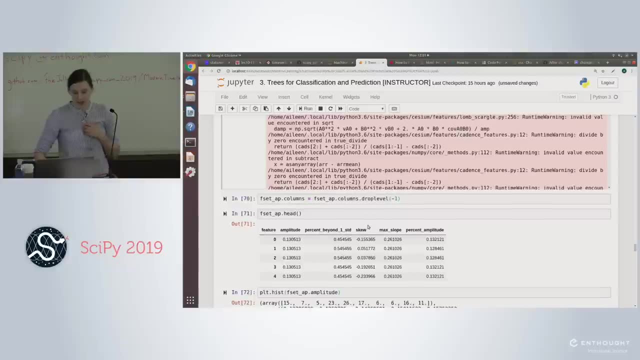 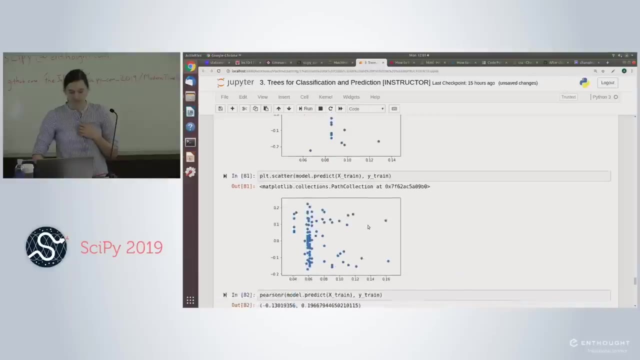 basically a year's worth of data, and then we summarized it with things like amplitude. what else did we use? Let's go back up Percent beyond one standard deviation, skew, max slope, et cetera. What else could have gone wrong there? 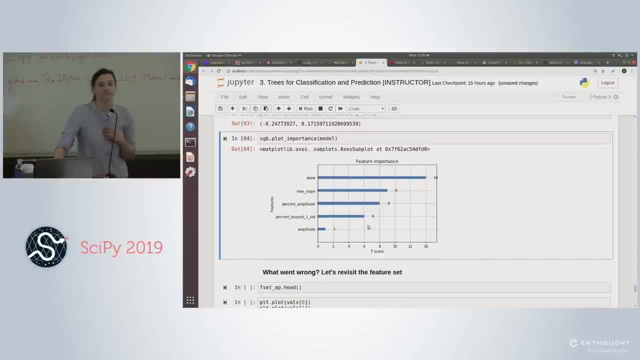 So I might buy that, and this is where it could be helpful to have the null model. I might buy this thing of. like you know, it's so much over time that it's not reasonable to forecast, But I guess I'd have two rebuttals to that right. 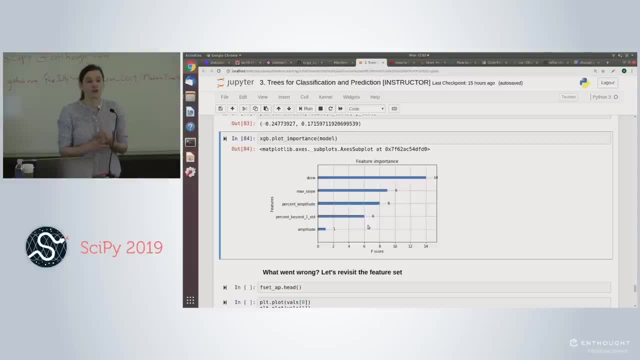 One rebuttal is: even with our eyes we can sort of see something. so we should be able to find some technique that can do that, And also, as I mentioned, the ARIMA can do it. So if we even know, we have a model already. 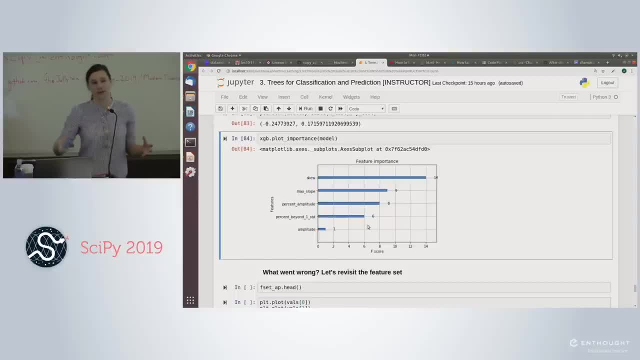 we know we can do it. That's not apparent once you have the log transform, but any, any algorithm worth its salt should not just not work, but it should be able to do things. I did detrend it, yes, So you could say removing the trend. 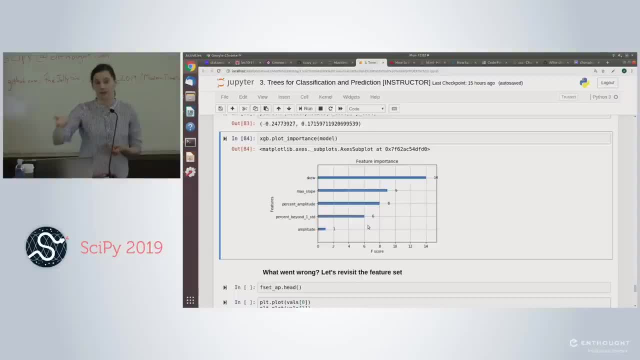 maybe removed all the signal. I think that's one way of framing what he said. So that's I'm saying that could be one possibility if we weren't aware that there is a model that works, And this is especially if you work in fields. 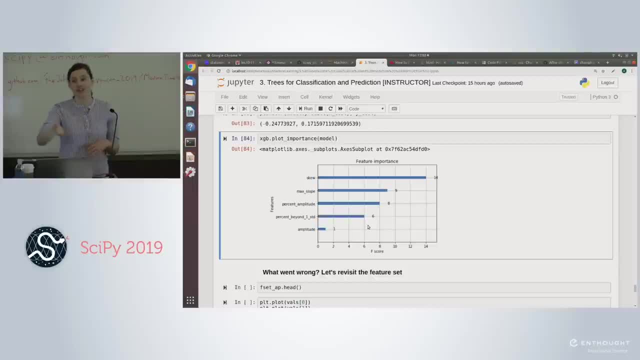 where actually even the best model is pretty bad. You can have these debates all day and sometimes you just don't know right. Is it that there's just no signal left, Or is it that we have a bad model And that, you know, for some people that's their whole job? 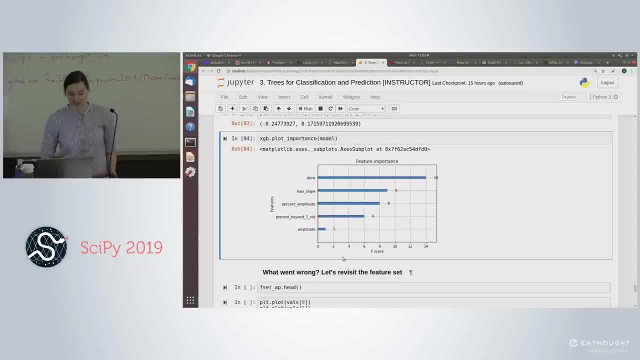 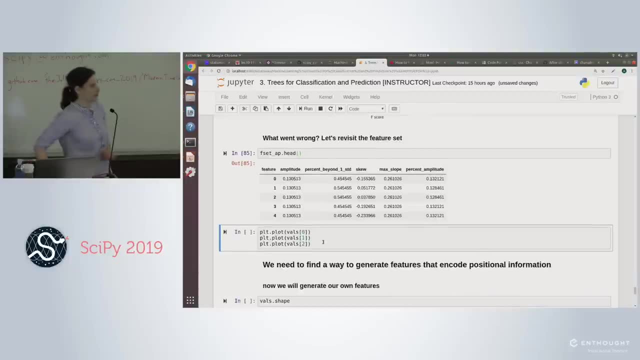 figuring that out or trying to figure that out, And it happens a lot in time series. In this case, though, there actually- let me call your attention to this- So we didn't really look at our feature set in this case once we computed it. 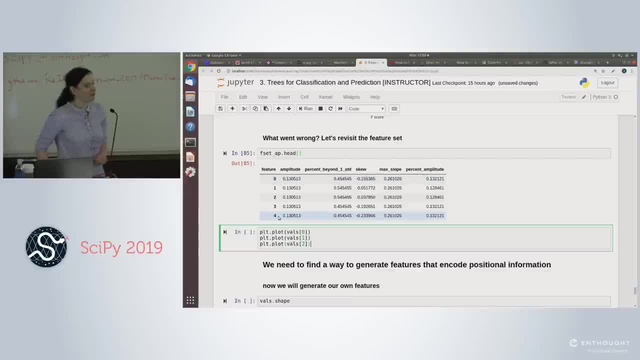 So here's the feature set for my first five data points. And what do you notice? here, A lot of the values are the same, right? So I mean, if this was what I was looking at, rather than say the picture of the time series. 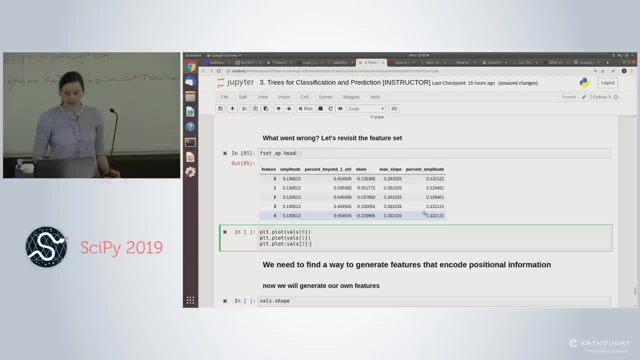 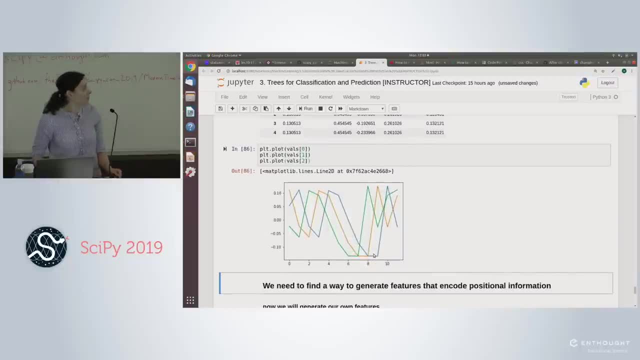 what am I supposed to do with this? The percent amplitude only has two different numbers here. The max slope has the same number throughout. And if we think about why, right, Let's plot three samples of the same data, right, Remember, it's a sliding window. 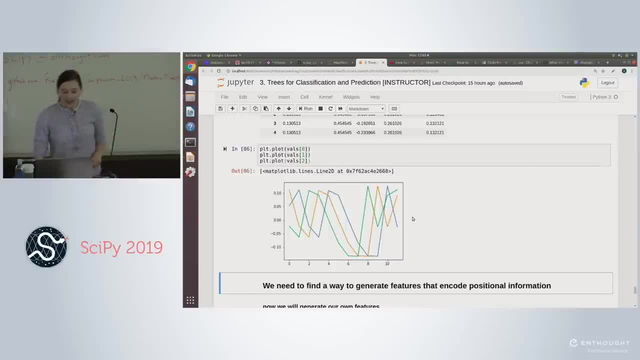 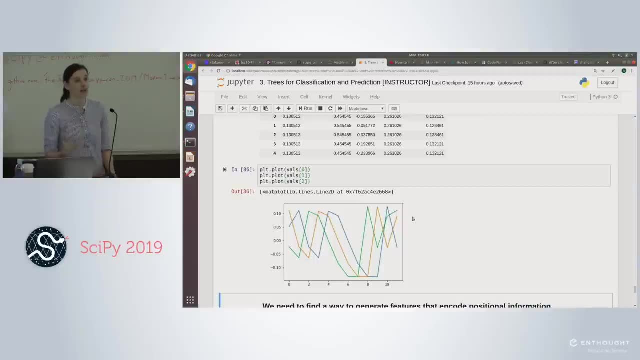 That's. the problem is, we have created these points out of sliding windows, But then the data that I have produced tends to just look at things like the amplitude, the numerical qualities, rather than say positional qualities, right? So if I look with my eye at these three curves, 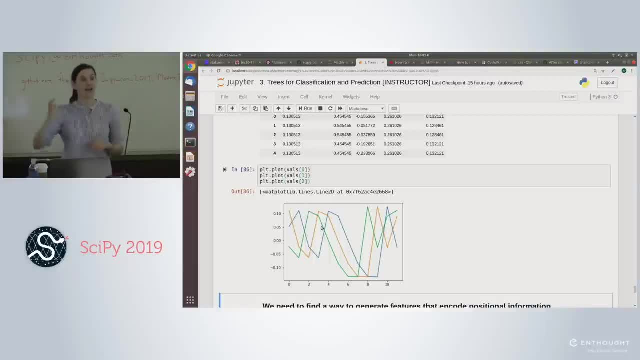 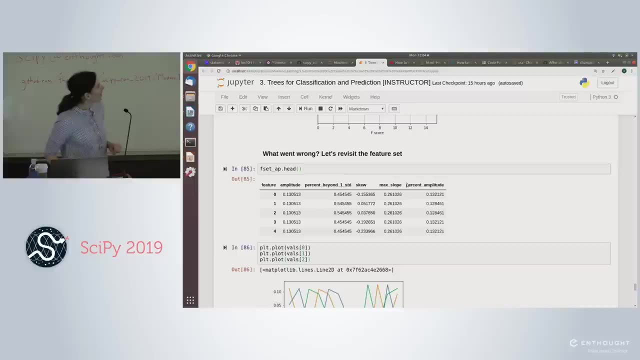 they're different. They're sort of at different phases of the same cycle. So if I can see sort of that phase information, which is positional information, I'm in a great point. But my algorithm right now is not seeing anything. that's sort of. 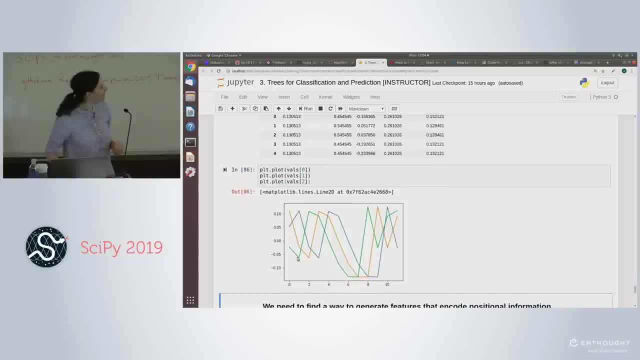 positional information, like telling me where a peak is. It's only seeing information about numbers, right? But if I'm only looking at these time series along this axis, I'm actually not seeing anything that differentiates these three, right? So what I've done here 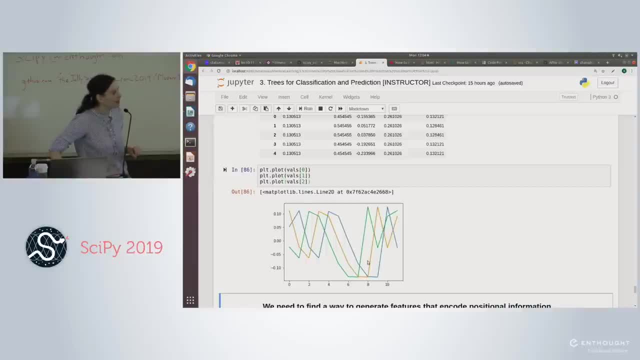 is I only used features that describe sort of the underlying values produced by the process, without providing features that describe the temporal structure right, The structure along this x-axis. That turned out to be reasonably okay for the EEG data because there was already so much variation. 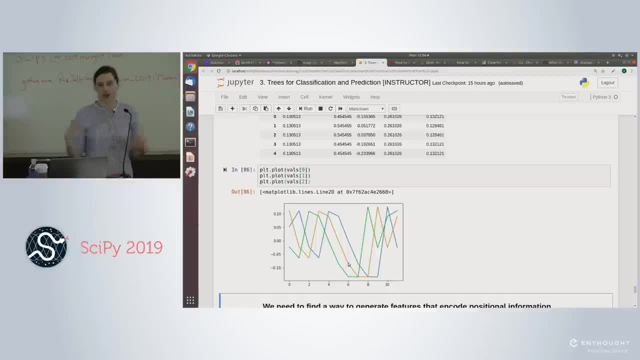 on the numerical axis. We didn't even really need to treat it as a time series right. We could just sort of summarize the values we saw, and that's gonna cut it right. The different samples are not different along their numerical axis. 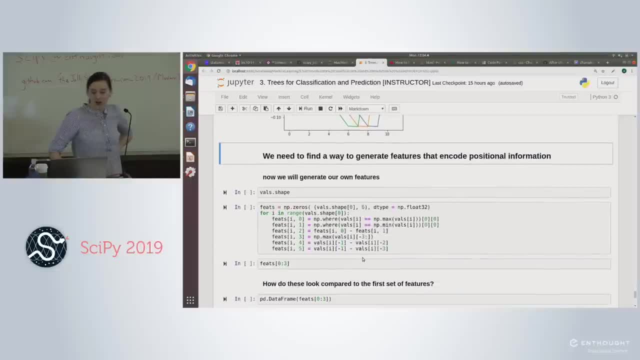 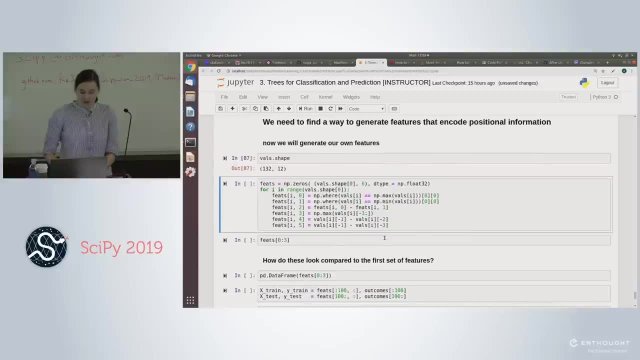 they're different along their positional axis. So let's revisit this and generate features that encode some kind of positional information. So this is just one stab at doing that. Basically, we're gonna generate six features, and what are these features that I generated? 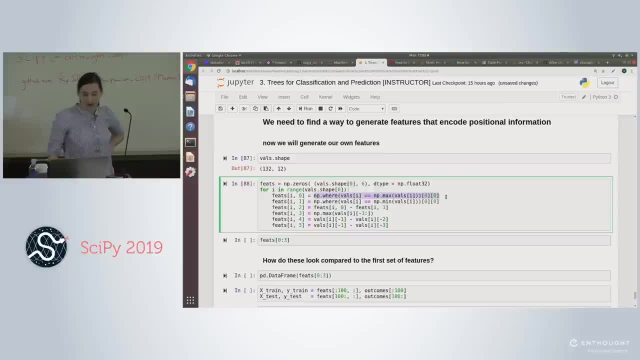 Let's just read them, Okay. so the first one is: npwhere the values is equal to the max. So now I wanna know at which time step does the max occur? My next feature is npwhere values is equal to the min. So now I wanna know at which time step. 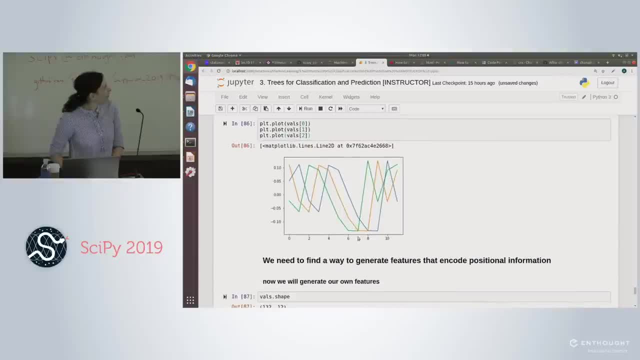 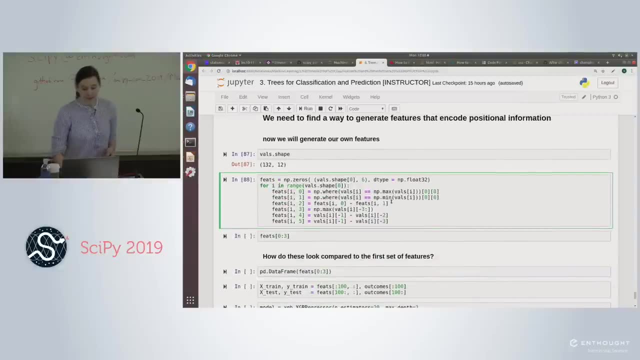 does the minimum occur, right? So now going back here, those two features are gonna give me information about this axis rather than this axis, because that's what I need to differentiate these samples. What have I got here? I've got the distance. 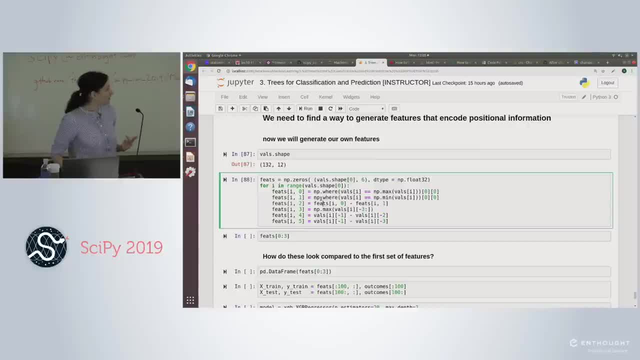 between the min and the max. and notice it's actually more than distance, it's positional right. So this is the distance between the min and the max versus after. this will be positive or negative right. So this is giving me directionality. 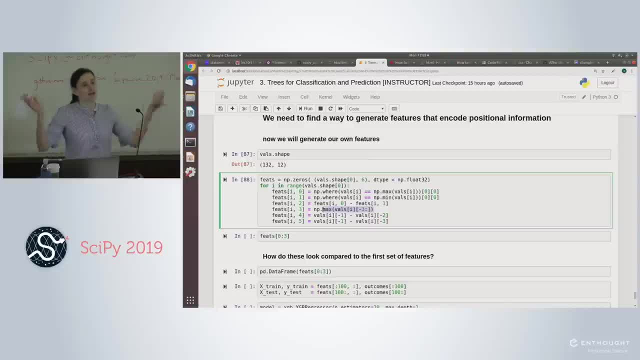 of the relationship between the min and the max. I'm also still gonna keep the max in. This might not be that useful, but I figure what the heck? just in case that matters. And now I'm gonna take. what am I taking here? 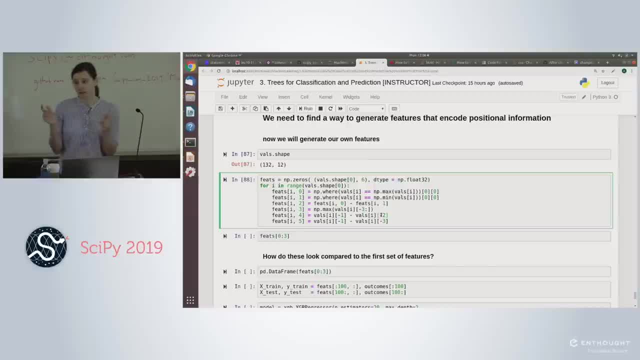 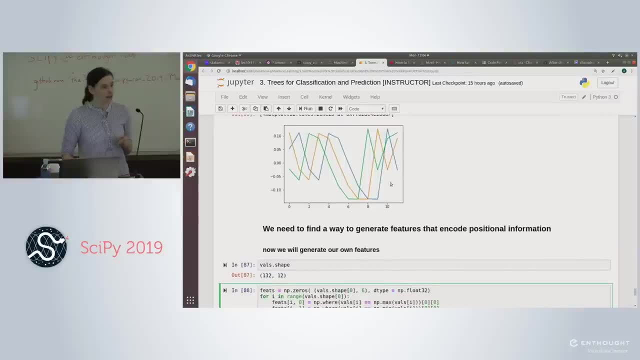 I'm taking the last one minus the next-to-last one. Why am I doing that? Because it seems like if I look at the end, the end last few points are where these three distinguish themselves, Even though they're sort of neighboring sliding windows. 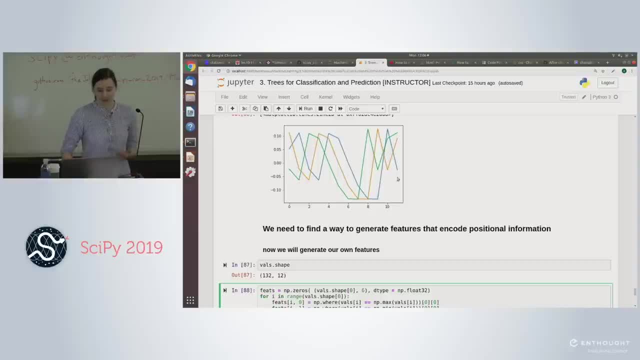 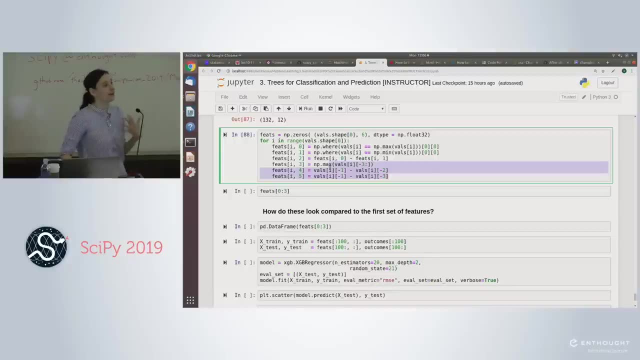 the part where they're most different is at the end. so I'm just saying I want some features to sort of focus on the behavior that occurs here at the end. So that's what I'm doing with these Again. I'm sort of blindly throwing these in. 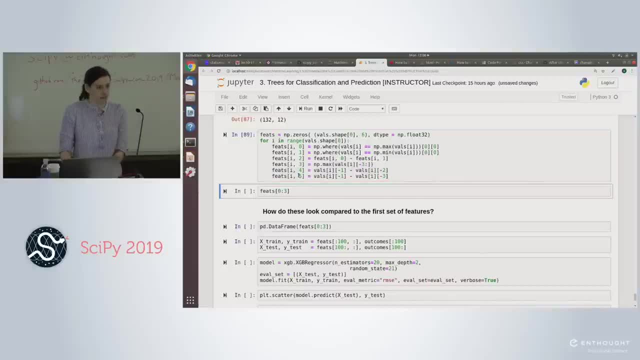 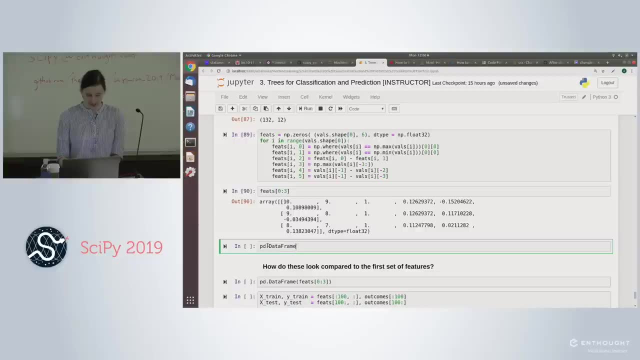 other than this idea that I need to understand this positional relevance, Because if they're not, I'm really in trouble. But these do appear to be at least a little bit different. Actually, can I look at this with a data frame? It just prints a little prettier. 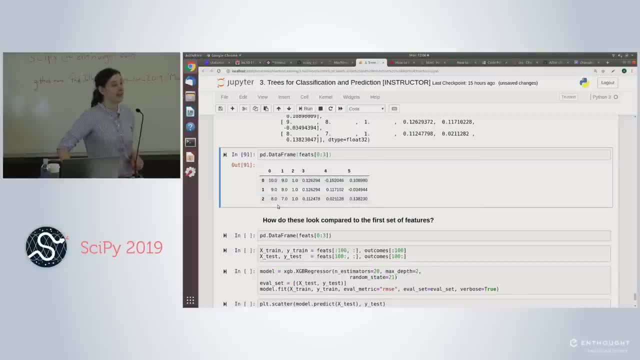 So you know it's not great. I'd have 10,, 9, 8.. But 10,, 9, 8 is a heck of a lot better than 10,, 10,, 10, right? So we at least go from having columns. 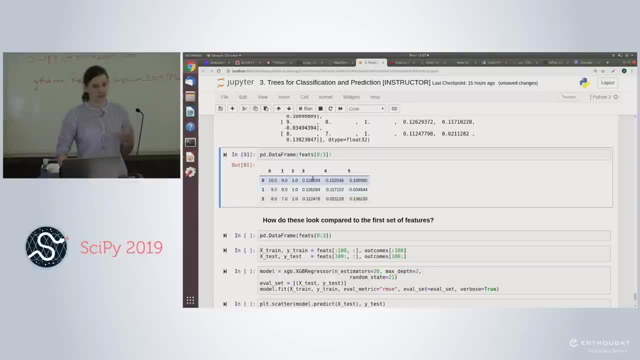 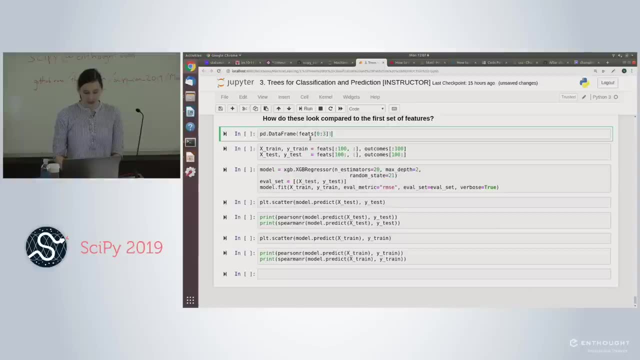 that are just absolutely identical, which are total garbage for our decision tree, into one where there are at least some meaningful differences, and that's what I'm trying to get at. Okay, So here we do that, So we're going to divide it up again. 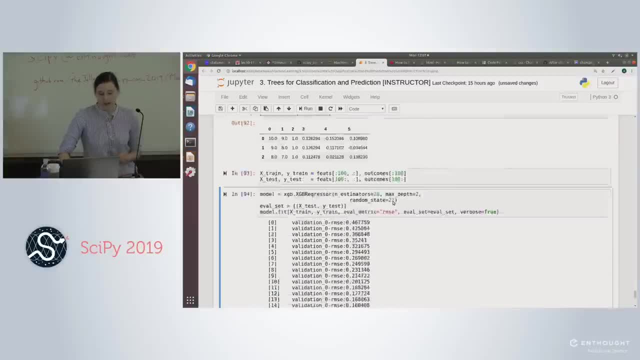 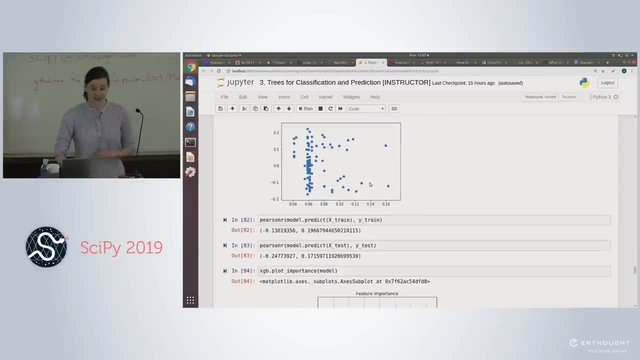 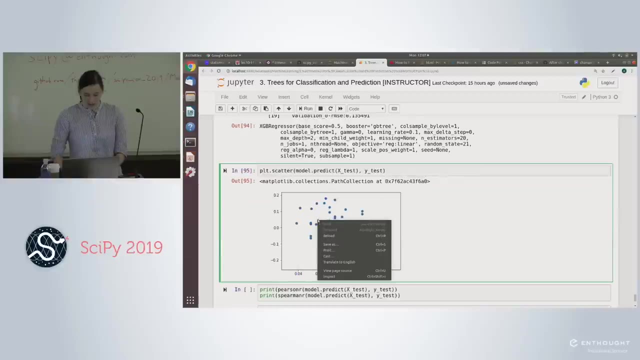 Let's fit this again. Notice here we've still got. our RMSE is about the same: .135,. what was it up here? Where is it .138.. So I'm not doing that much better on my RMSE front. Let's do a scatterplot though. 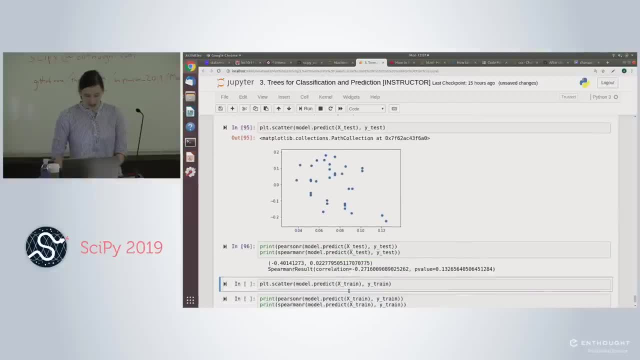 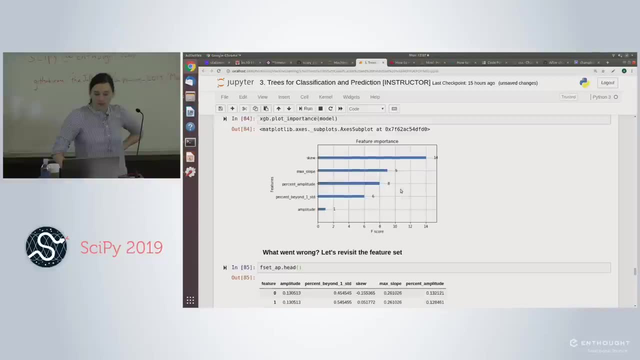 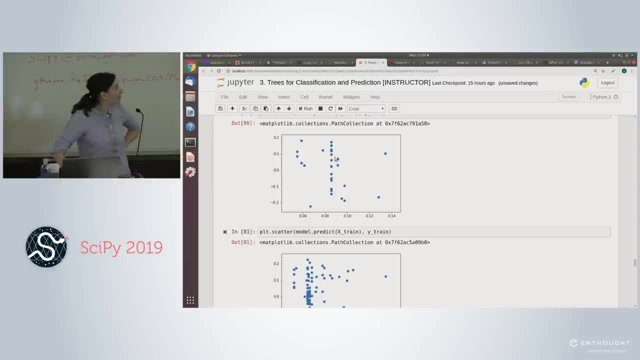 So here's my test And let's look at the correlation between the two tests. Okay, So how do I digest this? So this is my test plot. Let's remember what the first test plot looked like, with the total garbage features. I mean, clearly this plot is a lot better, right? 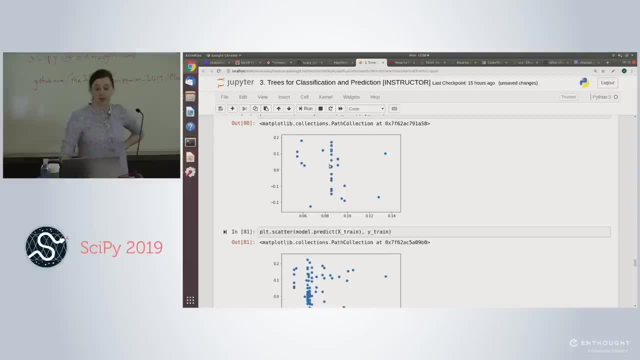 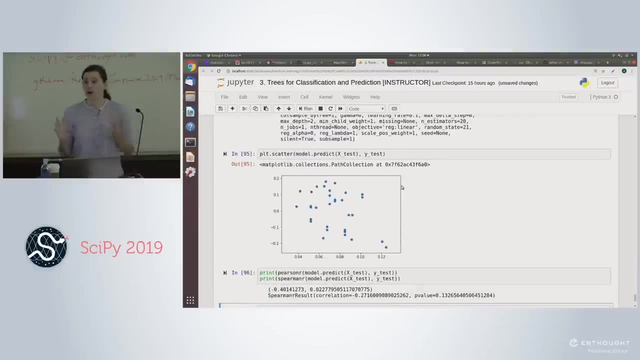 So our old plot with the garbage features. it's almost like they're just on independent axes. It's almost like there's no relationship at all between our prediction and our true value Here. that's not true at all. right, So I think we're seeing a case again. 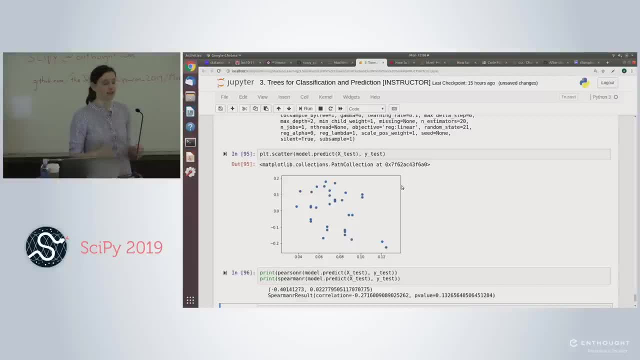 where RMSE won't tell you the full story. In general, with your time series models, no particular metric is going to get it right all the time. You want to take a more holistic view And it will also depend on your applications, right? 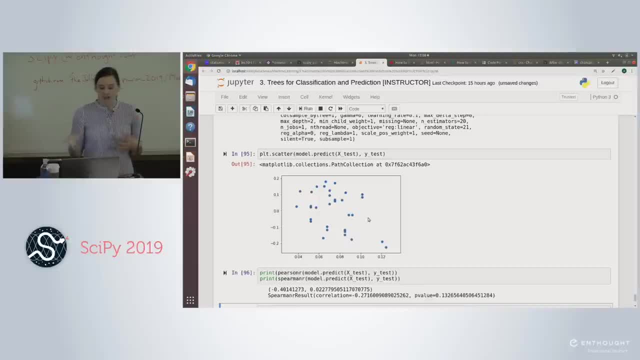 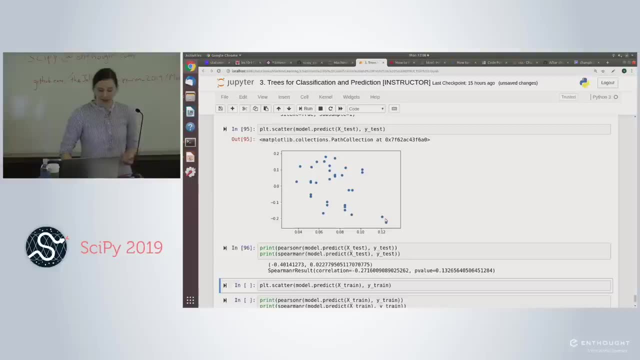 So RMSE gives me the same thing for a model that has almost no relationship to my outcome, versus one that does right. if I go by plotting- And I would also point out here, especially if you ignore these two outlier points, then you seem to have even more of a relationship, right. 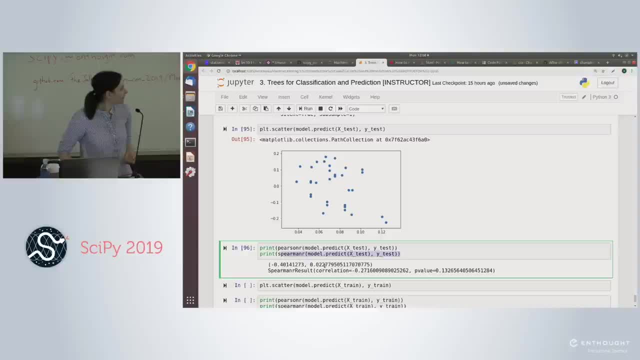 So if I do my Pearson R versus my Spearman R, my Spearman R, to get rid of a bit of the outliers, the correlation is a little bit less negative, although still negative, right. So this model still needs work, but at least now we're bringing some sense to the data. 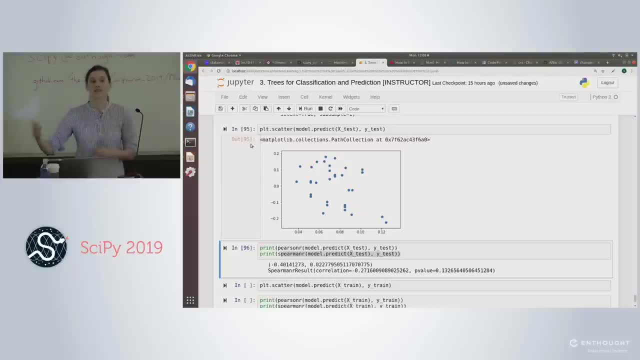 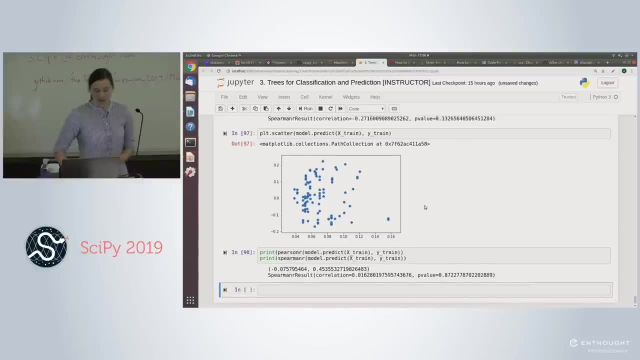 versus before, because our inputs were identical for different outcomes. There was just no way to get started for the algorithm, And if we do a scatterplot for the training, we see that we do even better right. So again, if we ignore that outlier in particular, 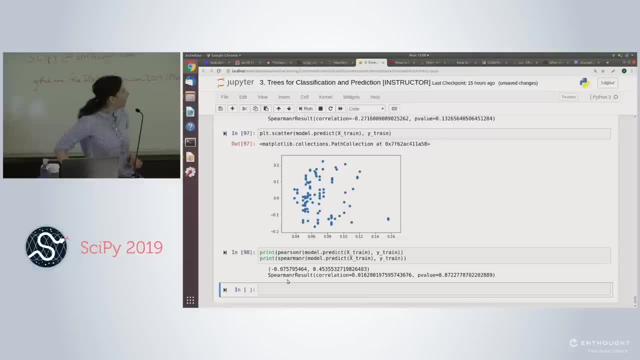 this begins to look like something of a relationship And actually, if we ignore the outlier, we might even finally be into the realm of positive correlation. Okay, So not super impressive results, because again we're dealing with a small data set. 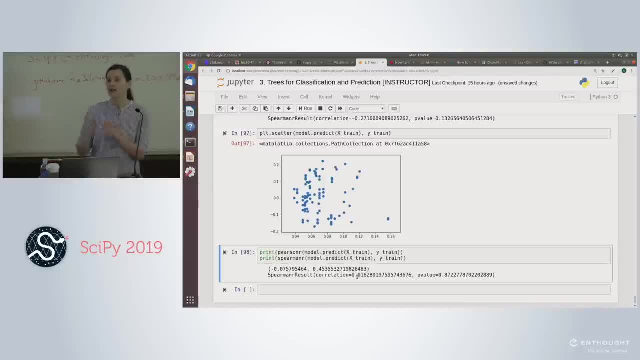 So actually, this exercise is here to show you a few things. right, We saw how we can take one time series and turn it into many sliding windows to produce enough separate samples to fit an algorithm safe for prediction. But on the other hand, 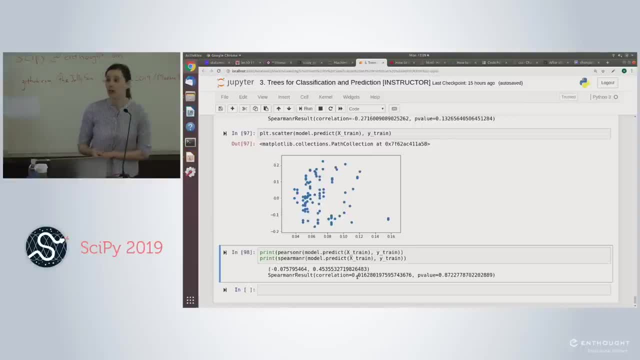 I think what we see here is A. it can be very easy to generate the wrong feature set and even a nonsense feature set, which is a reason you should be careful about using packages that are automated for generation to generation. It could be that your features 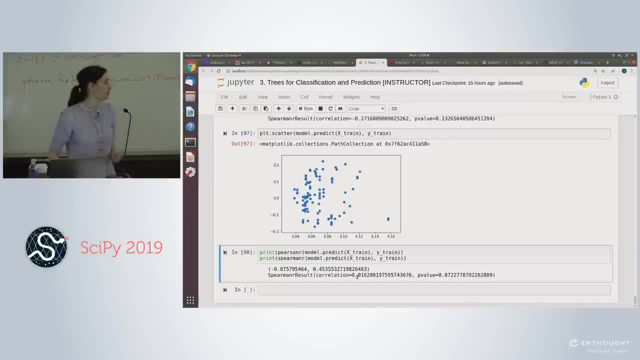 are not in any way meaningfully distinguishing between, say, neighboring time series, which is something you want to do, But you also want to remember that, especially for low data situations, machine learning is really not the way to go. So if you're doing some sort of forecasting, 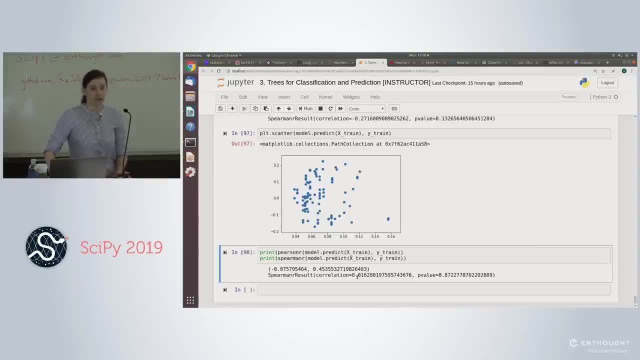 that involves low quantities of data. that's not really what machine learning is built for- right versus something like the ARIMA model is. So part of using machine learning for time series is knowing when to use it judiciously and when you just don't have enough data to justify it. 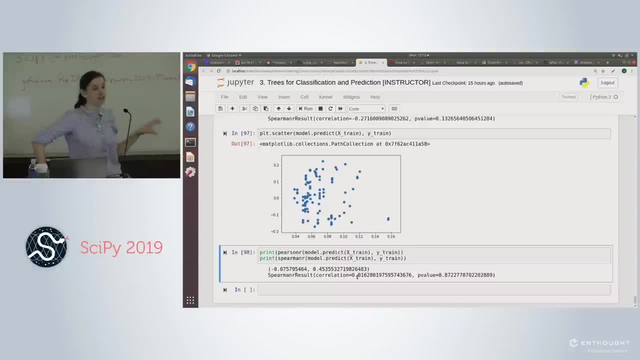 So all of these techniques should really be used on much, much larger data sets, and if you use them on the larger data sets, that's where you're going to see some really excellent performance, And the larger your data set, the more likely that machine learning is the way to go. 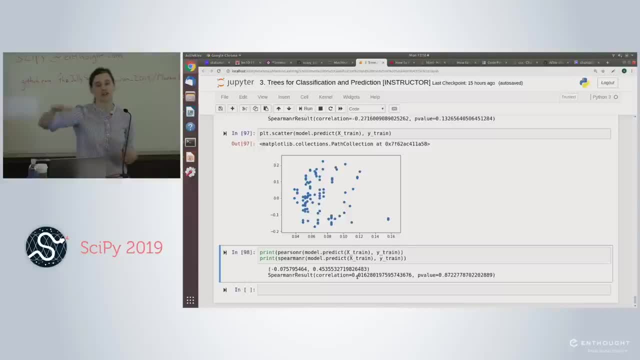 rather than the traditional statistical models because, as I mentioned, those do well on small data sets and then they sort of max out. Your estimation of your parameters can only get so good when you don't have that many, versus when you have many, many parameters. 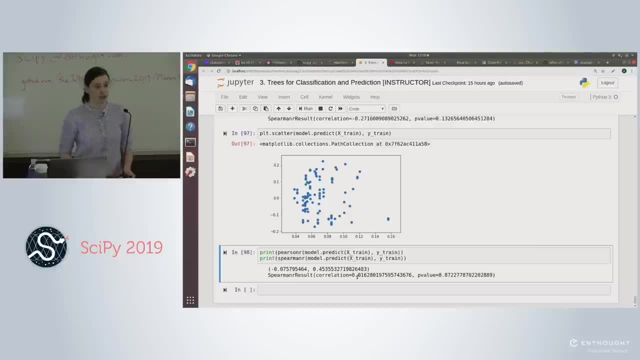 and a more complex model and you can see that, for example, in Kaggle competitions, in industry research papers, in academic modeling, competitions of time series forecasting. XGBoost is performing very well on large volume data. Okay, so any questions about machine learning. 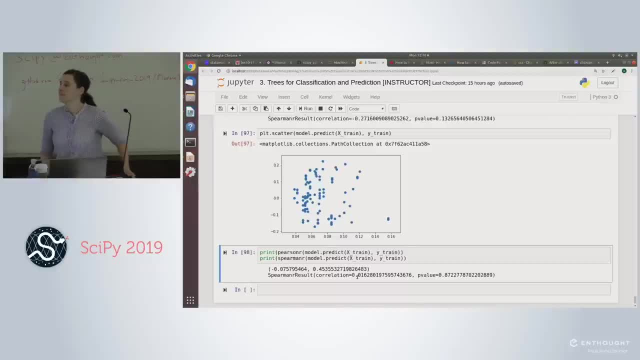 and time series. Okay, so can I look at your computer while we take a break, Because we're about to take a break. Okay, great, So we're going to take a break. Let's reconvene at 11.20.. 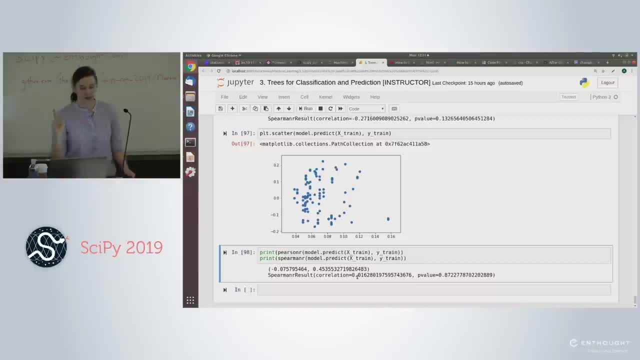 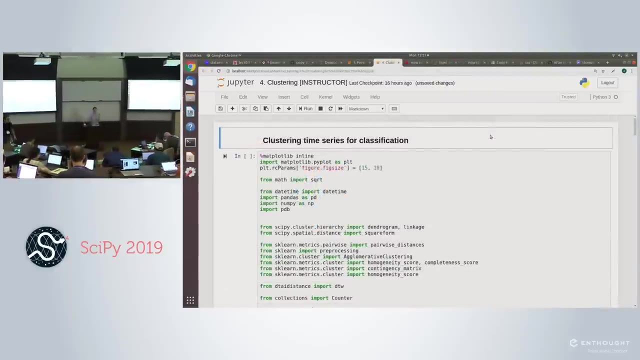 It's 11.11 now and we will cover deep learning as our last component. So we have, we're going to cover two more notebooks. I do want to briefly cover time series forecasting, and then I'm going to go back and talk a little bit about. 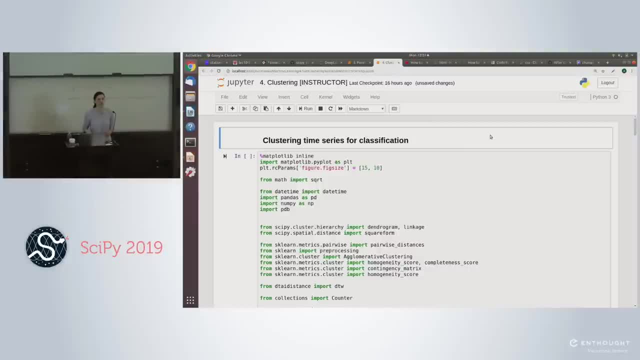 deep clustering. So I'm going to fly through this and then we'll get to the deep learning example. There are two deep learning examples in the notebooks, one on electricity forecasting and one on stock forecasting. The stock forecasting one is sort of supposed to be like a. 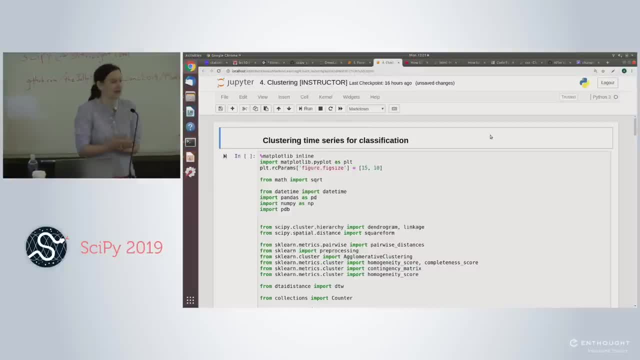 you know, do it on your own after the tutorial thing. That was because I wanted you to have a TensorFlow example as well as a MixNet example, just because I like those two libraries. So that's just the background. But let's talk about clustering. 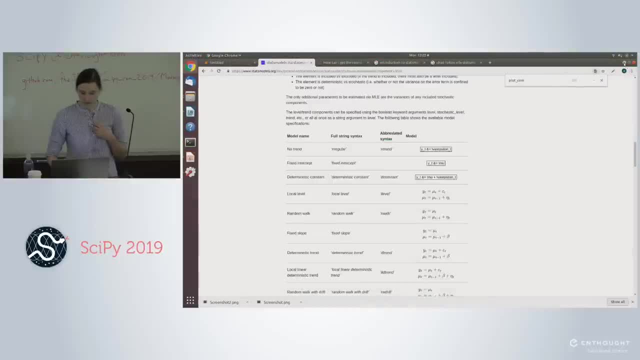 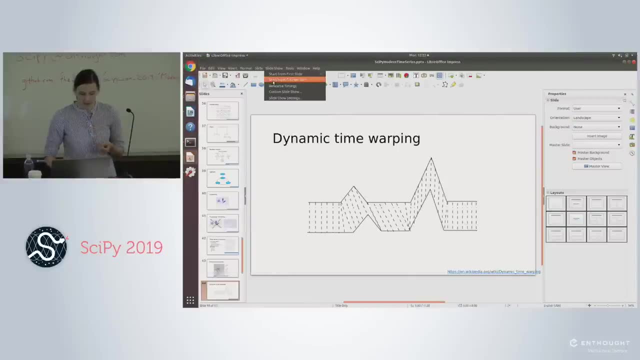 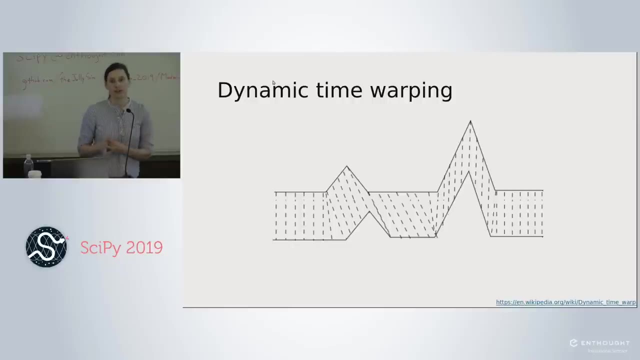 Let me just again briefly remind you of the dynamic time warping, just because that's the thing I want to cover. Okay, So what we just did? we looked at how we generate features for a time series. what can go wrong there, what can go right there. 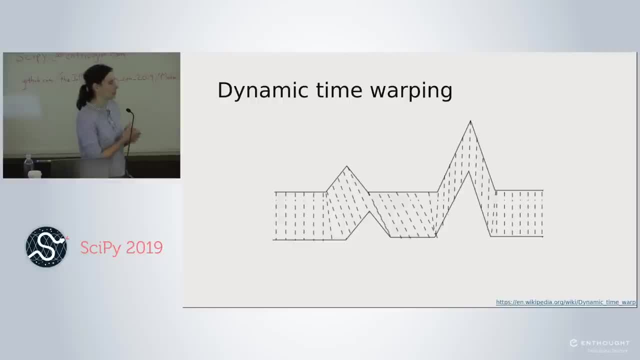 why we might not want to do it sort of blindly, why we might want to put some thought into it. We learned that time warping can be really time consuming. We learned how to extract many samples from a machine learning perspective- samples rather than just one time series. 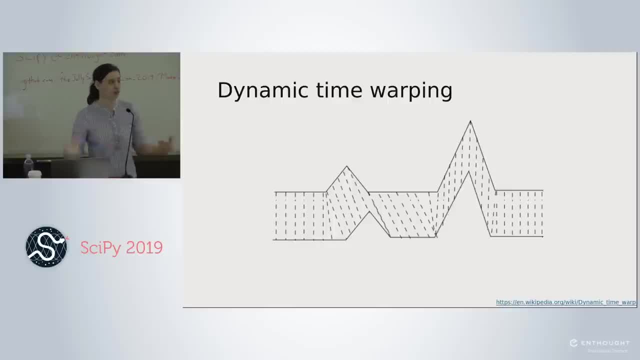 to accommodate the nature of how machine learning works and how it thinks in terms of samples rather than in terms of time series. So now, briefly, we're going to look at clustering and mainly I want to show you the value of dynamic time warping. So again, as a reminder, 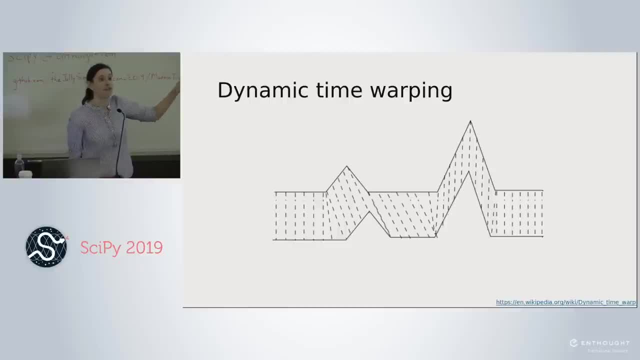 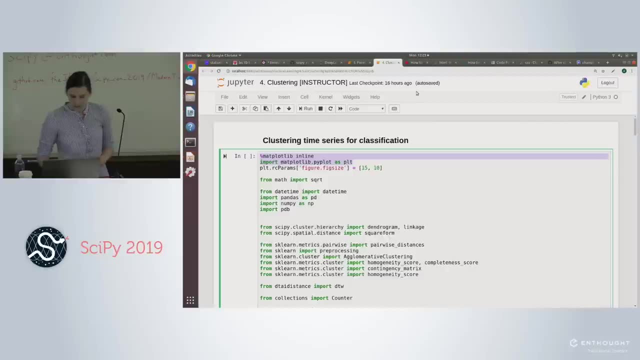 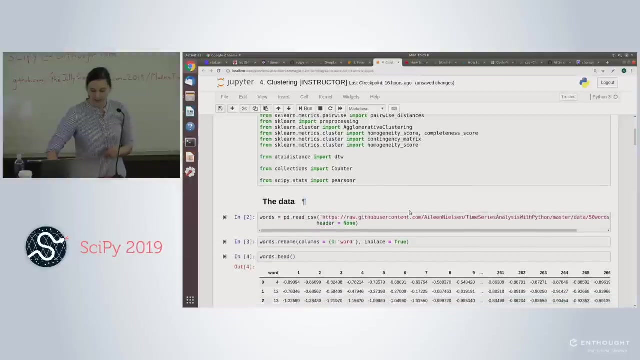 this is one way to map time series to one another in a way that looks like this. So we're going to compare those briefly and see how they work. Okay, So in this case, what we are looking at this is actually from the other tutorial. 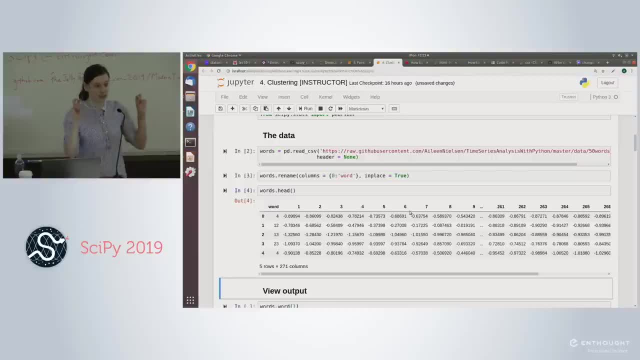 I gave a few years ago. This is sort of a test subset of what are some word projections. This is based off a paper from, I think, the 1990s or early aughts, before we had all this lovely deep learning and where people were thinking: 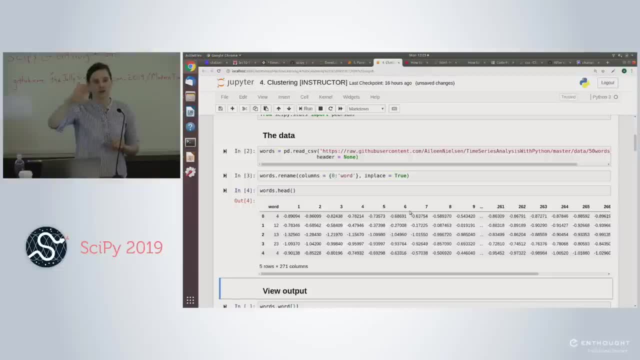 is there a way to sort of identify which words within the documents are the same And what they came up with is? let's look at a word in handwriting. we're looking at sort of historical stuff. let's project that onto a 1D axis. 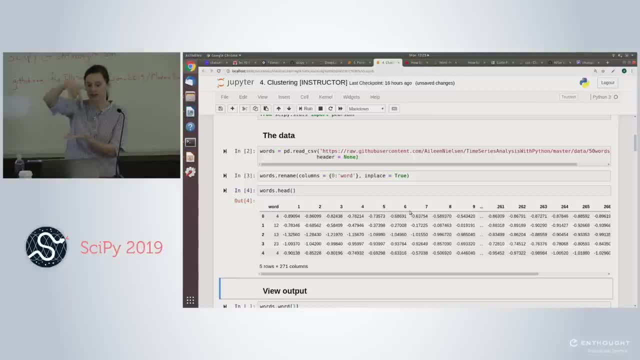 so sort of all the letters on the word. we just do a bin count of the density, convert that to a 1D axis. that is actually an ordered, evenly spaced axis, so it's like a temporal axis, even though it's not per se time. 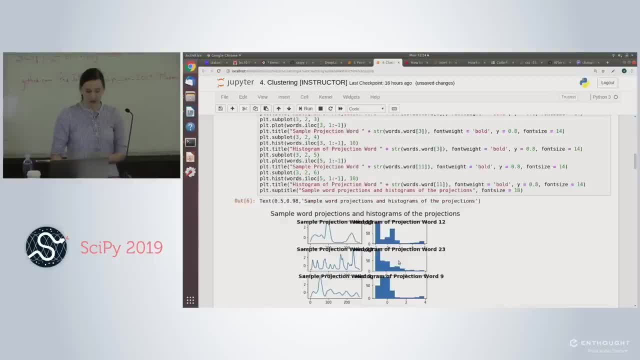 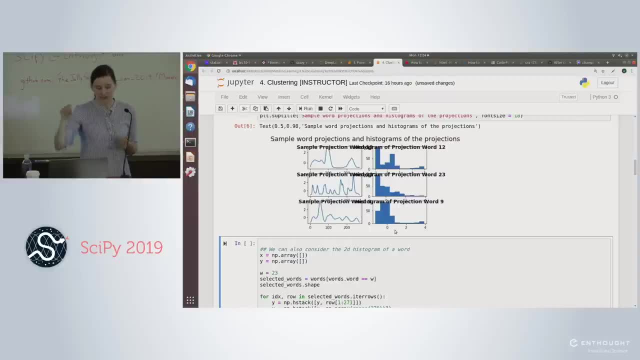 So if we do that, they basically boiled it down to 7 data points per word- and if we looked at what some of the words looked like- and they don't tell us what word in the classification corresponds to certain handwriting- but we can see there are sort of distinctive shapes. 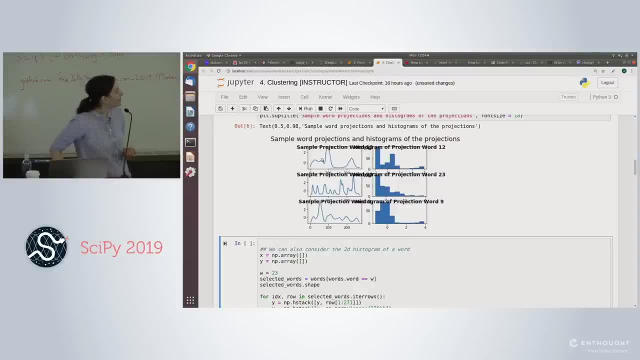 different numbers of peaks, different locations of the peaks, and I also just wanted to point out: sometimes you can just have a different way of summarizing the data and you almost create a new time series. So this on the left is sort of the time series. 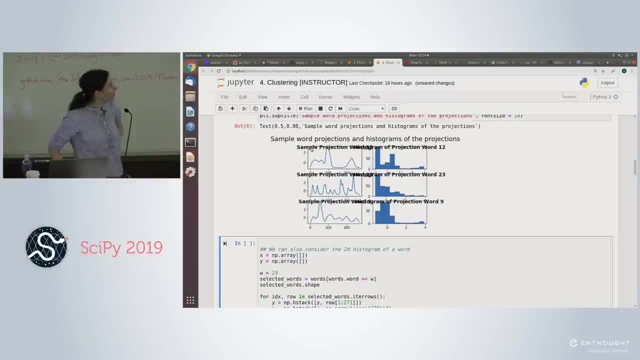 of the projection of the word. and then, on the right, I took a histogram and basically I took this, summarized it numerically, but you can even think of a histogram as a time series in the sense of your x-axis is again evenly spaced. 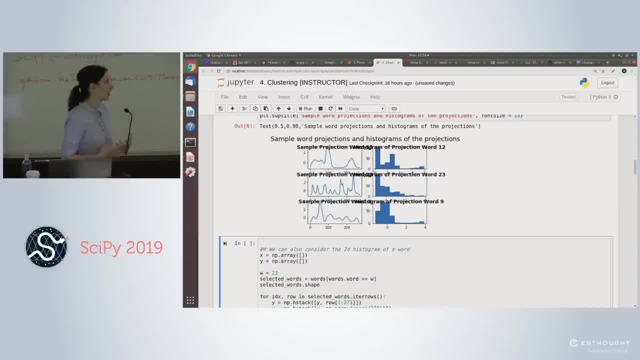 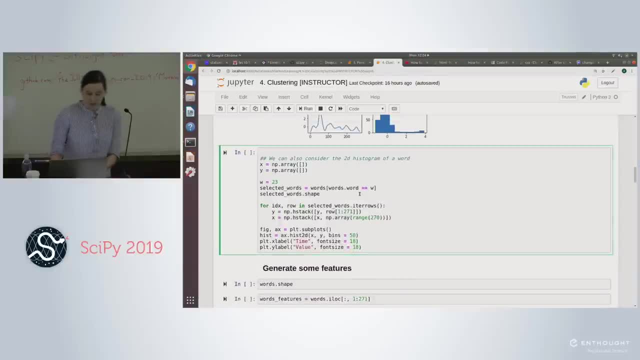 So once you start realizing that time series, temporal axis, can be a way to think about shapes of curves more generally, you can think of all sorts of ways to generate features. One really nice way to sort of visualize time series when you want to see many examples. 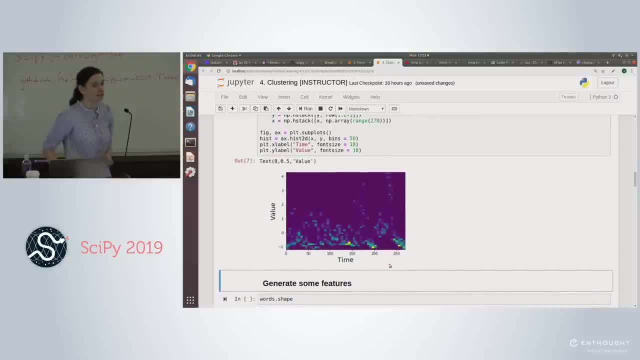 of the same sort of class of a time series is. you can think about things like producing a 2D histogram. So we're looking at the word 23,. so let's see, I believe this is word 23,. yeah, this is word 23 here. 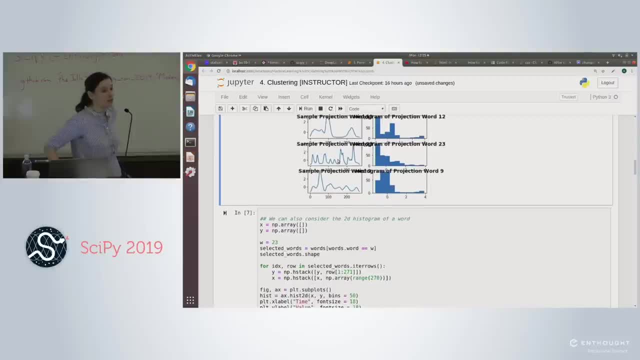 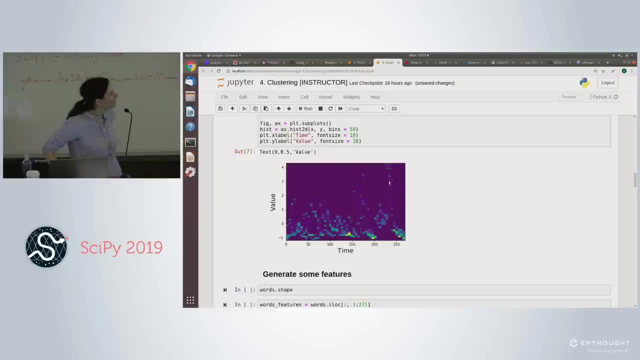 but that's just one example, right? What if we want to make sure that the features we see here are more general? We can do something like a 2D histogram and we see: oh yeah, it looks like there are sort of two peaks here. 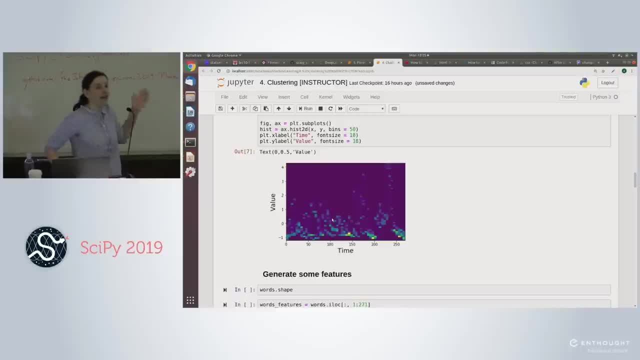 although the location is not set that specifically, and a couple of peaks going on here- And this is actually a good example of part of the reason we can't just see the raw time series as the inputs, because things like peaks, their location jumps around. 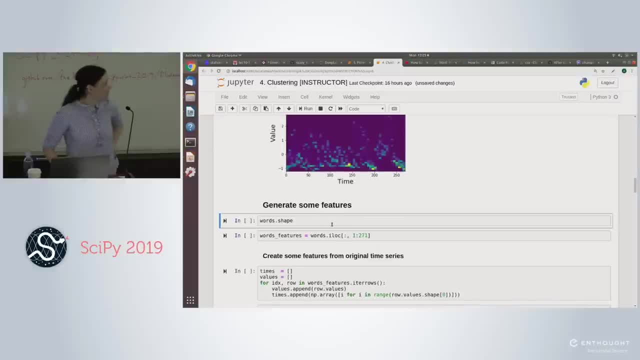 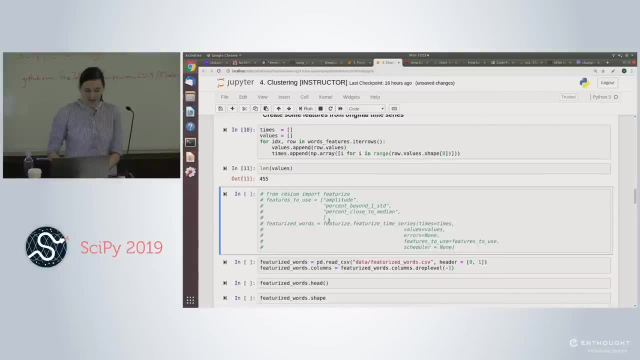 whereas if we were to just feed it in, that behavior won't really be documented. So we're going to just generate some features again off of what we've seen briefly. So again I used Cesium, and again this is sort of time consuming. 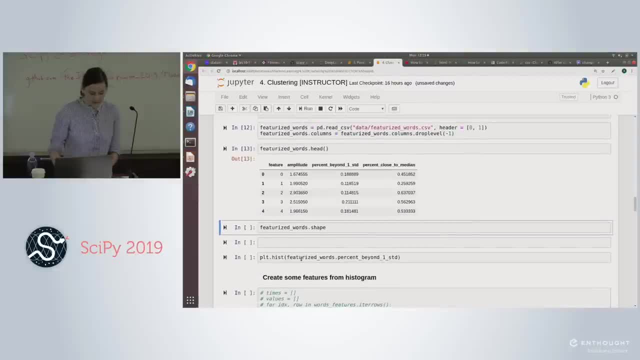 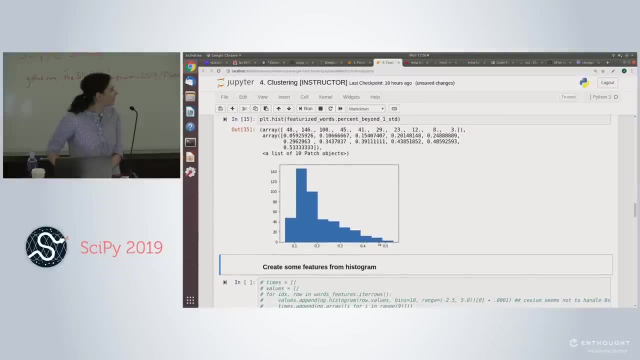 so I would recommend just reading it off the CSV. You could on your own time possibly consider generating them, but it can be quite time consuming And again we sort of look at a histogram to get a sense of what these features look like. 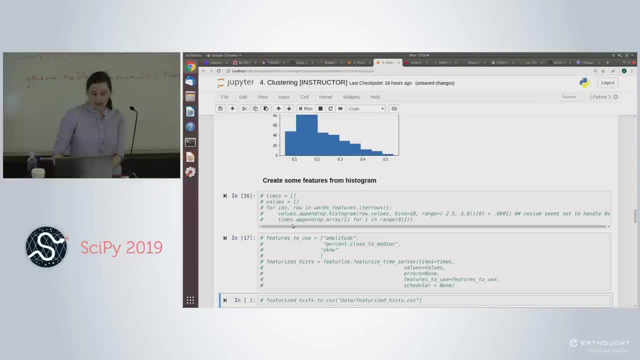 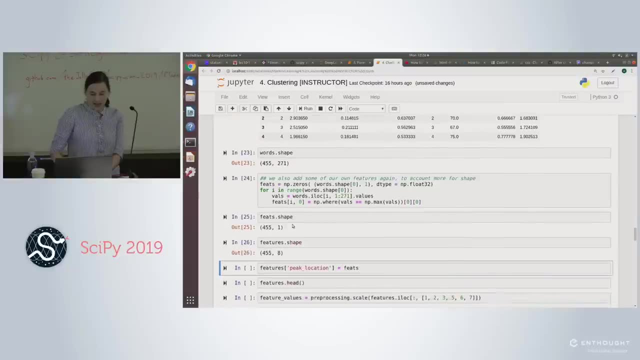 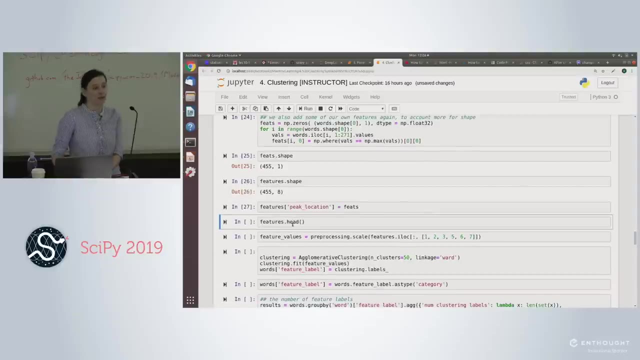 We at least want to make sure we've got some sort of spread. We're going to generate some features for the histogram itself as well, treating that as a sort of directional time series. We're also going to find the location of the max value. 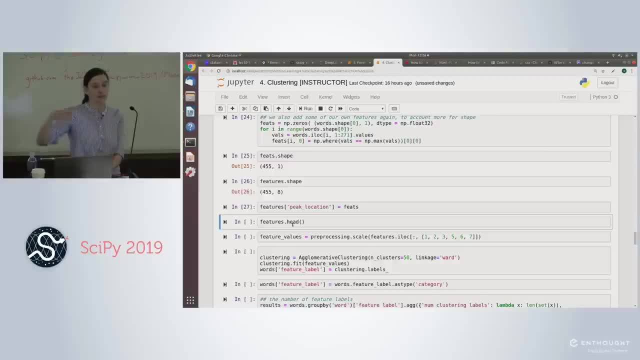 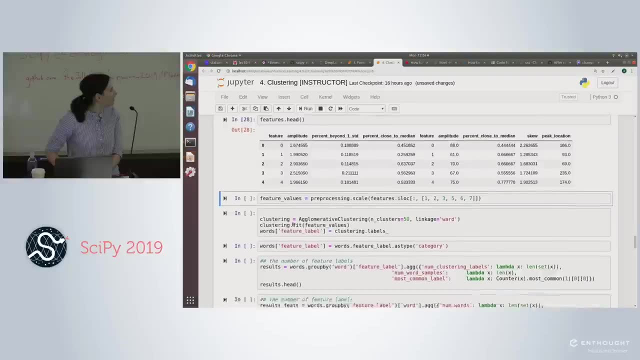 so we sort of learned our lesson from that last example we did with the air passengers. Let's put in some sort of positional information that we found ourselves in this case where the max is. And then, finally, for clustering, we want to make sure all the features 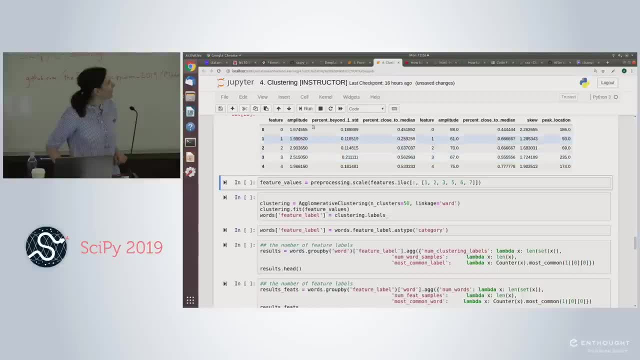 sort of count, equally right. So we want to make sure that it's not like amplitude just swaps out percent beyond one standard, deep right. So what's a quick way to do this? This is not time series specific, but in general we want to preprocess our features. 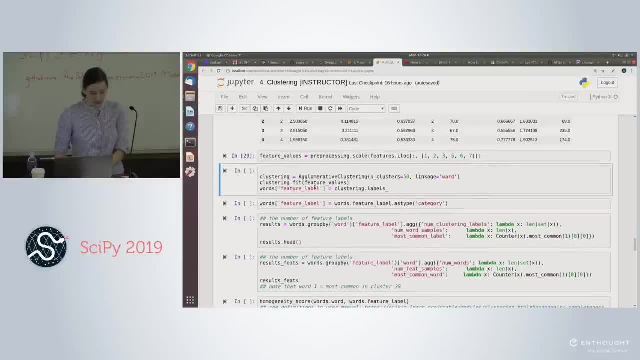 And then we're going to cluster them, and in this case I'm using hierarchical clustering. Why am I doing that? Because I don't really have a good sense of what my distribution looks like, so I don't want to use something like k-means. 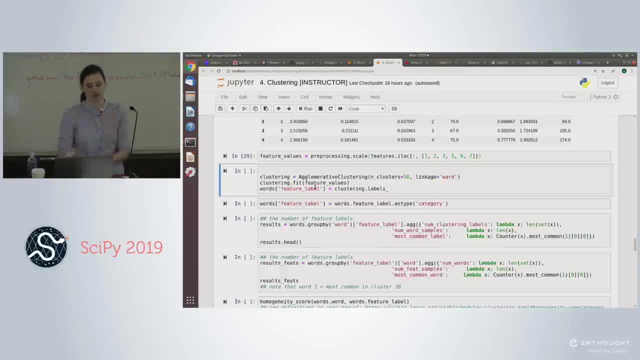 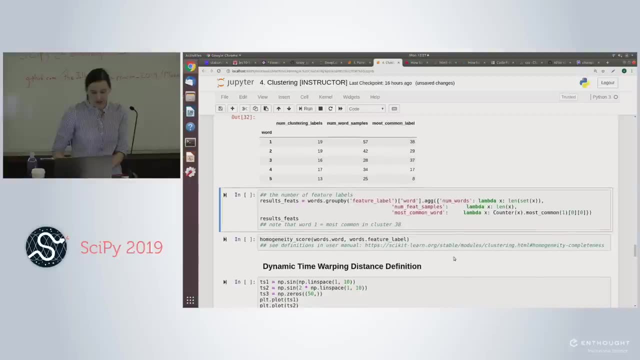 where I'm assuming that I necessarily have these various variants and that I have these sort of well-shaped spheres. I don't want to assume anything like that at all. So if I do that, what I'm going to see- this is just sort of the result of my clustering. 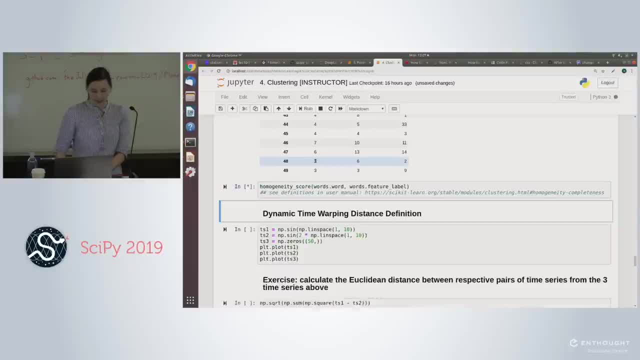 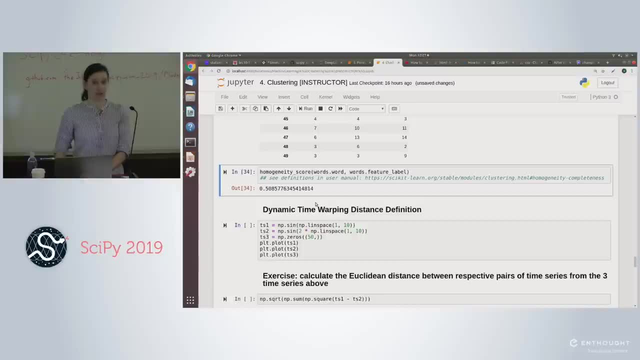 it looks pretty messy, Like I'm not really finding a good pattern, and one measure of that is like the homogeneity score, right. So like how homogeneous are any of the clusters I made in terms of the original class labels? The punchline is not very good, right. 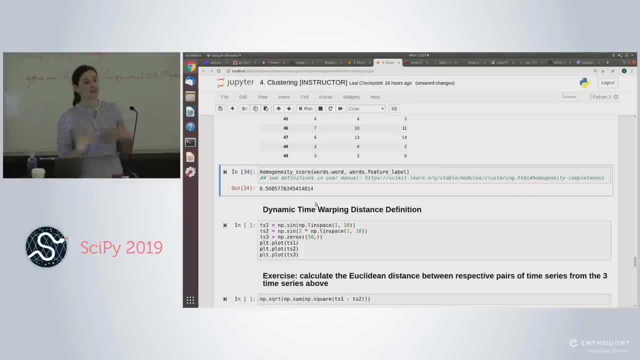 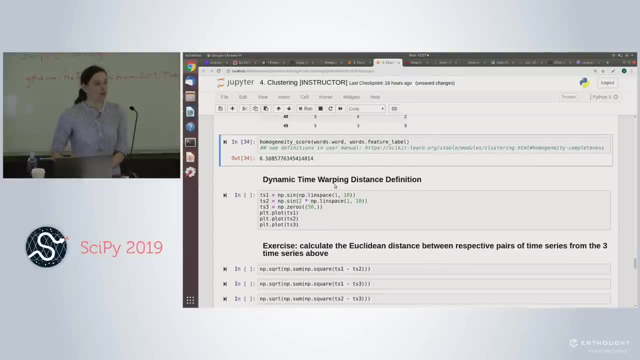 So the clustering I do is not very good and I don't want to use any of the features of my time series. at least for these features not great. Now I could put in more work and try to find good features, or I could remember. 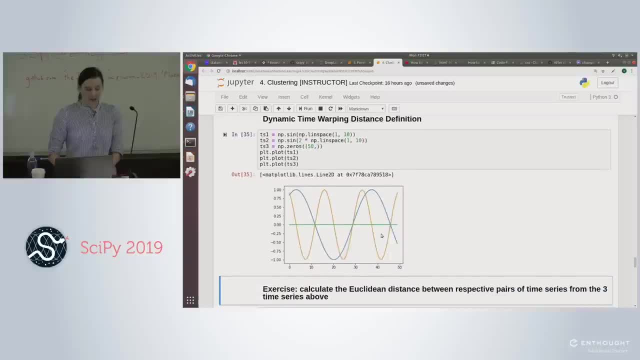 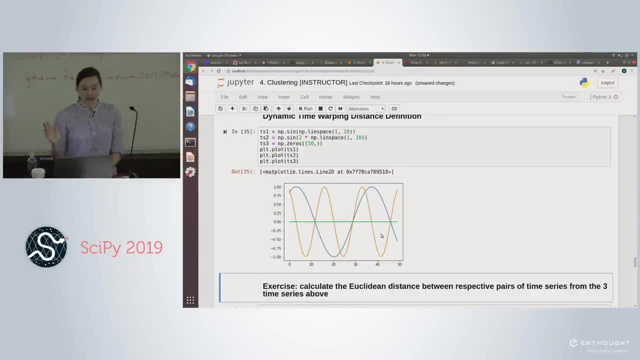 oh wait, dynamic time warping. I heard about this magical distance metric. that's really fantastic. let me check that out, right? So let's first look at a toy example. Here's my toy example, where I proved to you that we would rather match. 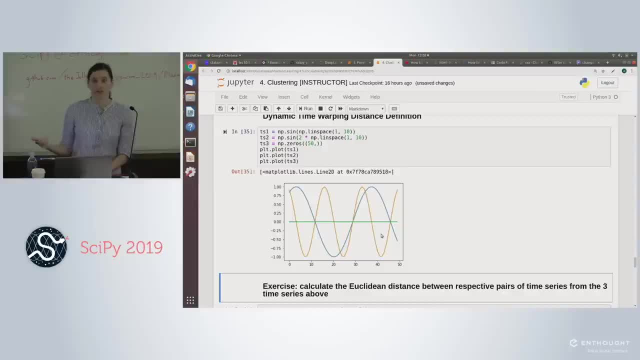 the two sine curves, even if they have sort of different frequencies. we'd rather think of them as being more similar to each other rather than thinking that either is sort of more similar to a flat line, right? So if I were going to group these, 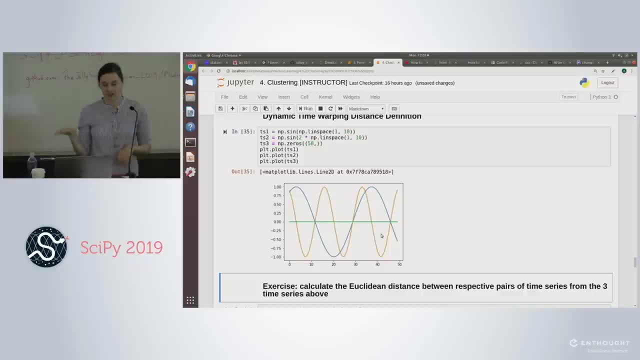 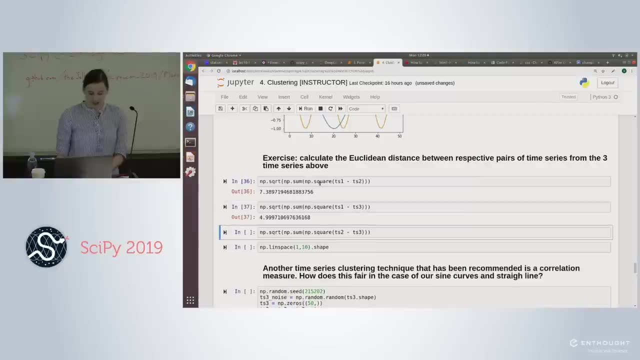 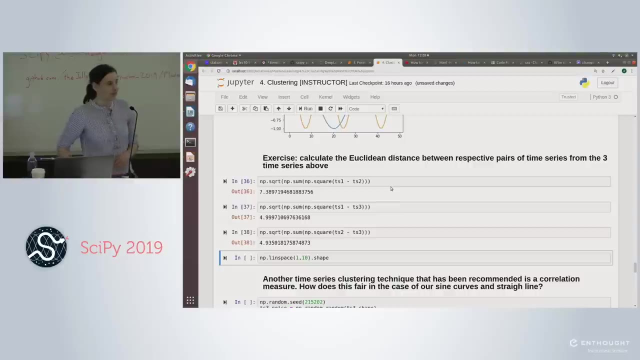 say into only two groups, we'd probably put the two sine curves together, right? There's more fundamental processing common for those two relative to just the flat line. So, as an exercise, if we do calculate these, both of the sine curves end up having a shorter distance. 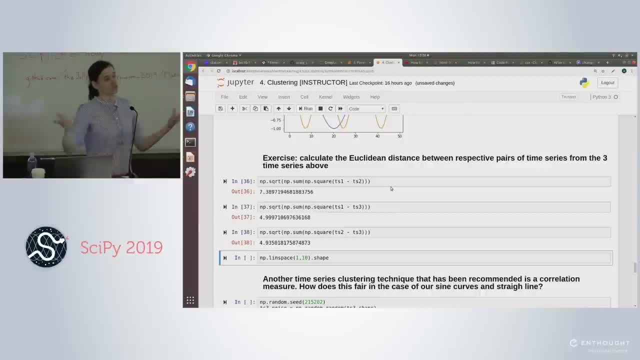 to the flat line than they do to each other. You know there's no magic behind it, that's just sum of squares and take the square root. that's the behavior you're going to get- Super undesirable behavior. So this has two components that concern me. 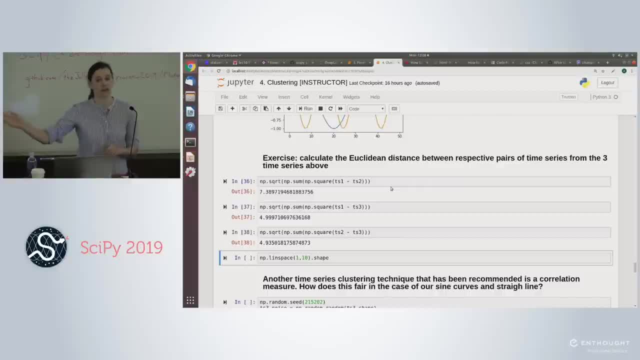 Firstly, it's not super computationally efficient. anyway, to do Euclidean distance right, You still need to go through all the data points. it's not like it's really fast. It's almost always true that you wouldn't want to use Euclidean distance. 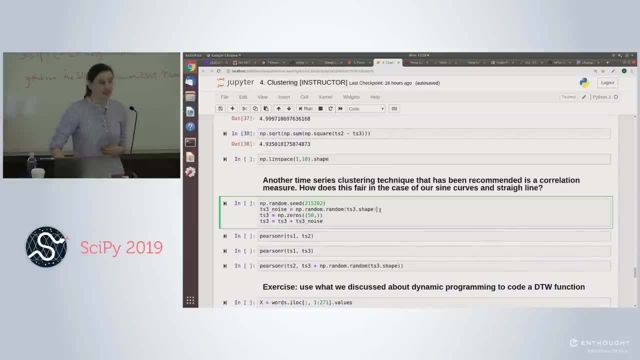 Another measure that has been recommended is a correlation measure, right? Like? how sort of similar are they? How correlated are they? That seems like maybe it could do better than Euclidean distance, So we're going to do the same thing In this case. you see that. 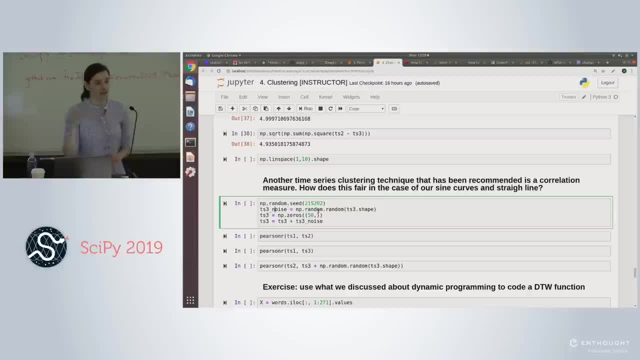 I am going to add a little bit of random noise to my time series 3, which is the flat line, just so that I don't have an undefined correlation right. So I'm going to use the same variance. That measure will just come back as a NaN. 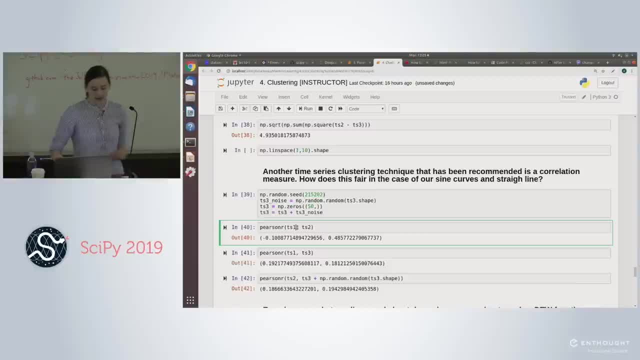 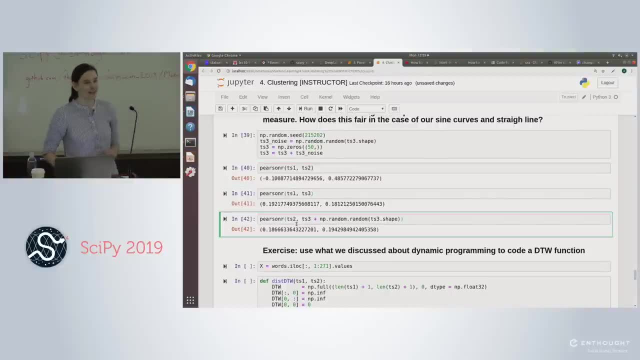 So let's do the same thing. Let's look at the correlation. So huh, interesting. Again, the sine curves are sort of negatively correlated with each other, versus they both have a positive correlation with the flat line. So again, if I use correlation, 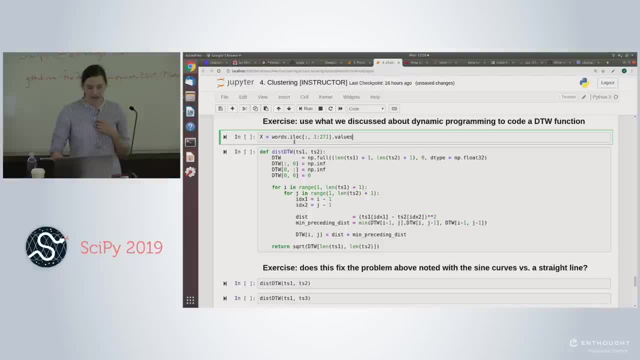 A- it's not a super efficient metric anyway, and B- it doesn't do an especially good job relative to my desired behavior. So what I would recommend is dynamic time warping. Here is one simple implementation. You can definitely code this on your own. 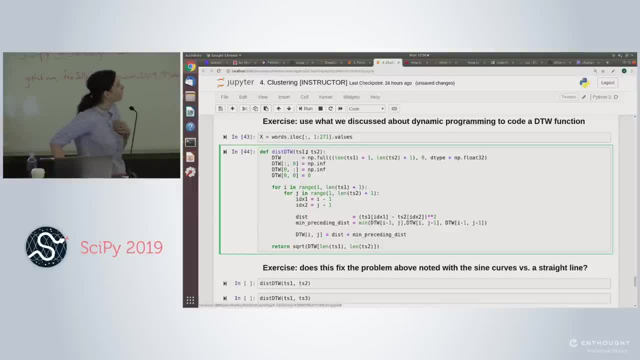 so I would definitely recommend this if you're ever going to work with dynamic time warping, so that you feel more comfortable with the definition. The meat of it is here, right, So I'm using this. This is the dynamic programming aspect. 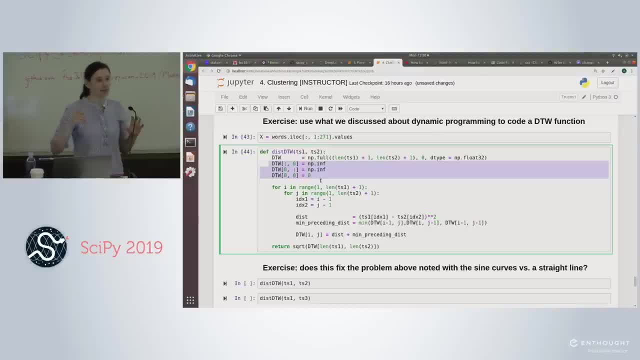 is, I have a matrix because basically, what I'm trying to do is for each set of points, right for going up to the i-th point on one time series and the j-th on another, to figure out what's the way to align them. 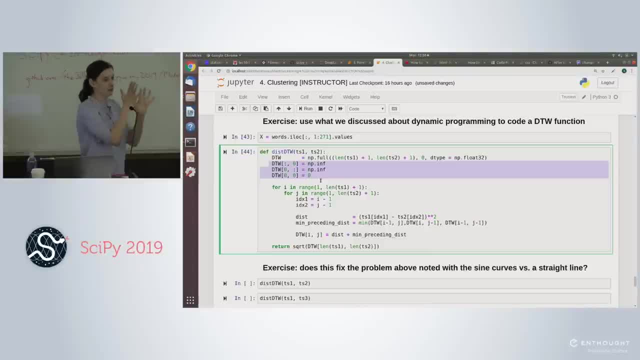 that results in the shortest difference in their values right, that best aligns their difference. So I do that by iterating. I start at the beginning of time series one and the beginning of time series two and then I calculate the distance between them. 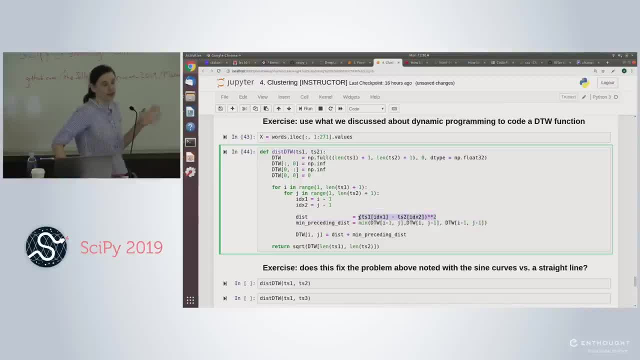 So this is, for example, one thing you can play with when you want to. even dynamic time warping can have many definitions. Right here, I'm just going to use the square of the difference as my distance, and then I want to think. 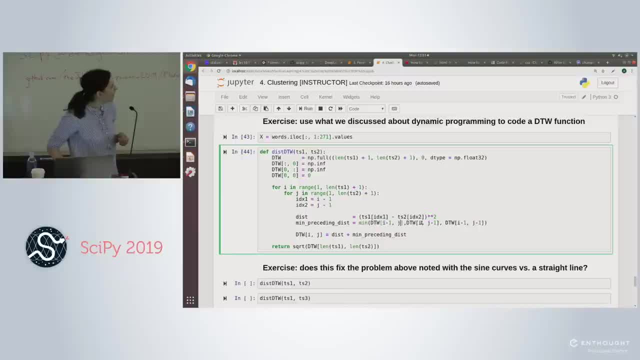 what is the difference between the distance from i minus one and j, or the distance from i- j minus one, or the difference with i minus one, j minus one? Remember, these i's and j's are how I'm moving along the temporal axis. 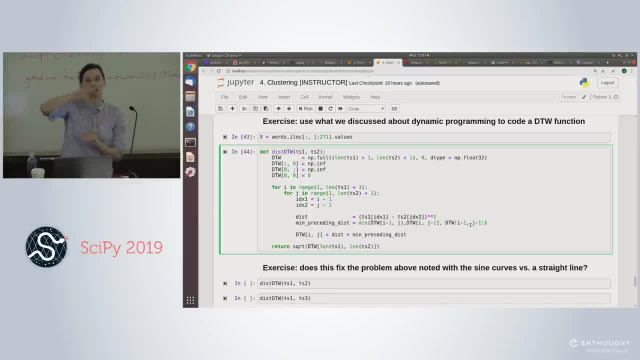 and remember I have disconnected the two axes of my curves so I can sort of move along one curve but not the other, or move along both only one step, the way I've defined it. but I'm sort of trying to move along the axes. 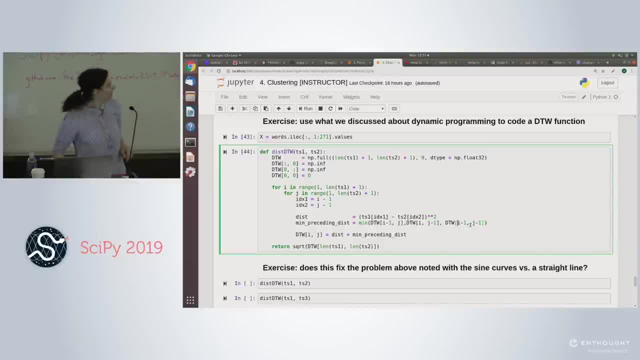 in a way having a path such that my square distance here is at a minimum. So it's sort of this iterative way of working through the data. so what if I move one here but not here, or two here but not here, and how can I sort of 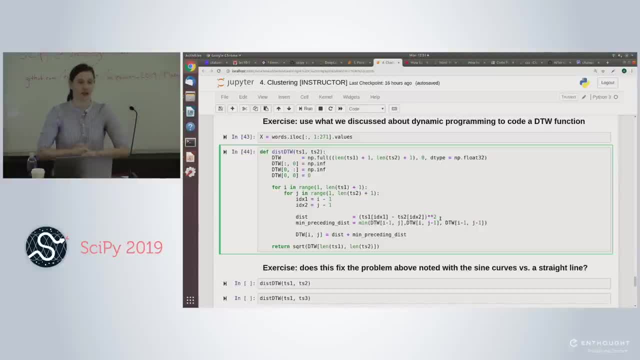 warp these two curves onto each other in the way that makes them fit the best. That's what we're doing, And then, ultimately, I return that minimum distance. I take the square root of that thing, and that's what I'm defining as my dynamic time warping distance. So now I sure hope this fixes the problem. I've wasted a lot of time, so now TS1 to TS2 is 3.7, TS1 to TS3 is also 3.7, and TS2 to TS3 is 4.16.. 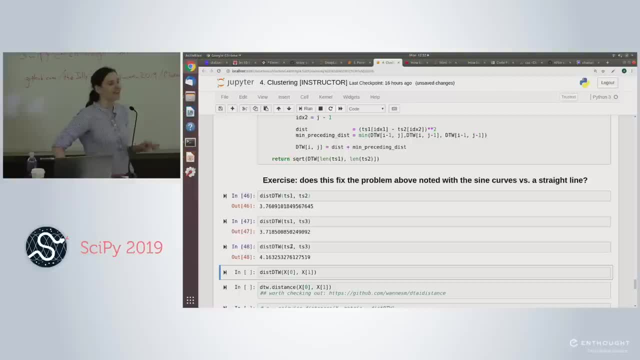 So notice it's still not perfect, right? I still have a problem of my flat line not being as different from my sine curve as I would like, but it's a lot better. At least it's not telling me that my two sine curves. 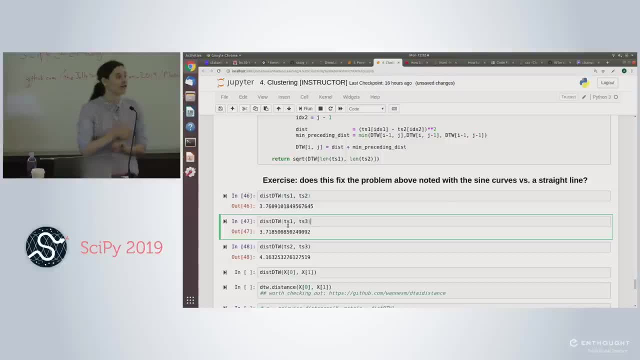 are way different from each other compared to the flat line. So dynamic time warping has a lot of parameters you could tweak. so one thing you might want to do for a particular dataset is explore different ways of stepping back and forth. so what sort of time steps you'll allow? 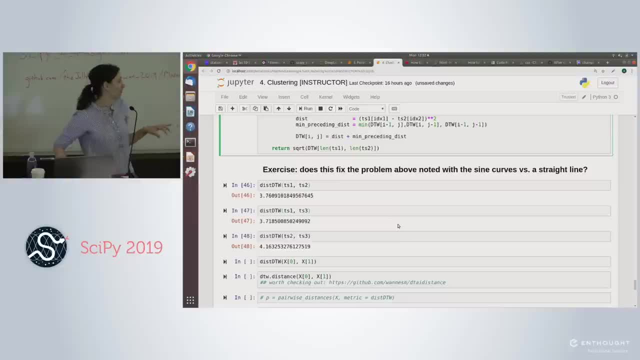 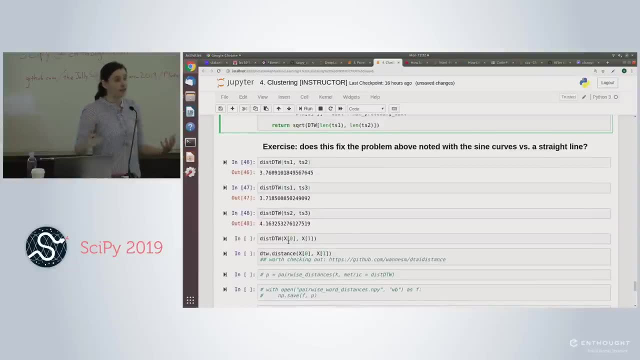 and different distance metrics to see if maybe you could improve the distinction depending on your underlying data. And then the other thing you might want to do is just accept it at some point, in the sense of it is extremely difficult to define differences between time series. 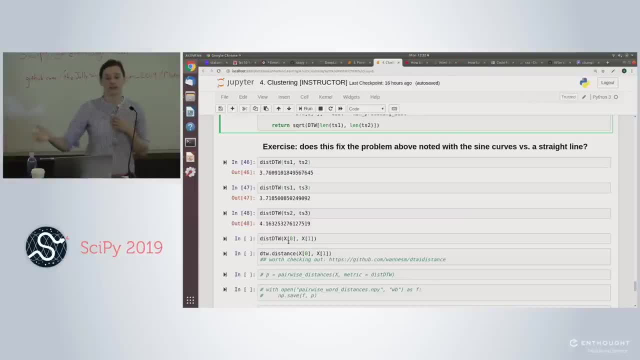 And this is where, if this is not good enough, you might even begin to look into deep learning and you say, okay, it's just an image analysis problem. instead, and let's you know, ratchet it up a notch. 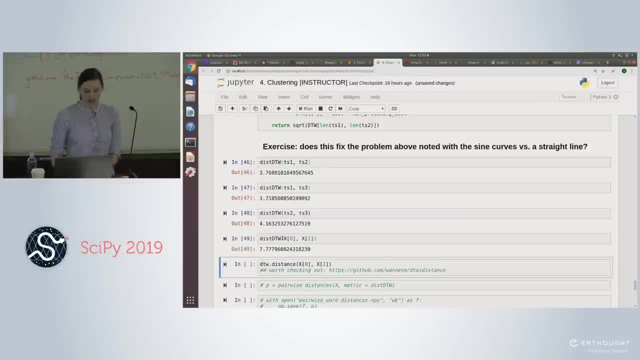 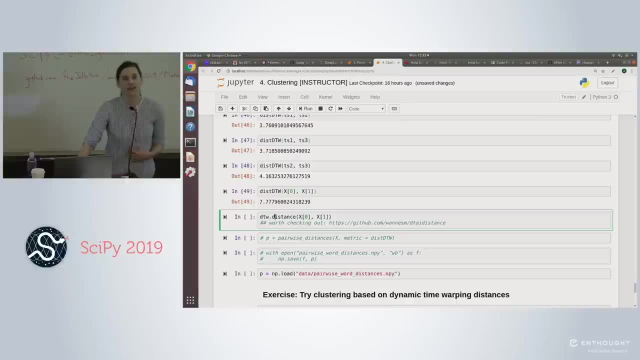 So that's something to keep in mind too, But to the extent we want to keep this as a clustering problem, this is how we want to do it. I also wanted to point out that there are libraries that code this up, so you won't find dynamic time warping. 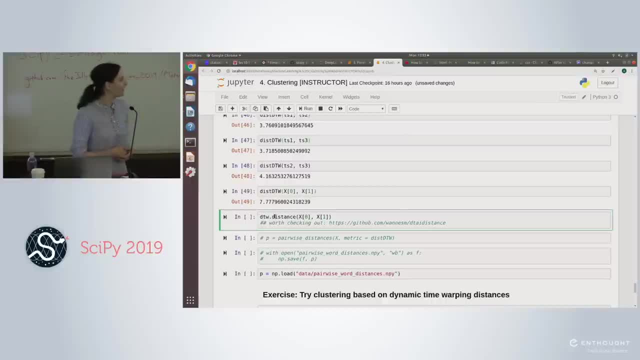 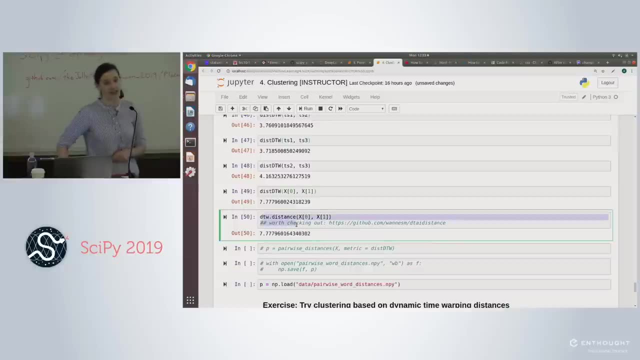 in any of the sort of major libraries like sklearn or scipy, unfortunately, but there are all sorts of DIY Githubs such as this one here. So you can see that actually we have the same definition for sophisticated implementation, where there are more knobs to turn. 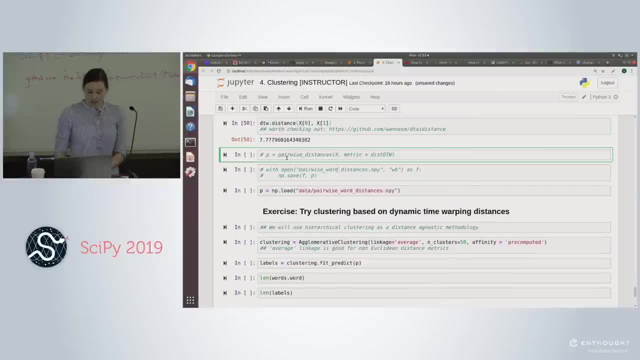 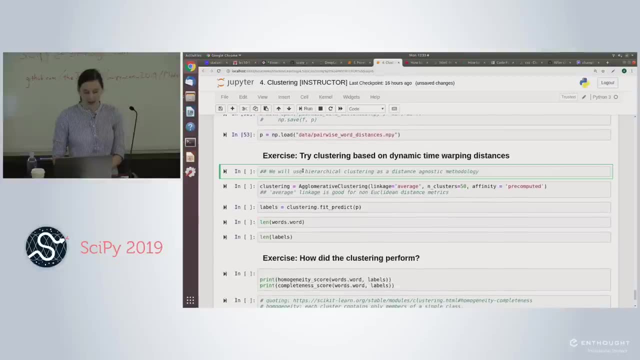 So these things are available, but you do have to do a bit of work. Now, if I were to compute this pairwise distance, it is really computationally taxing, so we would be here a while just sitting around. We're not gonna do that. 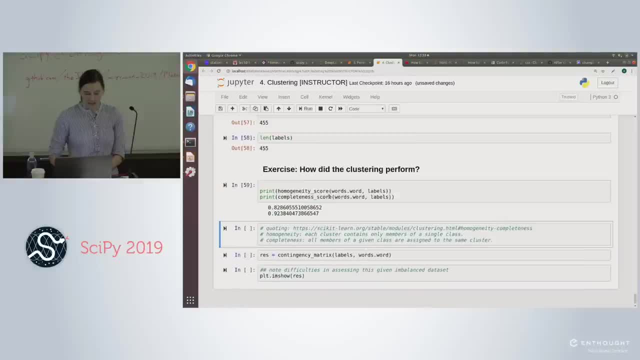 but we are gonna run through the clustering And if we look at how the clustering performed now, now we have fantastic homogeneity and completeness scores right. So the extent to which one class is covered by one cluster is really good and the extent to which one cluster 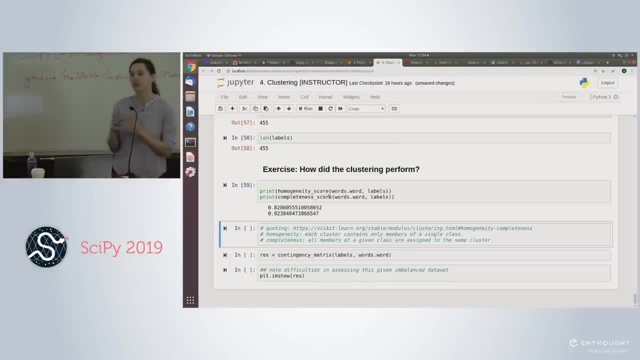 is composed of only one class is also really good. So now we have a really nice one-to-one mapping versus. if you remember, the homogeneity score for just the features was more like 50%, So your distance metric can make a tremendous difference for time series clustering. 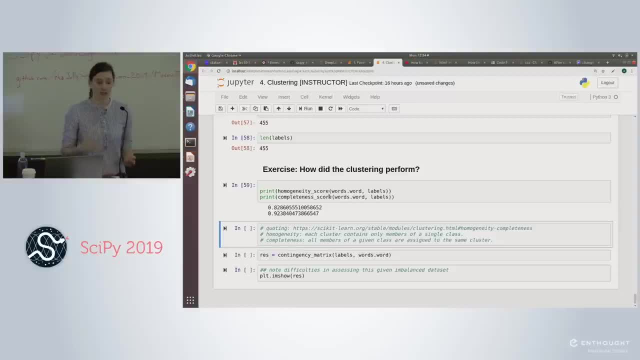 And similarly you can also use these sorts of things for forecasting or classification, right? So for classification, I think it's obvious, you would just sort of map something onto the cluster, and if your clusters are quite homogenous, that's already useful. You can also use this for forecasting. 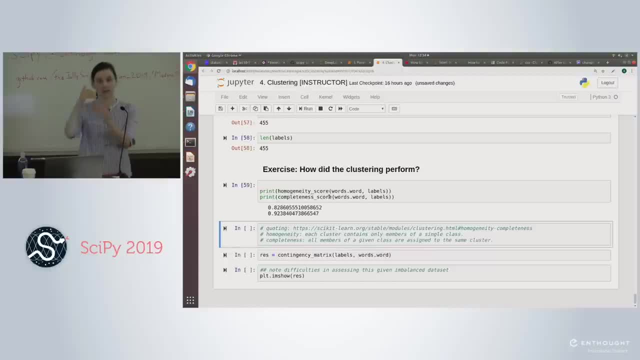 so if you have a little curve, you can say what curve or what time series is this closest to and then use that time series and its outcome to predict the outcome for your new feature. So that's something you see in finance. you see that in health as well. 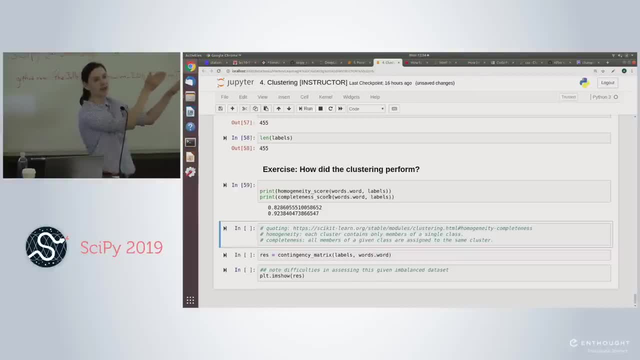 where you're just sort of saying, for example, this patient up to time t, who are they most similar to? and maybe that is a likely outcome for that patient too. And that's really interesting, because then you can use quite heterogeneous data. you can see the result here. 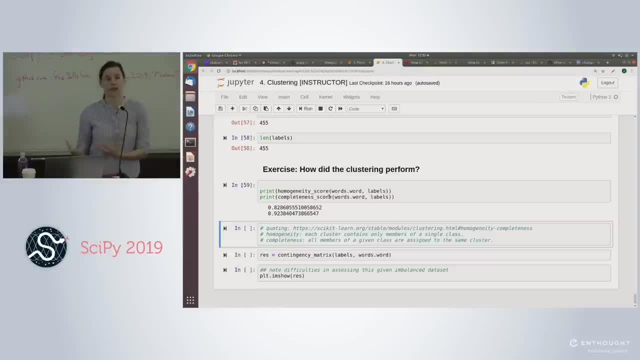 as compared to trying to come up with a feature set, which can be quite challenging. So this is an alternative way to do both forecasting and classification. Any questions? Okay, great, So we are on to our last component, which is deep learning for time series. 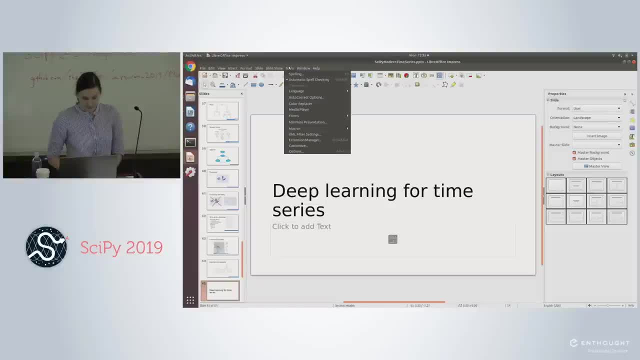 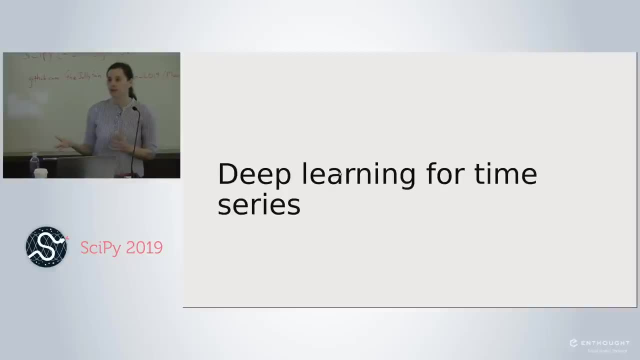 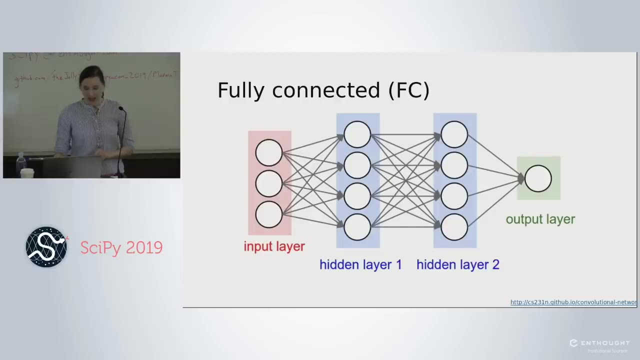 So we just have a couple of slides to cover. Okay. so show of hands. if you have worked with a deep learning, or at least on a toy example, Okay. so for those who haven't, I'm going to give like a very brief rundown. 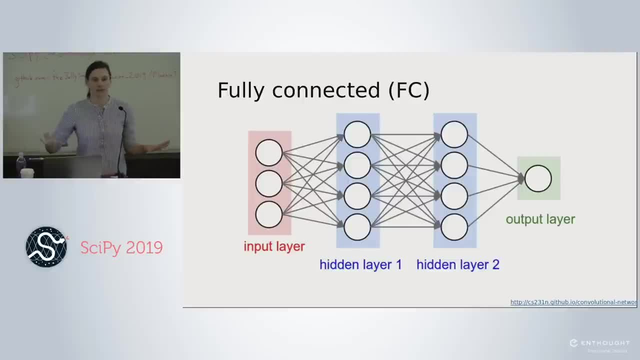 but this is in no way a good substitute for reading up on it and learning these packages. but I just want to give you a sense of how this would look in a time series context. So we start with the simplest of neural network examples, which would be something like a fully connected model. 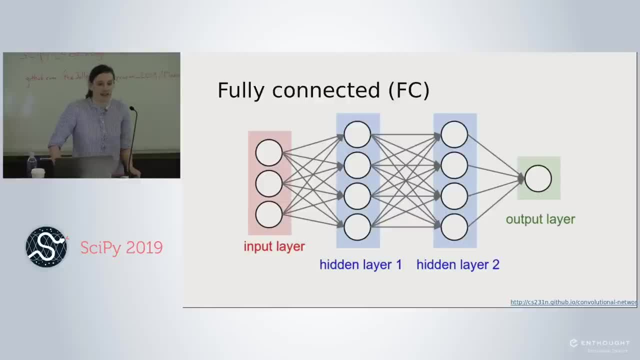 So neural networks are really just a form of machine learning, in the sense that they expect a series of inputs and they are not necessarily time aware. They are not looking for. give me your time series and I will fit a model to a time series. They are looking for samples. 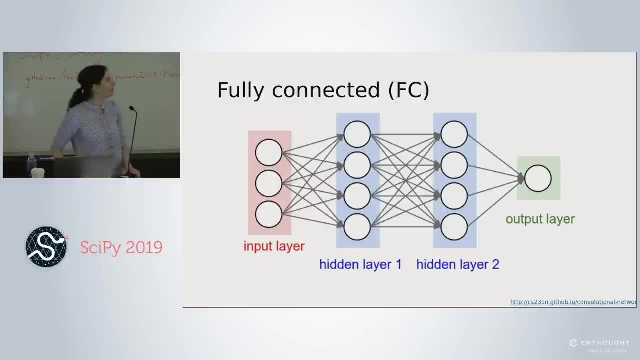 X and outputs. And the beautiful thing, just like machine learning is, deep learning is fairly agnostic. It doesn't really care what inputs you give it. To some extent, these have been billed as you throw anything you want at it and you may very well get a nice answer. 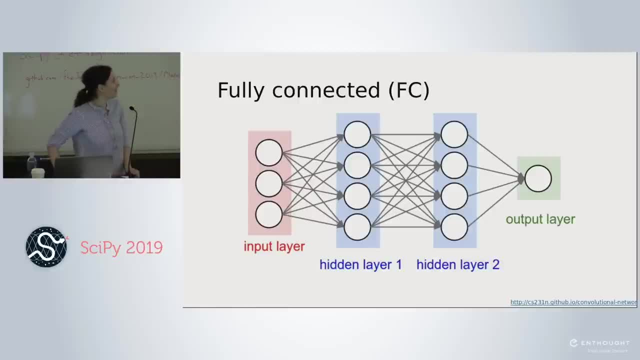 if you sort of tweak your parameters and you have your training. But what does this look like? in the simplest model, You have an input layer which would be, for example, could be features. So this looks a lot like a decision tree where we would create our features. 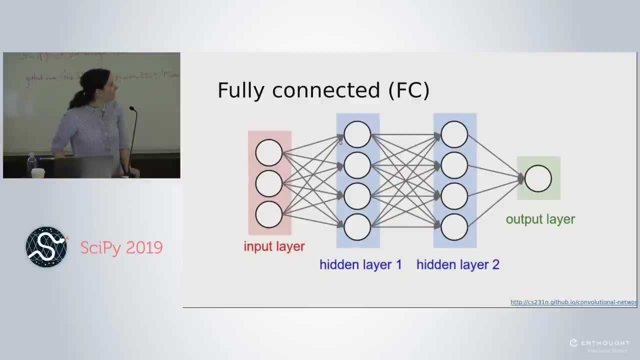 and then we would input them. and the difference between, say, a decision tree and a neural network is that a neural network will look like this. It will. for example, if you were using a fully connected model, then every input would go through some kind of multiplication with a weight. 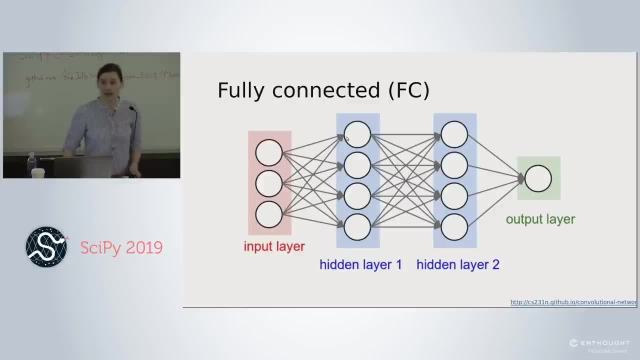 and activation function is essentially just a way of introducing non-linearity. So you would essentially have like a matrix multiplication coupled with a non-linearity to produce your next set of inputs into this layer. This layer would do the exact same thing, right. 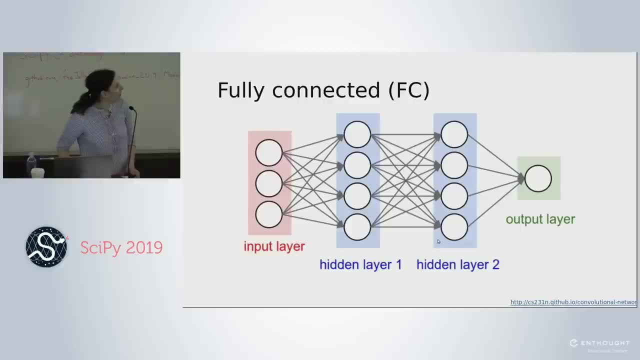 Some sort of matrix multiplication, followed by some non-linear activation, and output it, and then at the end you might have a bunch of new features that have come out through your model and you find some way of combining them to produce your output. That's, like you know, the very, very high level. 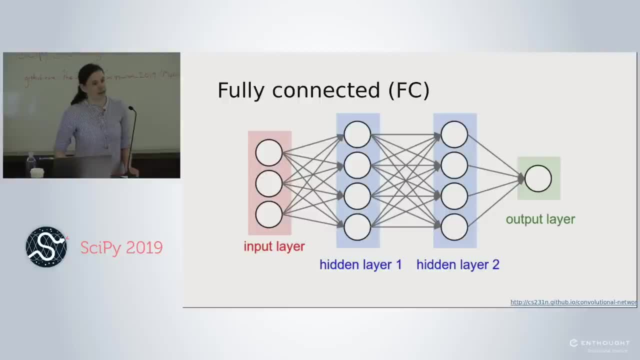 that we've not encountered this before, and obviously there's a lot that goes into figuring out how you should do that properly, how to initialize it. You very quickly get into the millions of parameters. so we're going to leave all that aside, and there are great tutorials at SciPy this week. 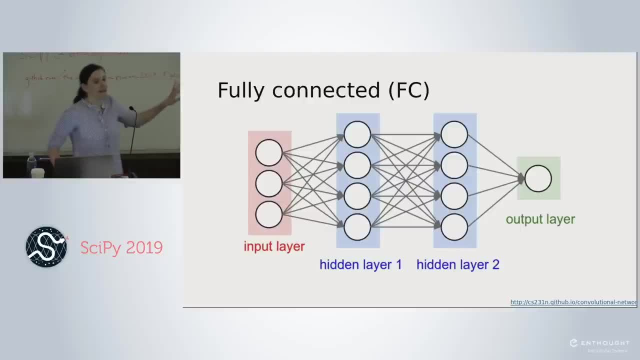 on this topic so you can learn more. But the main point here is that a fully connected model from a time series perspective is just like another machine learning model. it will still require feature generation and a lot of thought about how to sort of translate your time series into something. 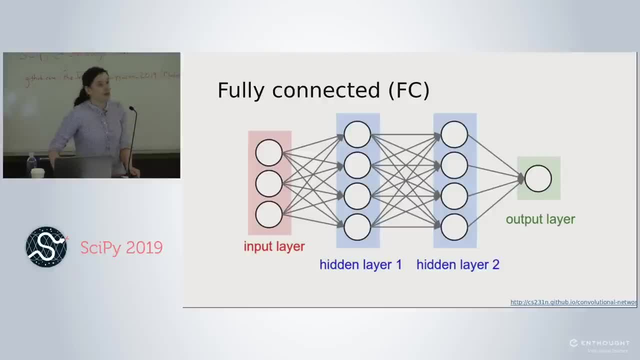 that the cognitive model can digest. So it may very well do better, say, than a decision tree, right? That's sort of an empirical question for a particular kind of data. but this is not in any way time aware, just like machine learning techniques are not in any way time aware. 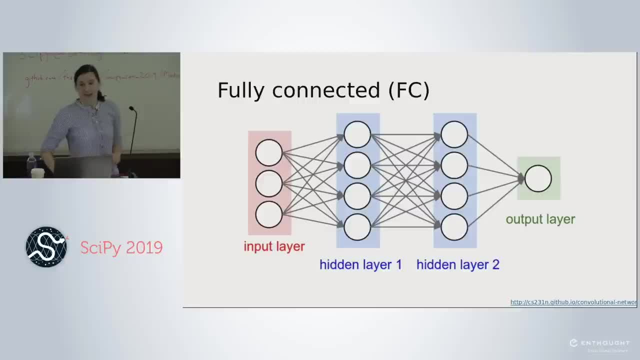 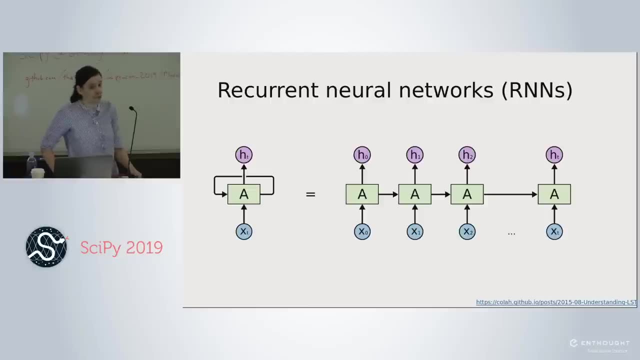 and we have to sort of cut up and pre-process our time into a format that this understands. There are other options, though, So the classic example of how you would put a time series into a neural network is called a recurrent neural network or RNN. you'll mostly see RNN. 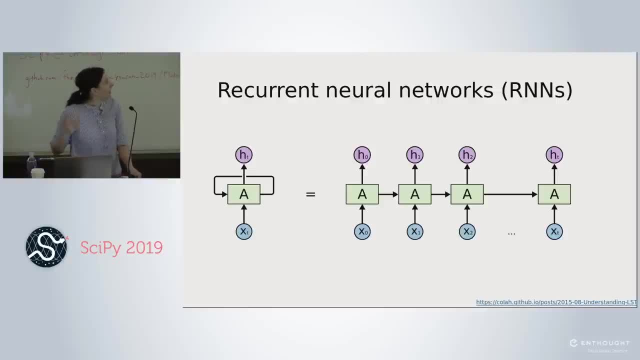 and the idea here is what this does- recognizes that your data will come again and again. your data recurs. so you build one cell, one cell, but basically what you do is unroll it and you reapply it at each stage with your new data. so this provides a unifying slash. 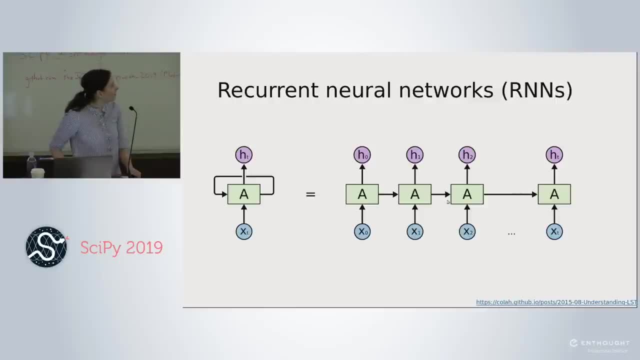 temporarily aware way of looking at your data, because you have a model that understands it's going to be rolled out and used on the same data. so what does this look like? So this is a multivariate case. in either example doesn't matter. you have your existing neural network model. 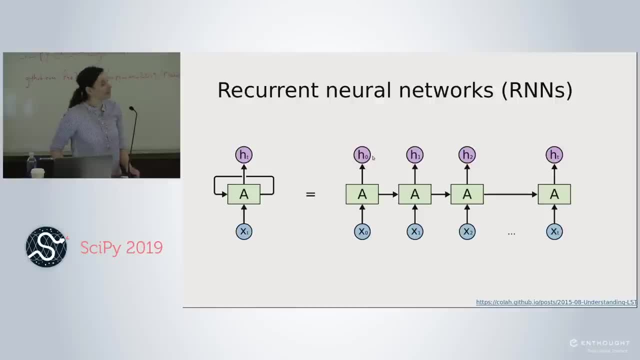 first, you put in your first value of your time series, chug chug chug. it produces a hidden state. you don't need to worry about that, but that's part of its internal accounting. why does it need a hidden state? Well, that's what makes it temporarily aware. 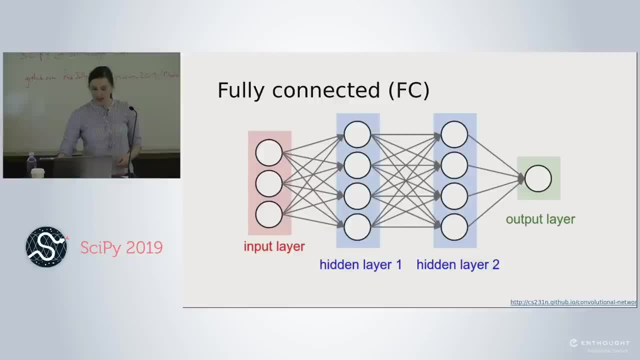 that's what gives it the ability to remember things from state to state, rather than in this example, where it just gets something and chugs out one response and there's no time it itself has a temporal axis. it produces its hidden state. then you put in your next value. 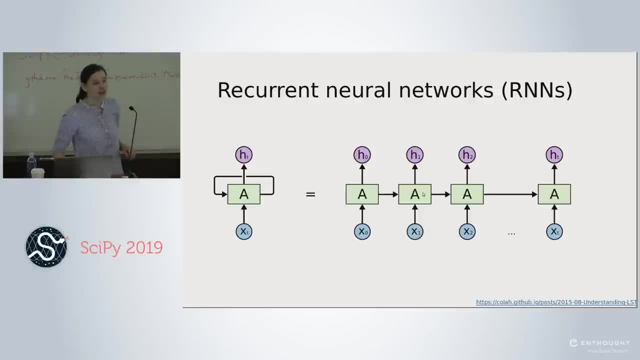 it remembers its hidden state that affects what goes on in here and out comes a new hidden state. so your model has some form of memory or some way of evolving over time, recognizing that your data wants something that recognizes dynamics that are evolving over time, so recurrent neural networks. 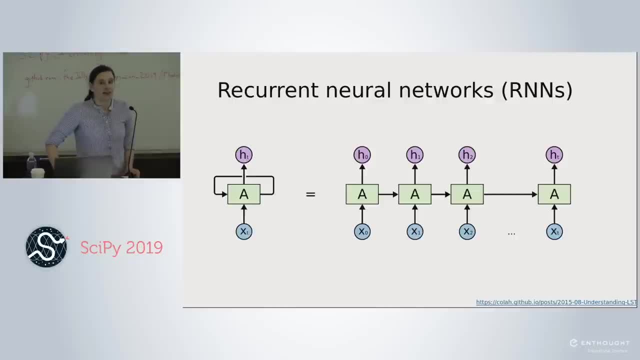 just like everything else we've talked about today- not a new idea. I don't know the exact time, but I believe it's early 1980 that these were envisioned, and even things like you probably know the term GRU or LSTM. my understanding is even an LSTM. 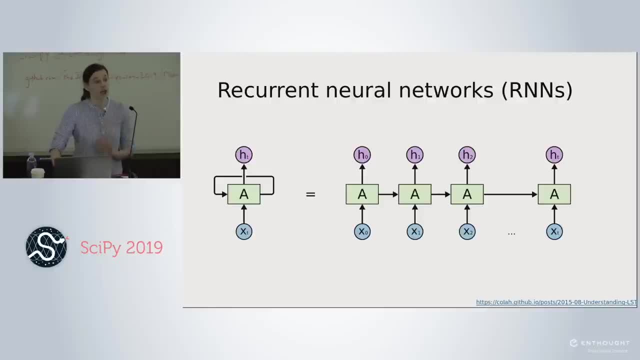 was envisioned in the 80s- although maybe I'm wrong and it's the 90s, but it was certainly a long time ago. even though these are still considered relatively cutting edge, exciting new technologies, what's really exciting is A we've developed much more of an art. 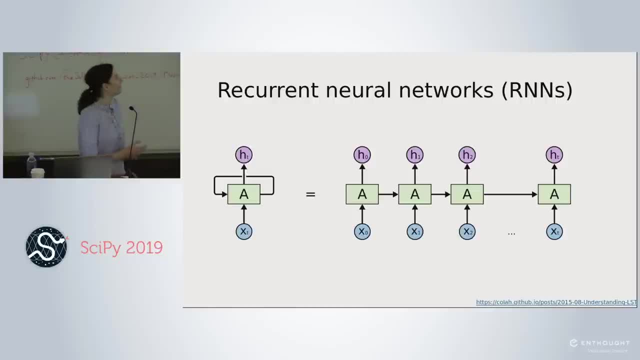 as to how to fit these. how do we initialize these things? what does back propagation look like? and, of course, much more exciting is that the ability to imagine something. this was there in the 60s, but the ability to actually do it is what's fairly new. 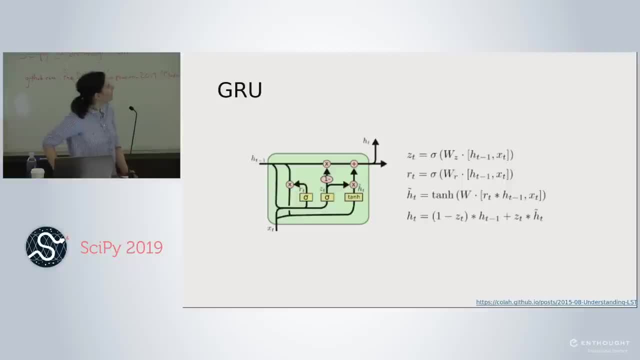 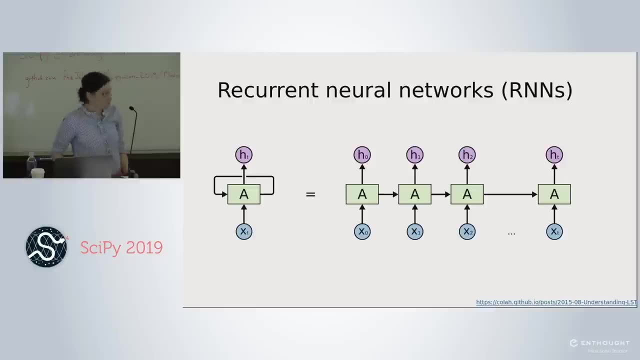 and also the presence of enough data to get good results is fairly new. so the two variants of recurrent neural networks that have turned out to be quite successful. one is called a GRU, so you see an example here. what we're looking at now is if we were to actually unpack the guts of this thing. 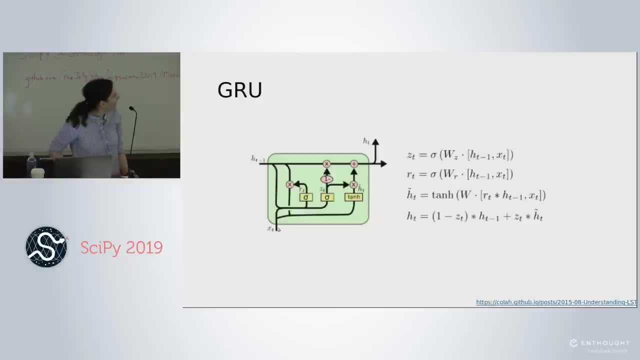 so if we unpack the guts, this is what we've got. we've got our XT that comes in, it goes through several different variants of transformation and people have the update gate, the forget gate. the idea is that you have different components. one is supposed to help the model. 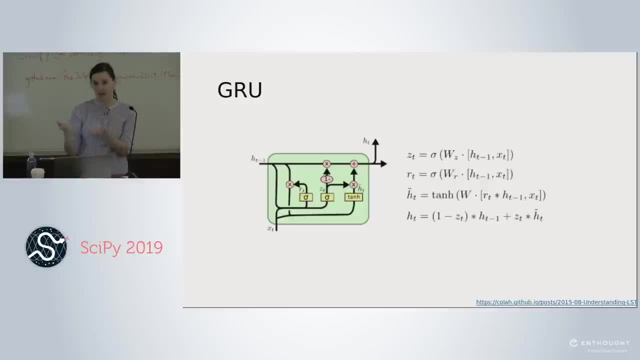 to decide how much it should update its hidden state based on new information. another looks at the new information coming in and transforms it before it even talks to the hidden state. and so you have all of these parameters that can specialize to describe different properties of the temporal dynamics. 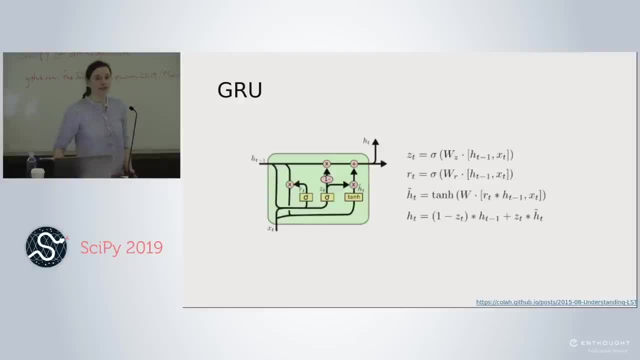 of your data, depending on how they allow the updating. now the interesting thing is: in a way this sounds a bit like what we talked about with structural time series and state space models generally. it is developing some sort of internal model, just like the common filter, of how it should adapt to new information. 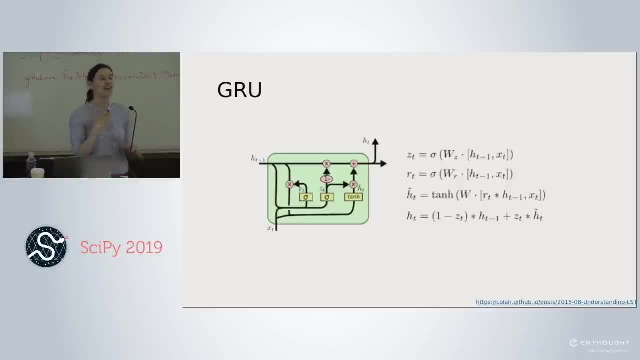 given its prior expectations, although in this case its prior expectations are a hidden state. that is not sort of a well described statistical thing. it's more like a set of parameters in a matrix not as well developed as I'm sure it will be in a decade from now. 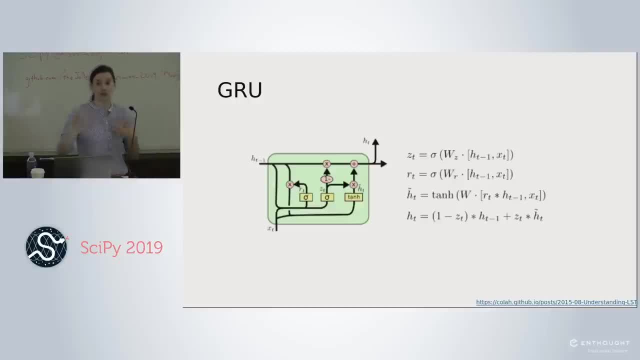 and we'll eventually figure out. these are still models. they can still have statistical properties. it's just so much harder to think about them. but that's what a GRU is. a GRU versus an LSTM- you've probably heard of these two. an LSTM tends to be a little bit more complicated. 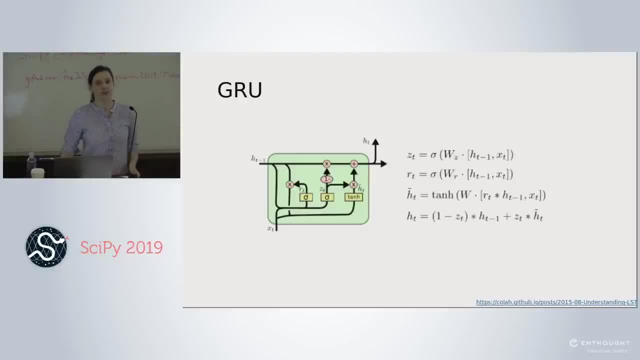 it has one more gate compared to a GRU. in many cases it doesn't perform any better, but it's sort of worth looking at both of them, depending on your data set. LSTM, people say, has sort of a longer memory, so it depends very much on what kind of data you're looking at. 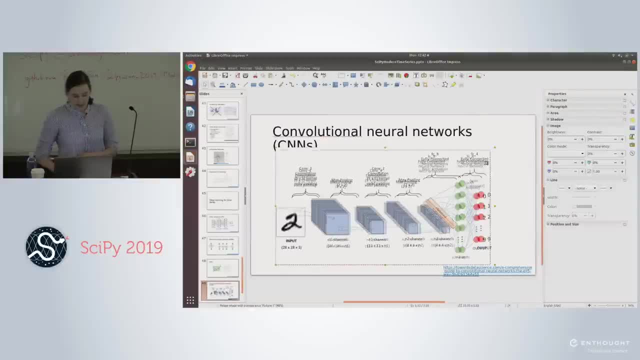 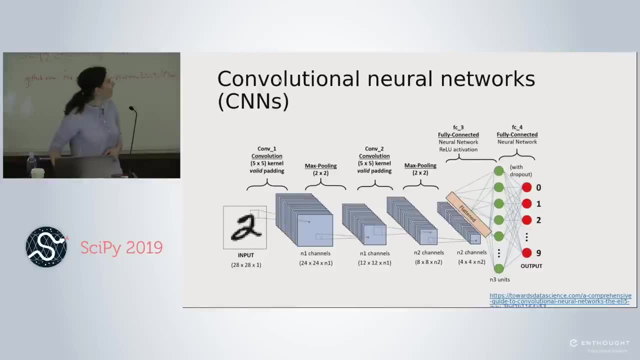 okay, so convolutional neural networks. you might be surprised to see this here because you're thinking, oh, I heard RNNs are actually RNNs are time aware, but actually CNNs can also be time aware in the sense that an image is very much like some of the things. 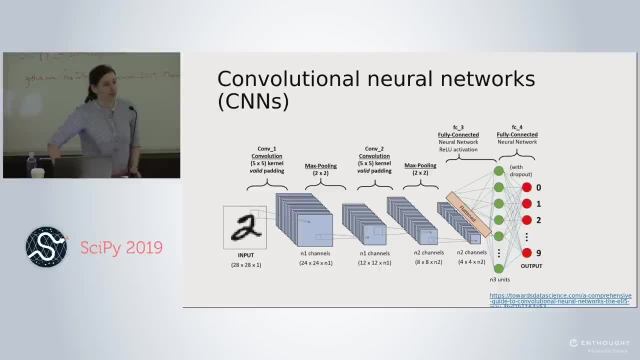 we've done today, such as time series classification. time series clustering does not look all that different from image analysis, so we can also use convolutional neural networks as a way of understanding our time series as a picture that can be on its own already a good way. 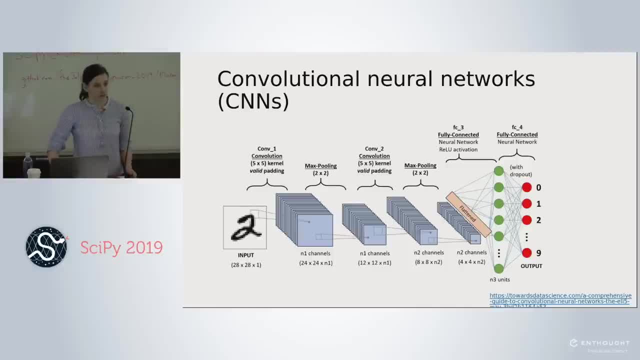 to classify a time series. we can also do modifications to convolutional neural networks that make them temporarily aware. so one example of that is what's called a causal convolution. so in a standard convolution, if you do image analysis, it sort of treats all directions as the same. 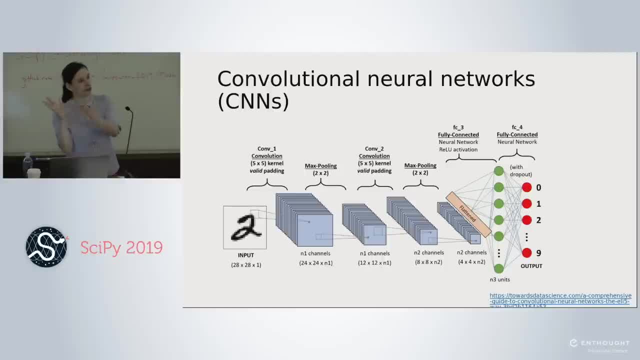 and all areas are equally spaced. so you have convolution where convolution sort of only goes in one direction temporarily, and in that case you have convolution that is also time aware. that can be used as an input to other components of a model, or it can just be its own model. 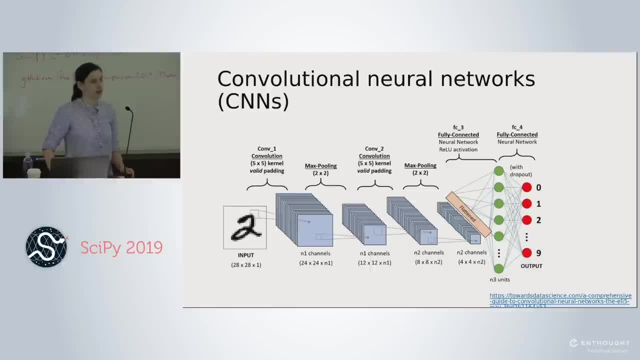 which of these performs better will very much depend on your data. what kind of patterns are in your data and what kind of task you're trying to do? are you trying to predict or are you trying to classify? CNNs tend to be more successful, or are you still sort of working out? 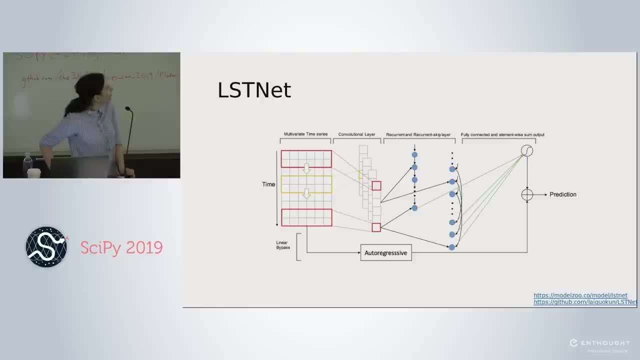 the science of how these things work, and so one actually really cool architecture I wanted to highlight. this was published about two years ago, I think- LSTNet. so these researchers actually said: well, why do we have to pick and choose between convolutional and recurrent behaviors? there's actually no reason we shouldn't use both. 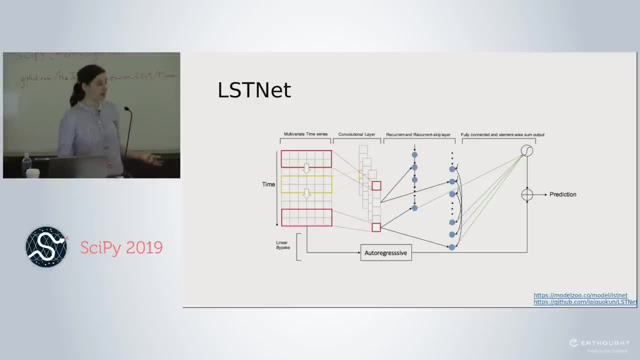 and in a way that makes sense, because if we think about something like the airline passengers data, there's sort of both aspects. there's this sort of aspect of we see a trend, sort of more like RNNish to see a trend. I'm not sure convolutional understands that. 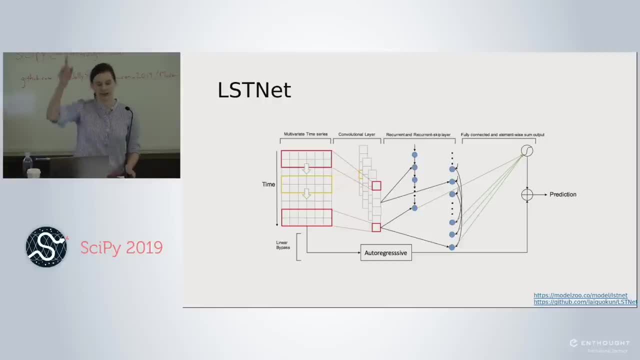 but on the other hand we have this seasonal component where there's sort of winter, fall, summer etc. and that part seems a bit more like an image analysis type of component. so they had this idea. they also said we can use the convolutional bit. 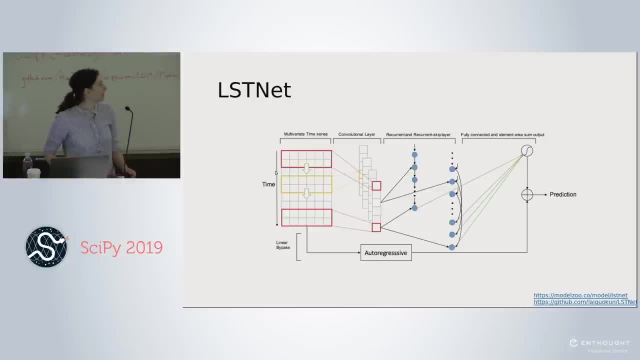 to understand better how to use multivariate time series. so to the extent we want to relate different inputs, if I have different inputs into my model and it's not just a univariate time series, do I want to sort of convolve these? there are a few advantages to that. 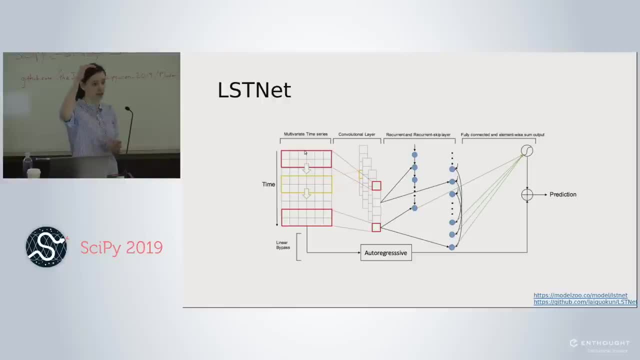 one is: maybe you'll discover there are relationships between them, especially if we convolve on time and input and we sort of take almost like a sliding window image of our time series. but we can also think maybe the convolution itself might identify some seasonality, because that's sort of image-like. 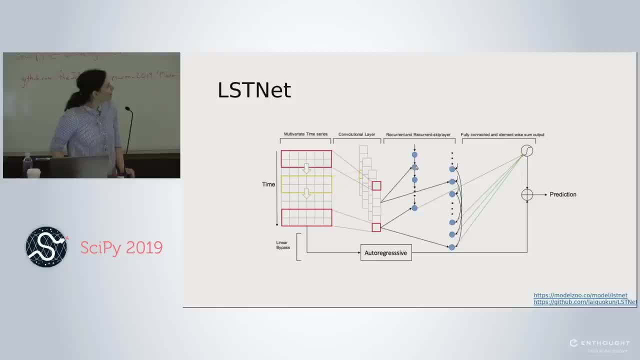 they also said: well, why do we always do sort of recurrent, where we just sort of feed it in one at a time? what we might also want to do in architecture to better reflect certain realities is we might want to have something that reflects the reality of seasonality. 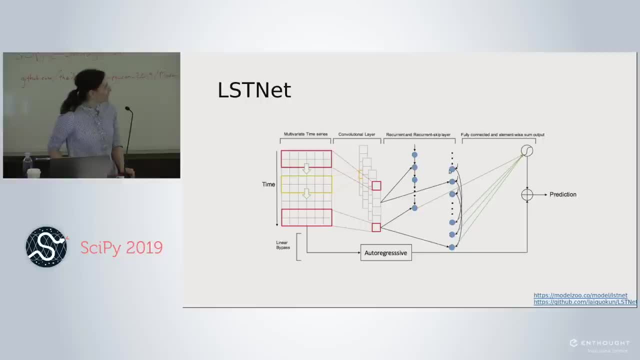 so we might also want to have something where we skip. so maybe if I have 24 hour data, I might want to have both an RNN that looks at all the hours, but I might want to have an RNN that, in addition to looking at all the hours, 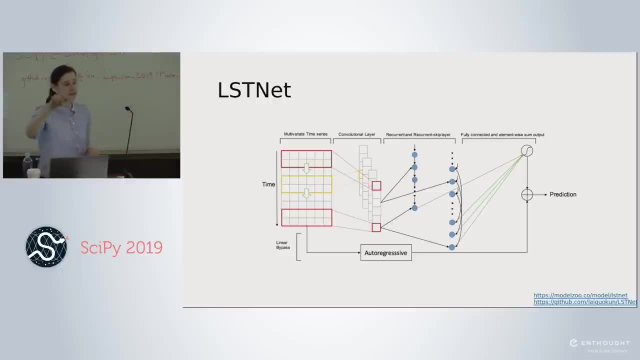 only looks at the same local hour for previous day. so if I'm at 3 am trying to predict the electricity for 4 am or whatever up to 3 am, that sort of slice. but I might want to look at 3 am from the previous day. 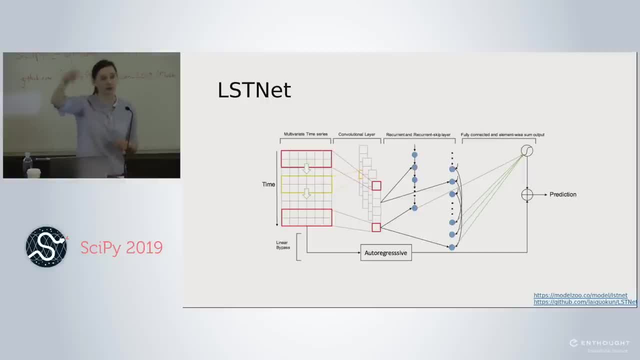 and the previous day and the previous day and think of that as its own time series and have a recurrent neural network that runs only through that, or, if not, that maybe only look at the states of the recurrent neural network at those points. so for those of you who have worked with neural networks, 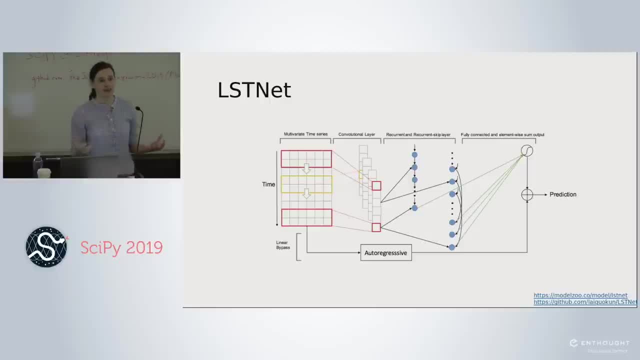 you know that there's actually sort of infinite architectural permutations. you can make anything you can imagine. you can build and train it properly. of course, is always where you run into trouble in figuring out if you actually have enough data to train it. but the wonderful thing about this- 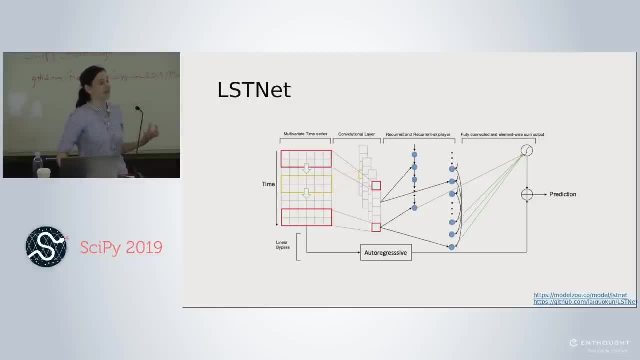 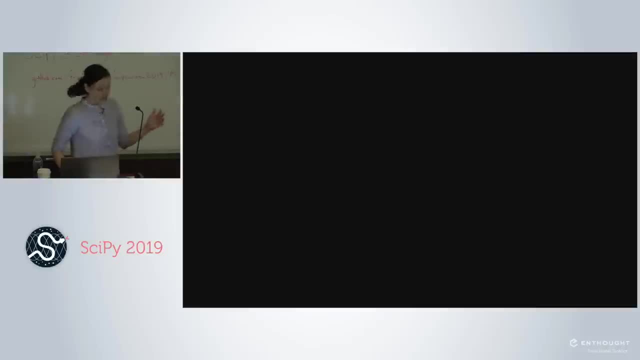 as compared to some of the other models we've looked at today, is you can imagine any sort of dynamics and describe it with some kind of neural network and see if you can improve your forecasting or classification or what have you, so that that is prediction. so let's see if I can get my 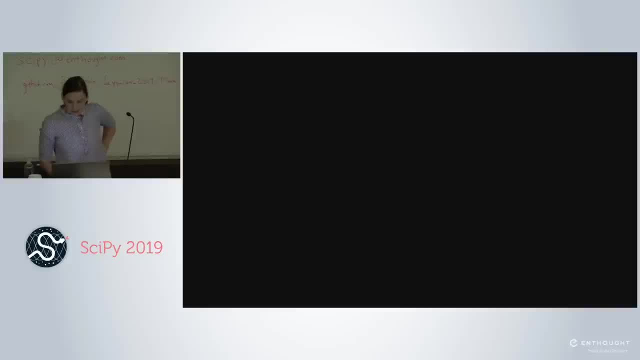 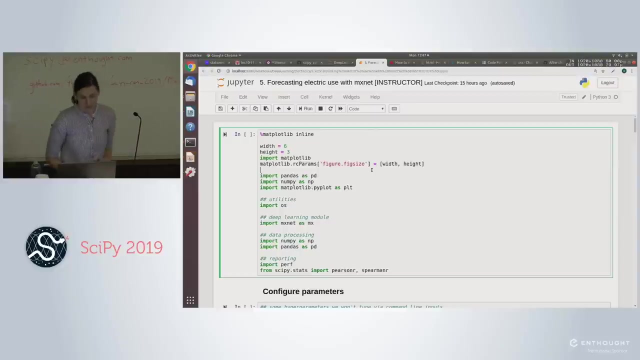 hopefully it will come back up, okay, so in the meantime, I would ask everyone to open your notebooks. so we're going to look at notebook five. this is supposed to come back on electricity. okay, I'm going to see if I can. oh, excellent, thank goodness. okay, remind me not to move at all. 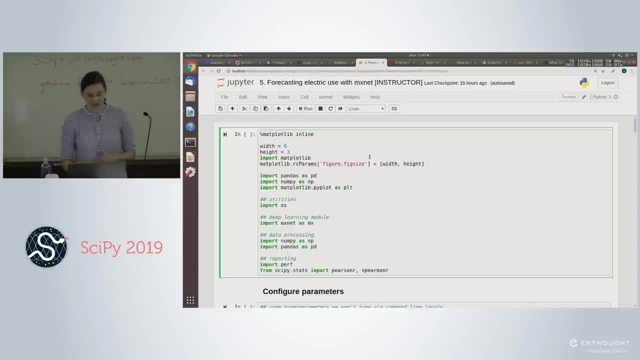 until for the next 13 minutes. okay, so we're going to try to forecast electricity. this is one of the original data sets that was used when the LSTNet model was published. the LSTNet model: when it was published, they saw pretty big gains compared to say, 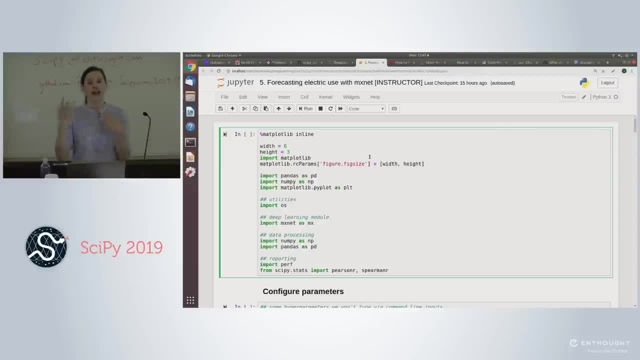 something like just using a GRU or just using a convolutional neural network. and this point of you know, building an architecture that reflects especially sort of the temporal cadences of human activity works really well. and also they were making the point that with multivariate time series, 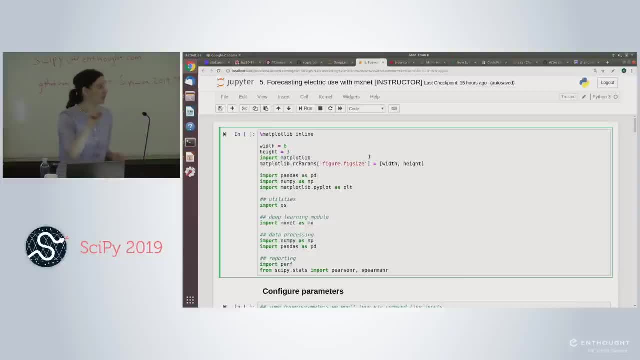 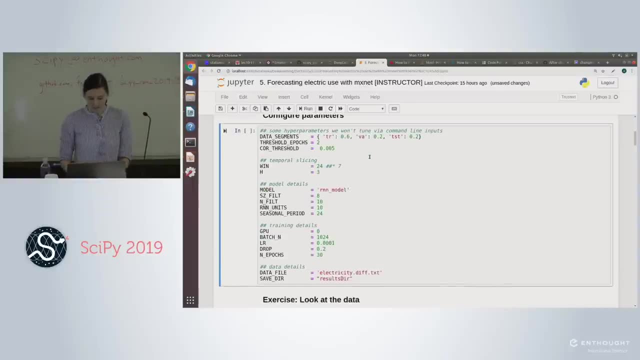 it can be interesting to find ways to combine those information channels. so those were what they pointed out. so one of the data sets they used was this electric data set that we're going to use now. so the first thing we're going to do is look at the data. 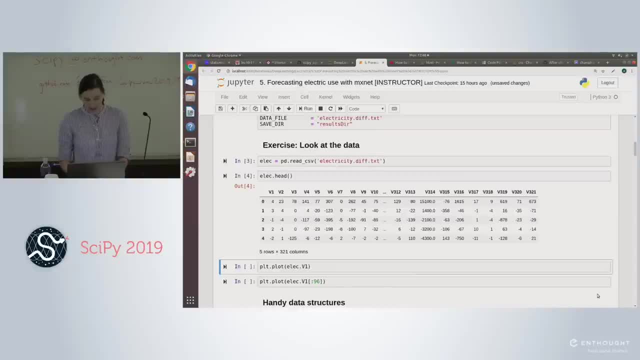 let's look at this together. so if we read it in and look at the head, as you can see this is like very multi-channel. this is 321 parallel time series of electric use, hourly electric use at 321 different sites. I want to say it's the state of Alabama. 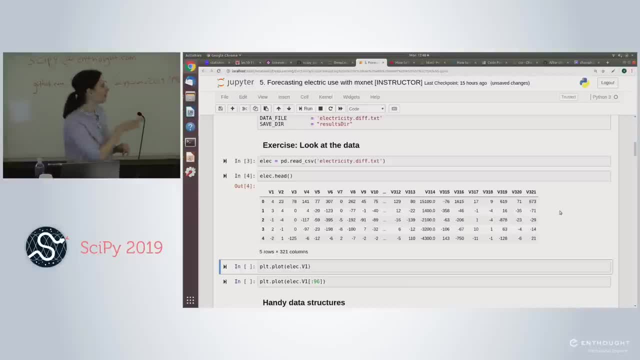 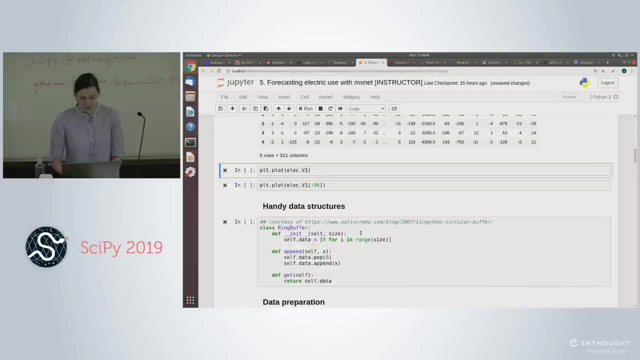 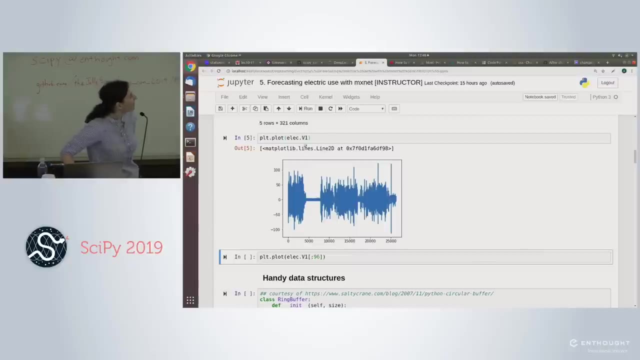 but I don't remember you'd have to check the reference to the data they do mention. but it's hourly electric use in some state in the US and if we plot this, as always, there are, you know, sort of better and worse ways to plot. but look, this is really interesting. 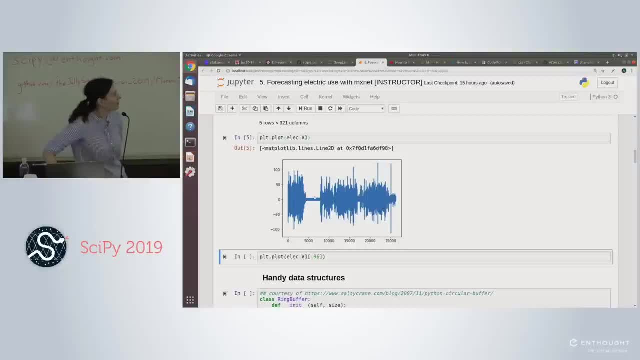 this is just that one site for the full range of time. it's interesting to me because you have sort of drastically different regimes. so if I were doing, say, a traditional statistical model or even a machine learning model, I would be really hard pressed to think: oh my goodness, how am I going to make 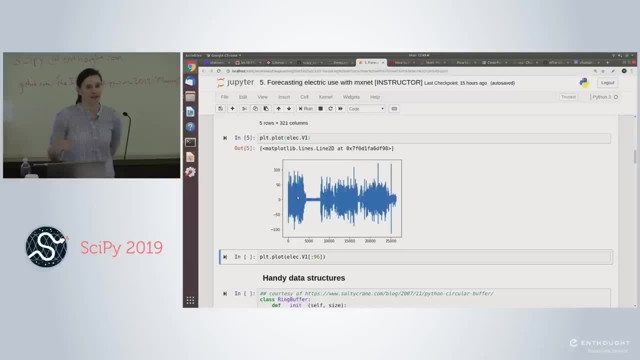 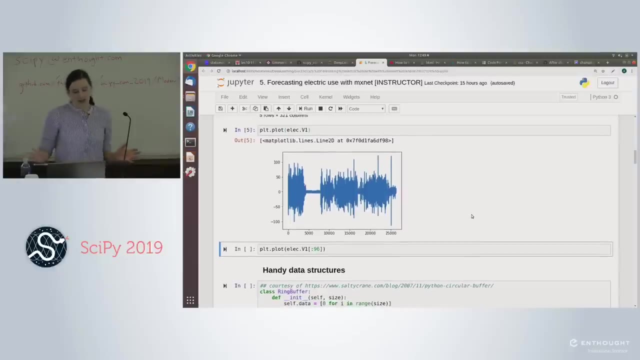 all of these different points in time comparable. this looks really different. it would take a lot of thought, whereas with a neural network sometimes- because we don't for now have those assumptions built in- we can look at the data and maybe even notice things that we wouldn't notice. 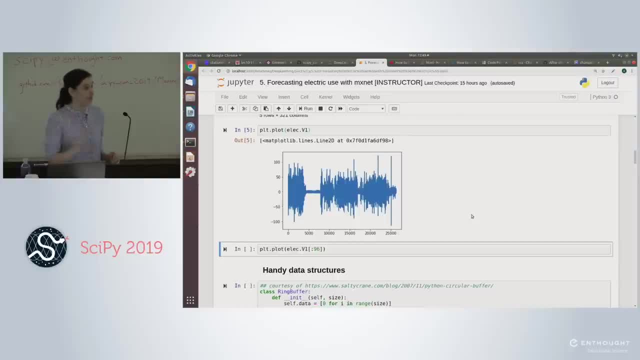 but this long term plot. this gives us one view. it tells us that we've gone through sort of different regimes of electric use at this one site- and this is just one of 321 inputs- and unless I were doing this as a full time job for years. 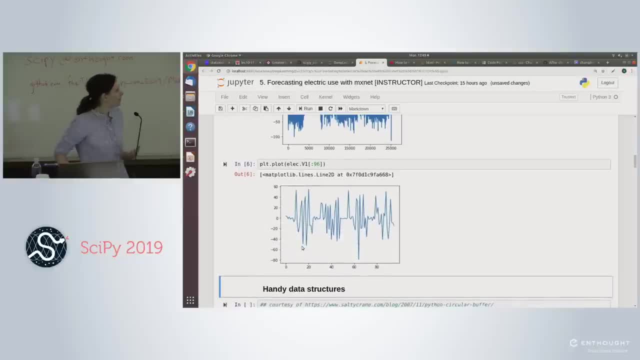 I'm not sure I'd be able to look at all 321 and know them, although great if you can, right. but also let's remember, if we look at it at this spot is some kind of recurring pattern right, which makes sense because this is hourly electric use. 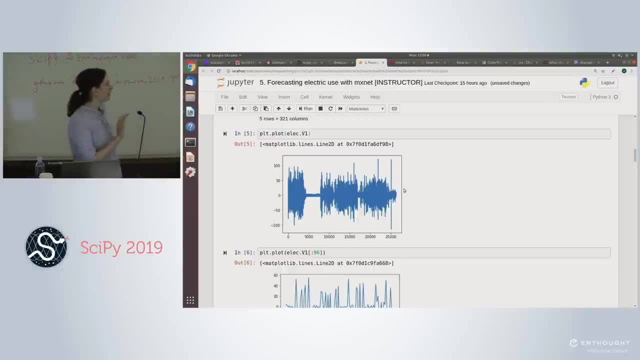 now you might be thinking, oh well, I would have expected to see better use than this and this is because we have. I have pre-differenced this data for you. so actually the original paper fit to the original time series, which looks more like the air passengers. 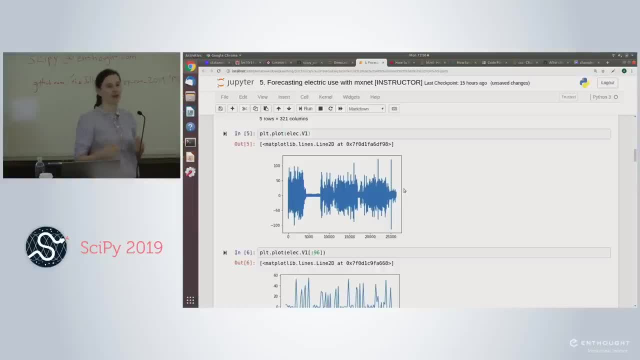 it's sort of a count, but A, that's too easy and B that tends to over represent with a null model. so if we difference it out, we are being really strict with ourselves that, like the model has to add something useful that can predict from hour to hour. 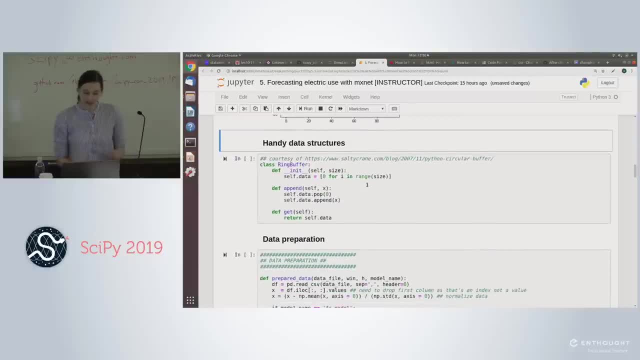 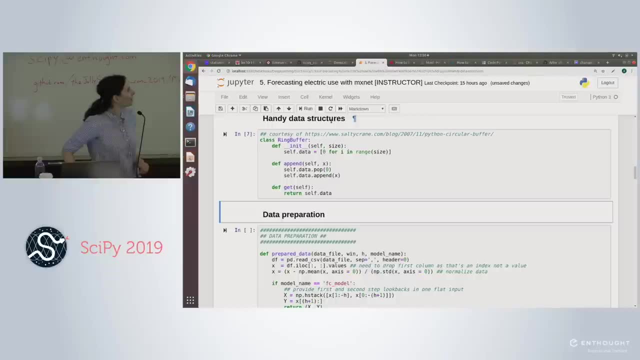 rather than just sort of globally getting it right. so I encourage you, whenever you can, to use differenced data. ok, so handy data structure. this is nothing to do with time series, but I like to use something like a ring buffer when I'm sort of thinking about a way. 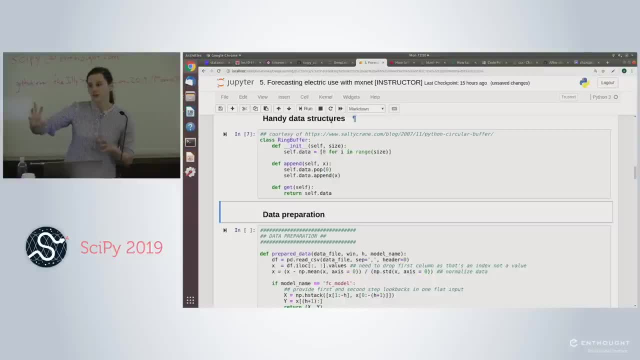 to do early stopping. so another thing for those new to neural networks: there's no sort of predefined limit as long as you're getting better. but you want to make sure you don't over fit. so that's similar to other techniques we've discussed today. the difference being is that now we could. 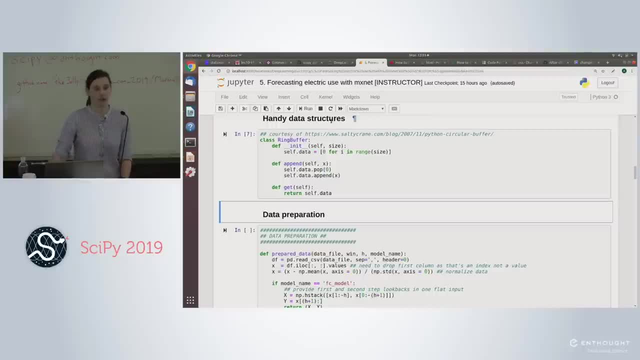 potentially have way more parameters than even the most complicated model we've looked at. we talked about how structural time series- there's so many knobs to turn- looks like you could really game it if you wanted to. that is like orders of magnitude different from this. this is really a lot of knobs to turn. 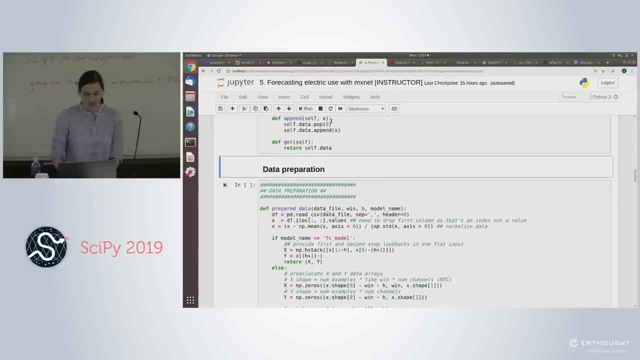 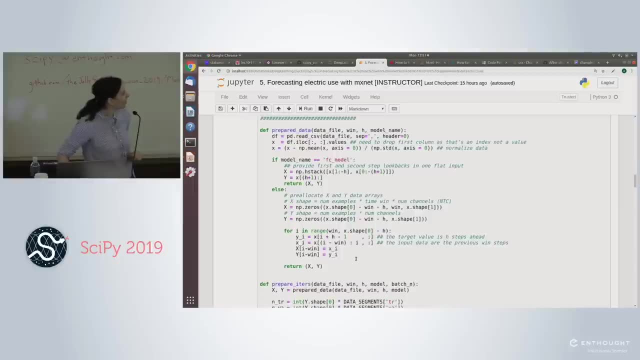 so we need to make sure to be disciplined in our fitting. so that's just one way that I did early stopping. ok, so data preparation. I want to call your attention to this, because this part actually looks a little bit like what we had done before, where we take one long time series. 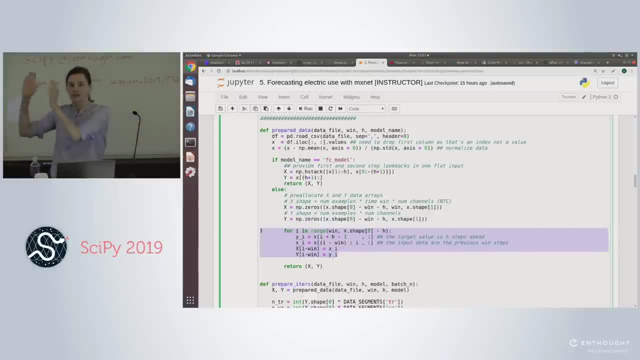 and we reshape it into many slices of a time series. in this case we have multichannel, so we're not just slicing along one axis. we actually have to slice all of our multivariate time series and make sure that all of them sort of: are these sliding windows? 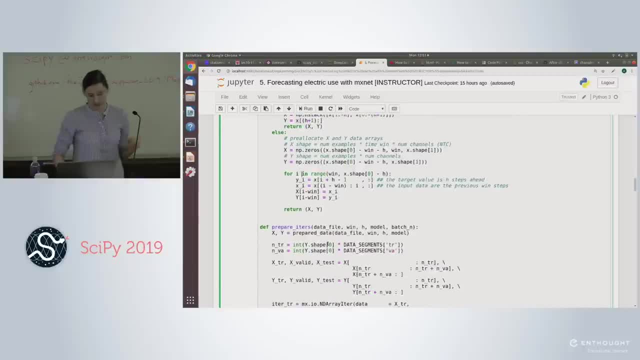 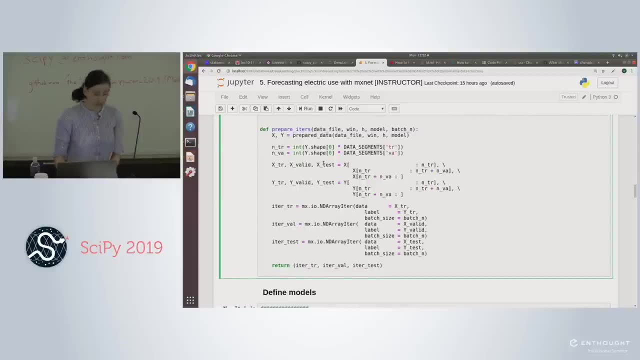 and keep them in sync. so that's what this data does. I encourage you to look at it on your own as well to see how that works. we also build data iterators so that we can prepare batches of data. ok, so here's the interesting part. so I provide examples. 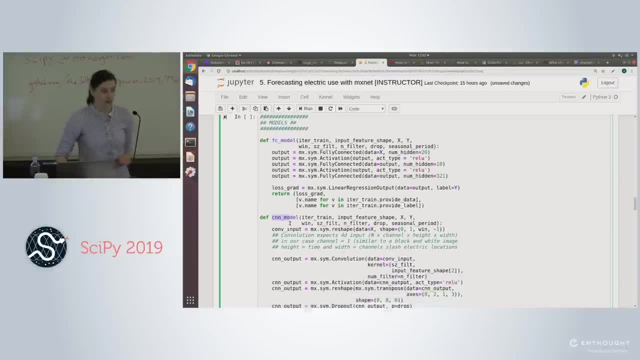 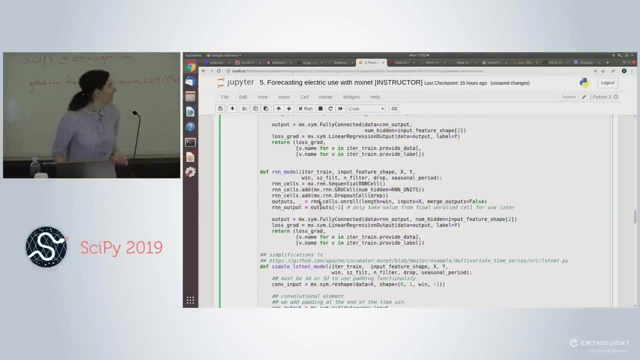 of how you could use a fully connected model or a CNN model. I would encourage you to try those out on your own. you'll find that they don't tend to do as well as the RNN model or the simple LSTNet model that I've introduced here. 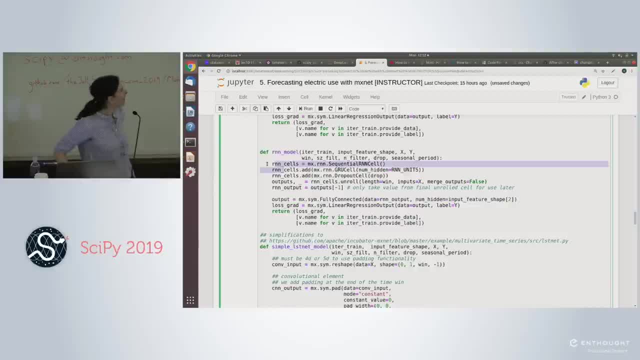 so just briefly, the RNN model. how do you build an RNN model in MixNet? well, you need to have a cell and then you need to add that cell. you decide how many hidden units you have, which is basically saying, how large of a hidden state matrix do I want to have? 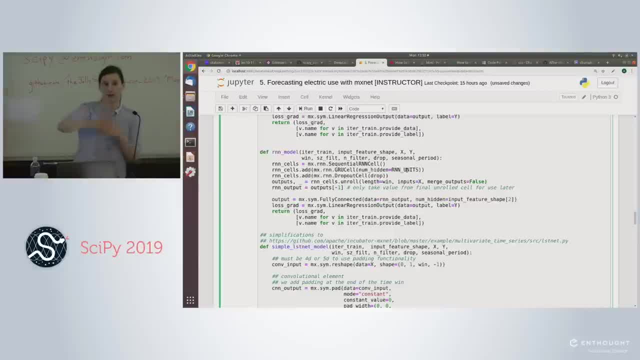 how many different parameters do I want to have to describe this behavior of how it should update and how it should retain information? so, with an RNN model, that's essentially just one layer of this RNN rollout that we did already. now let's look at this LSTNet model. 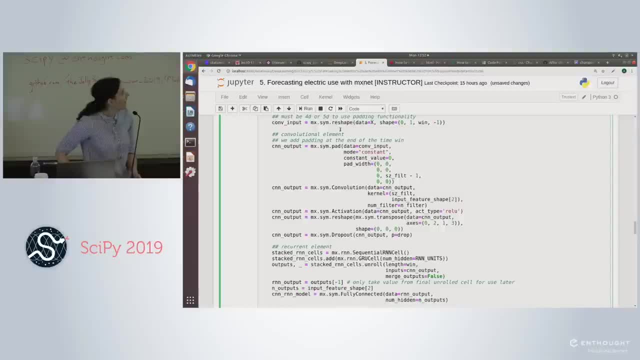 this is really interesting and this corresponds to that architecture I showed you. the first thing we're going to do in this case is we're going to apply a convolutional filter to our inputs, so we're going to take our inputs, which is multichannel. so actually, in this case, 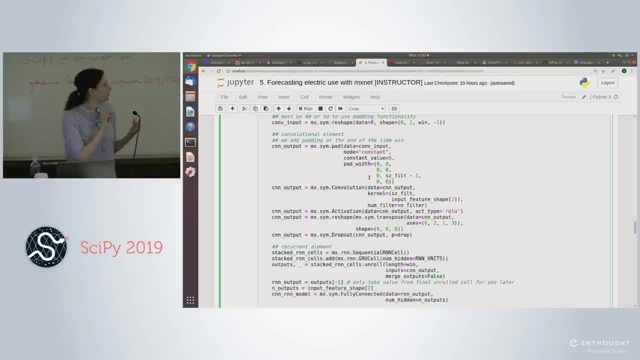 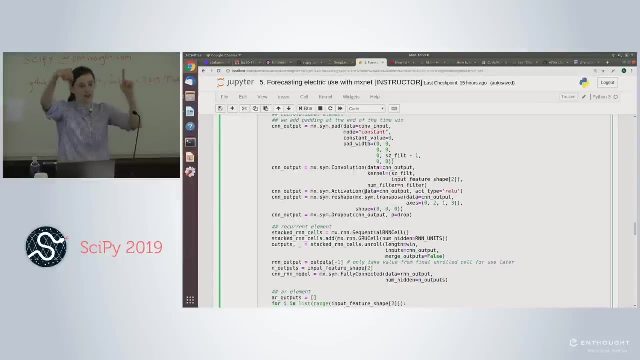 we have time by batch number by TNC, time by batch number by channel, where channel is like 320. so the first thing we're going to do is run that through a filter where we're basically looking at a sliding window as an image, so the window slides both over time. 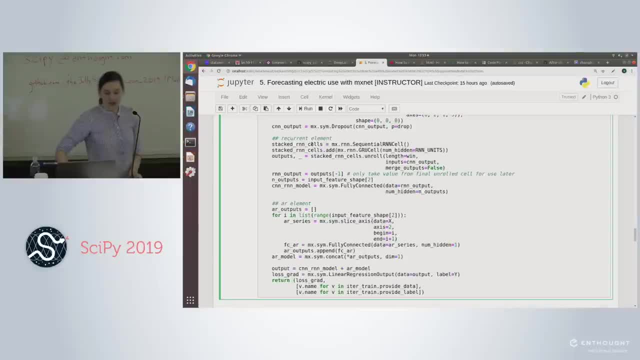 and over all of our features. we then take the convolutional output and that becomes the input to our neural network, RNN, the recurrent neural network. so in this case we've said, instead of just feeding in our raw values, we could also consider processing those with other neural components. 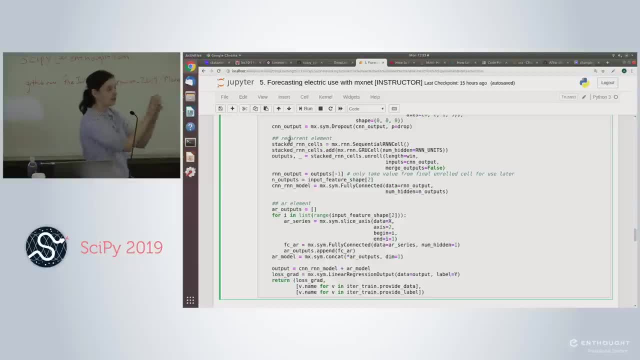 it's almost a way of saying the convolutional component is going to produce features from our raw features. it's going to boil those down to fewer features and then those features are going to go into the recurrent bits that are going to do the feature generation, but some portion of our network. 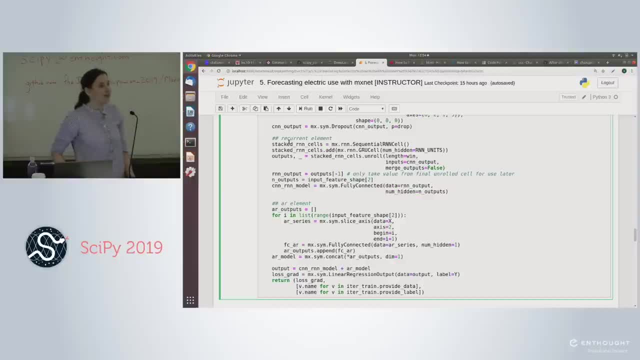 is going to do the feature generation before we feed it into the recurrent neural network. and if you think about that, that makes sense, because why should I be putting in 320 parallel measurements into the recurrent neural network, which then A has to decide how the measurements are related to each other? 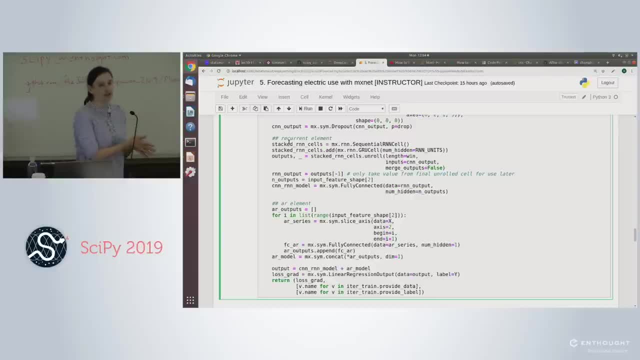 and how they're interesting. but B has to keep track of the temporal component. so if I can sort of shrink down the multivariate aspects so that the RNN can concentrate on the temporal component. now there are two RNN, there are two RNN models, there's one that sort of. 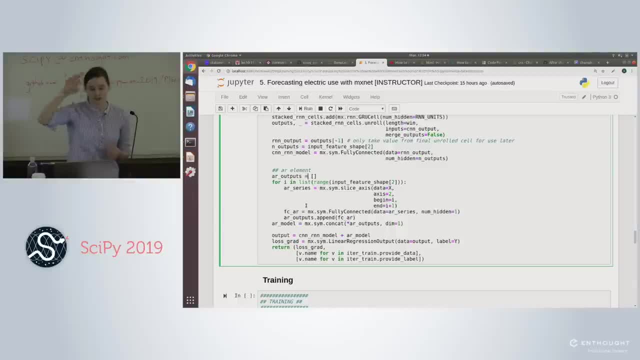 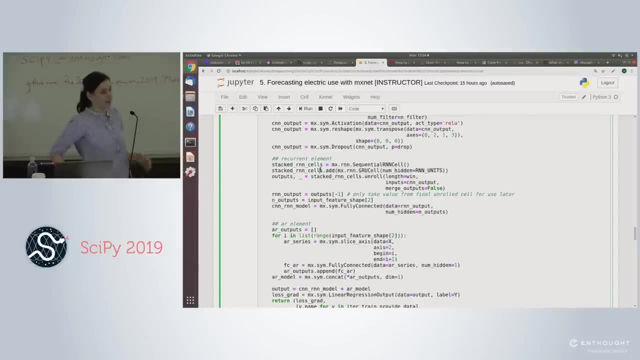 looks at every data point and then there's one that sort of skips seasonality. but here I have left that out and I just have the regular RNN, and the reason for that was I just found that for this particular data set it wasn't especially important. 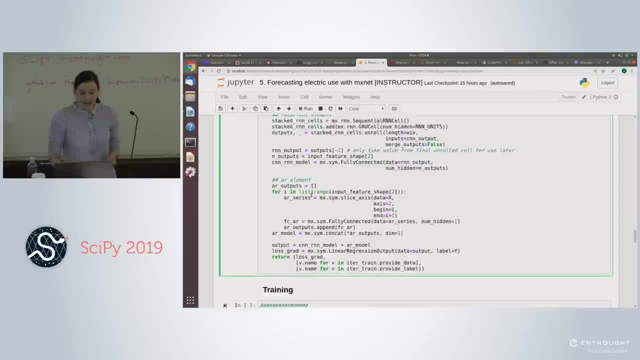 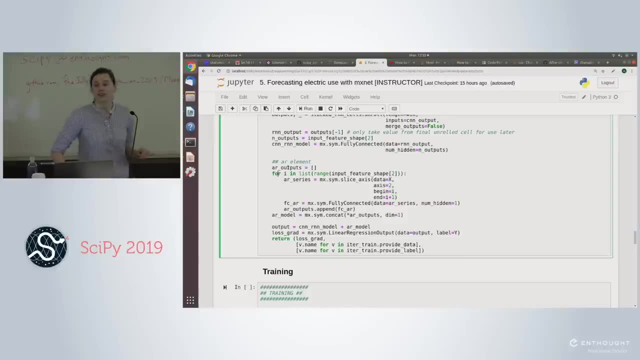 so that's something else you want to keep in mind- is what architecture actually improves your process for a particular model. and then, finally, what I didn't mention is we included an autoregressive element. this is just an element that uses the past values to predict future values. 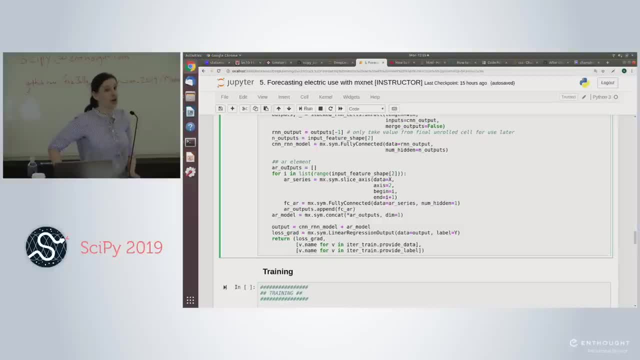 this is the same as an ARIMA model, so actually, what we're seeing here also is combining a statistical approach with neural networks, and this is something that is increasingly common and that has actually proven quite successful in time series in particular, much more than in other areas of machine learning. 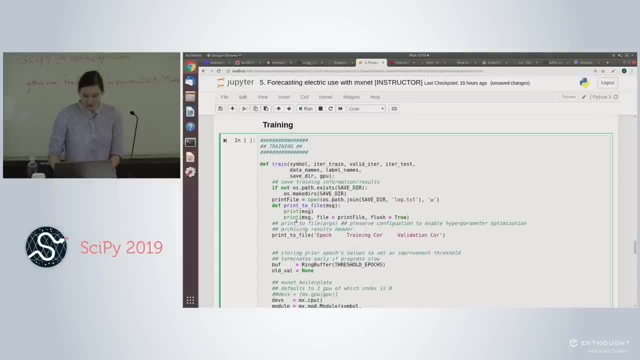 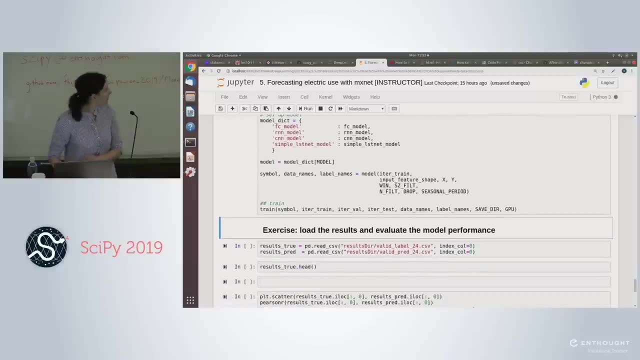 so those are our models. we can define our training and we can run this. let's see, am I running? my screen is well, my screen is frozen, so we must be running, because that's what happens on my rinky dink laptop. obviously you don't usually really want to do. 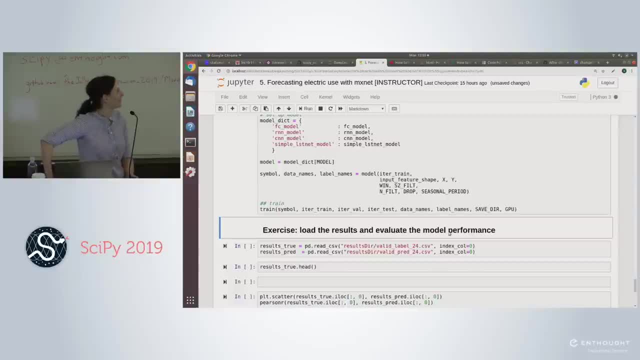 deep learning on a laptop, and you don't usually want to do it on a small data set. so, keeping both of those in mind, let's see. ok, well, I would encourage you to check out the output and experiment with this, but the punchline that I wish we had time to train on, 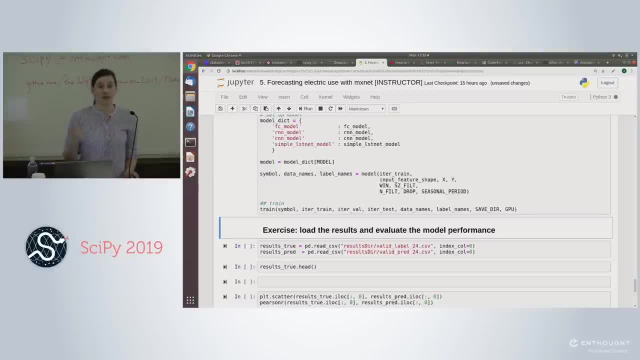 is that the LSTNet model does quite a bit better than the recurrent neural network alone. so it's really important to design structures that are like savvy about how they allocate the labor. so in this case, the labor of the convolutional bit, the feature generation, is separated out. 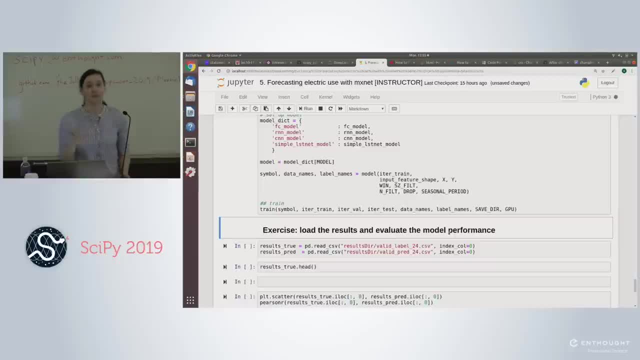 from the temporal analysis. that's one thing that makes this model really successful. the other thing that makes this model really successful is the inclusion of this AR component, the autoregressive component, and in fact, if you remove that component, you take an enormous hit to performance. so this, I think, is great inspiration. 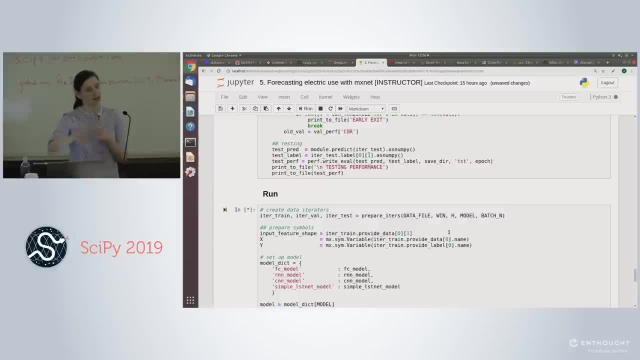 for how you can take your traditional statistical knowledge and work it into your neural networks, and you will find that that gets you a really great outcome, and in fact so. most recently there was an academic research competition on time series forecasting, and both the number one and number two. 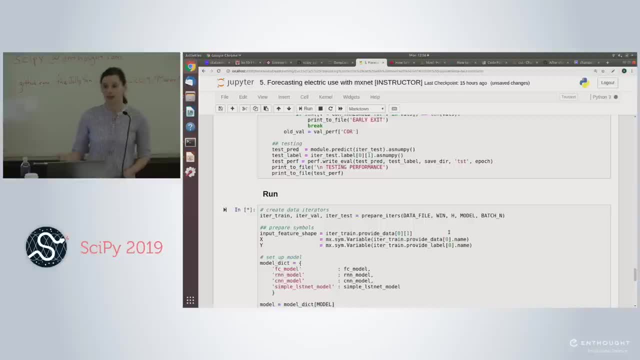 winners of this competition, which took place on 100,000 different time series over many domains, and they were really integrating machine learning and statistical analyses that are quite traditional, in one case combining statistical analyses with deep learning, and then another case using XGBoost to choose the coefficients. 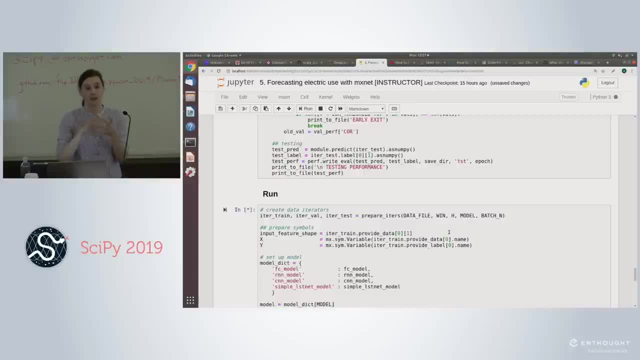 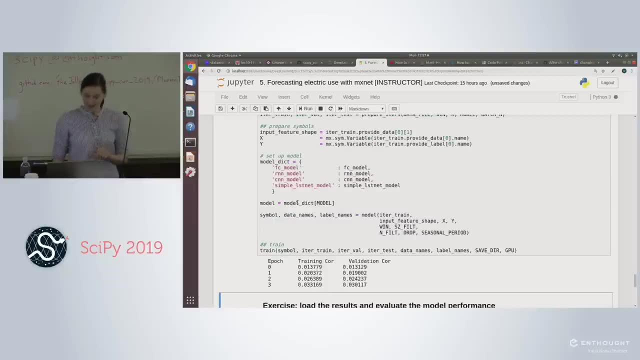 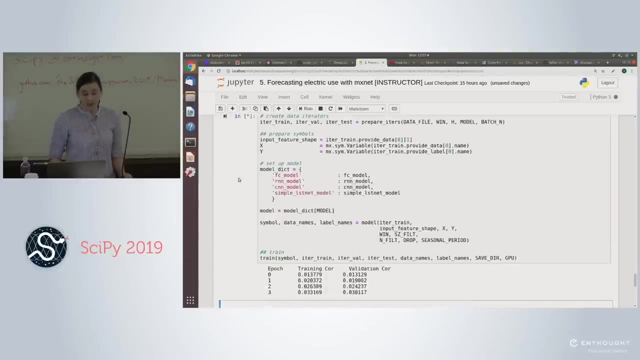 to combine statistical models, so also the ways that you can sort of permute these things are quite varied. gosh, I could have sworn, this ran faster when I was. oh, here we go, okay. so in this case you can see, I'm printing out the correlation- which metric you like. 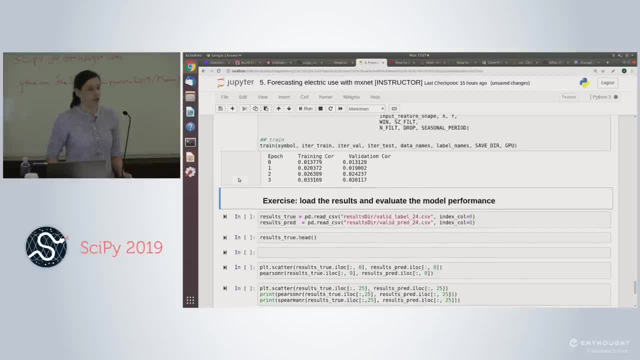 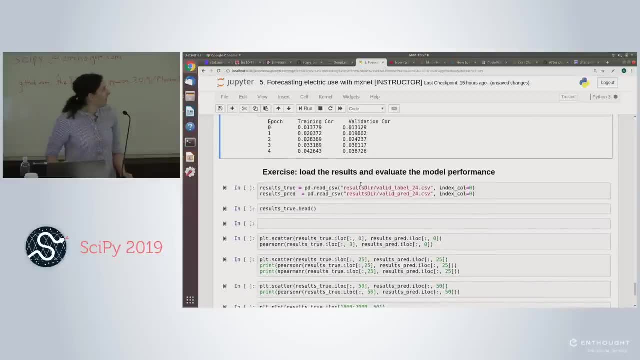 can be a matter of personal preference. it can also be a matter of what is meaningful for your problem, but basically, what we want to see here is that it's improving, especially on the validation. I think we will stop it here if we can. yes, okay, so stopped it here. 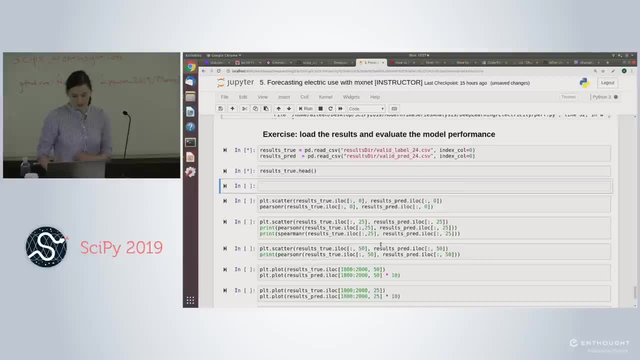 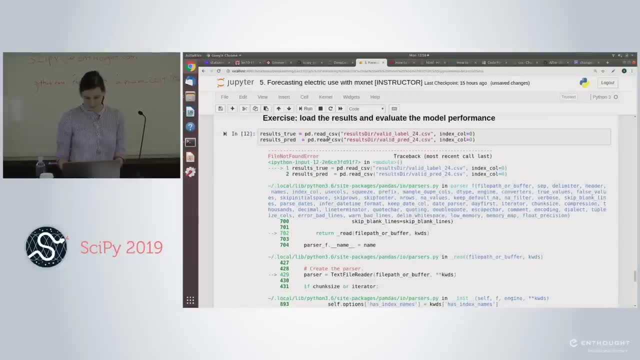 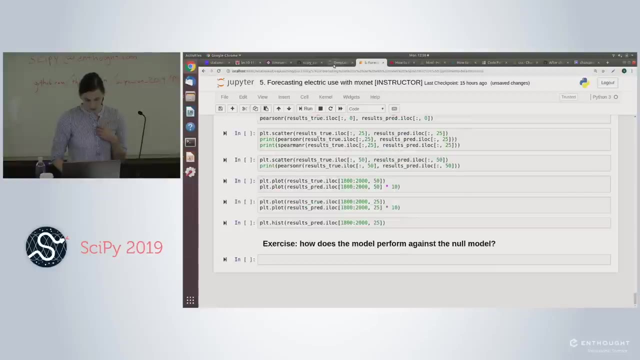 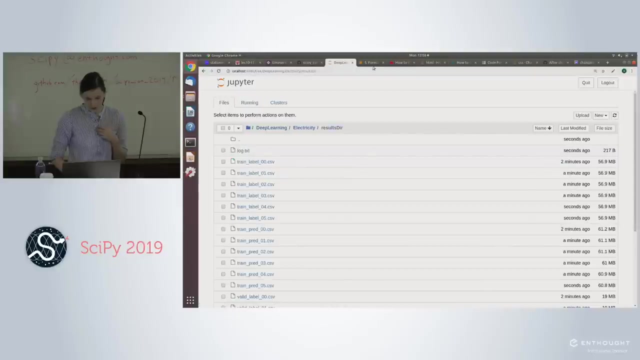 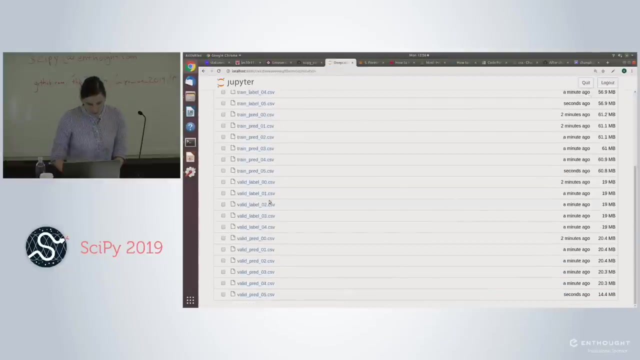 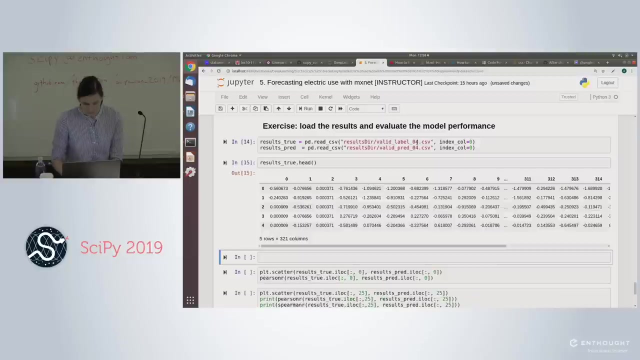 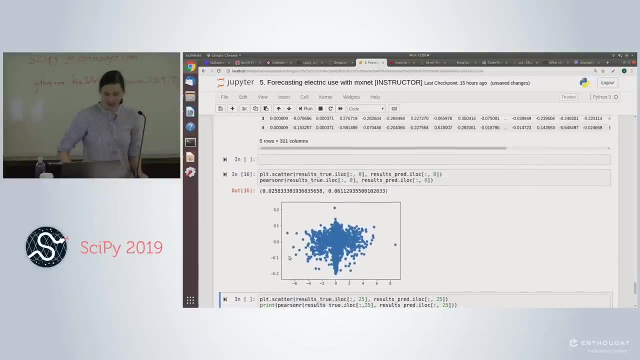 I also have the results from the last time I ran this already loaded. no, no, no, I'm lying. oh, I see, because I only went up to five. okay, let's do this. okay, so in this case, we can see what we're looking at after only four iterations and we can see. 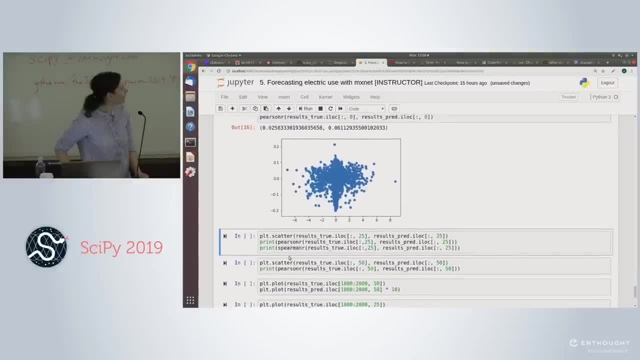 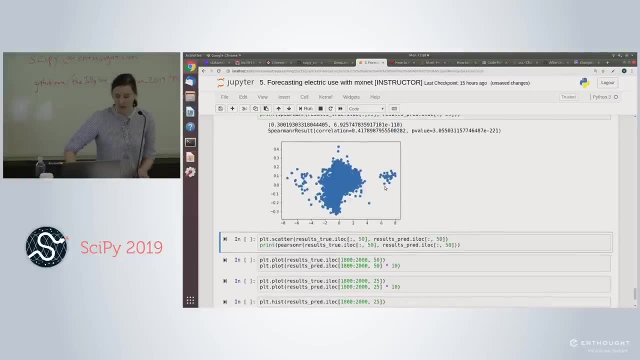 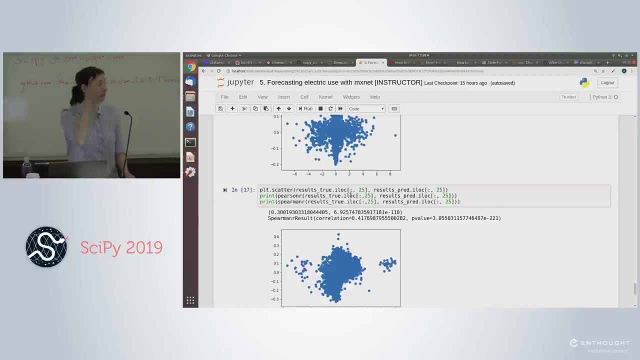 so far for this first column, it doesn't look especially fantastic. let's look at this column, quite different right, and this actually looks a little bit more promising, especially if we ignore outliers. but we can see here that we've actually managed to fit many time series right. we're fitting 321. 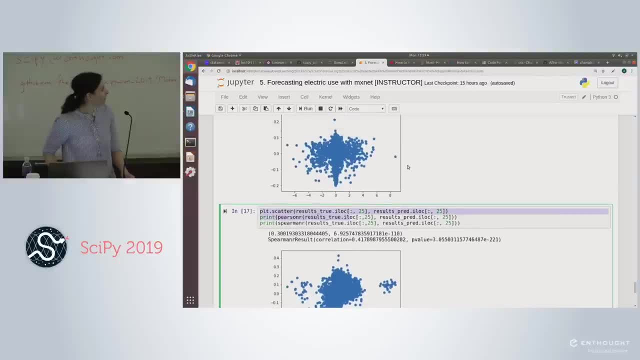 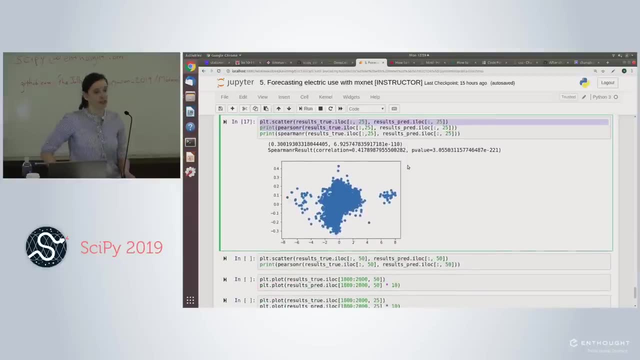 time series in parallel with one generalized model, and so we can sort of expect results to vary between one and the other. so if you let this go for about 20 to 25 iterations, you get really excellent results, but not after five epochs. so I'd encourage you to keep this running on your own computers. 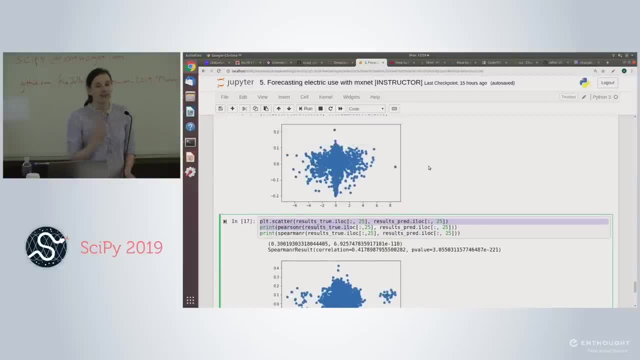 but takeaways here are: this is not even an enormous time series data set. right, I can fit this all in memory on my rinky dink laptop. so I actually, in my experience, have found that deep learning works even better than like sort of regression trees and things like that for cases. 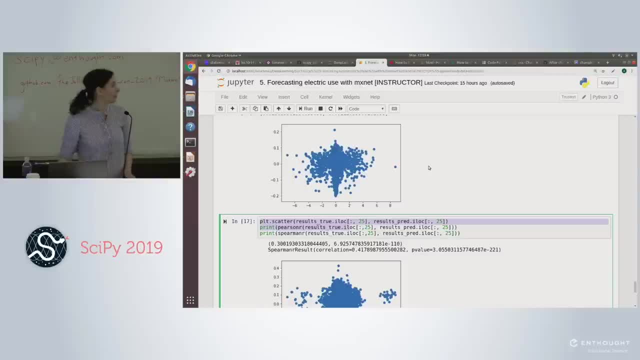 of small-ish but not tiny data sets for deep learning compared to statistical models, and also that you want to be creative about combining your statistical models and your deep learning. so this is where you see, especially for time series analysis, having a broad domain knowledge of many different sort of classes. 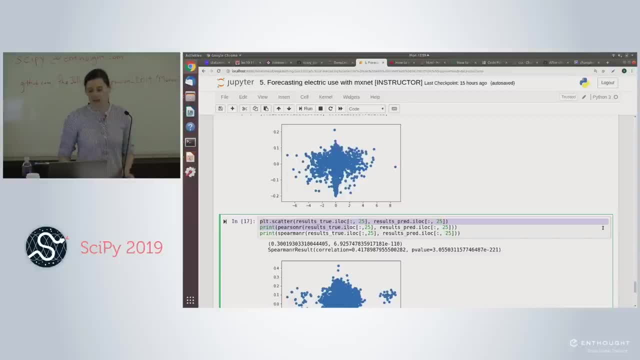 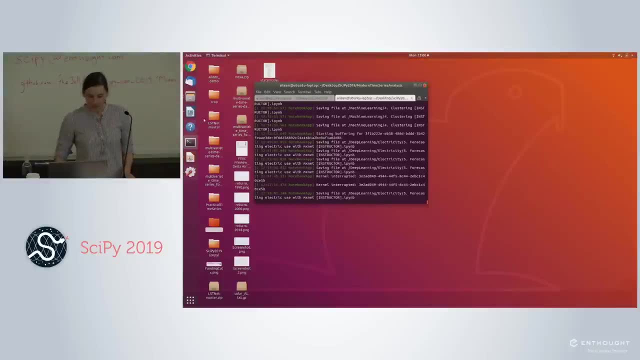 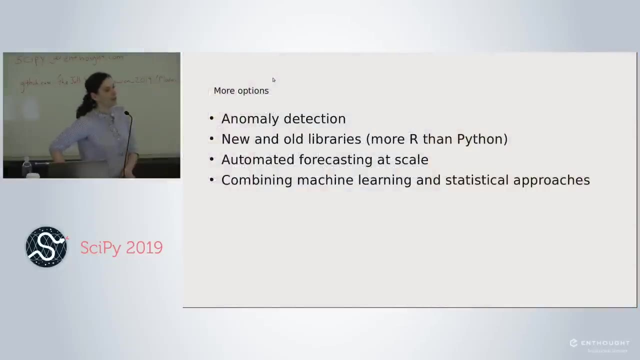 of analysis will also help you to build more creative models. so even when you want to do something more cutting-edge like deep learning, having that traditional knowledge will really help you. okay, so I have one slide to wrap up, because I did want to talk about okay, so just to wrap up. 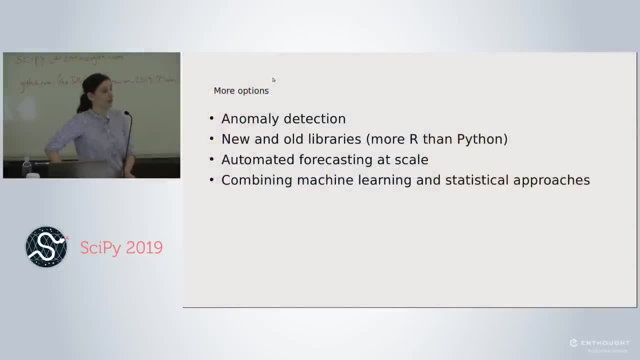 to highlight some things that we haven't talked about but that are important also as being on the horizon or just active areas in modern time series analysis, I think the huge one that we didn't have time for but that you can very much address with what we. 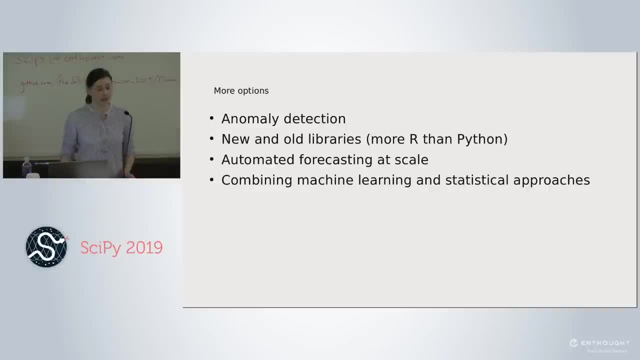 talked about today is anomaly detection, right, so maybe even some of you work in this field. um, things like structural time series, hidden markov models, uh, regression trees, xg, boost and deep learning can all be applied to the question of anomaly detection. so anomaly detection is not something where you need one specific. 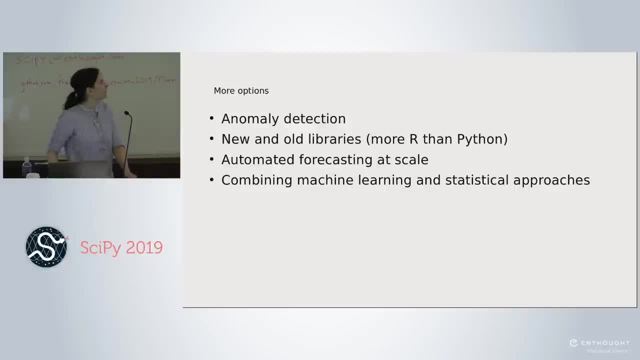 technique. actually, all of these are available to you and may even be combined successfully. there's also so many new and old libraries for time series analysis, especially for more modern methods. there are literally hundreds of packages. um, definitely, this is an environment where R's options are richer than 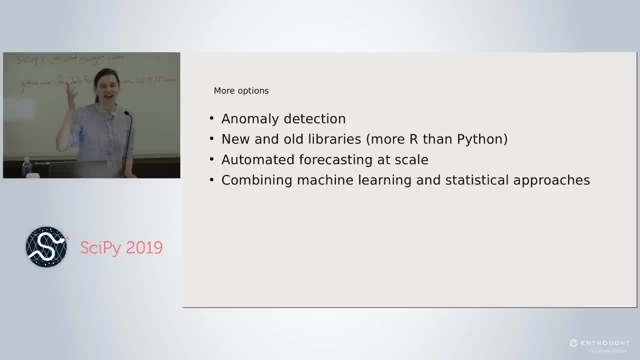 Python. so you might also want to get more comfortable, especially like with at least being able to access R packages through Python, to have access to those um. time series analysis obviously is an area of active research both in industry and in academia, but most people who are doing cutting 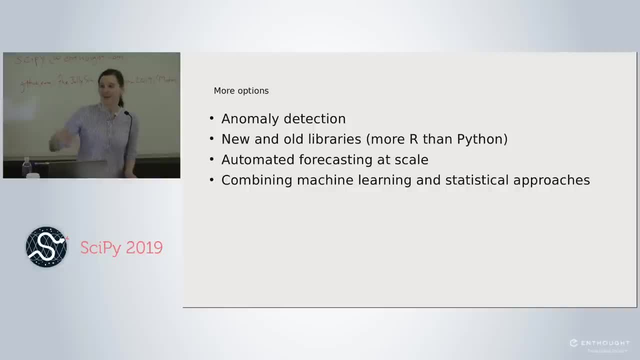 edge research work in R. so I'm a bit of a downer on that front- that if you want to have access to those methods, you also want to be looking at the R ecosystem as well as the Python ecosystem. and then the two things I would highlight that we didn't talk. 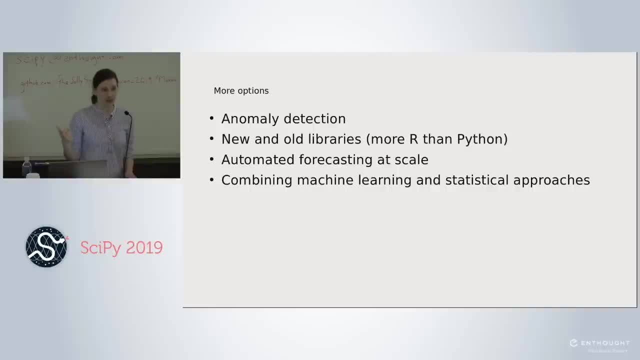 about. but you would also want to look into is automated forecasting at scale. so somebody had brought up Facebook's profit package. there's also a Google package, there's also a Twitter package. I'm probably forgetting some others, but there are some massive tech companies- Uber- looking at really massive data. 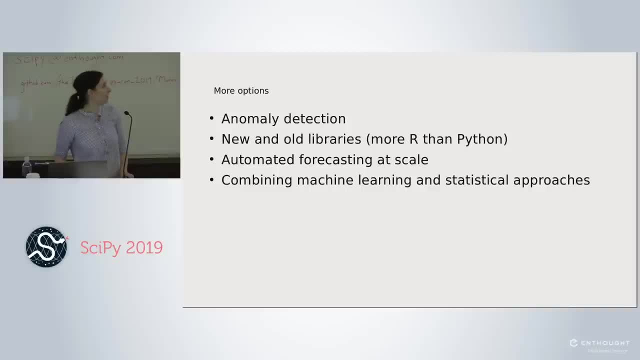 sets of time series developing ideas for their own research and then sometimes either open sourcing them or sometimes offering forecasting as a service. so an example of that is Amazon now offers via AWS is offering forecasting as a service using sort of their expertise at their at their own data right. so if